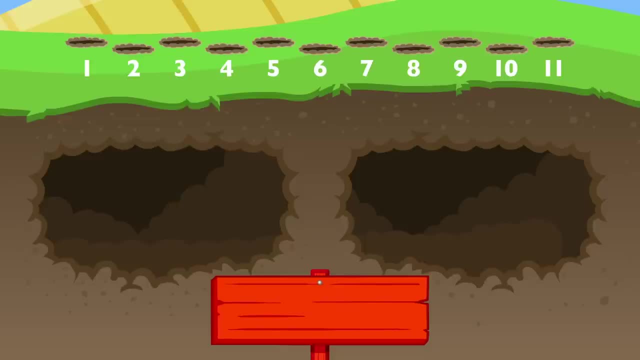 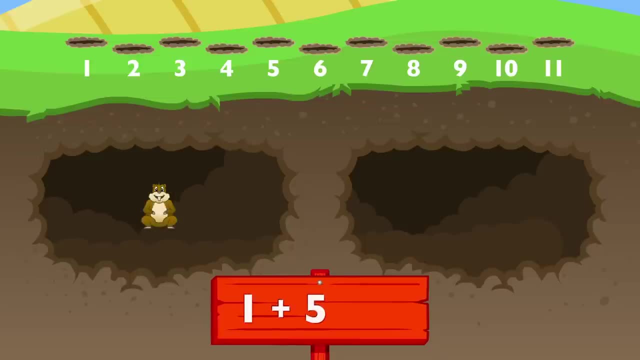 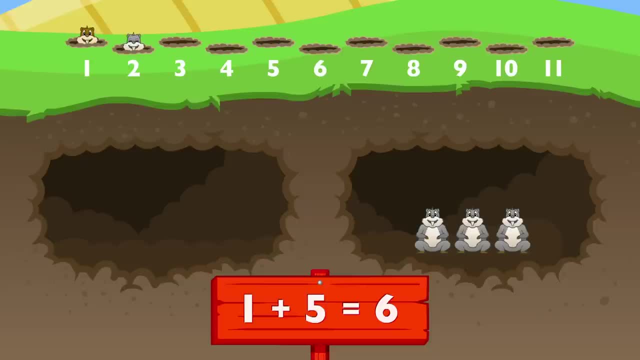 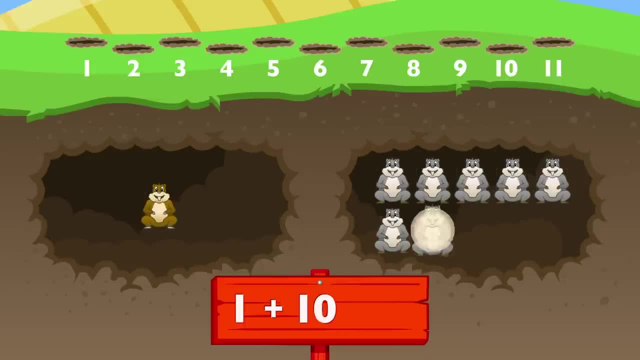 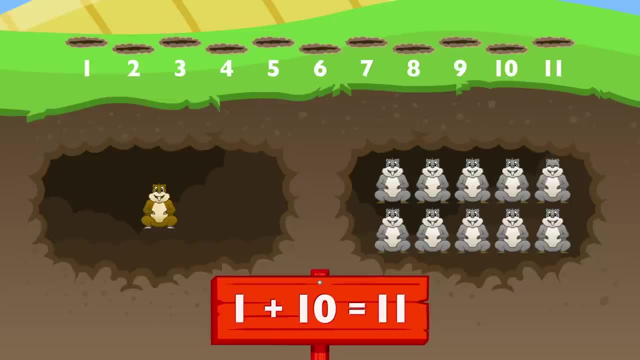 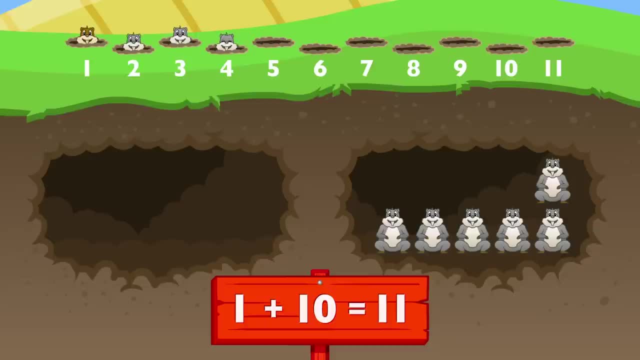 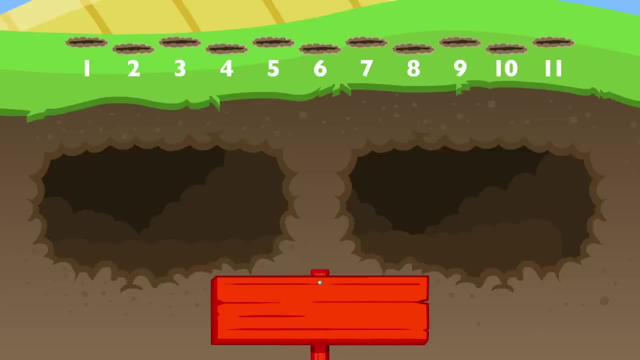 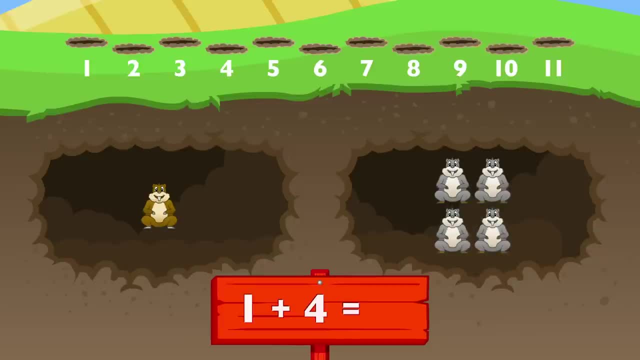 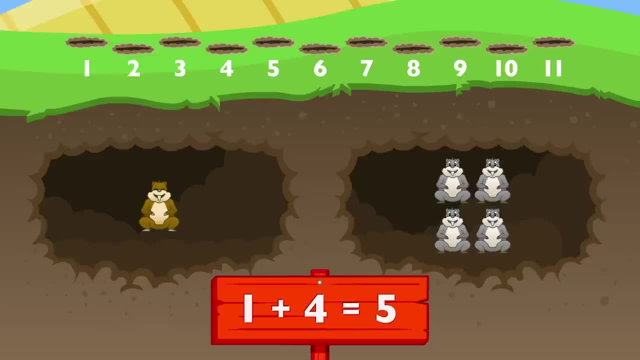 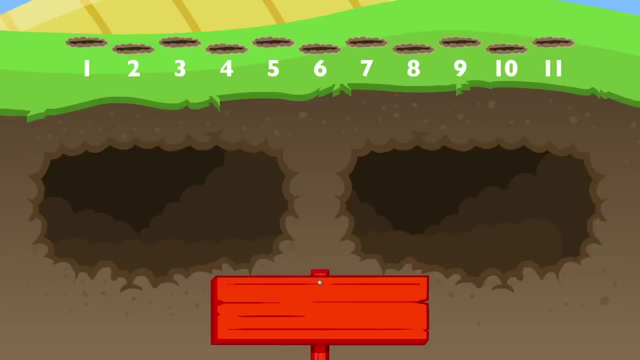 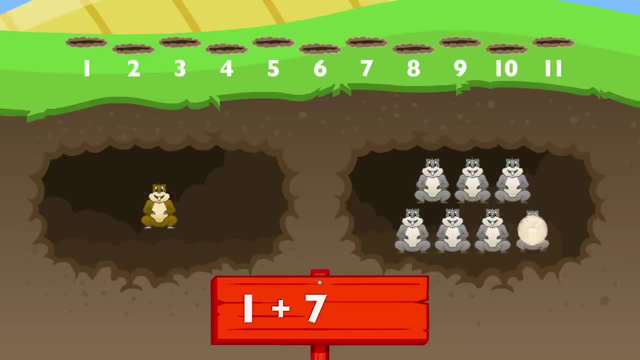 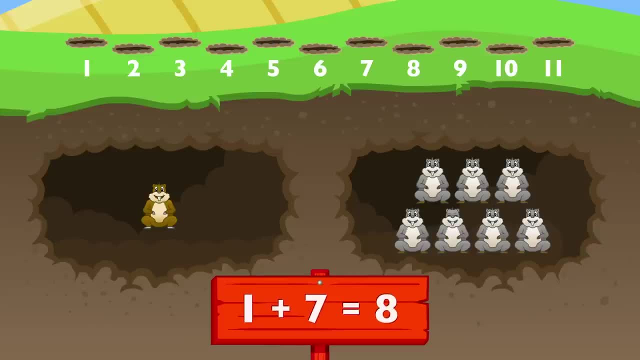 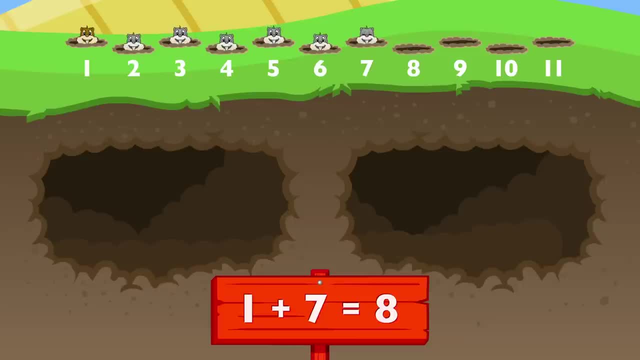 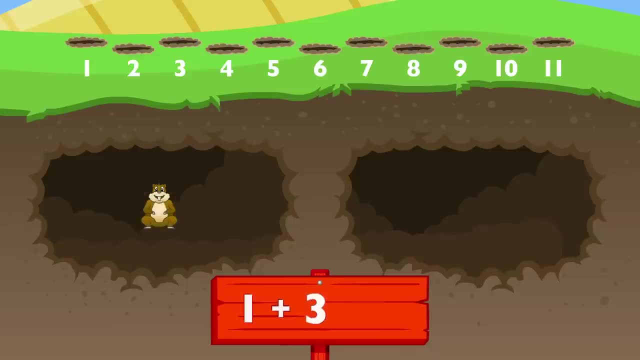 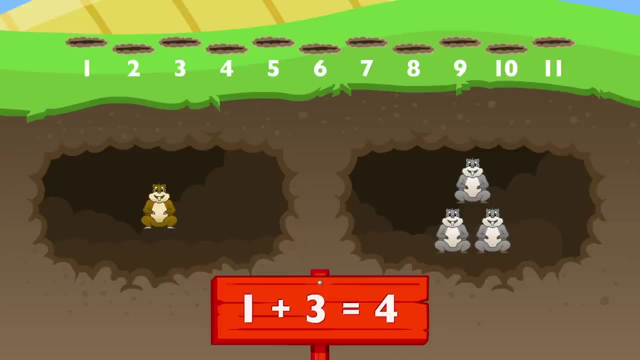 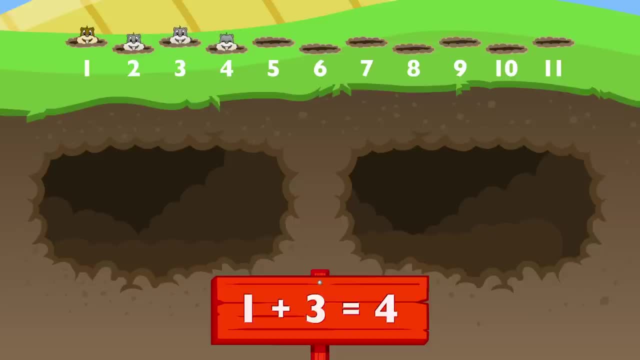 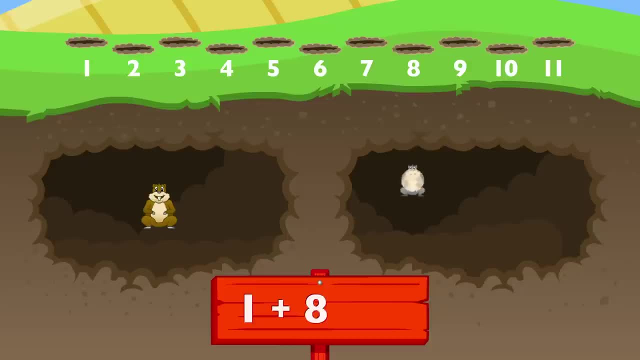 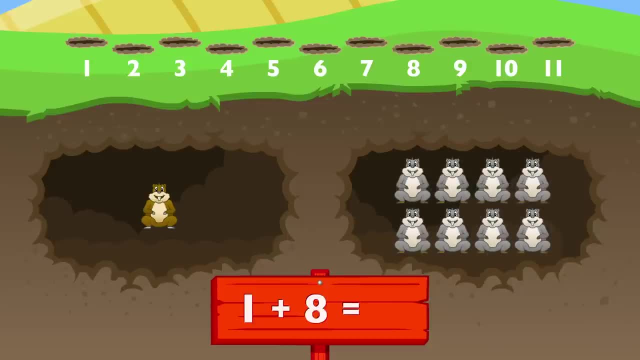 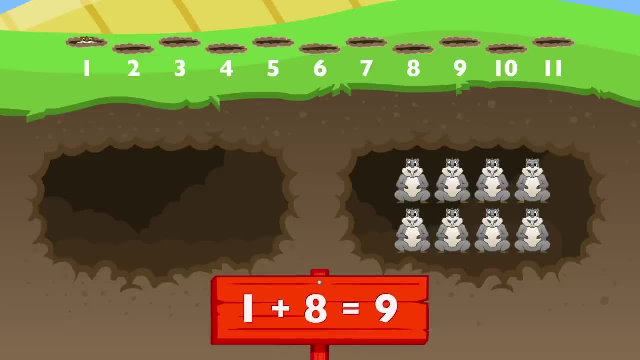 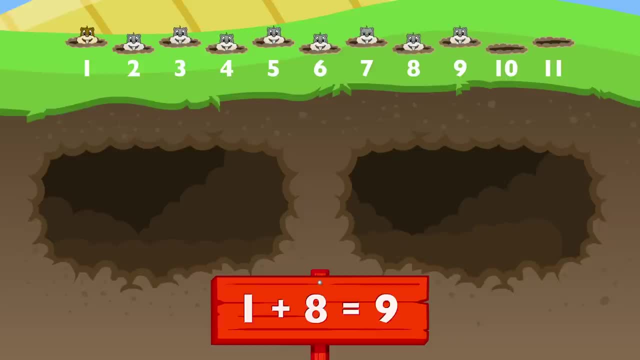 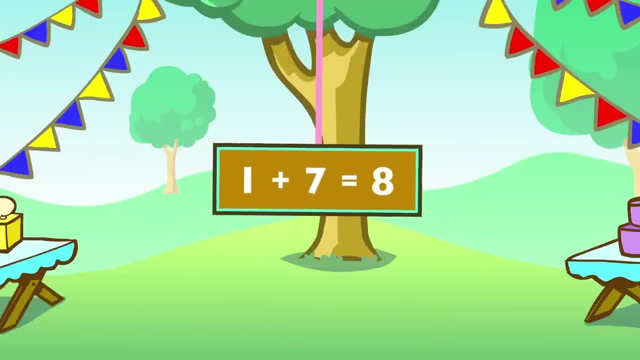 1 plus 1 equals 7.. 1 plus 1 equals 7.. 1 plus 1 equals 8.. 1 plus 1 equals 8.. 1 plus 1 equals 9.. 1 plus 1 equals 7.. 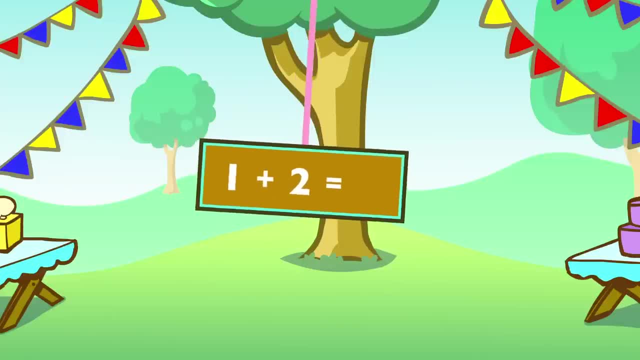 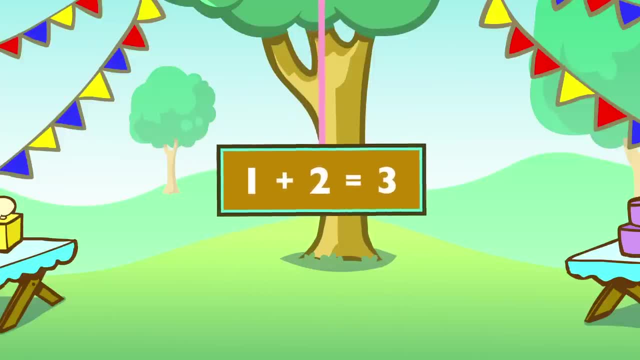 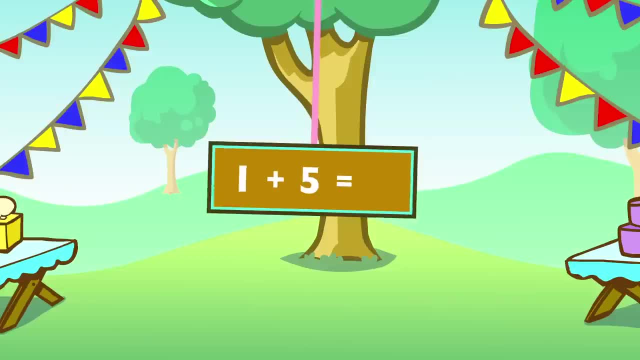 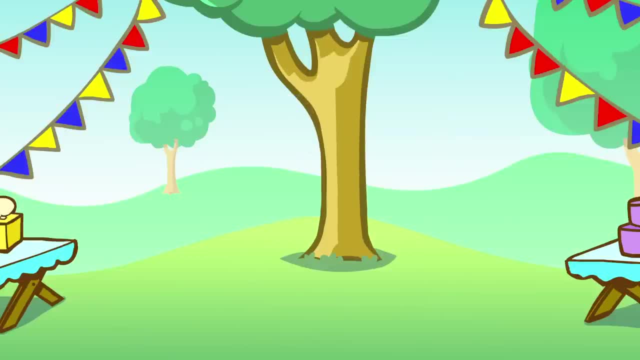 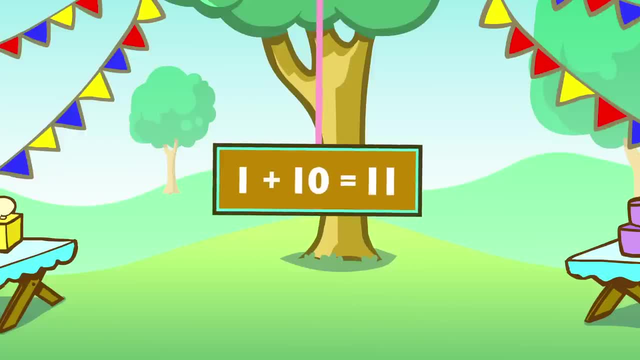 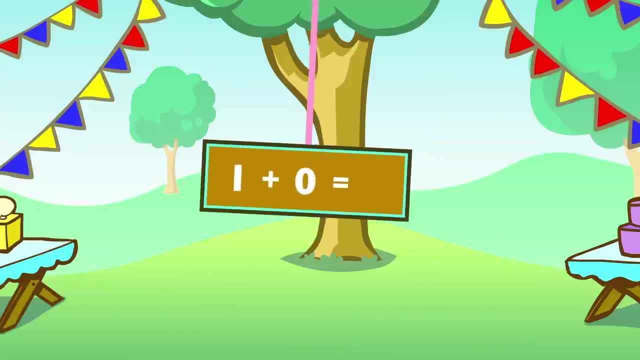 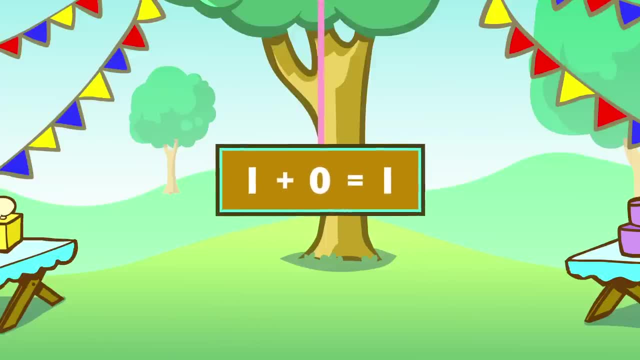 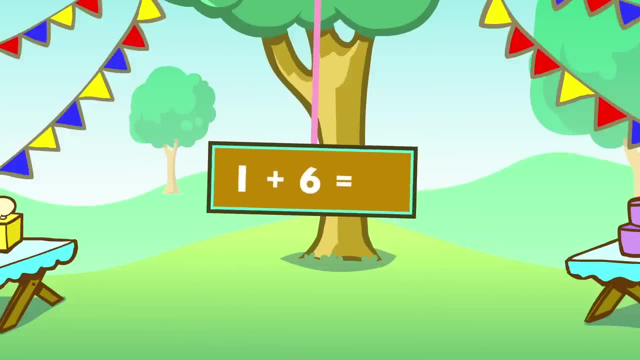 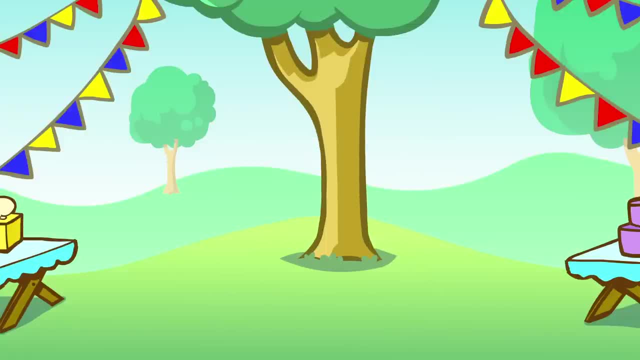 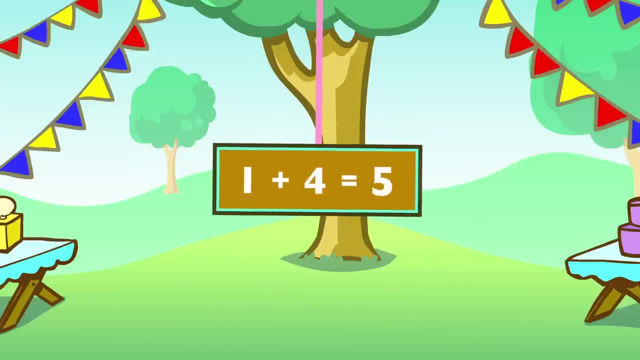 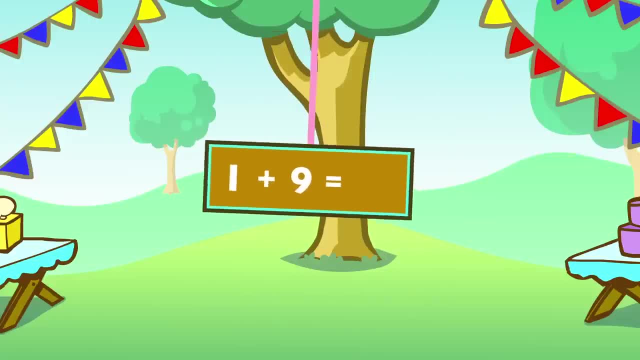 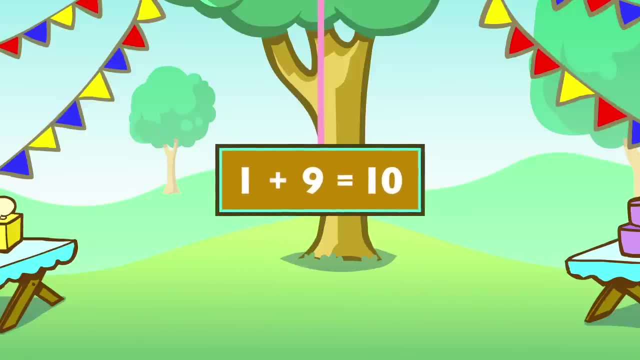 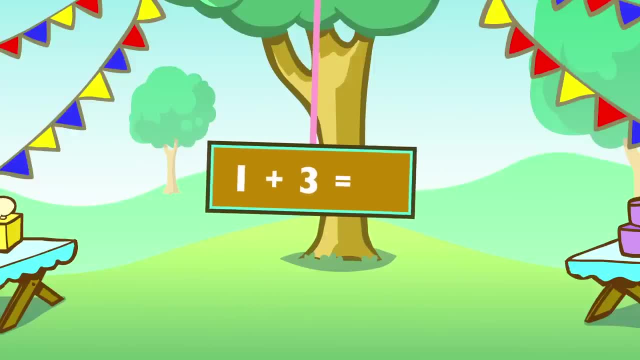 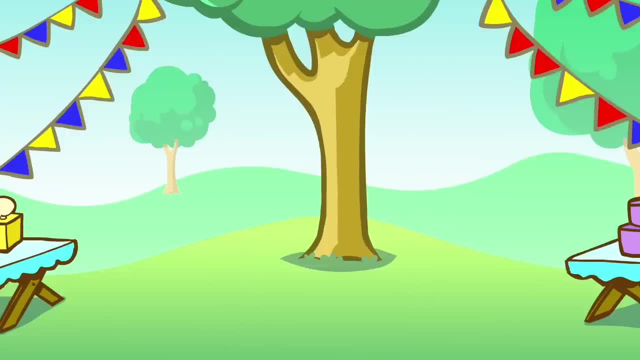 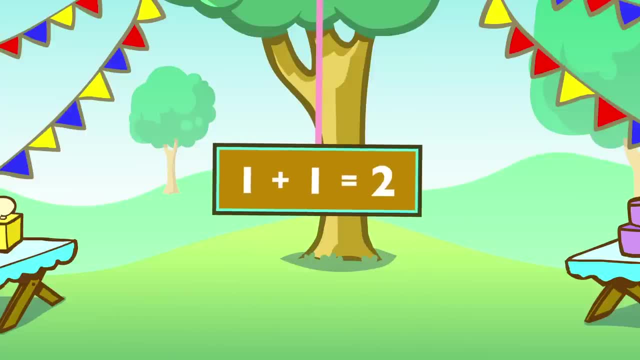 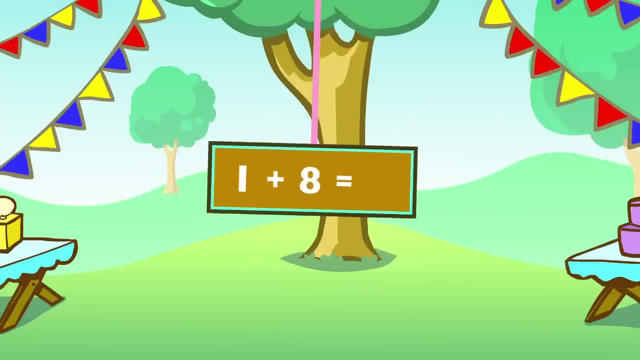 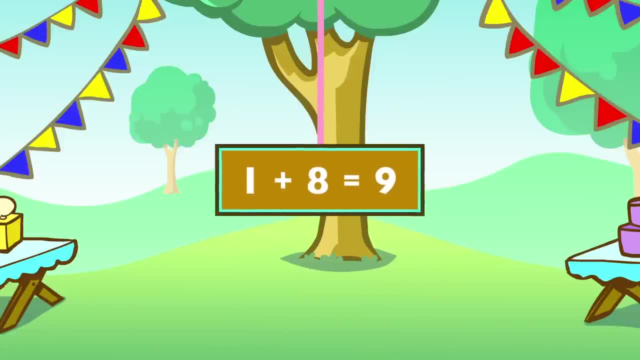 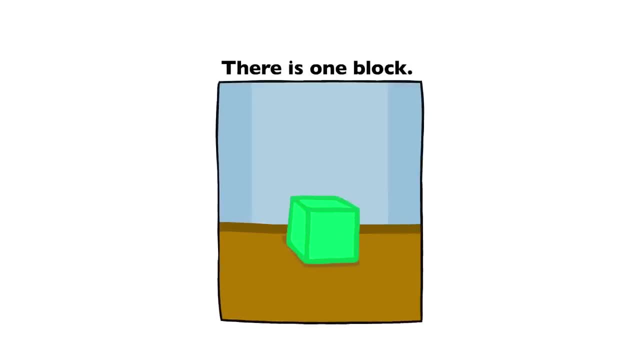 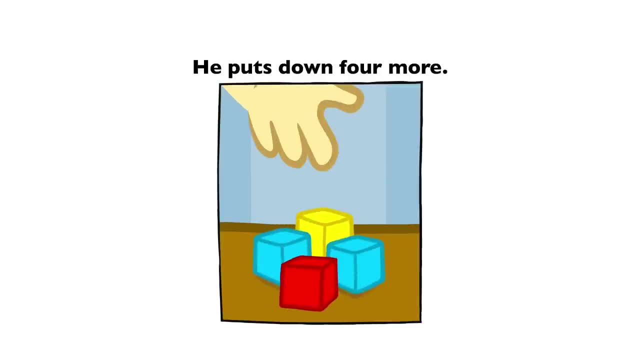 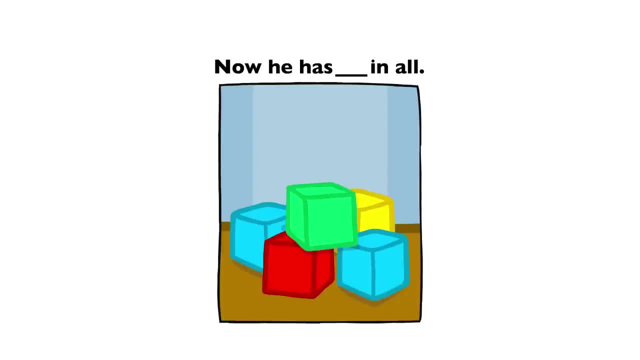 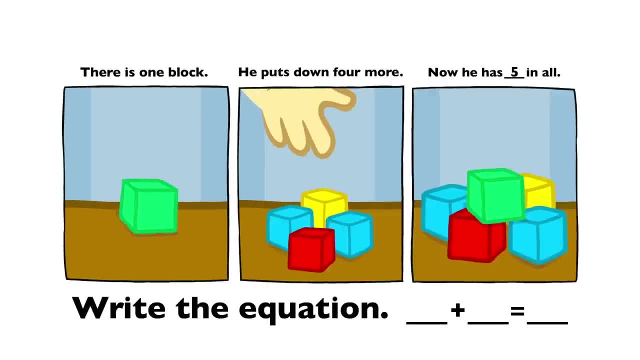 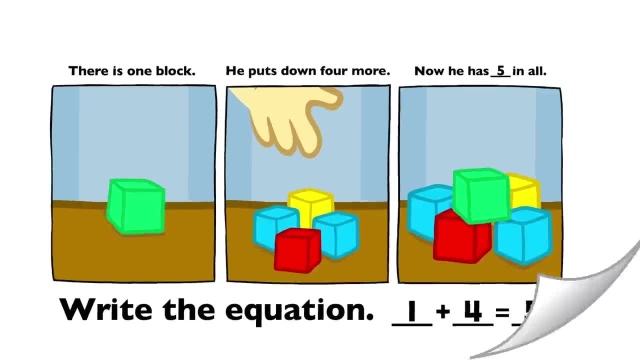 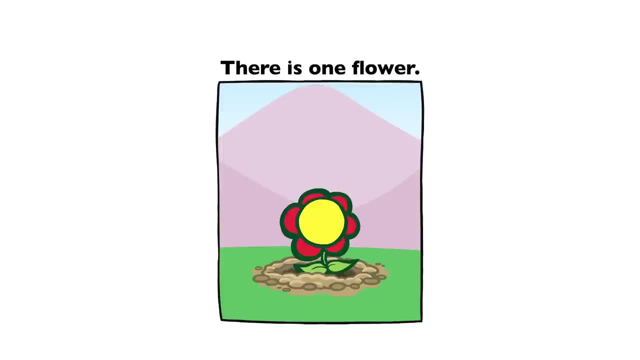 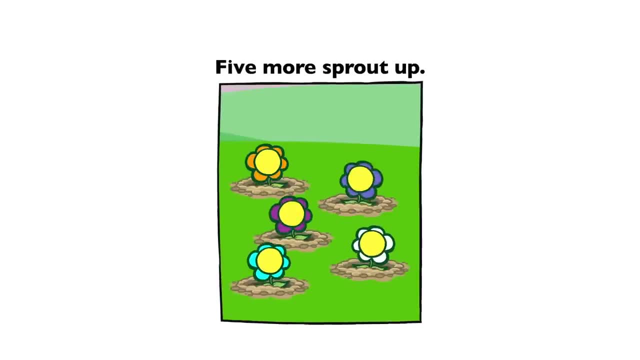 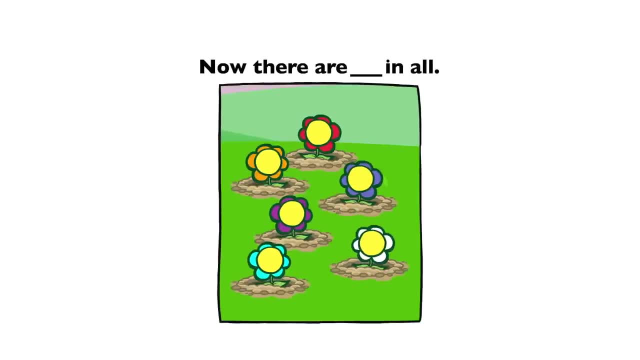 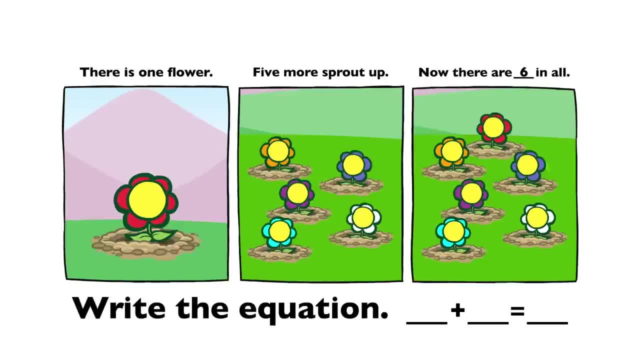 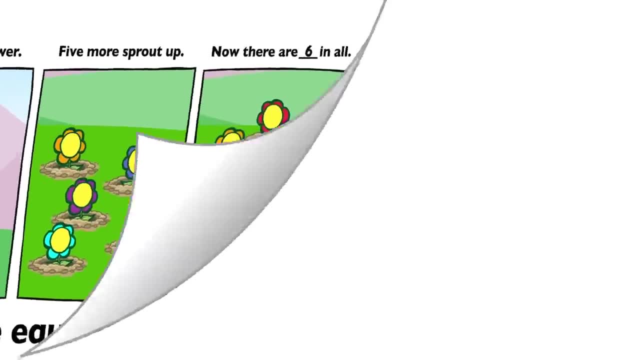 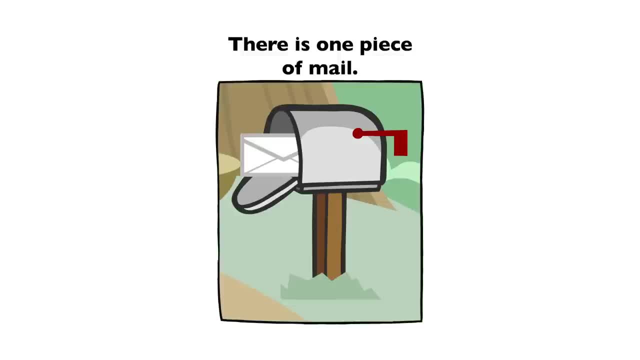 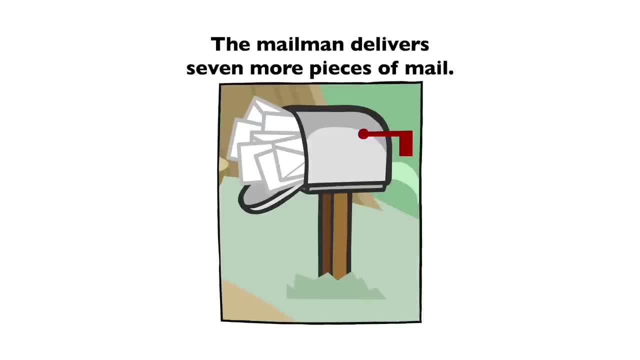 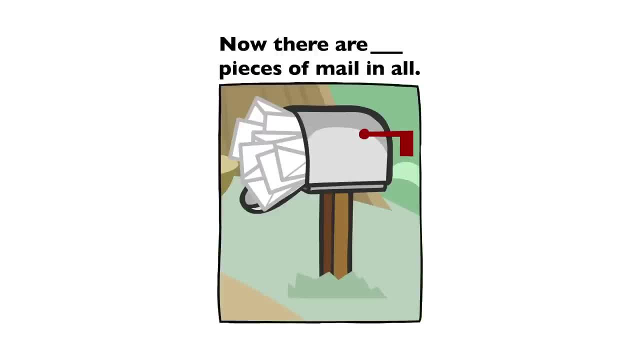 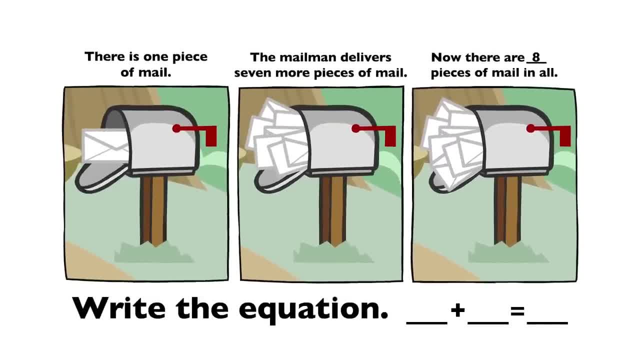 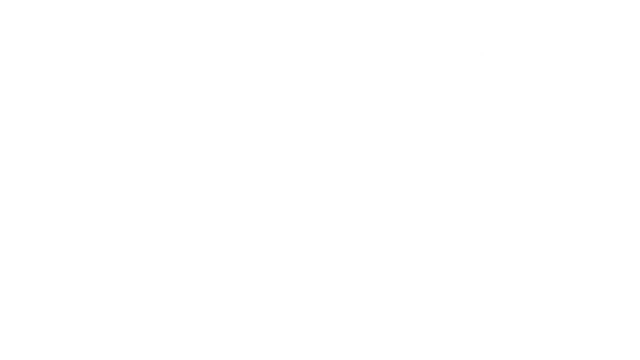 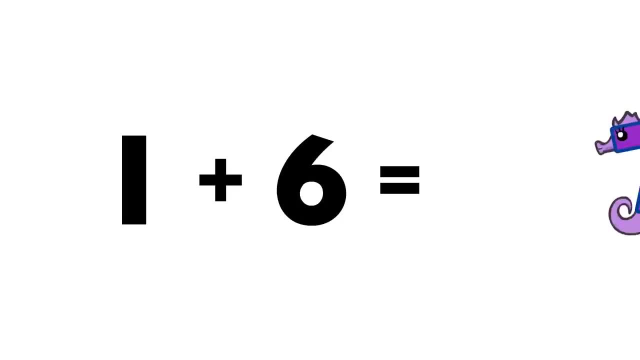 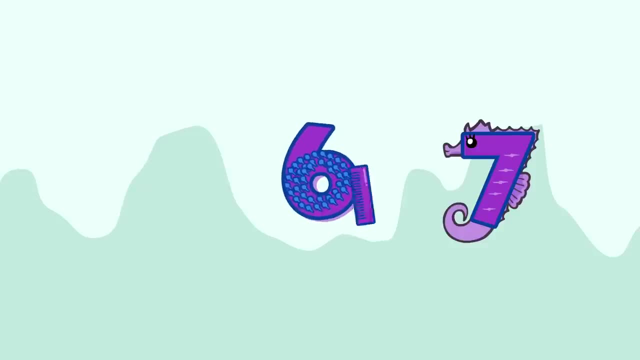 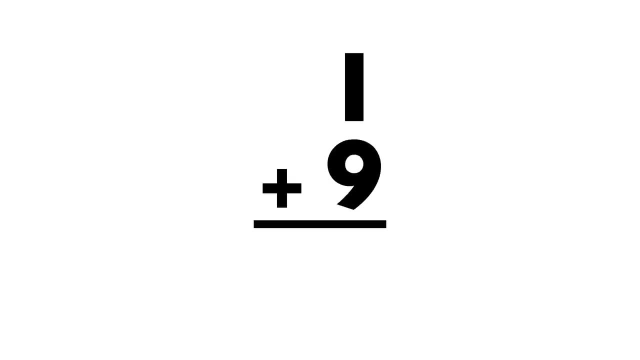 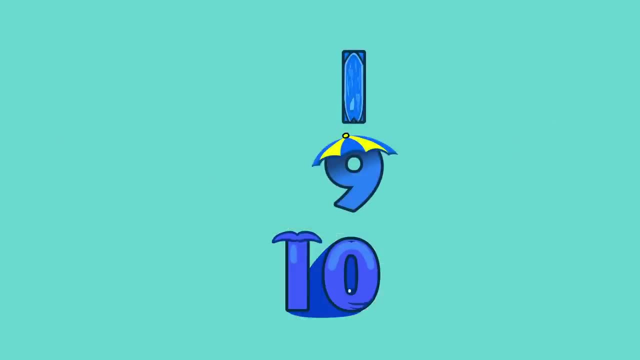 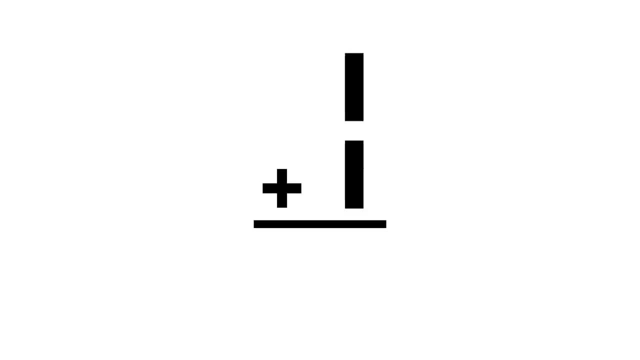 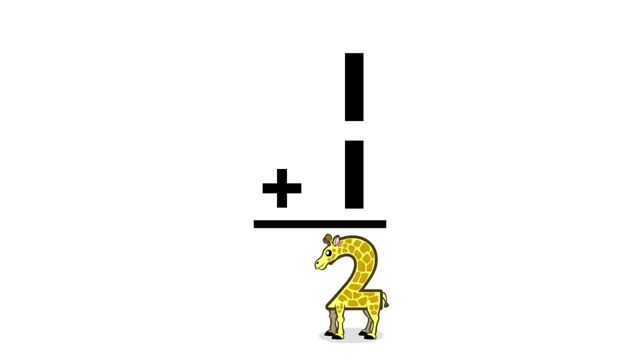 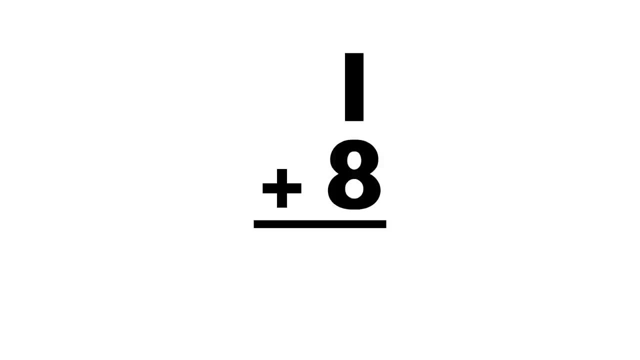 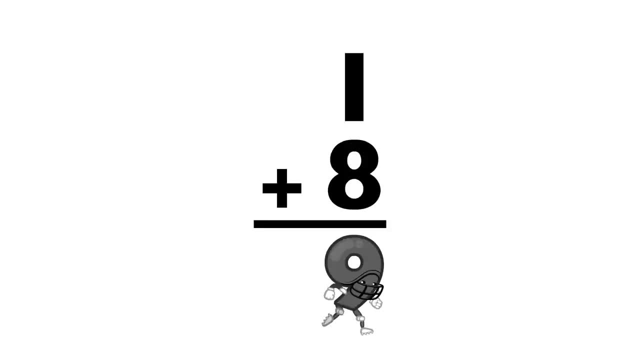 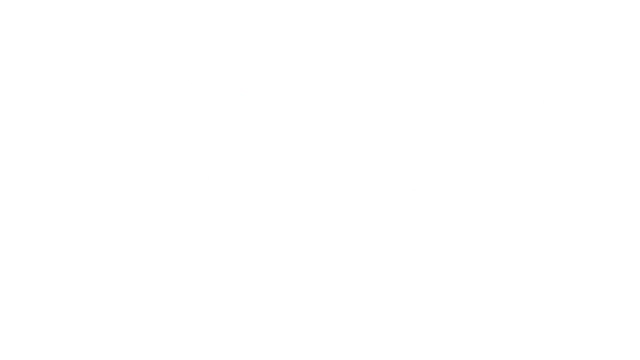 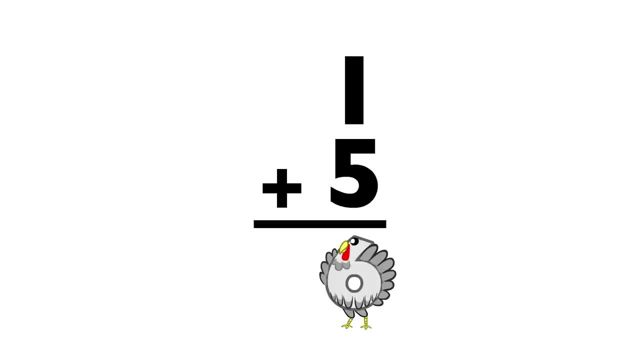 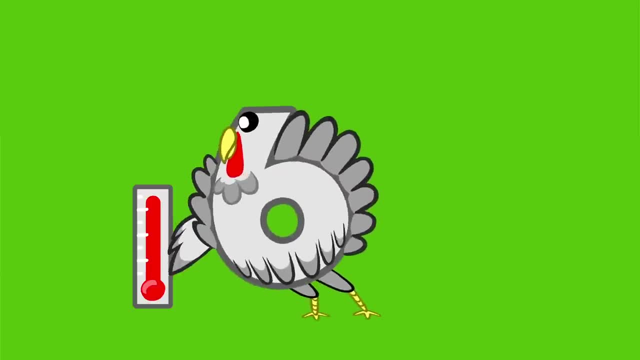 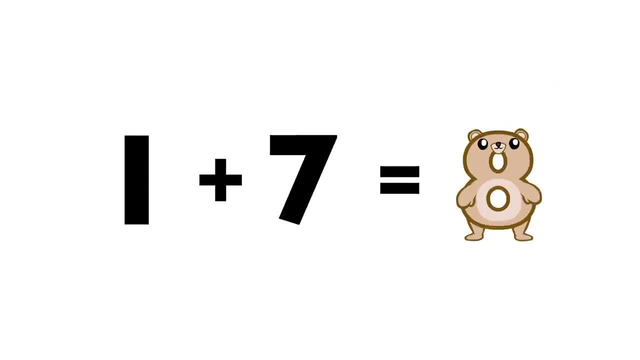 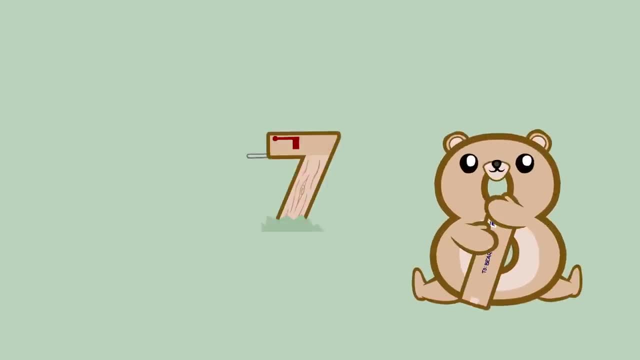 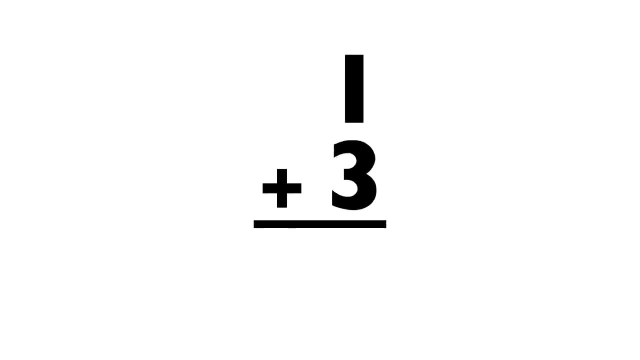 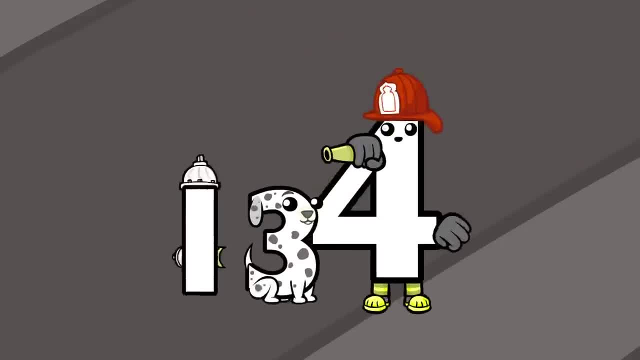 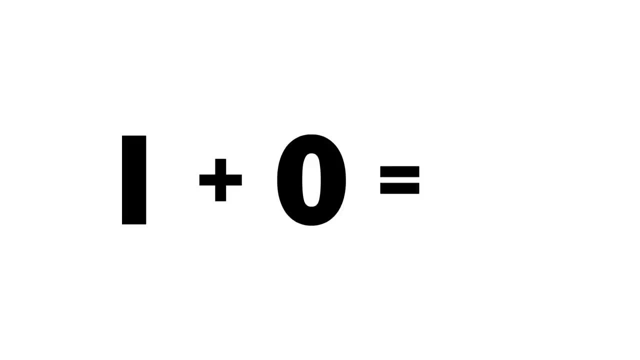 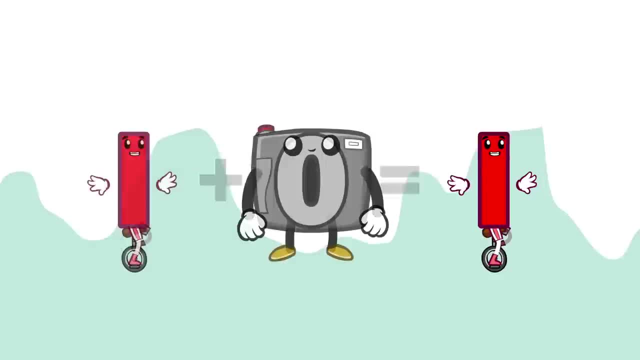 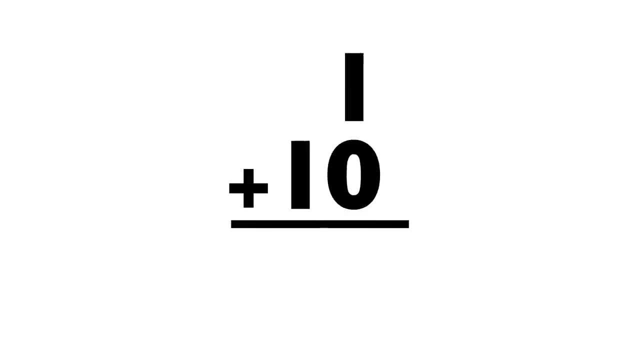 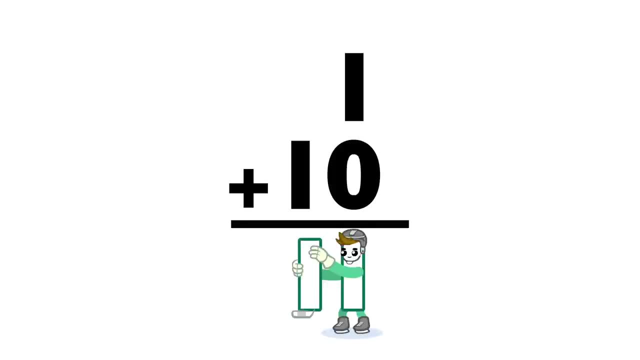 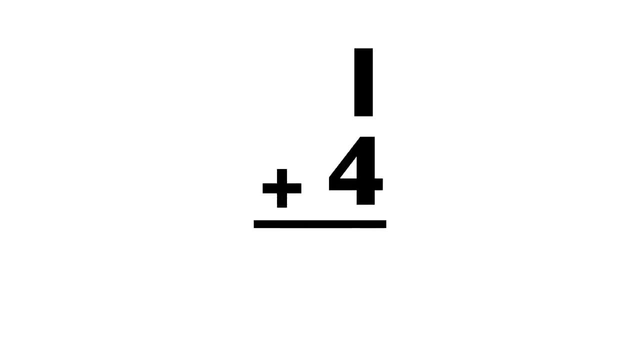 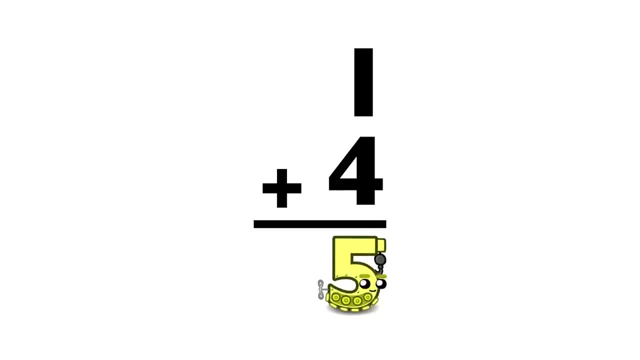 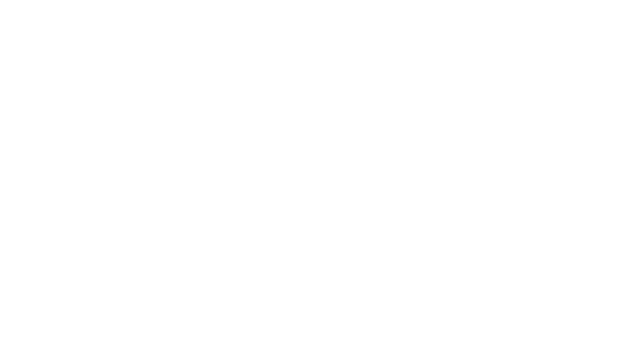 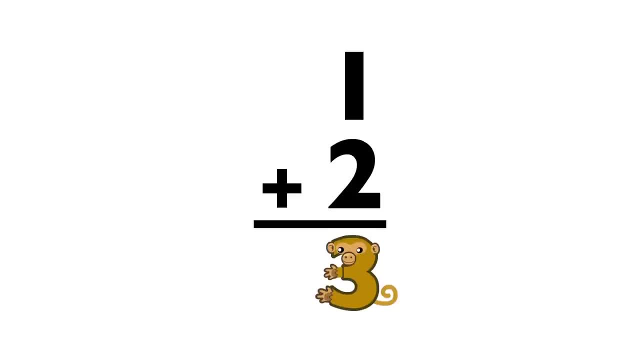 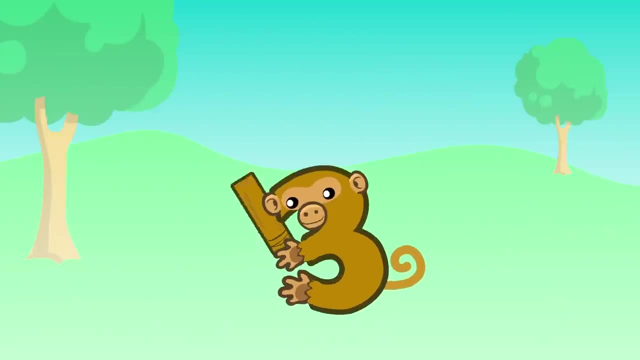 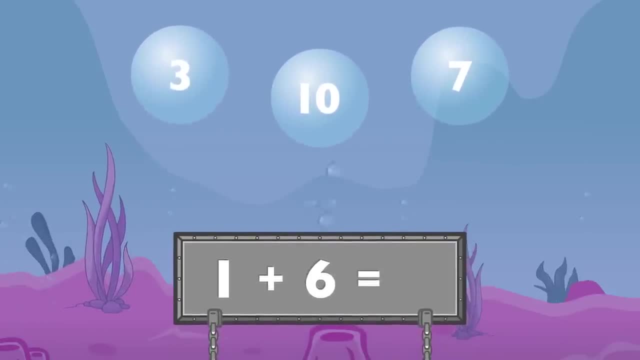 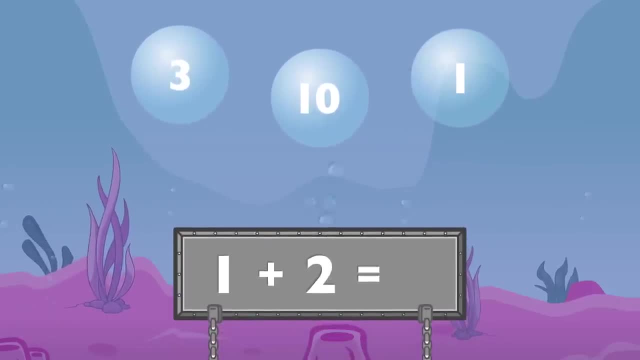 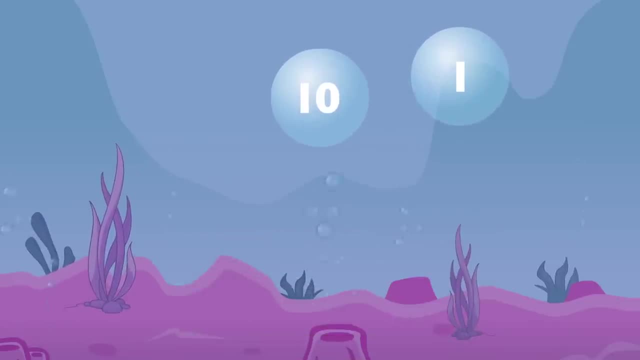 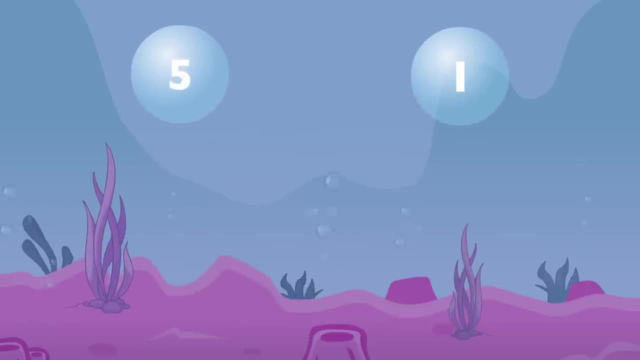 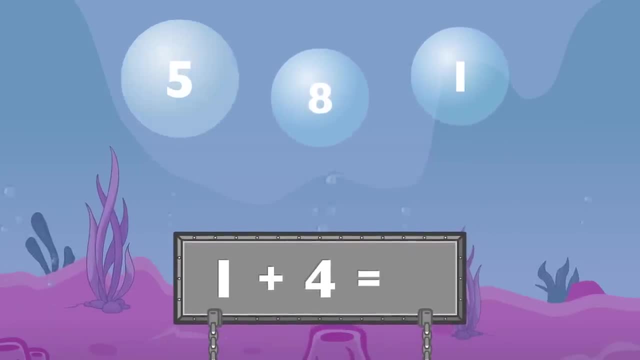 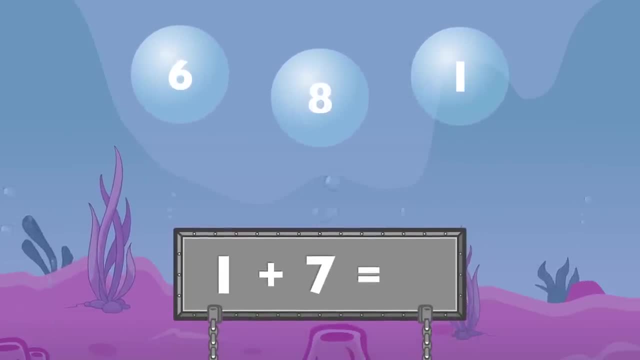 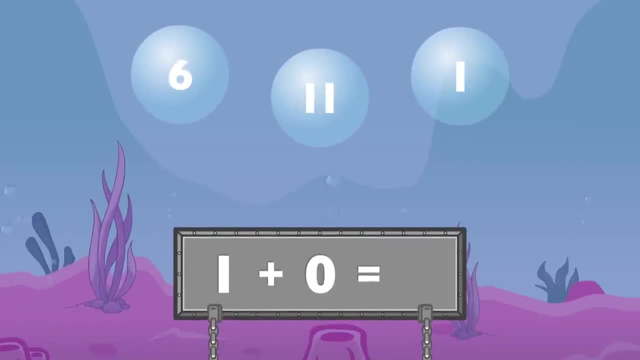 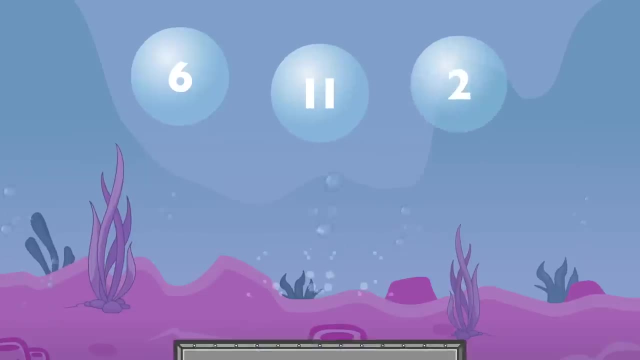 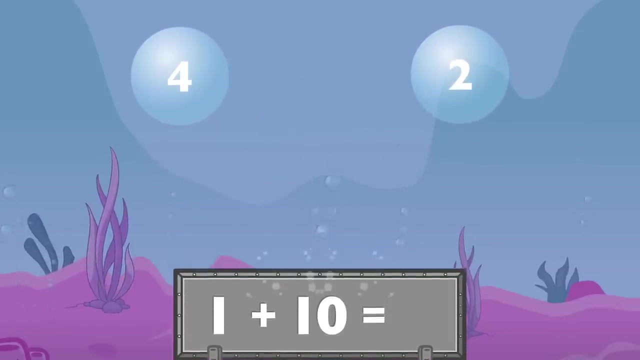 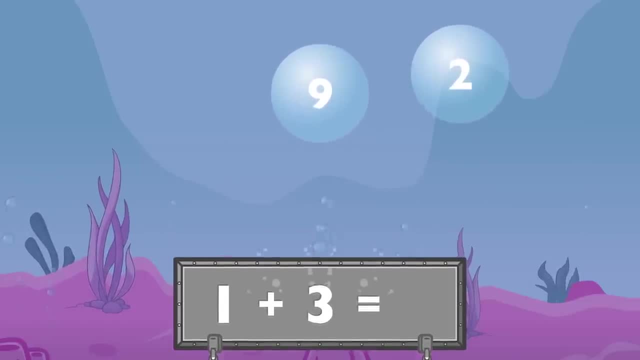 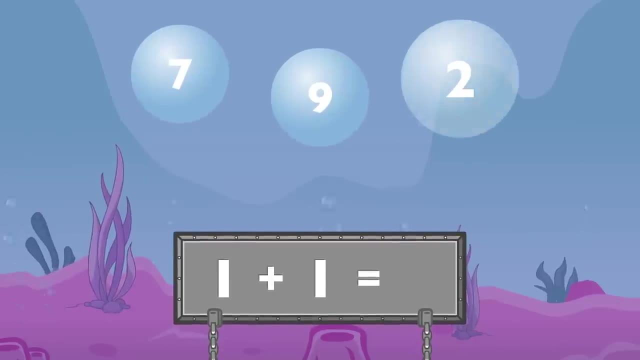 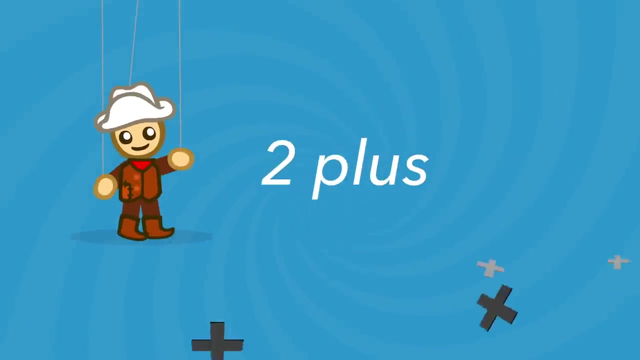 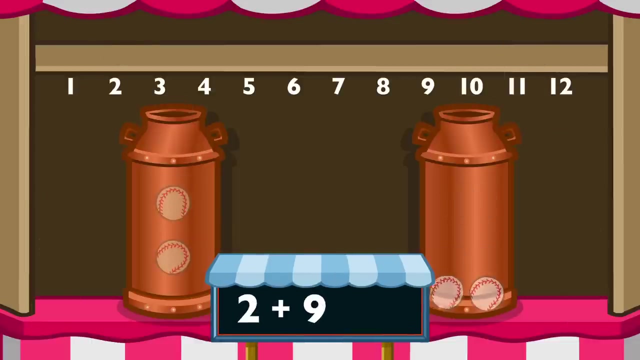 equals four. One plus one equals two. One plus eight equals nine. Speaker 2. Speaker 3. nine equals eleven. Two plus nine equals eleven. Two plus three equals five. Two plus three equals five. Two plus five equals seven. 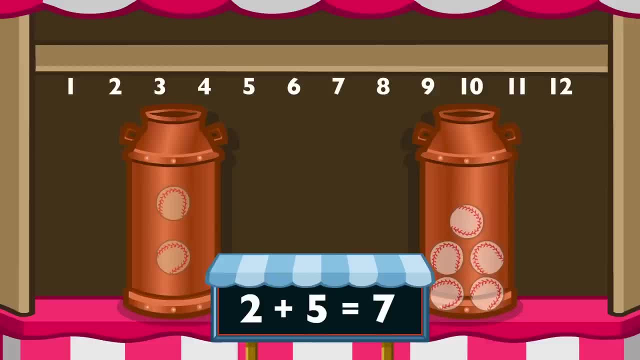 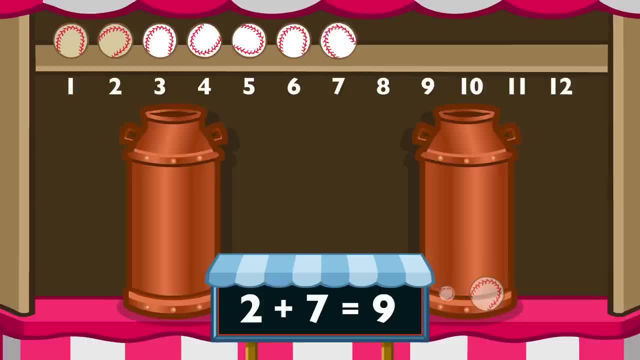 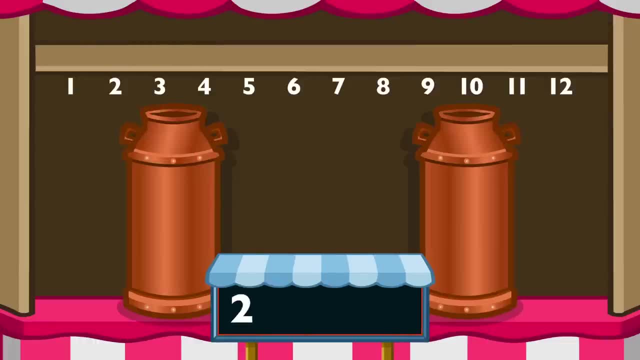 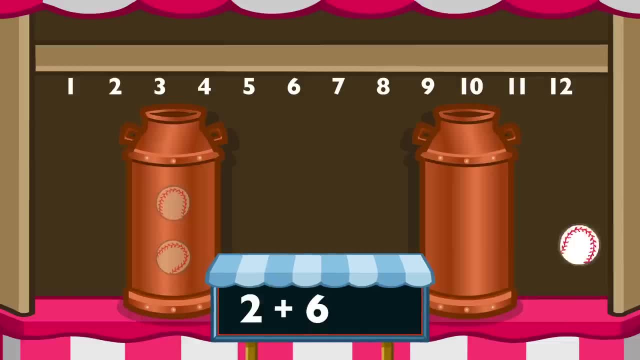 plus 6 equals 8.. 2 plus 6 equals 8.. 2 plus 1 equals 3.. 2 plus 1 equals 3.. 2 plus 8 equals 10.. 2 plus 8 equals 10.. 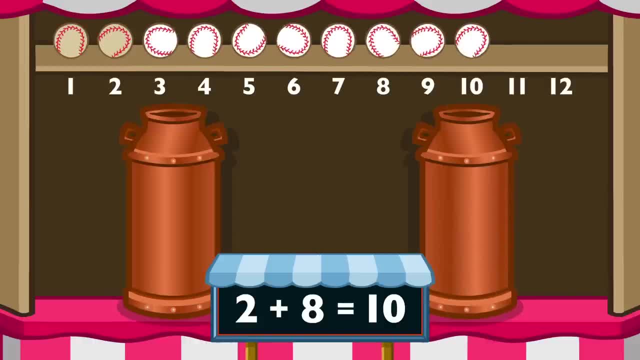 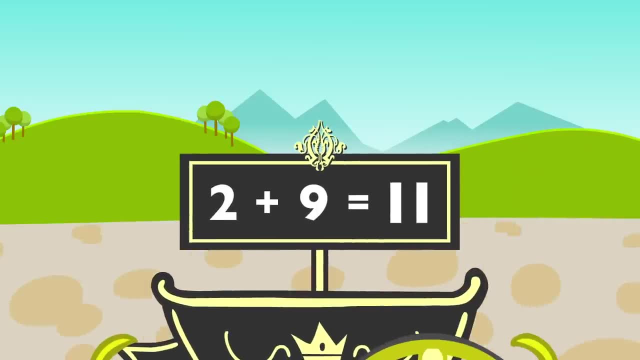 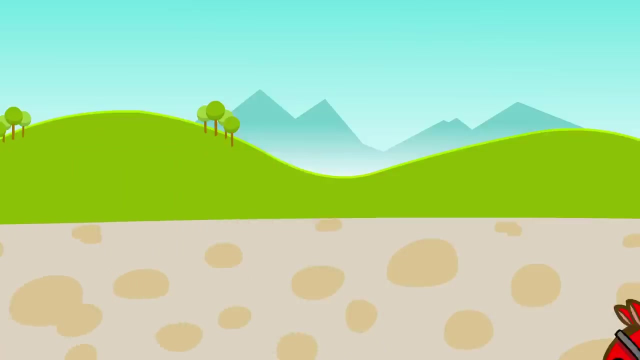 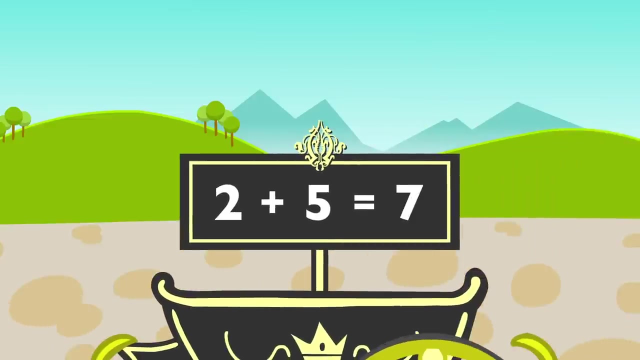 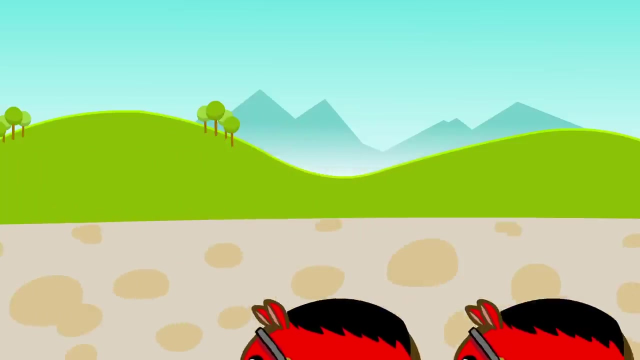 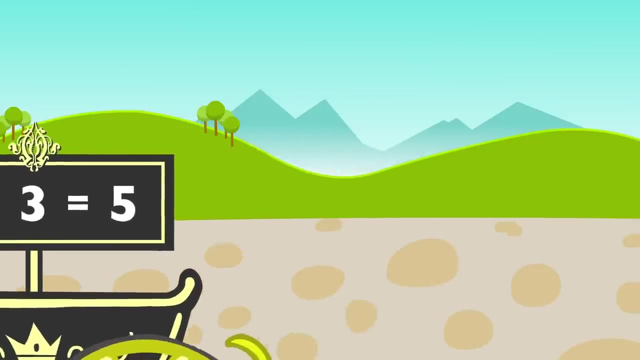 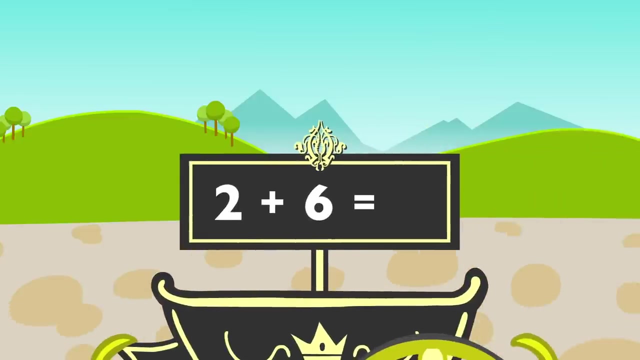 2 plus 9 equals 11.. 2 plus 1 equals 3.. 2 plus 5 equals 7.. 2 plus 7 equals 9.. 2 plus 3 equals 5.. 2 plus 6 equals. 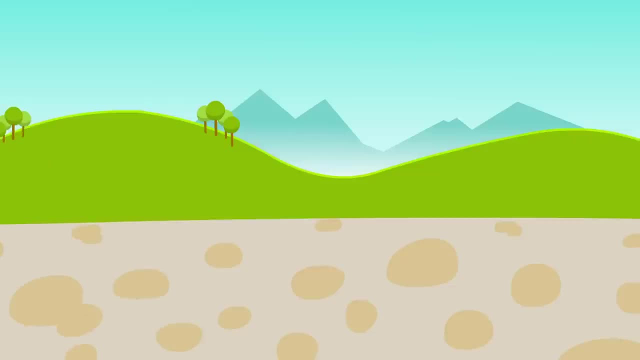 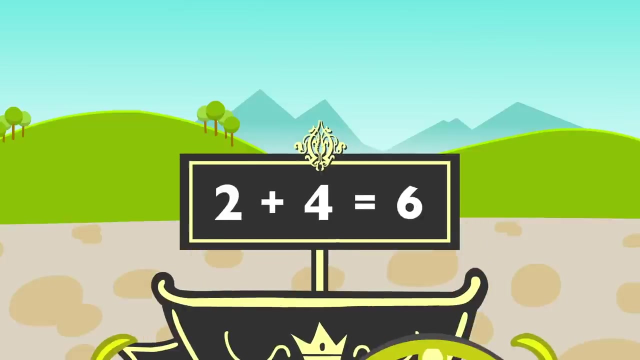 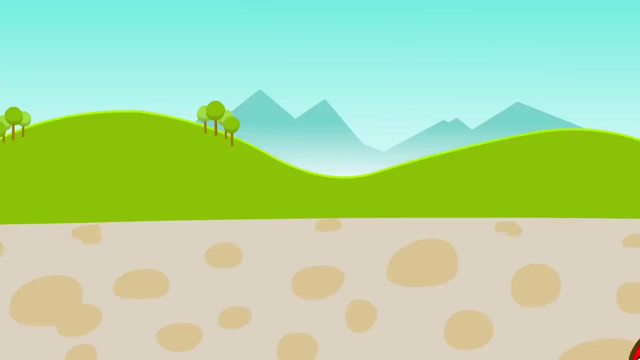 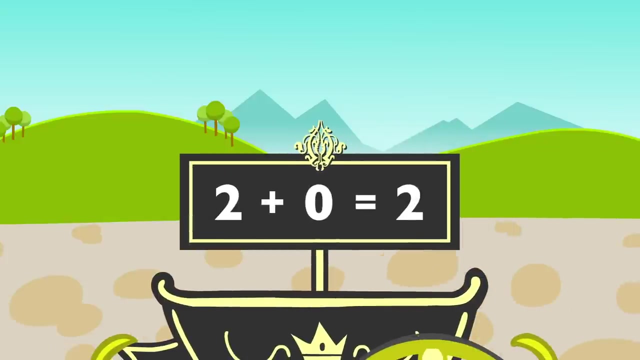 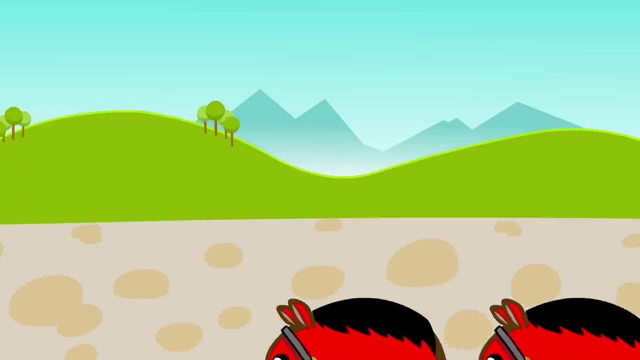 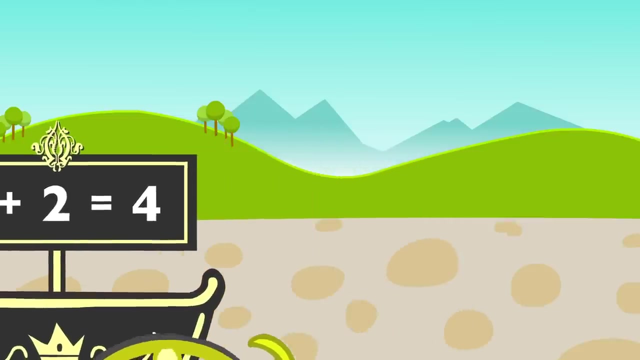 8. 2 plus 4 equals 6.. 2 plus 10 equals 12.. 2 plus 0 equals 2.. 2 plus 8 equals 10.. 2 plus 2 equals 4.. He has 2 medals. 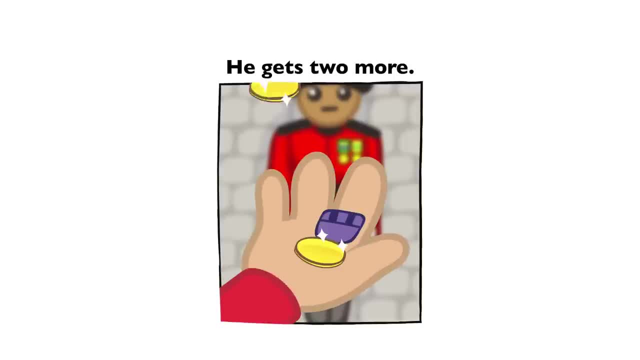 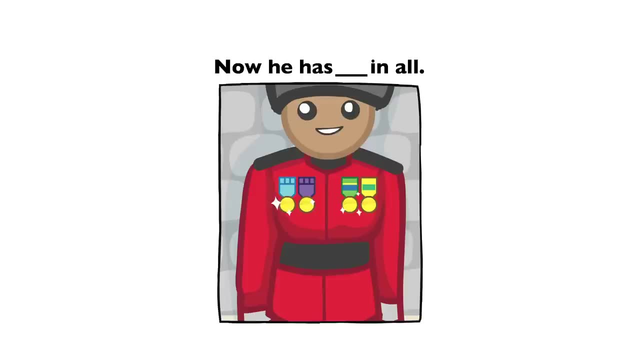 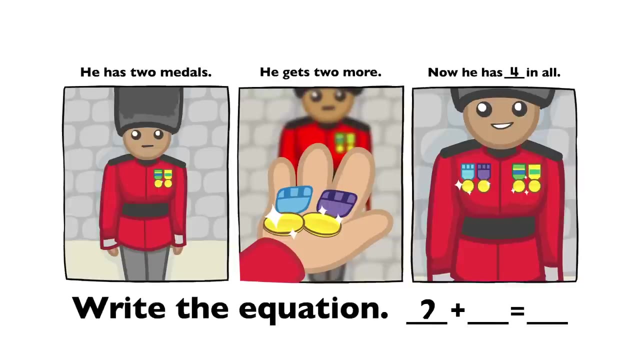 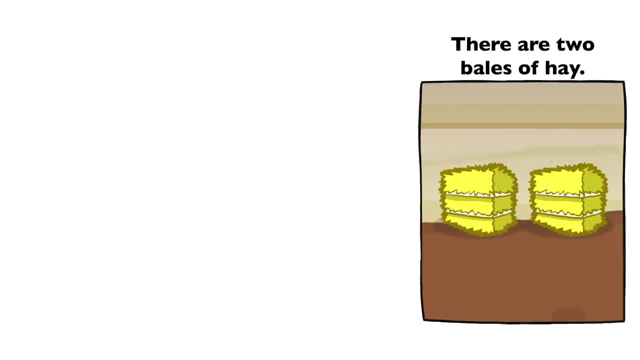 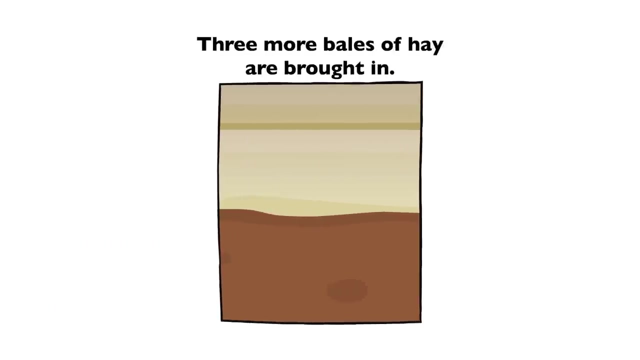 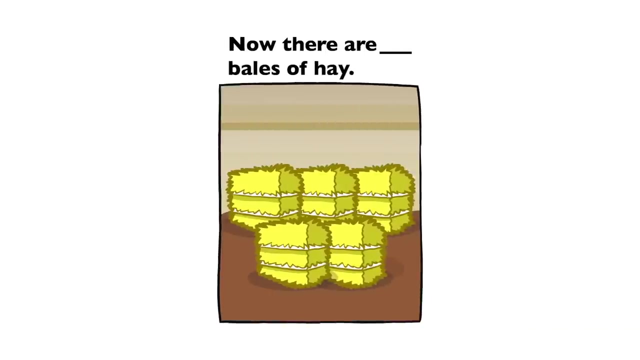 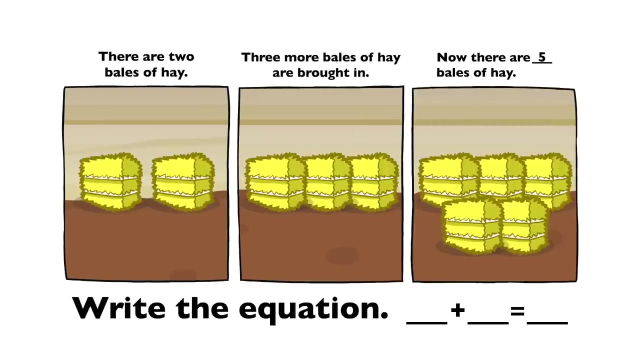 He gets two more. Now he has four in all. Two plus two equals four. There are two bales of hay. Three more bales of hay are brought in Now. there are five bales of hay. Two plus three equals five. 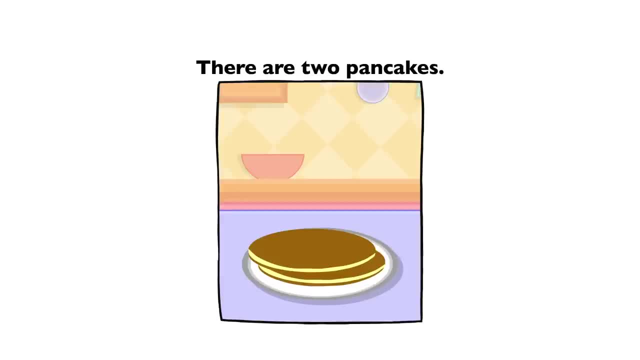 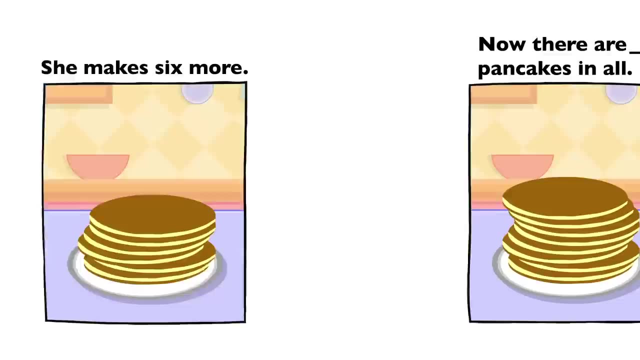 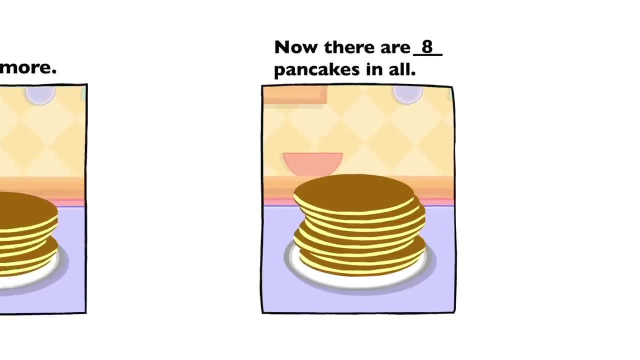 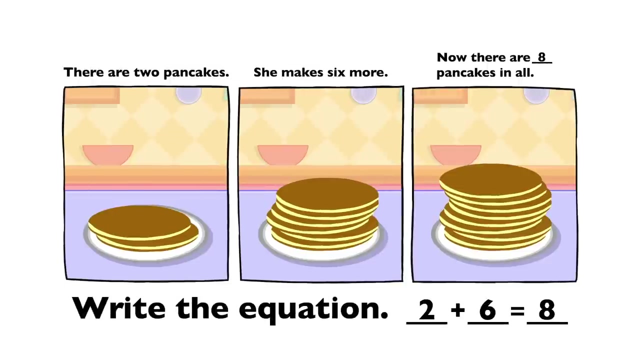 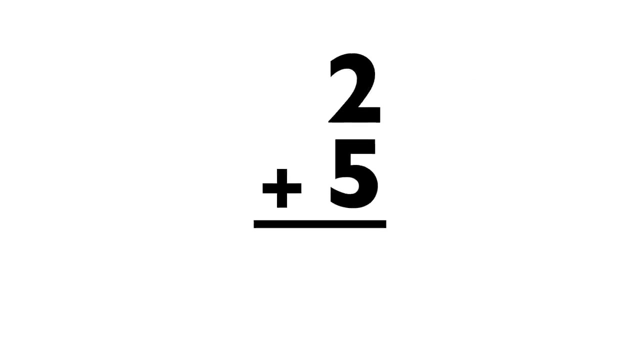 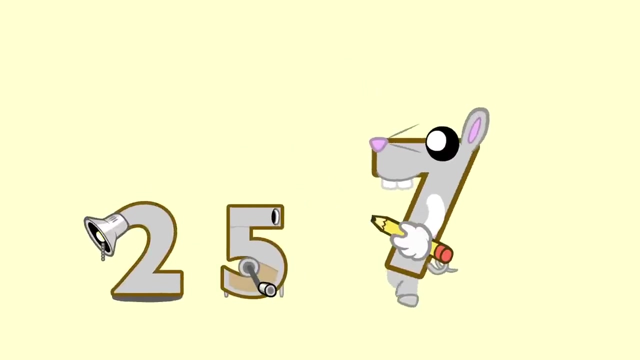 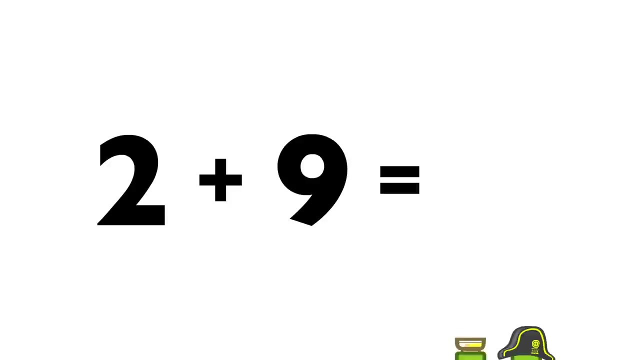 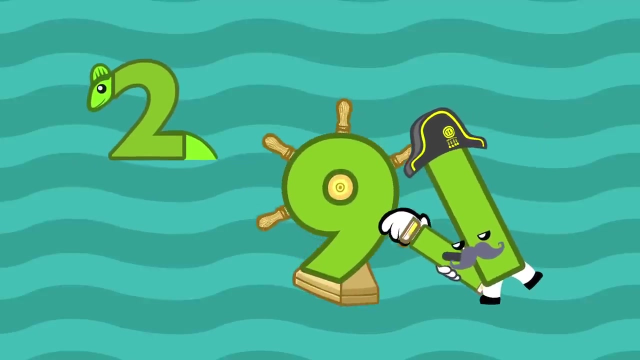 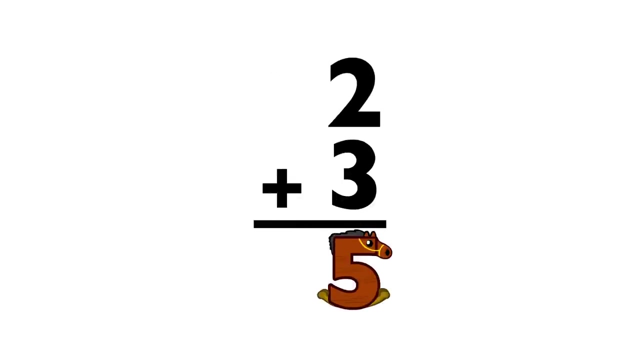 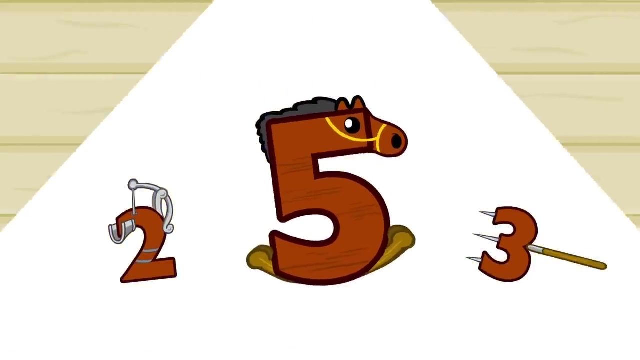 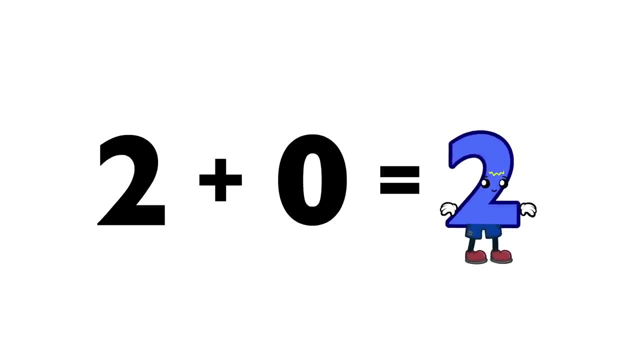 There are two pancakes, She makes six more. Now there are eight pancakes in all. Two plus six equals eight. Two plus five equals four. Two equals seven. Two plus nine equals 11.. Two plus three equals five. Two plus zero equals two. 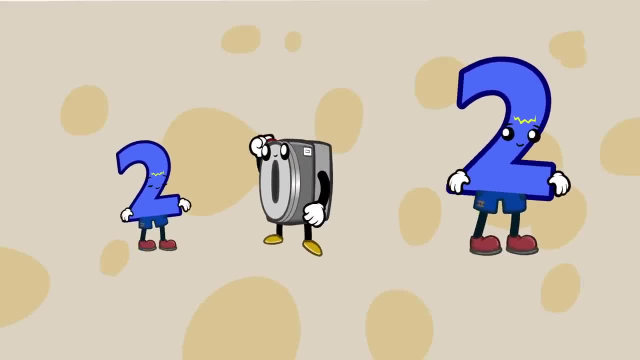 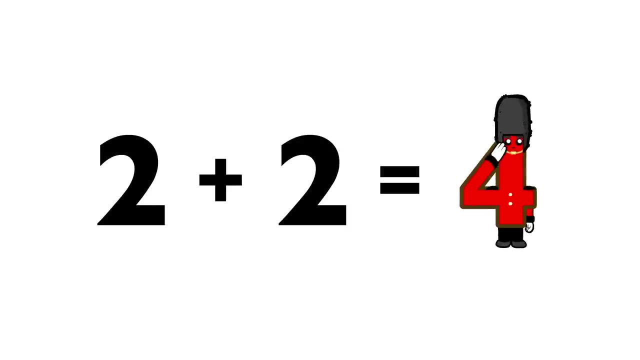 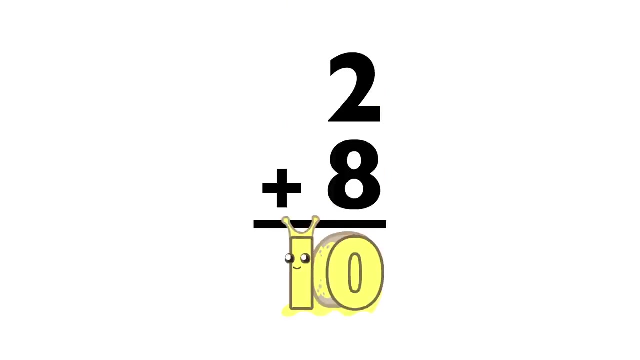 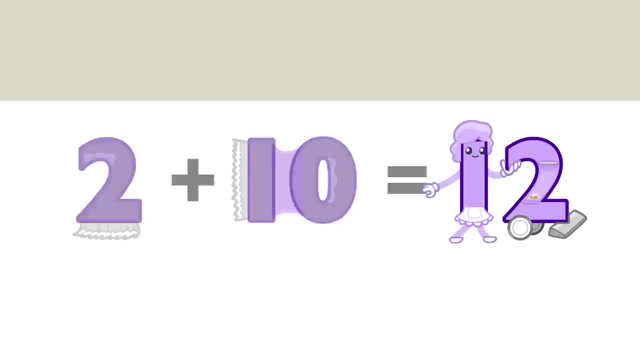 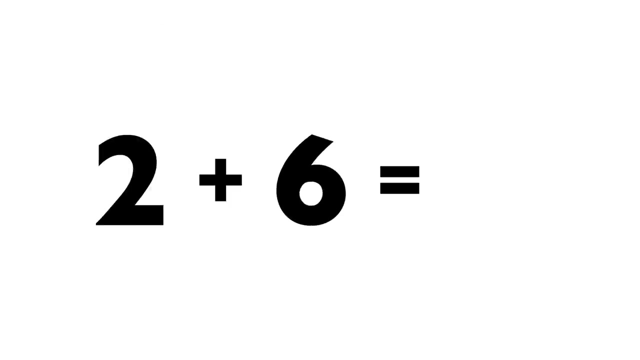 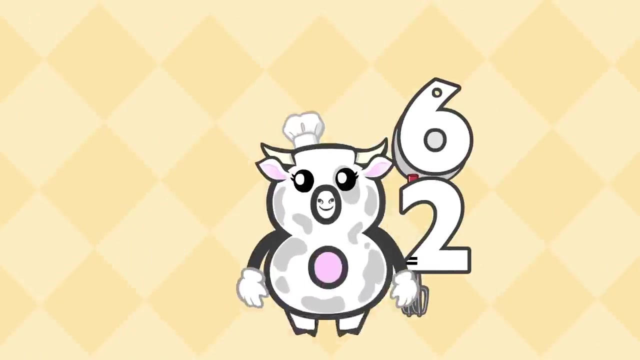 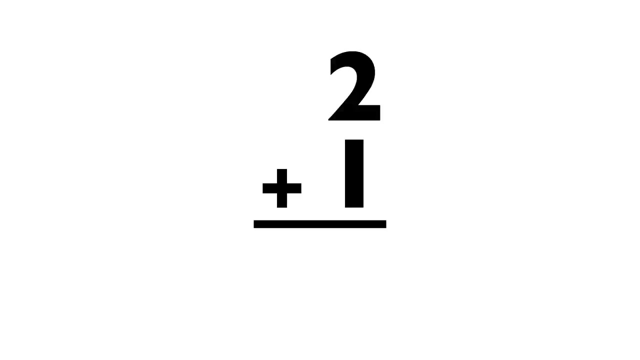 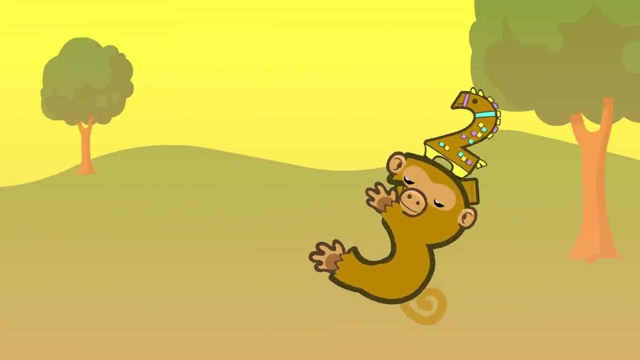 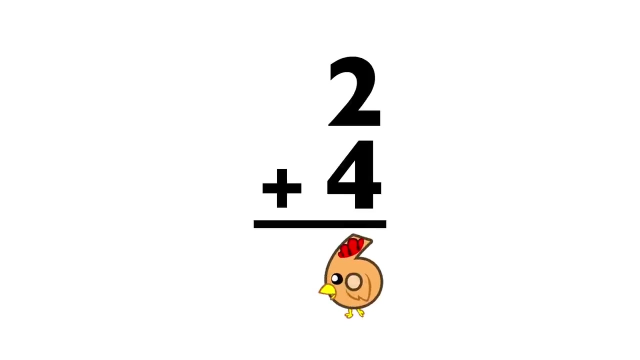 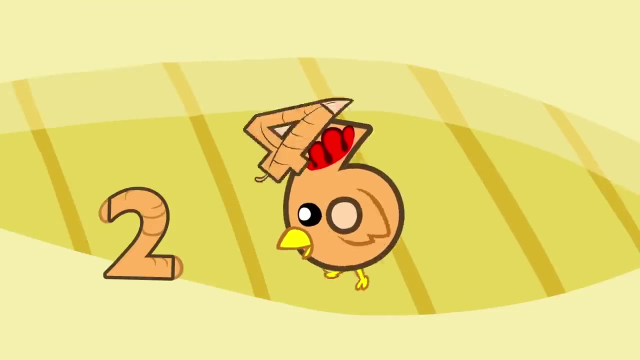 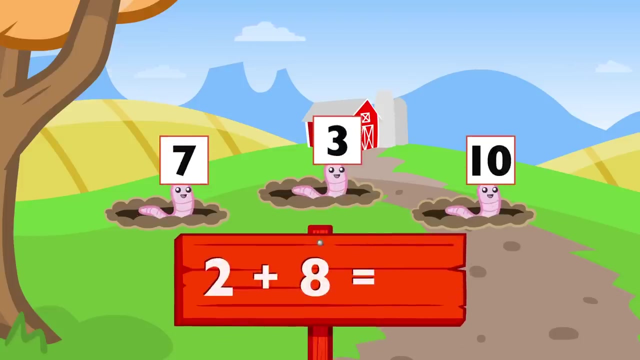 Two plus two equals four. Two plus two equals four. Two plus eight equals ten. Two plus seven equals nine. Two plus ten equals twelve. Two plus six equals eight. Two plus one equals three. Two plus four equals six. Two plus eight equals ten. 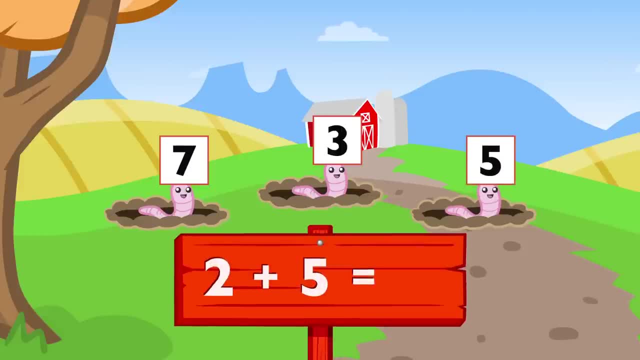 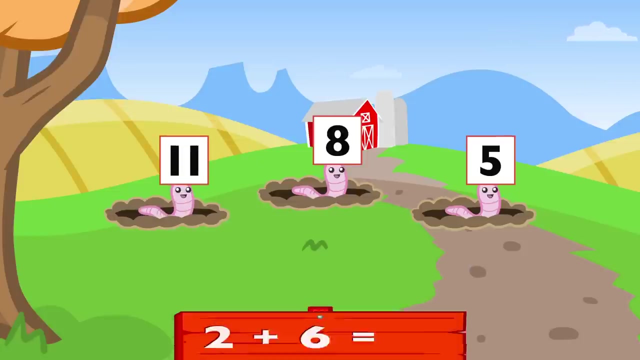 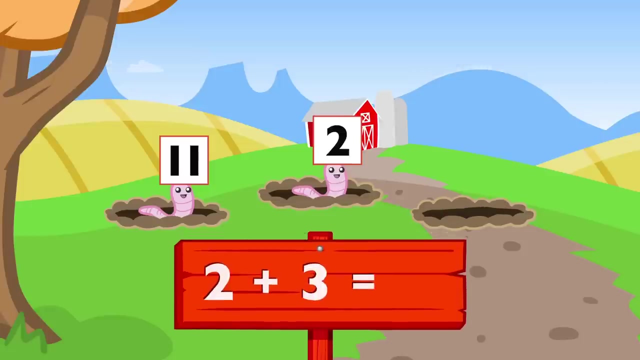 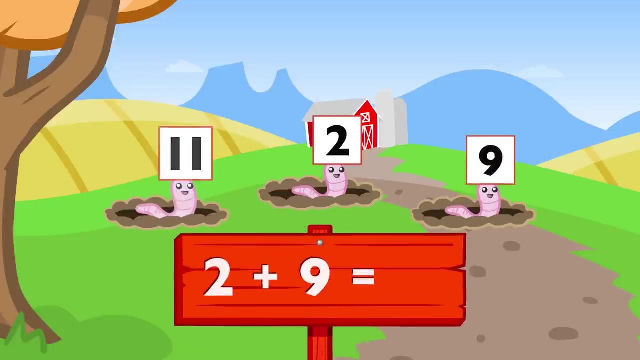 Two plus five equals seven. Two plus one equals three. Two plus ten equals twelve. Two plus six equals eight. Two plus three equals five. Two plus nine equals eleven. Two plus zero equals two. Two plus four equals. 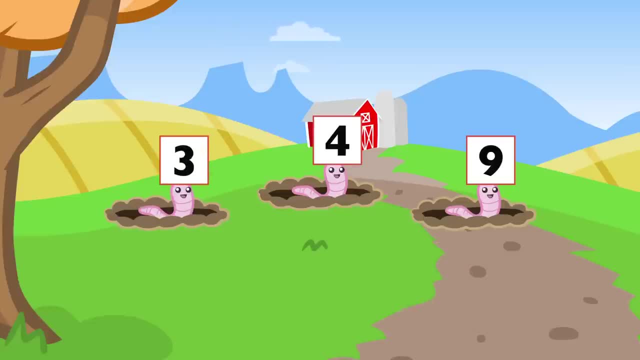 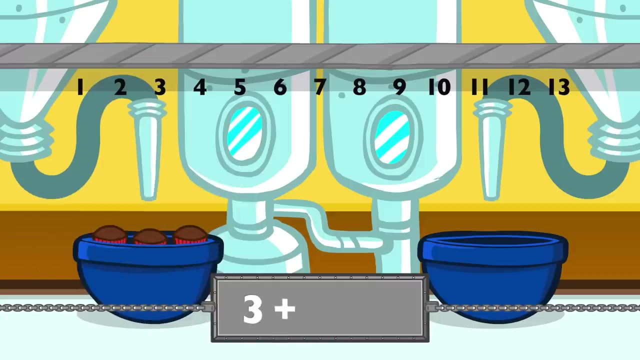 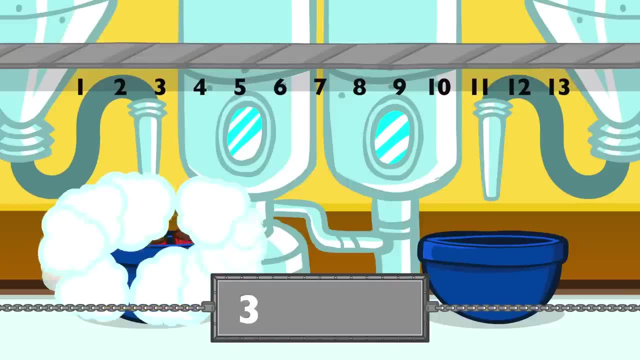 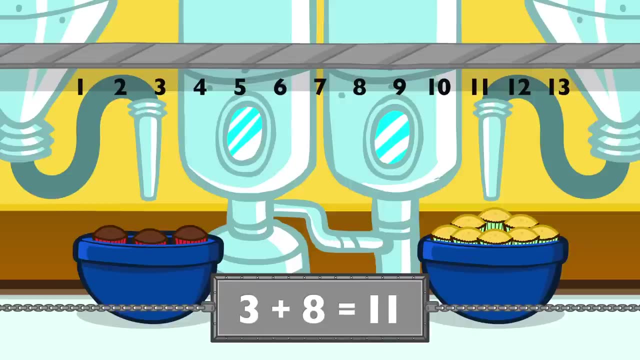 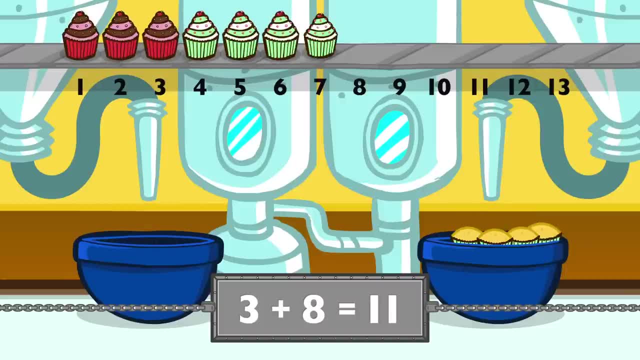 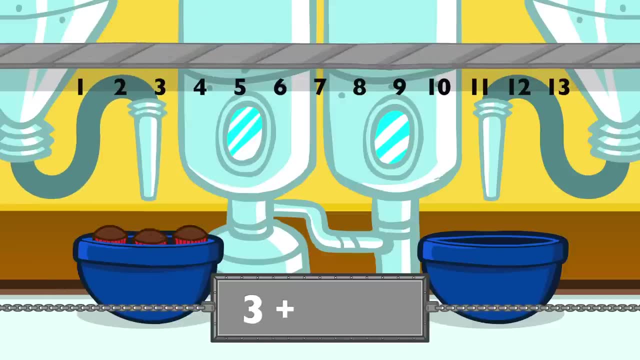 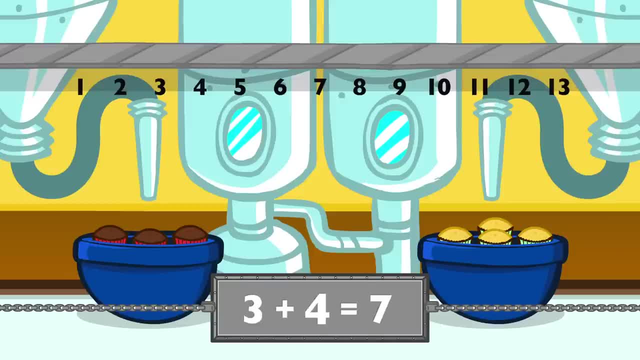 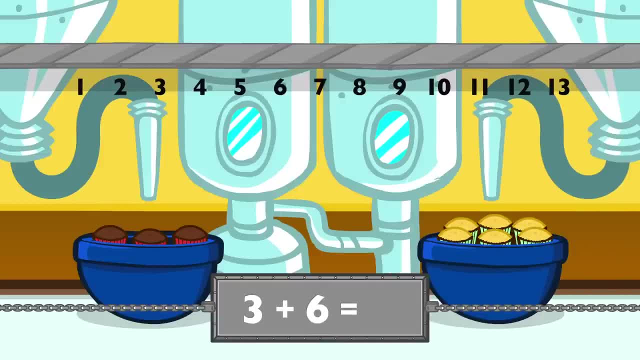 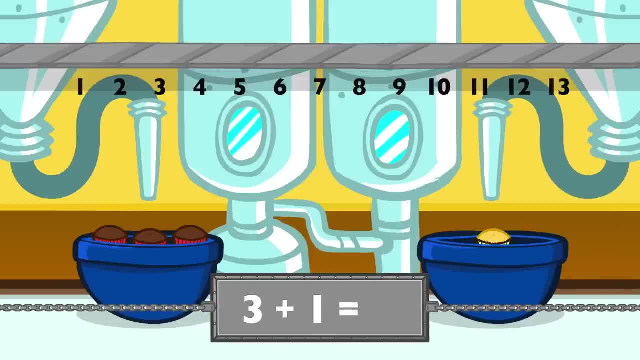 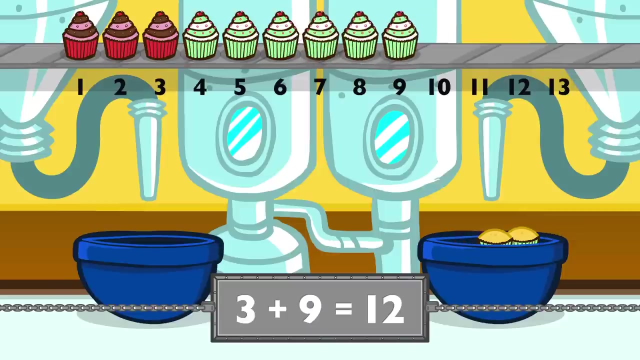 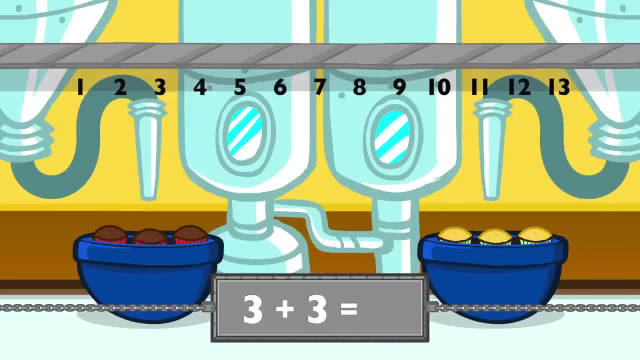 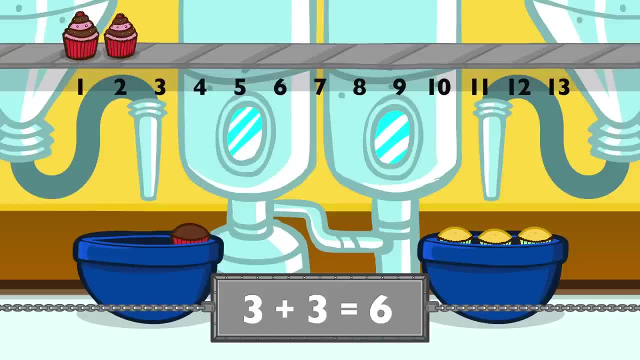 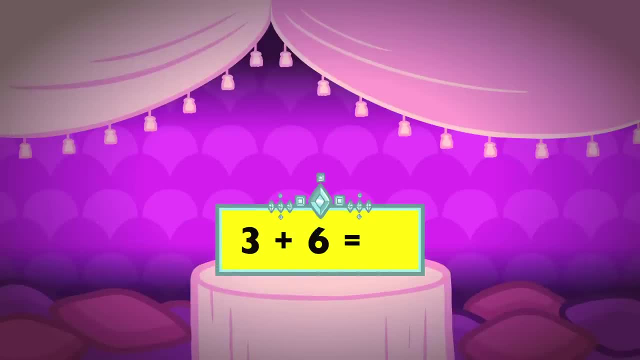 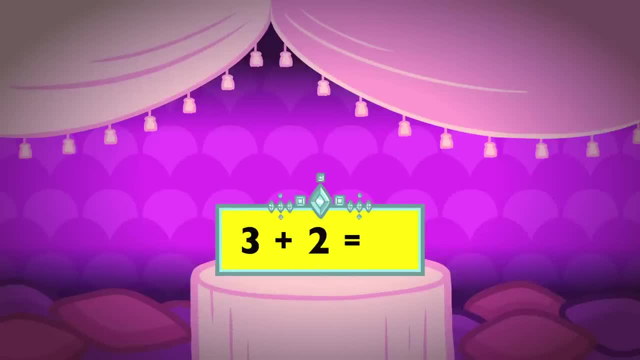 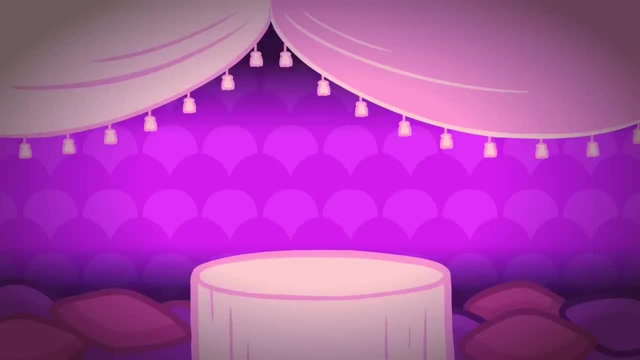 3 plus 9 equals 12, 3 plus 9 equals 12, 3 plus 5 equals 8.. 3 plus 1 equals 4.. 3 plus 8 equals 11.. 3 plus 10 equals 13.. 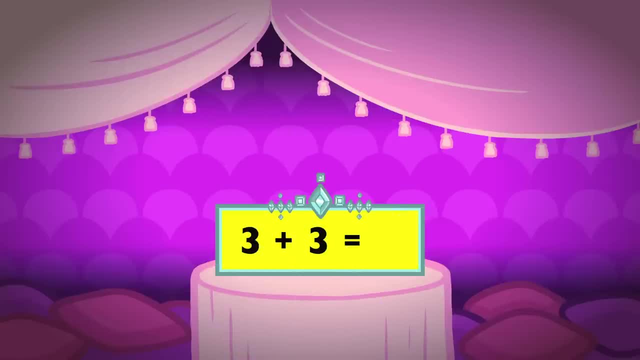 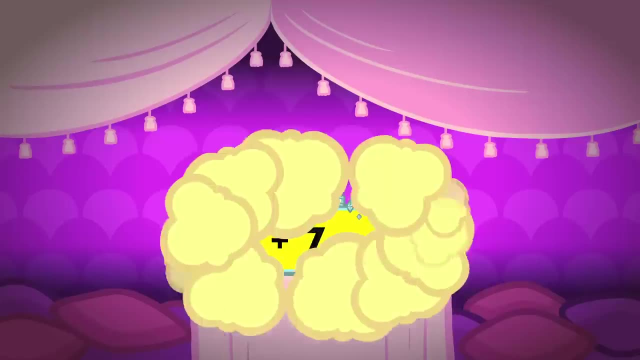 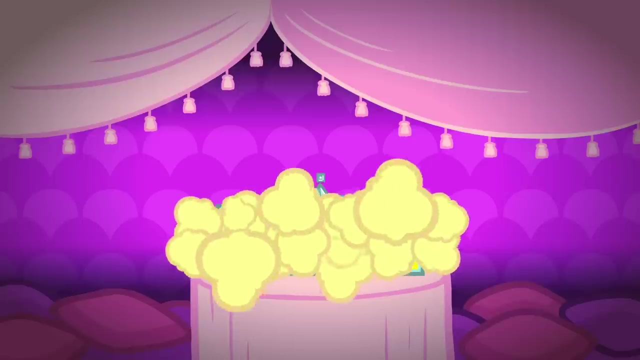 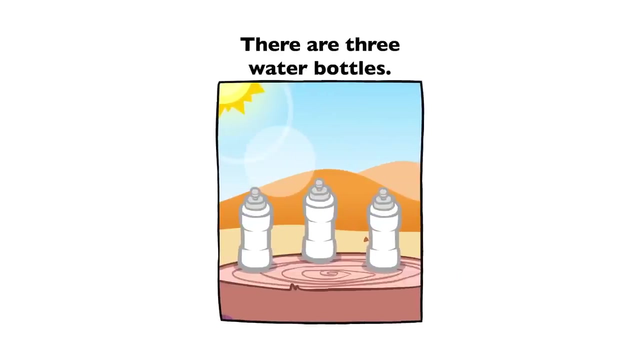 3 plus 3 equals 6.. 3 plus 7 equals 10.. 3 plus 0 equals 3.. 3 plus 9 equals 12.. 3 plus 4 equals 7.. There are three water bottles. 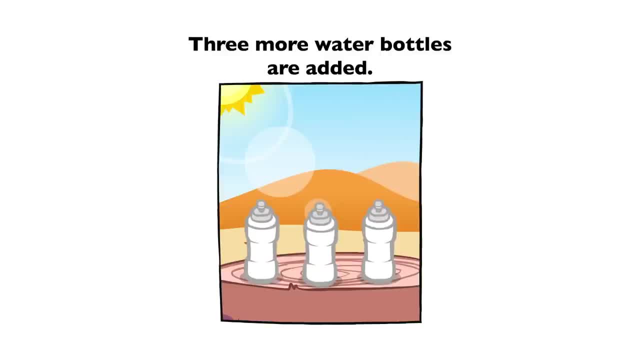 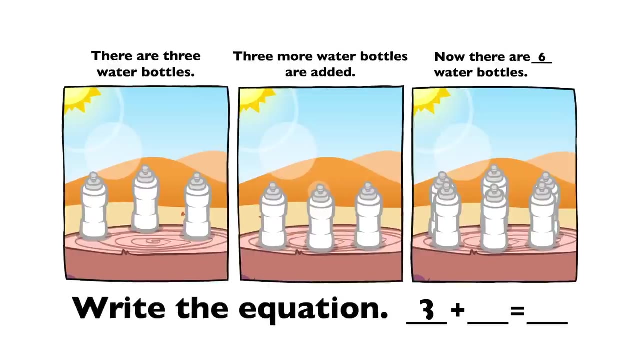 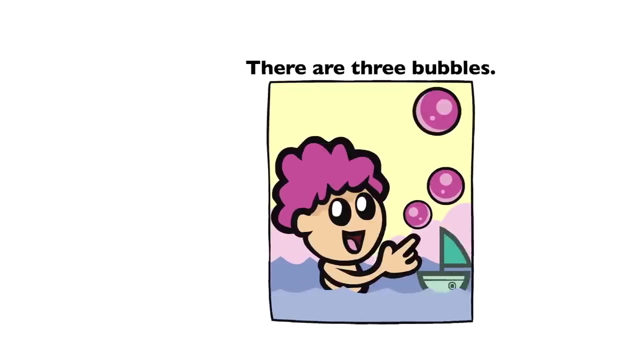 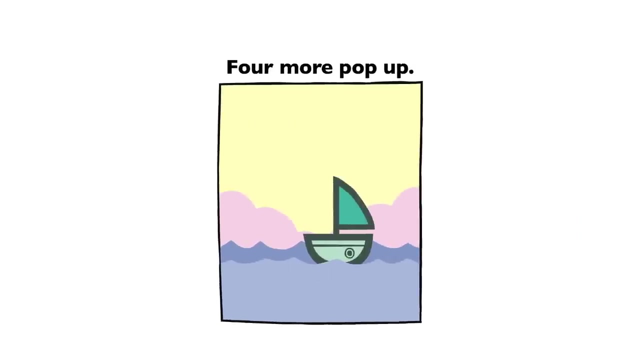 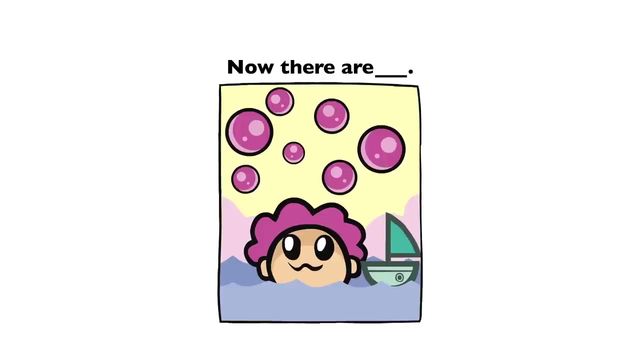 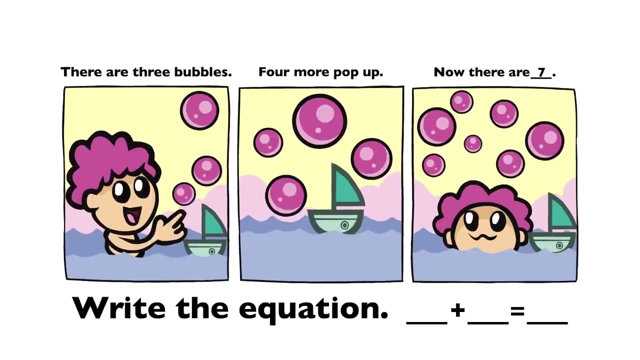 Three more water bottles are added. Now there are six water bottles. 3 plus 3 equals 6.. There are three bubbles. Four more pop up. Now there are seven. 3 plus 4 equals 7.. 3 plus 4 equals 7.. 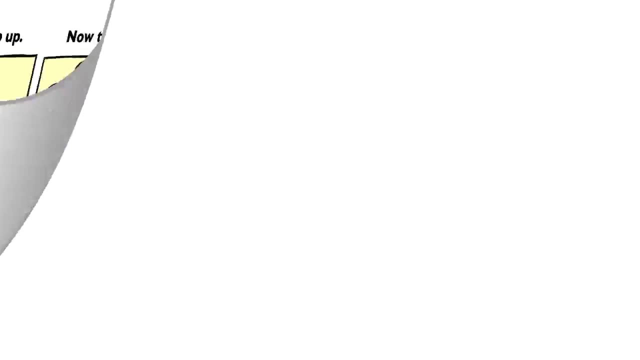 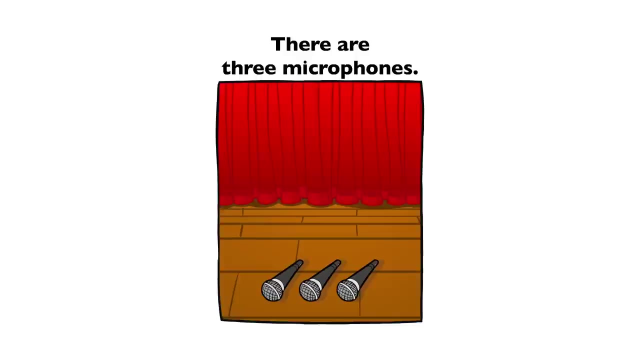 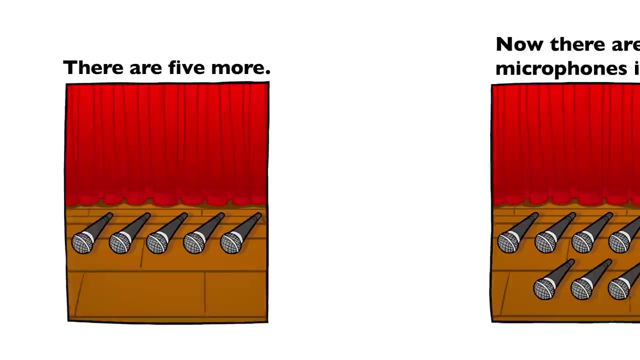 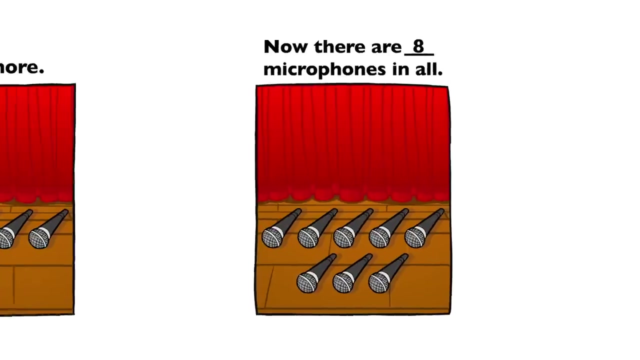 3 plus 4 equals 7.. 3 plus 4 equals 8.. There are three microphones. There are five more. There are three microphones, There are five more. Now. there are Eight microphones in all. Three plus five equals 8.. 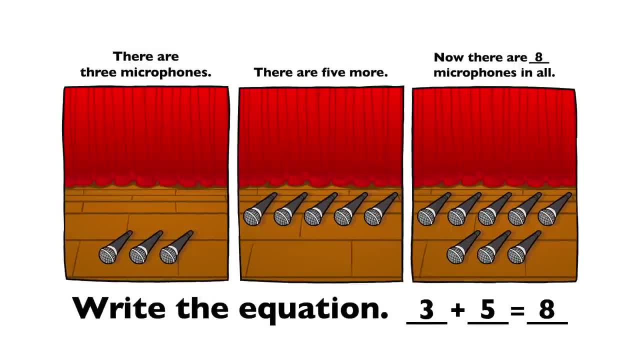 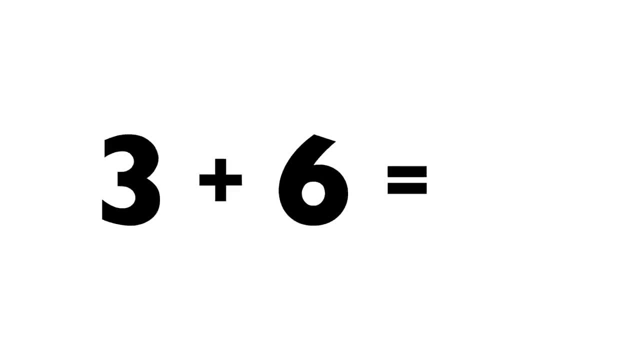 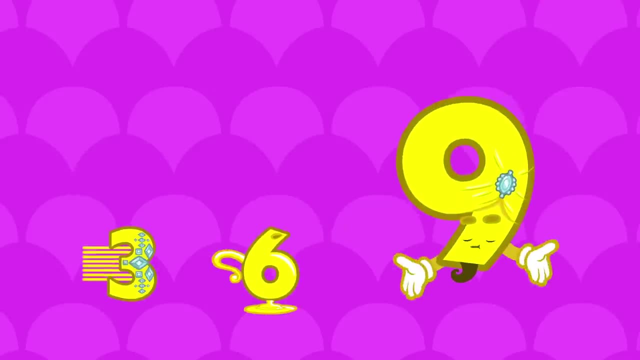 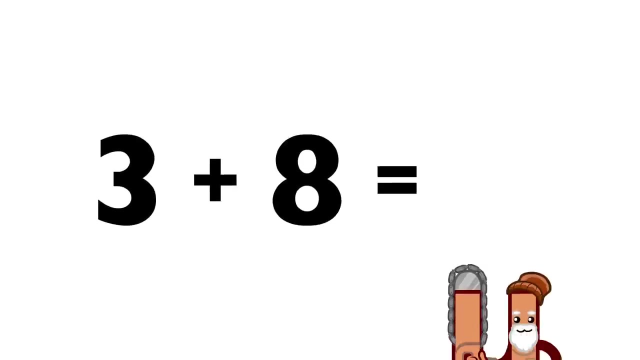 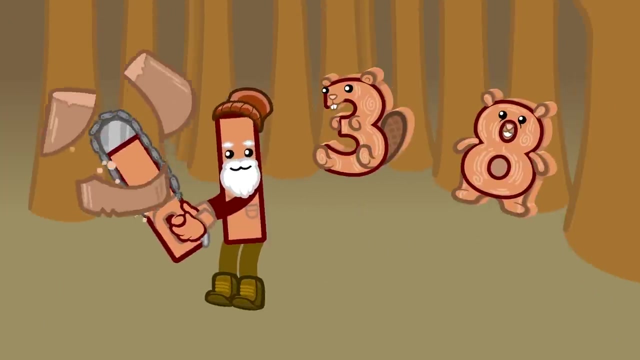 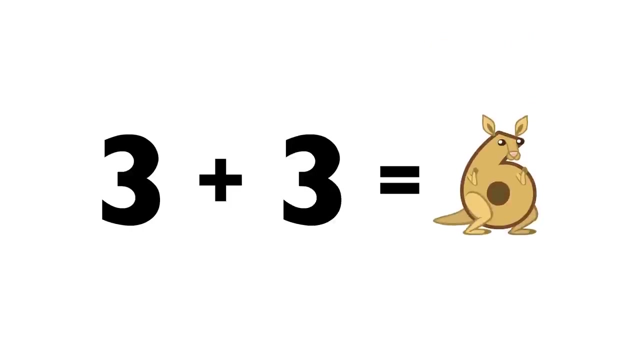 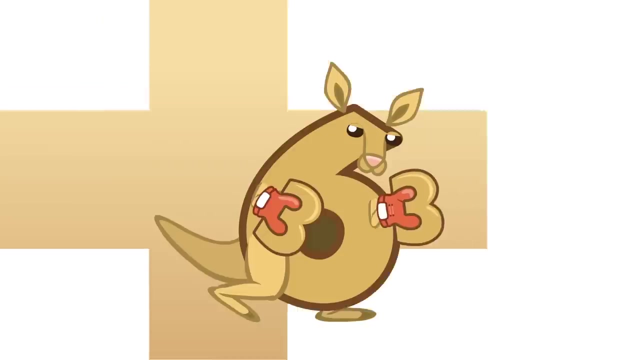 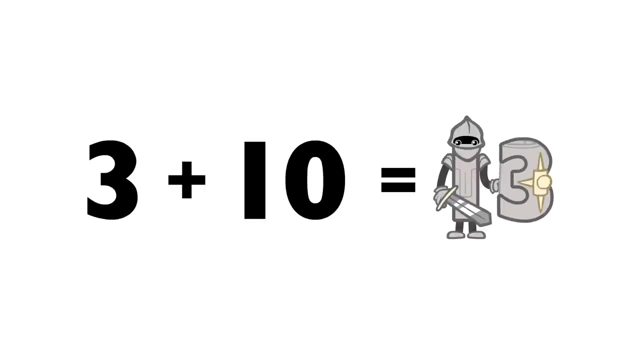 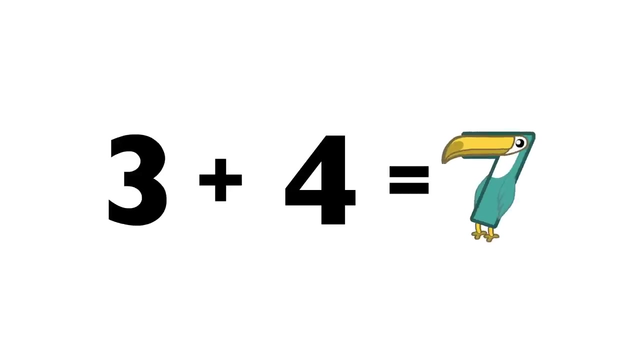 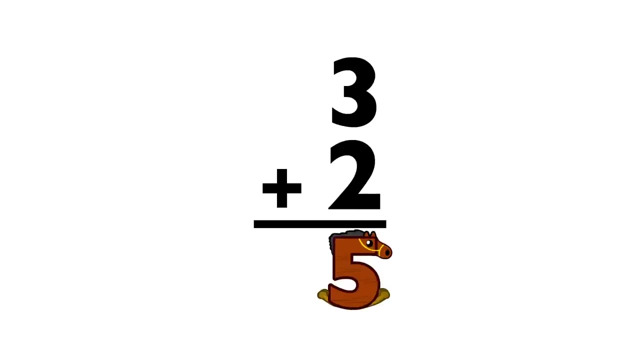 Two microphones in all. Three plus five equals 8.. three plus six equals nine. three plus eight equals eleven. three plus three equals six. three plus ten equals thirteen. eleven, three plus four equals seven. three plus two equals five. 3 plus 7 equals 10. 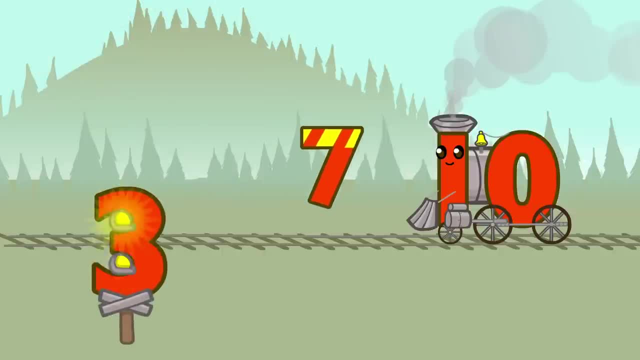 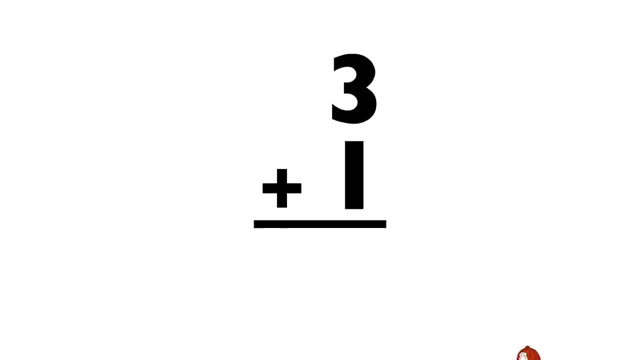 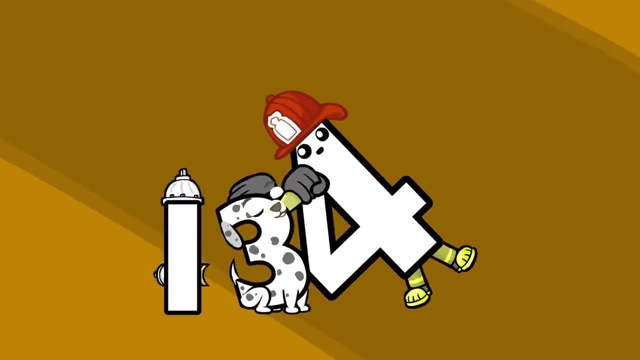 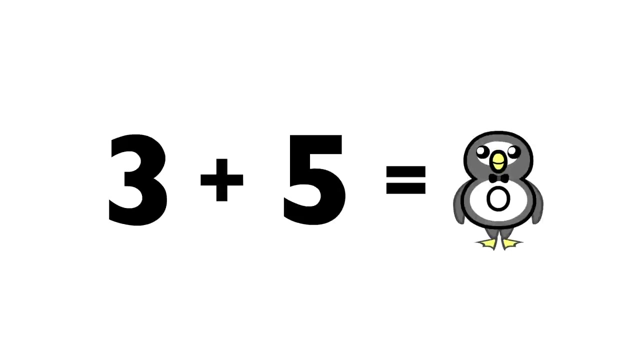 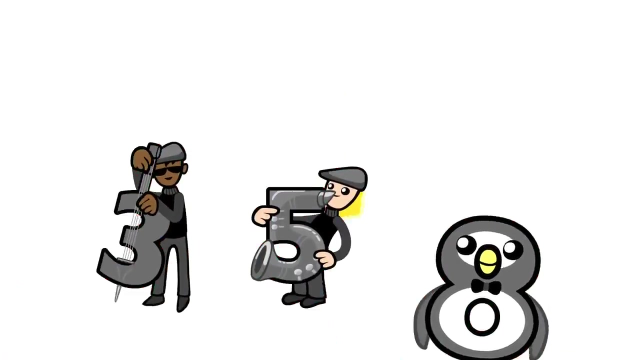 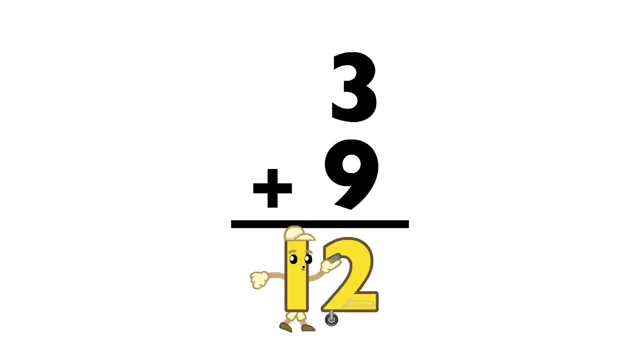 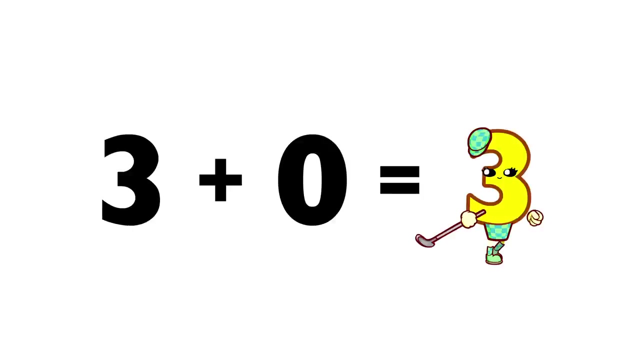 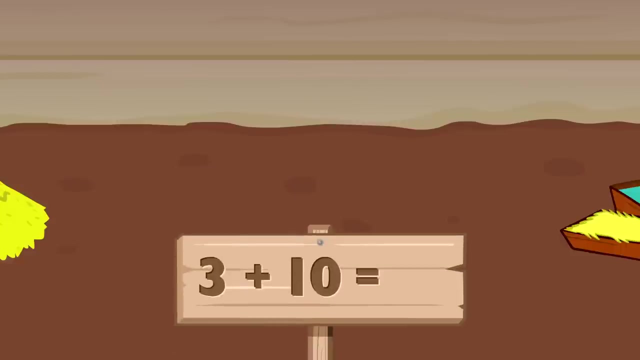 3 plus 1 equals 4. 3 plus 5 equals 8. 3 plus 9 equals 12. 3 plus 9 equals 12. 3 plus 9 equals 12. 3 plus 0 equals 3. 3 plus 10 equals 13. 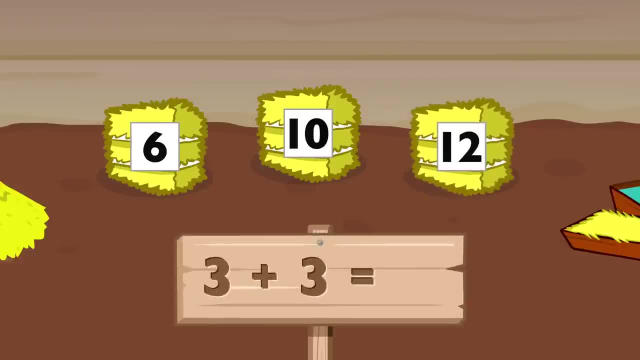 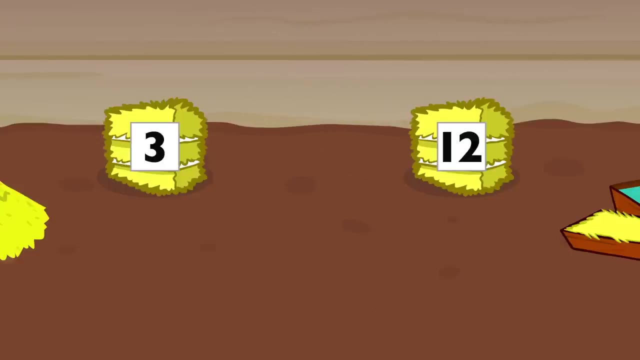 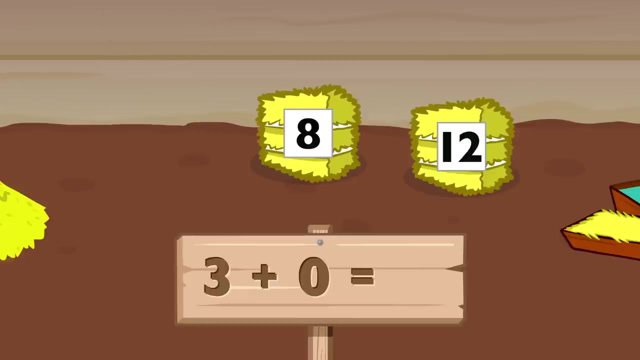 3 plus 3 equals 6. 3 plus 7 equals 10. 3 plus 0 equals 3. 3 plus 5 equals 8. 3 plus 9 equals 12. 3 plus 10 equals 12. 3 plus 1 equals 4. 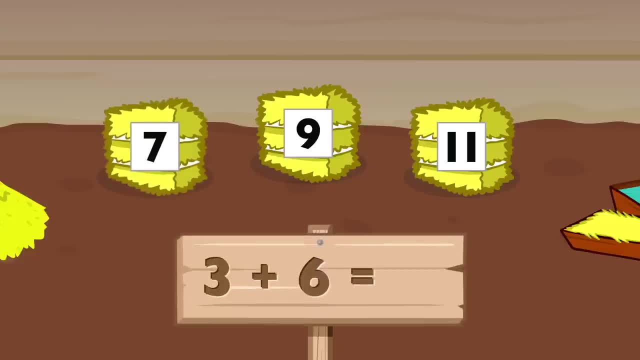 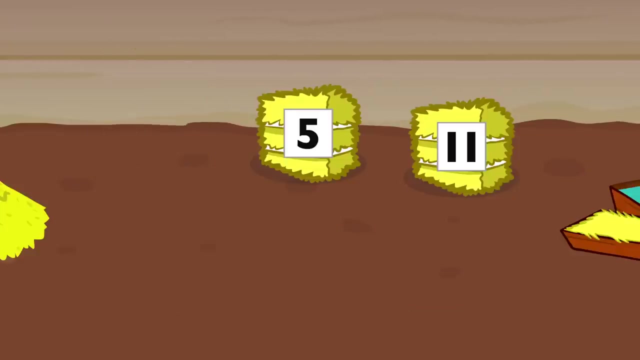 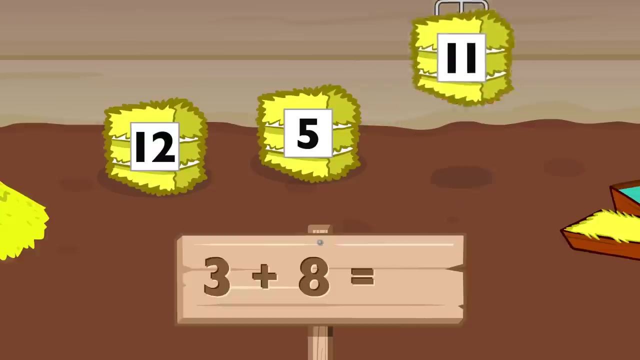 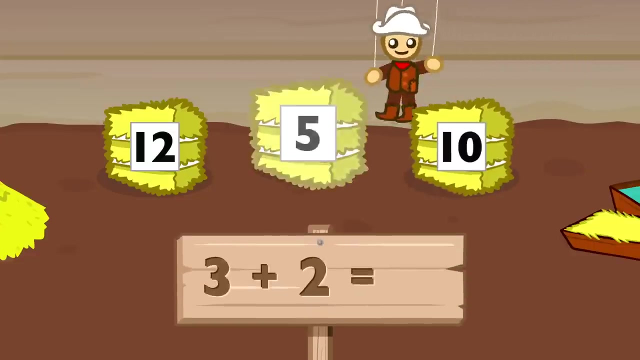 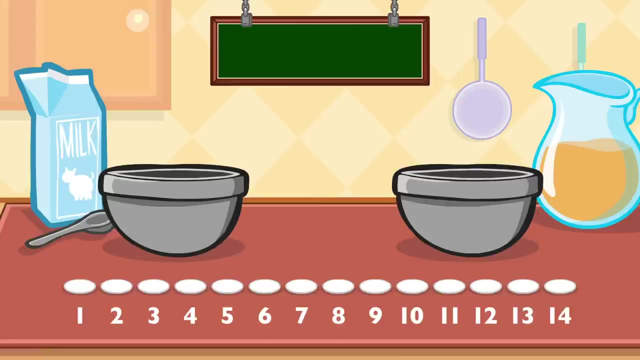 3 plus 6 equals 9. 3 plus 4 equals 7. 3 plus 8 equals 9. 3 plus 8 equals 11. 3 plus 2 equals 5. 3 plus 2 equals 5. 4 plus 3 equals 7. 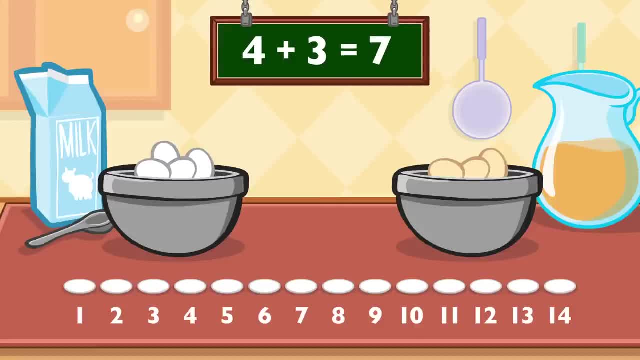 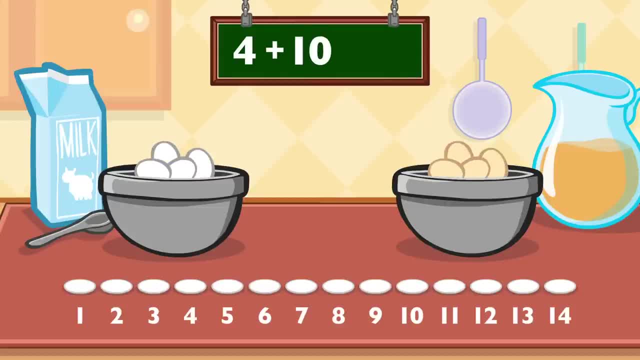 4 plus 2 equals 7. 4 plus 2 equals 7. 4 plus 3 equals 7. 4 plus 3 equals 8. 3 plus 3 equals 11. 1 plus 1 equals 6. 4 plus 4 equals 11. 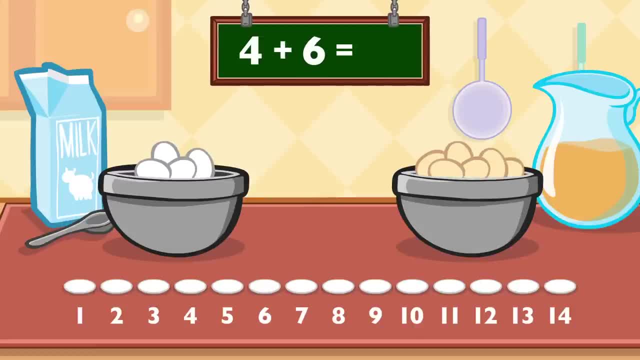 7 plus 10 equals 12. 3 plus 2 equals 12, equals 10.. 4 plus 6 equals 10.. 4 plus 0 equals 4.. 4 plus 0 equals 4.. 4 plus 7 equals 11.. 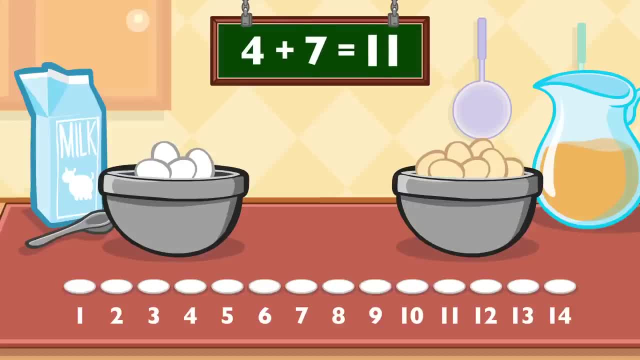 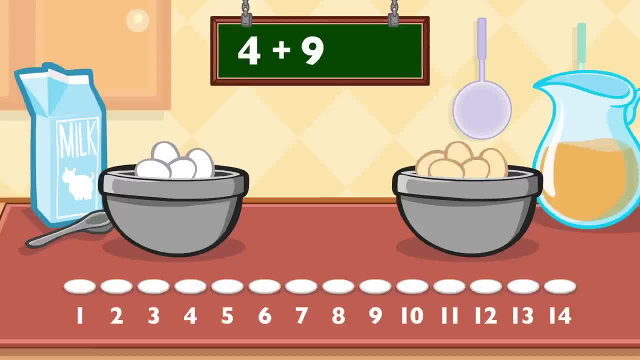 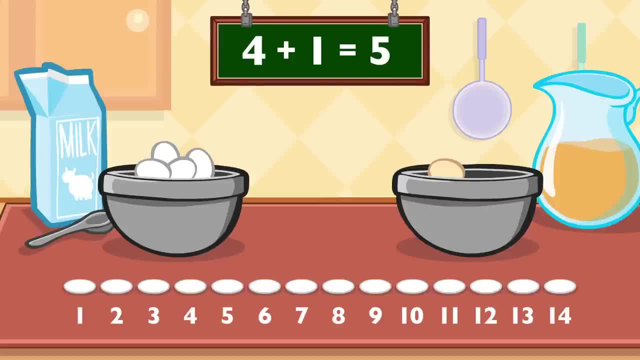 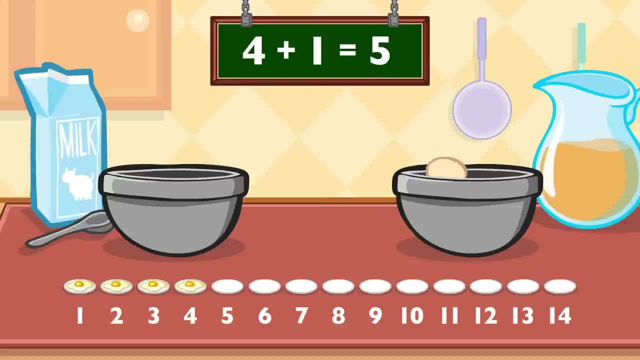 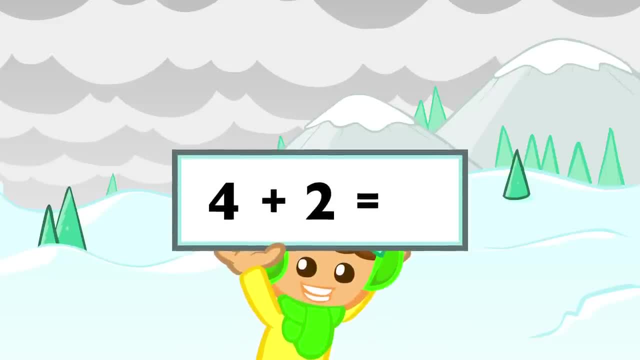 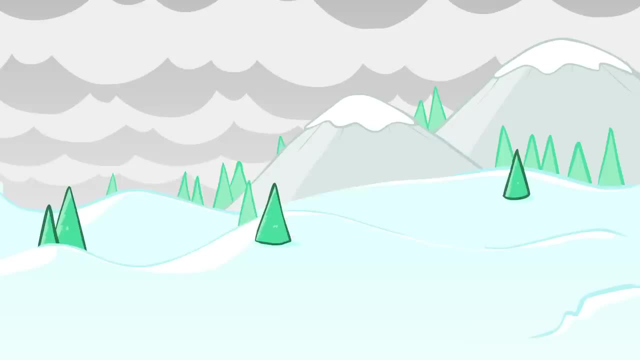 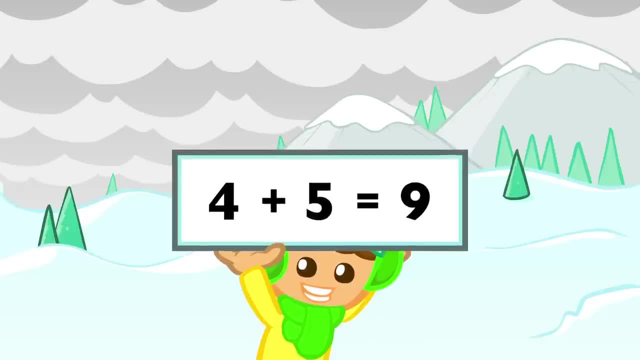 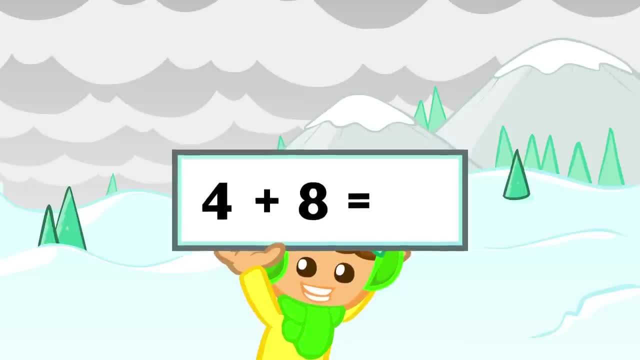 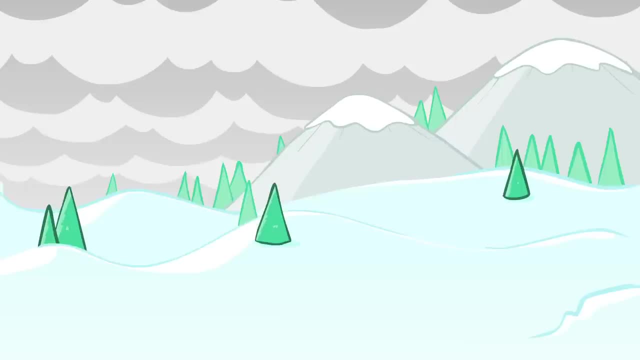 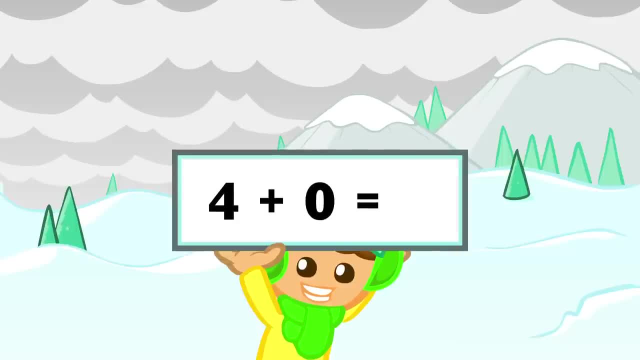 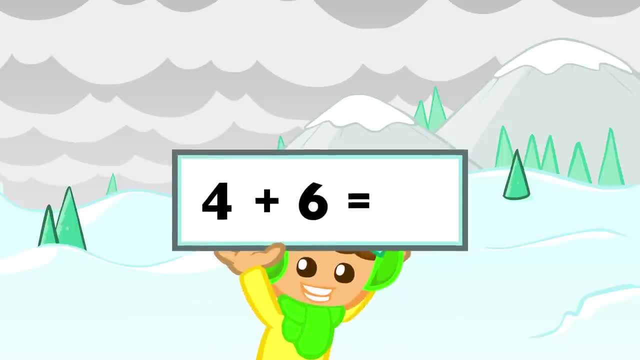 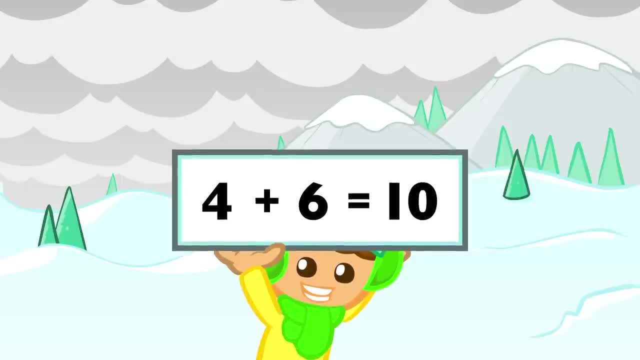 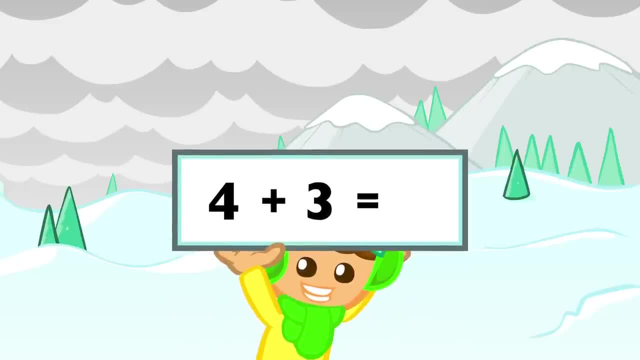 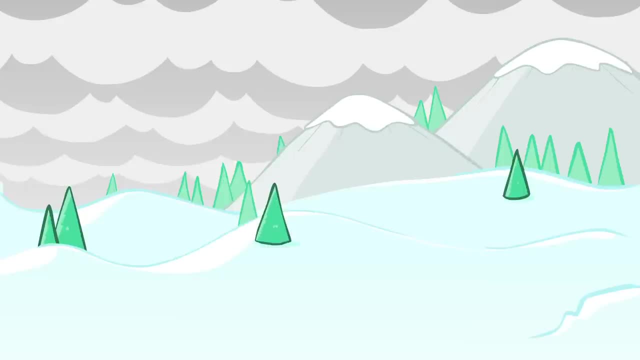 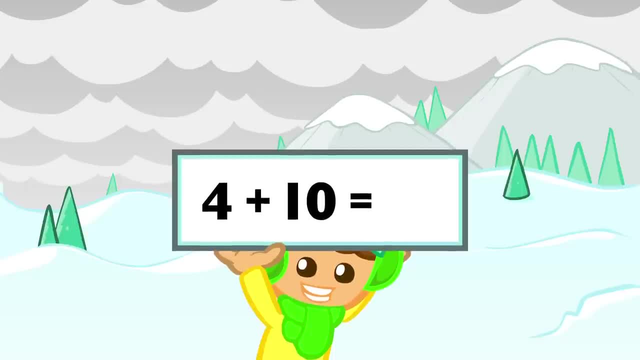 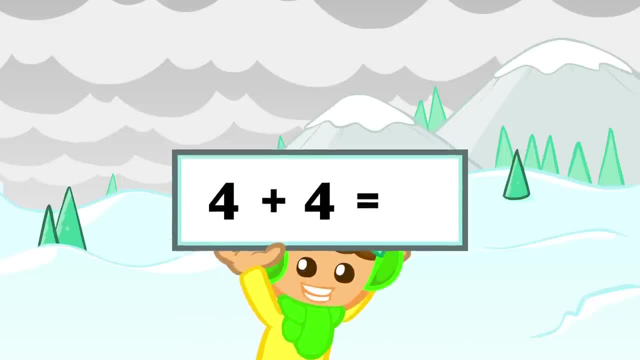 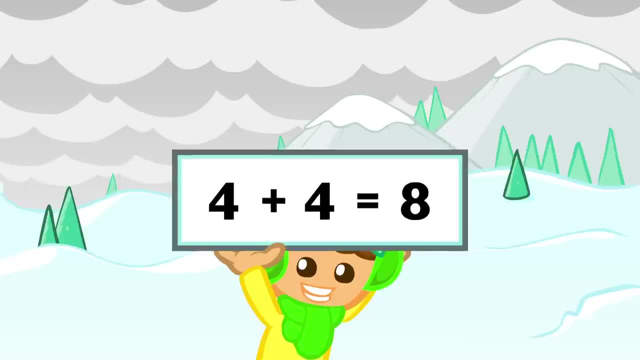 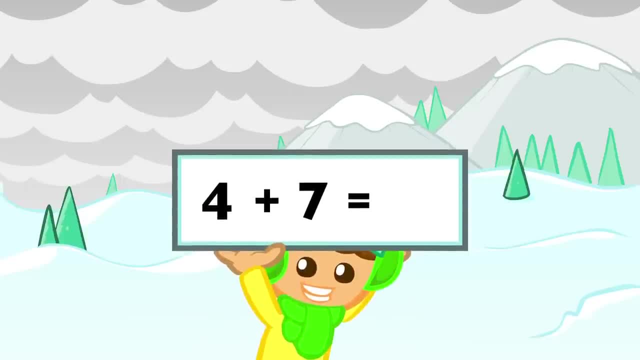 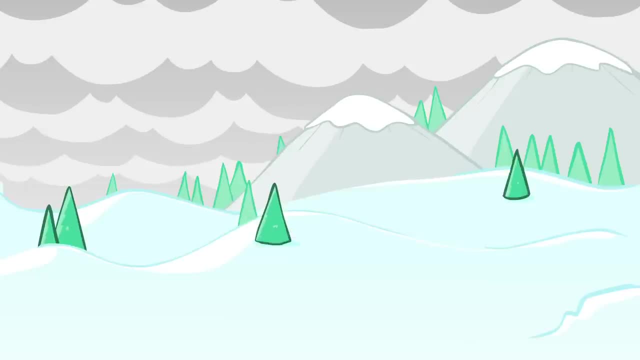 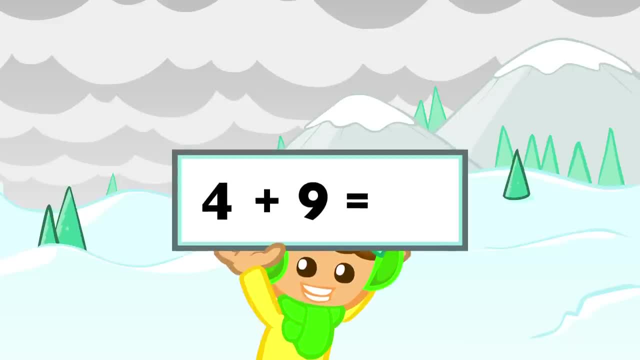 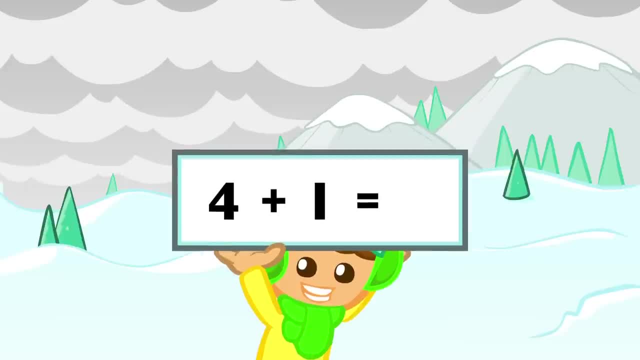 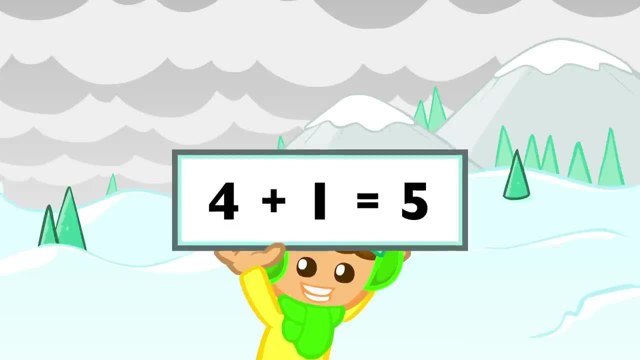 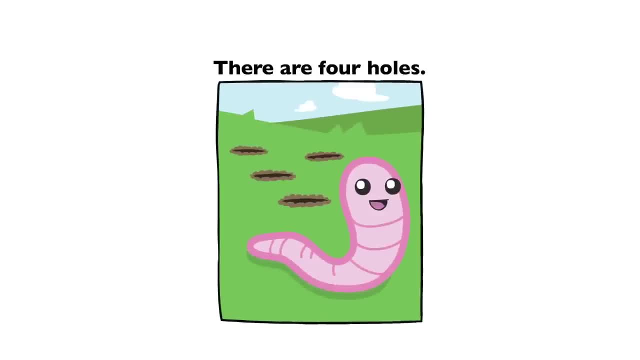 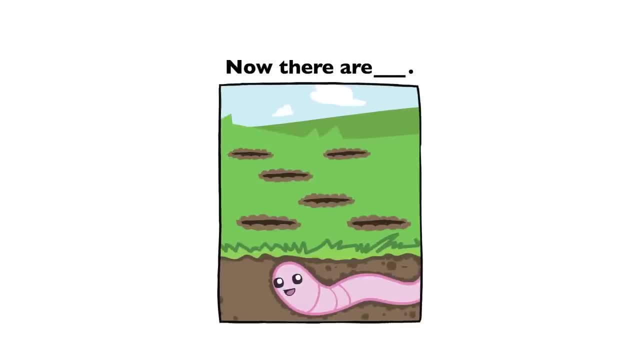 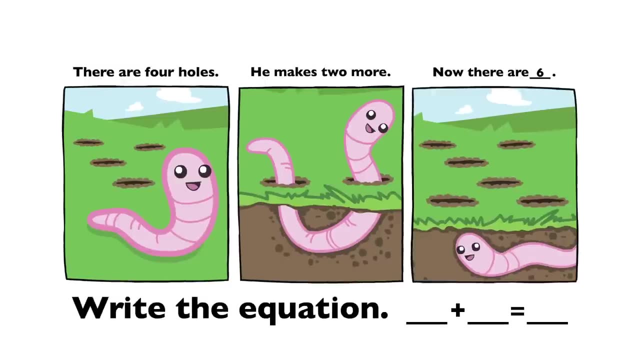 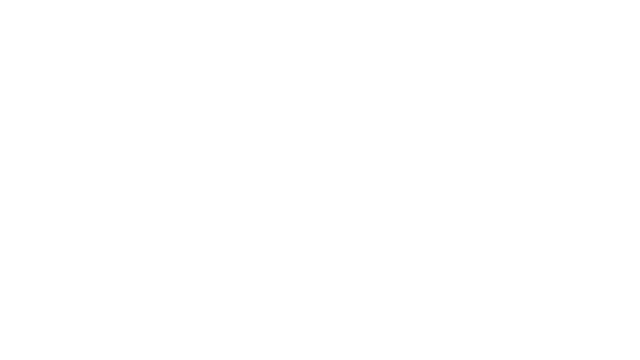 4 plus 9 equals 13.. She picks 2 more. She picks 2 more. 委 і veц adjustment by Deposit. Now there are 6.. Now there are 6.. 4 più 2 equals 6.. She has 4 snowballs. 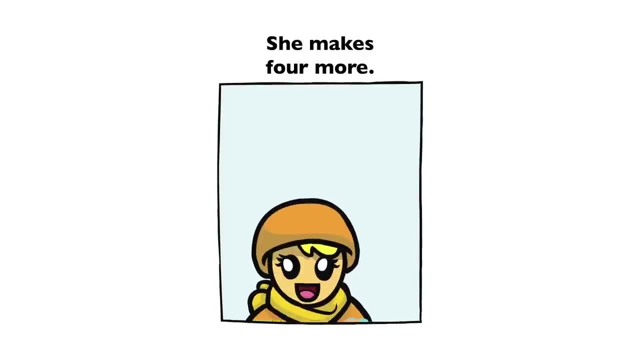 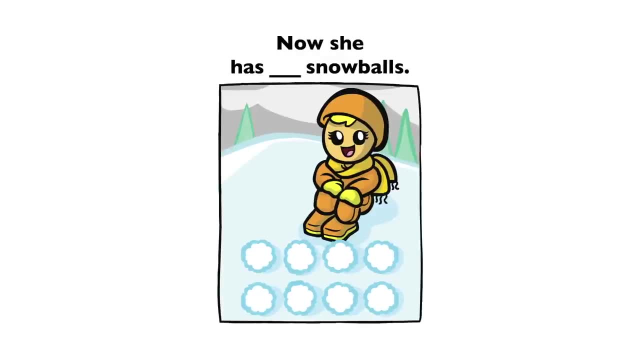 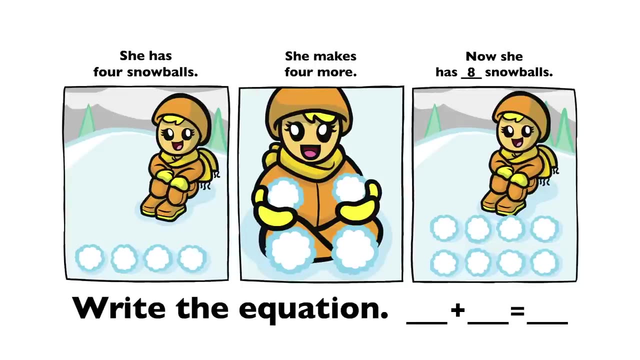 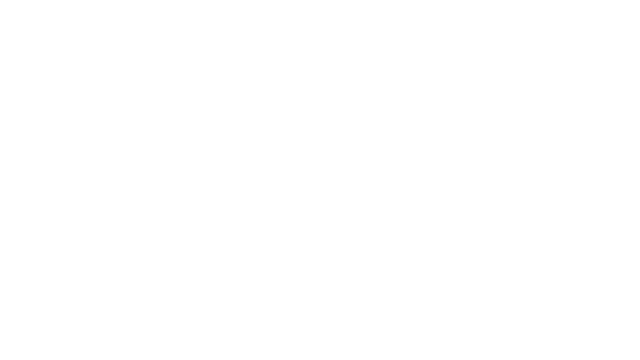 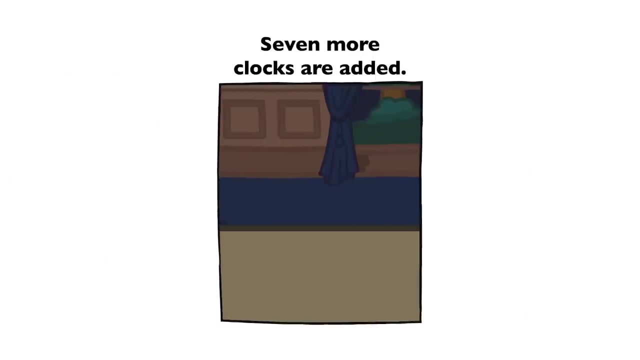 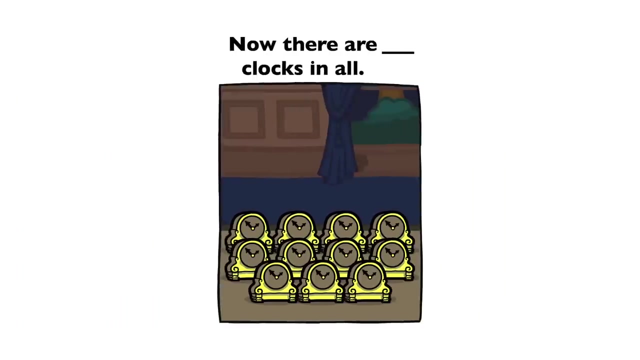 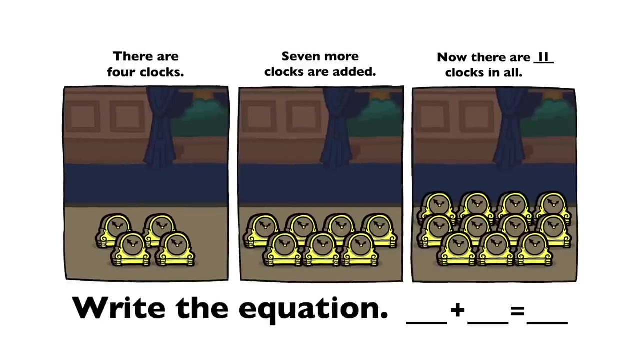 She makes a Deadpool, She makes, She makes a Four more. Now she has eight snowballs. Four plus four equals eight. There are four clocks. Seven more clocks are added. Now there are eleven clocks in all. Four plus seven equals eleven. 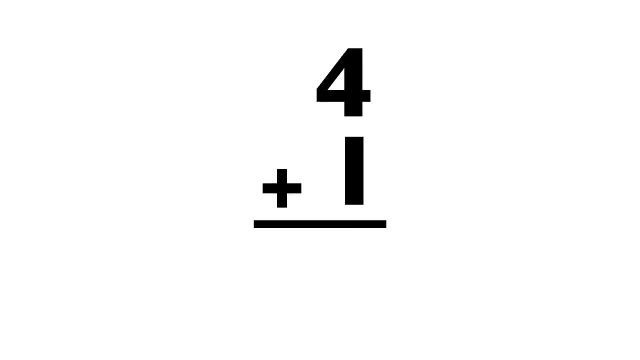 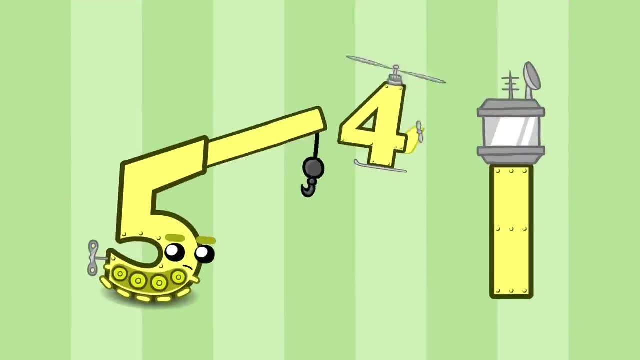 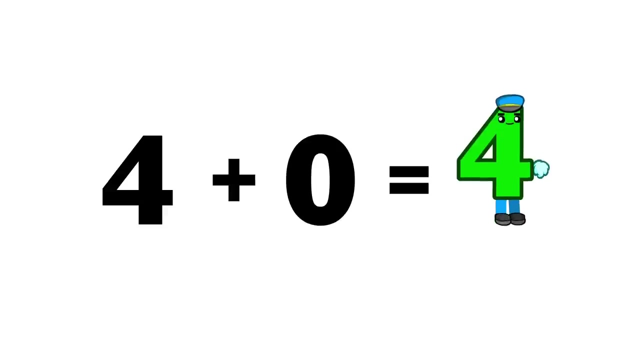 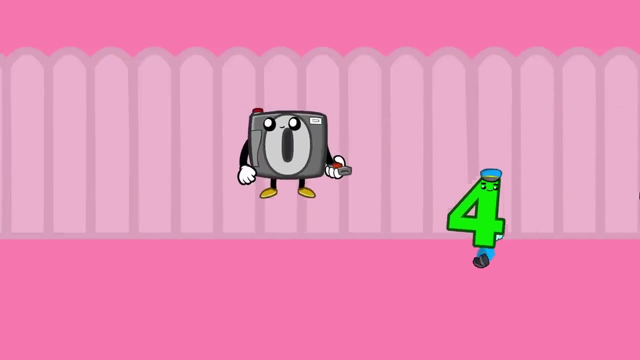 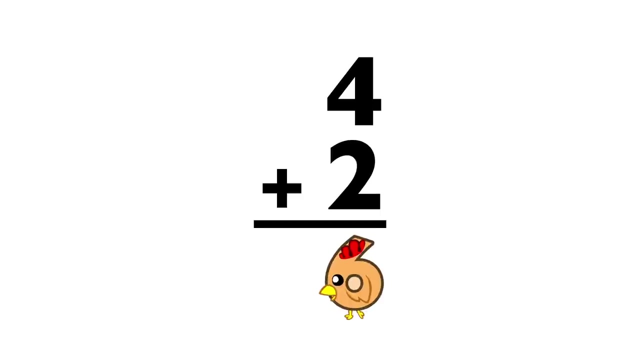 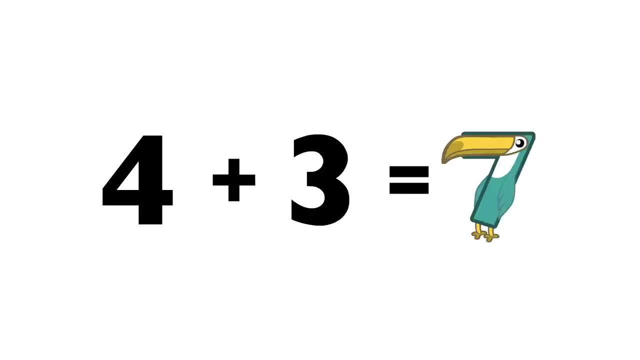 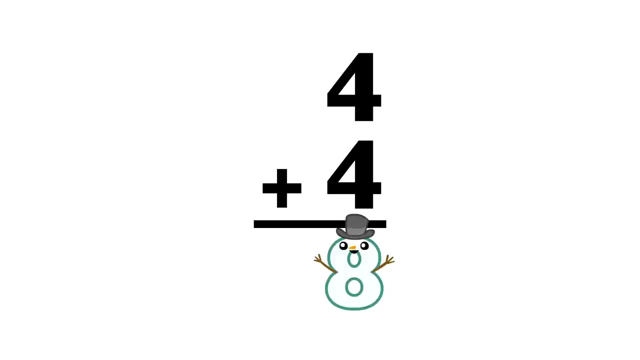 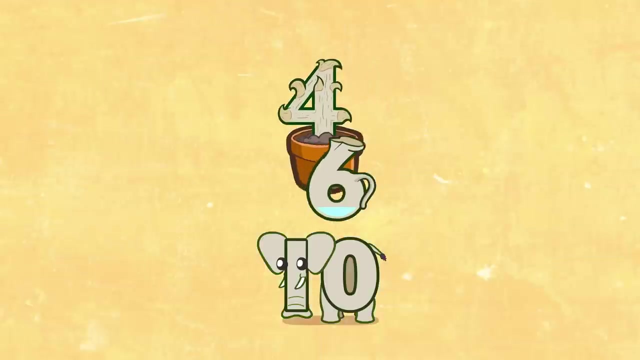 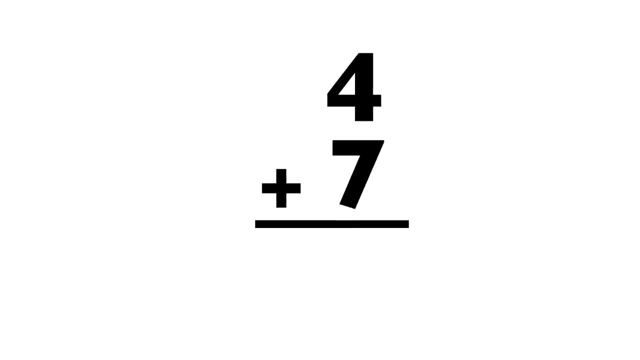 Four plus one equals five. Four plus zero equals four. Four plus two equals six. Four plus three equals seven. Four plus four equals eight. four plus five equals nine. four plus six equals ten. four plus seven equals eleven. 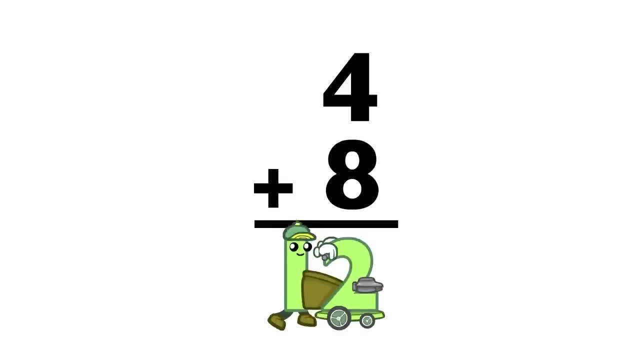 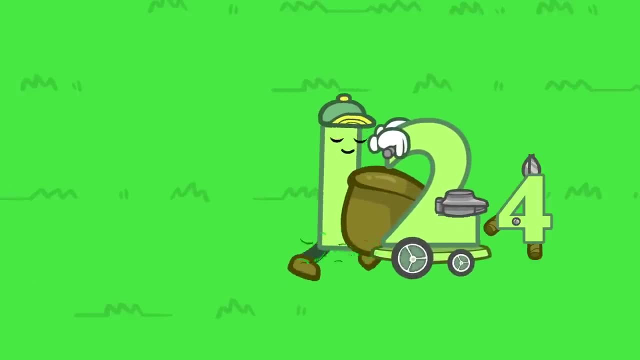 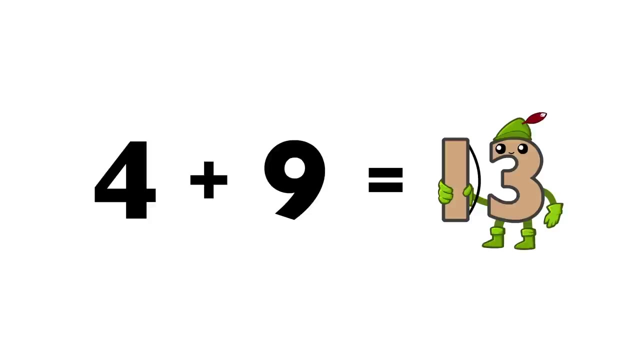 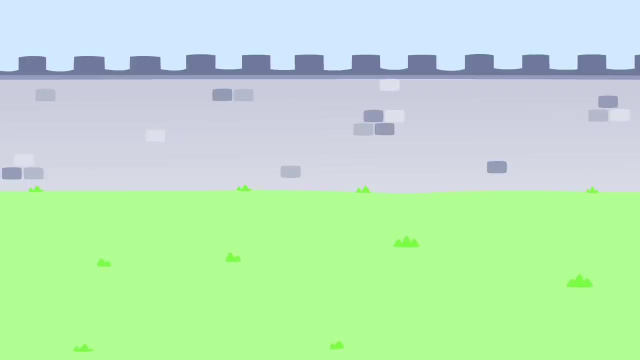 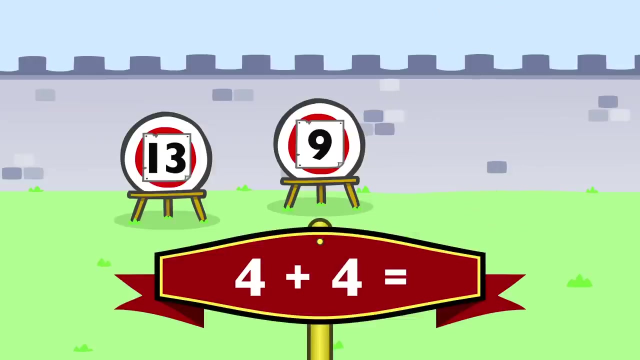 four plus eight equals twelve. four plus nine equals thirteen. four plus ten equals fourteen. four plus five equals eleven. four plus nine equals thirteen. four plus four equals eight. four plus nine equals thirteen. four plus five equals nine. four plus one equals five. four plus seven equals eleven. four plus ten equals fourteen. 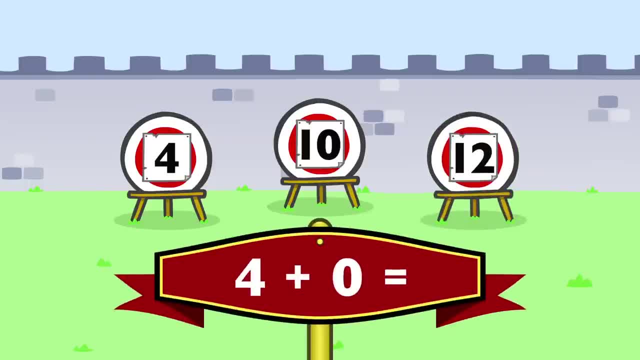 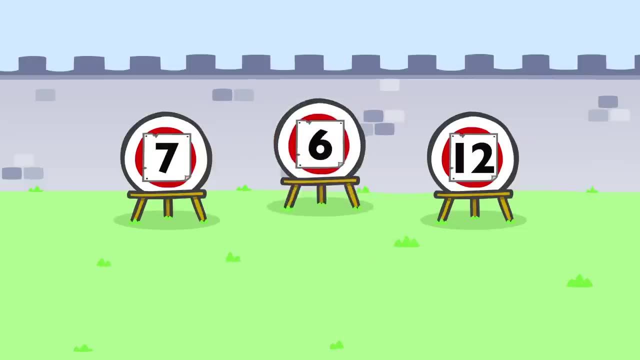 four plus zero equals four. four plus six. equals eleven. four plus ten equals fourteen four plus ten equals sixteen four plus ten. equals sixteen four plus ten. equals sixteen four plus ten. equals seventeen four plus ten equals seventeen four plus ten equals eighteen four plus ten. equals seventeen four plus ten. equals seventeen. 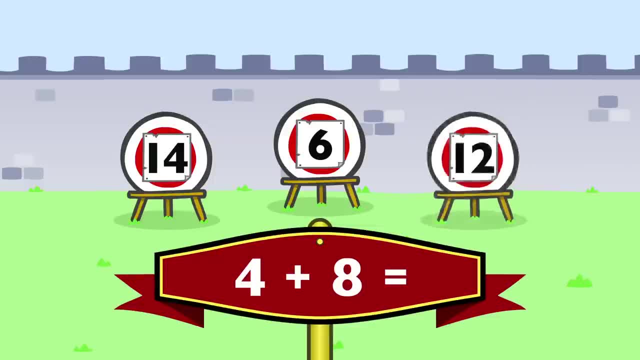 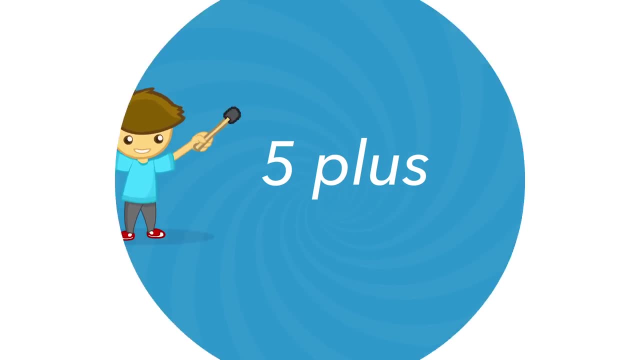 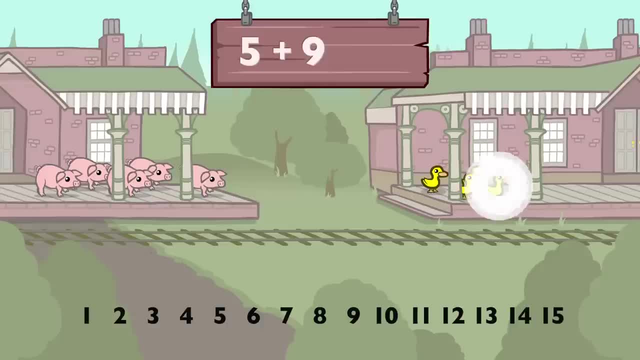 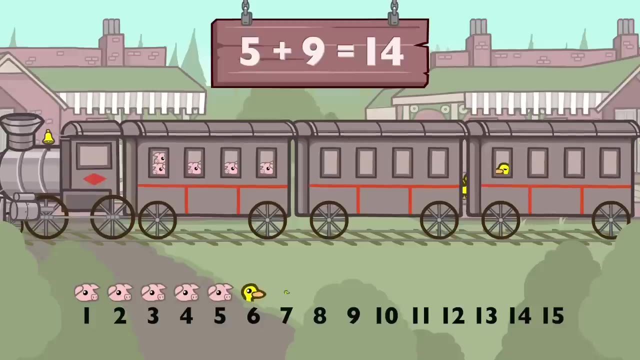 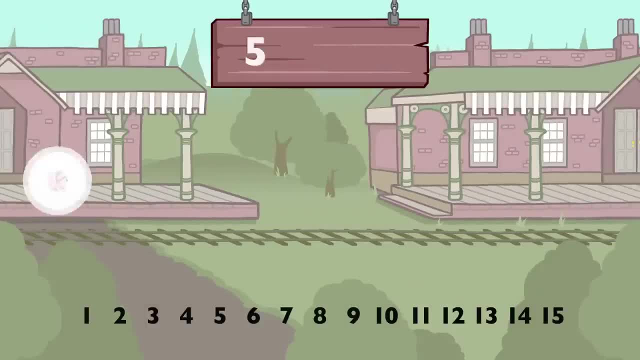 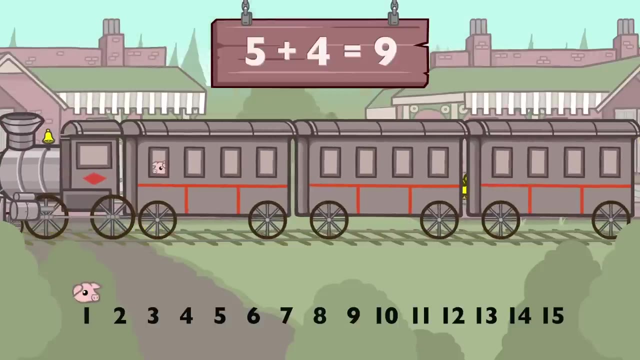 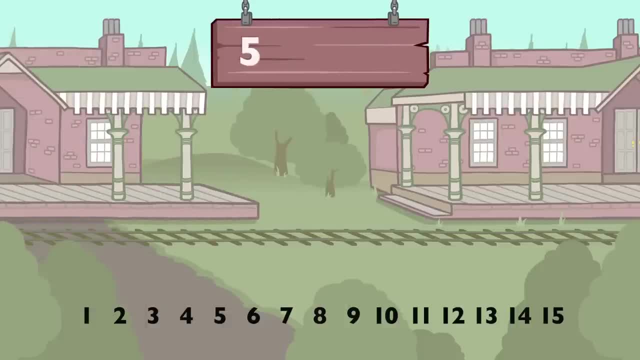 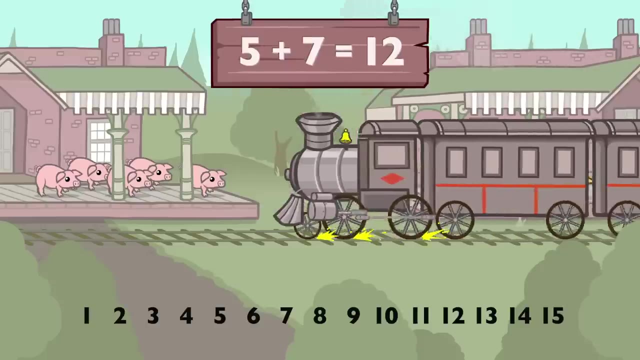 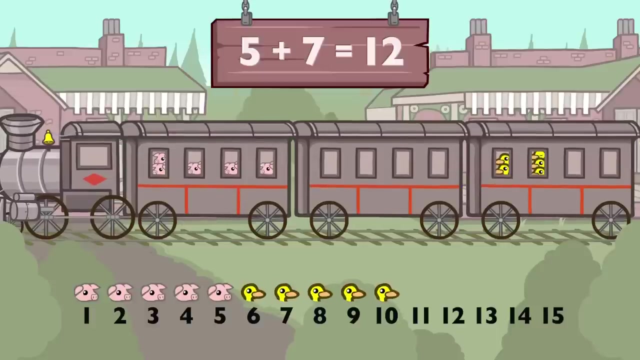 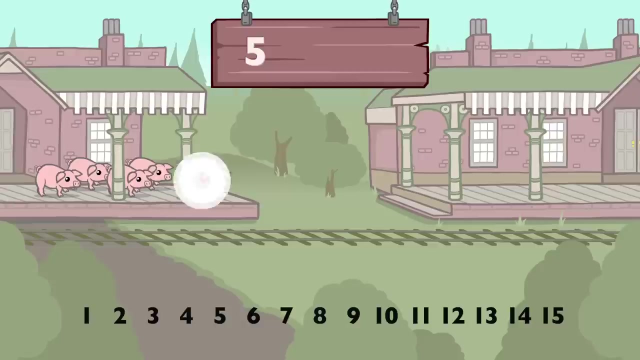 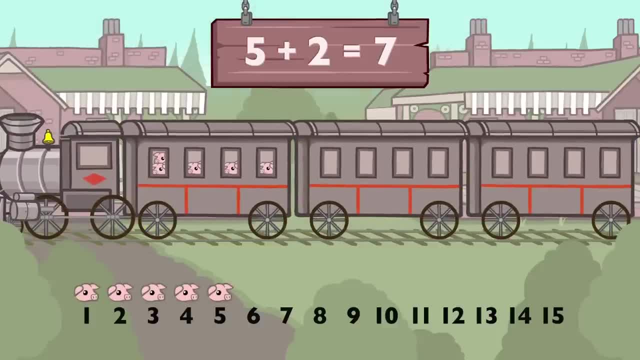 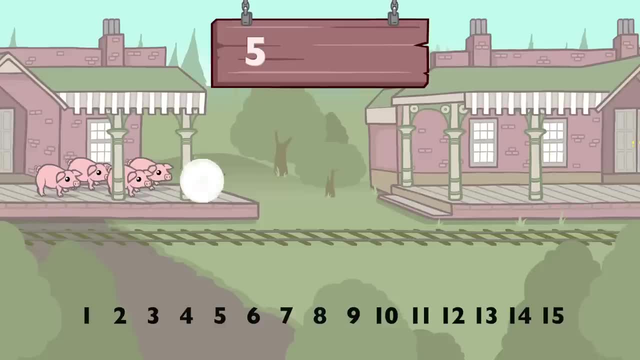 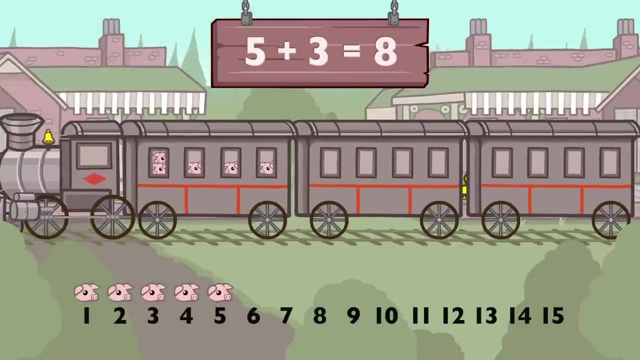 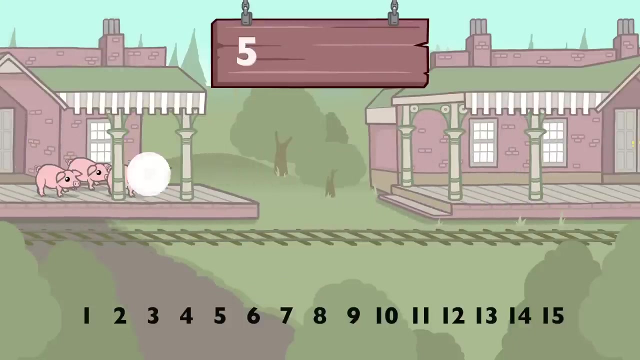 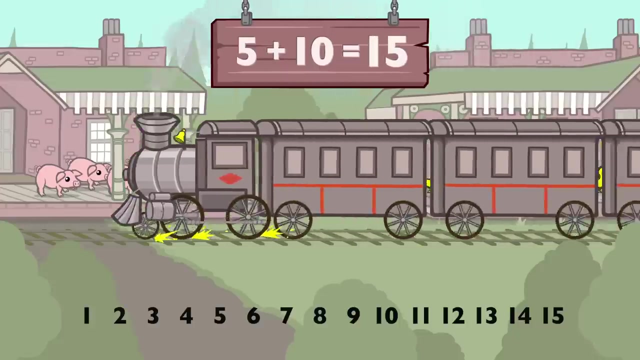 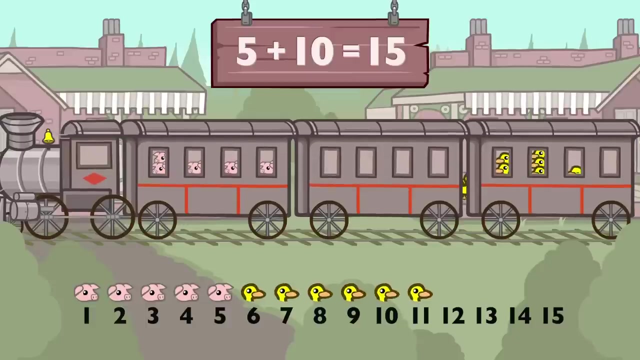 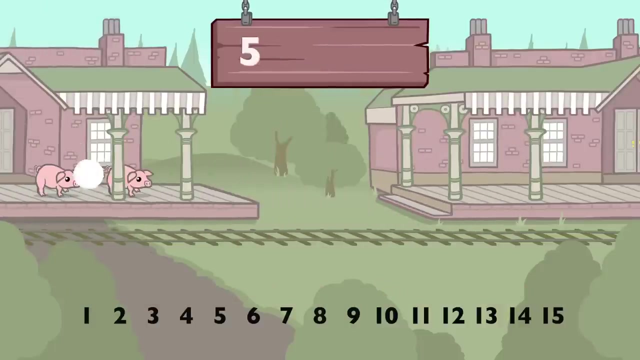 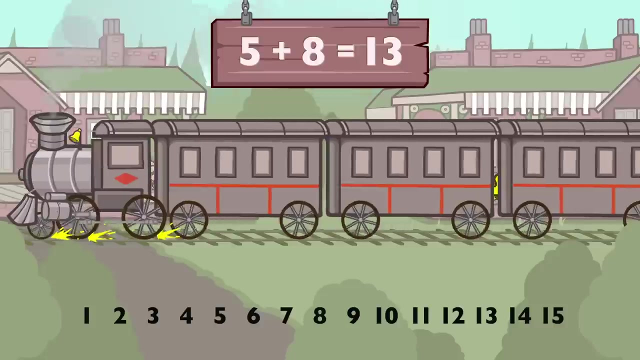 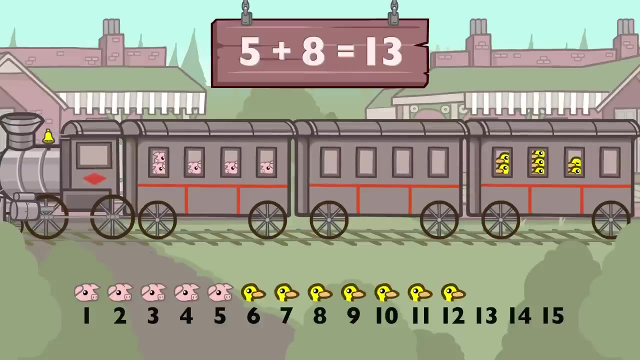 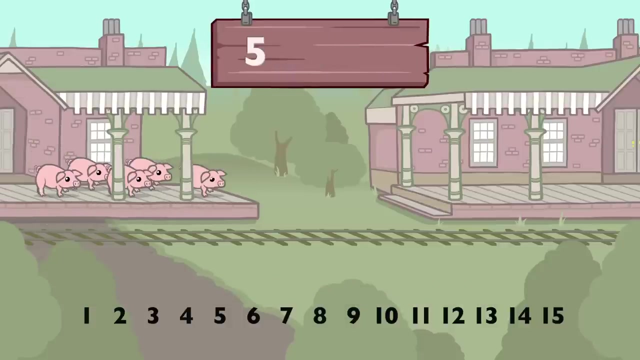 5 plus 3 equals 8. 5 plus 3 equals 8. 5 plus 10 equals 15. 5 plus 10 equals 15, 15. 15. Five plus eight equals thirteen. Five plus eight equals thirteen. Five plus zero equals five. 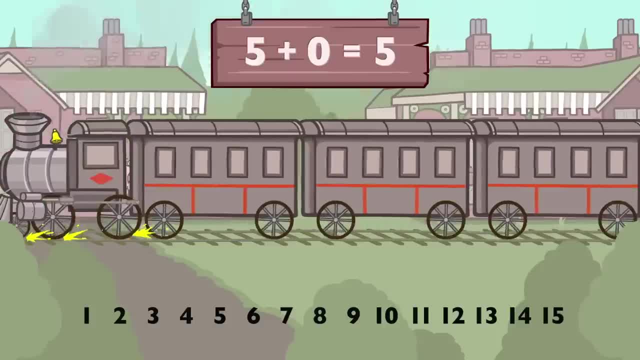 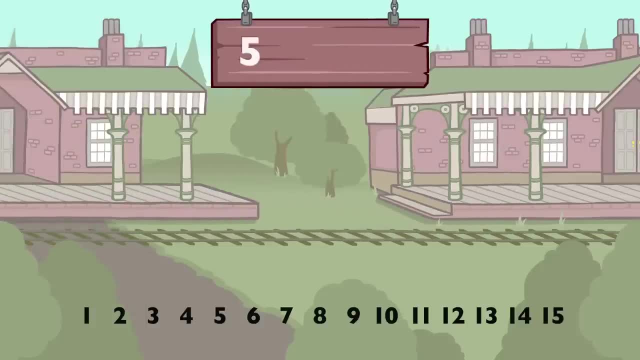 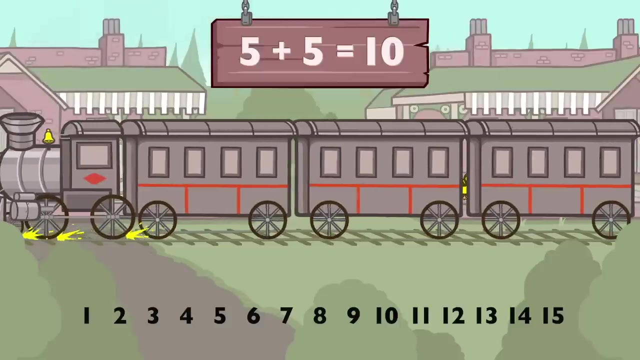 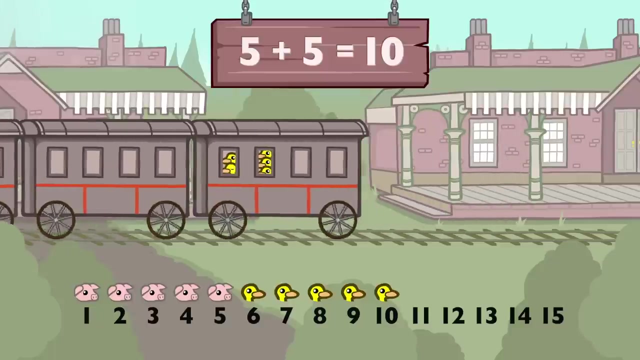 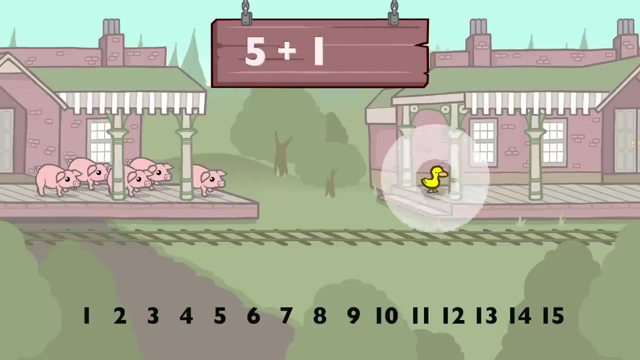 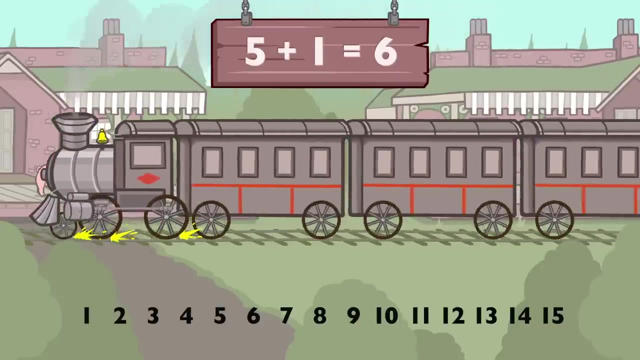 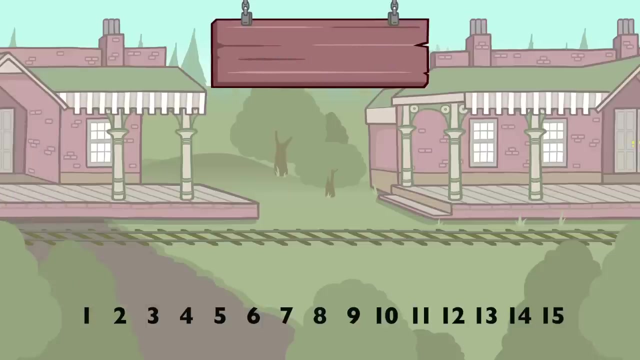 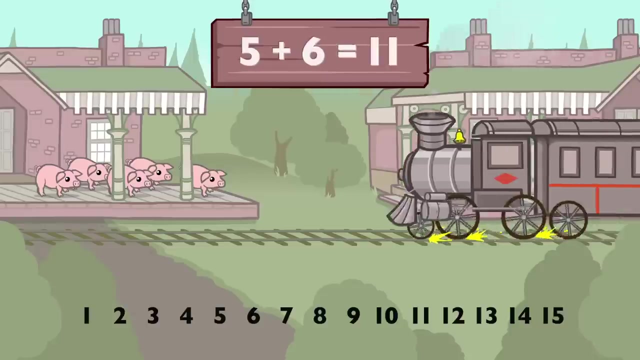 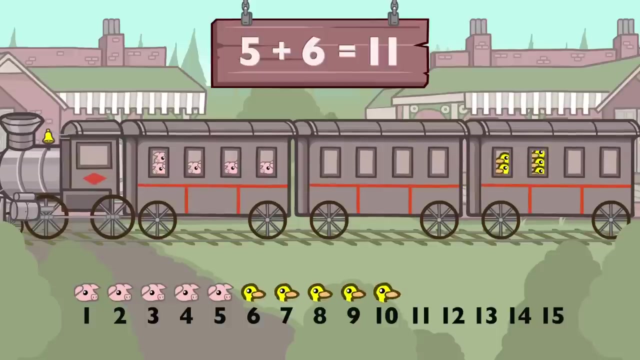 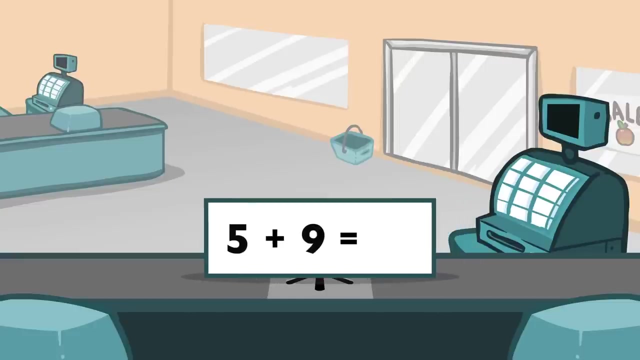 Five plus zero equals five. Five plus five equals ten. Five plus five equals ten. Five plus one equals six. Five plus one equals six. Five plus one equals six. Five plus six equals eleven. Five plus six equals eleven. Five plus nine equals. Five plus nine equals fourteen. Five plus one equals six. 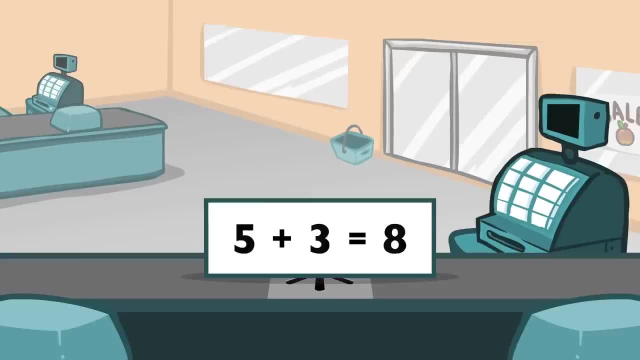 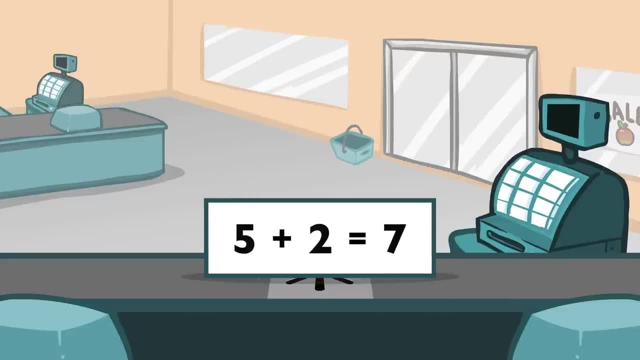 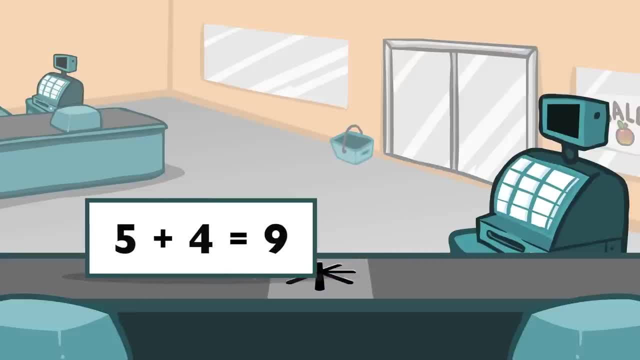 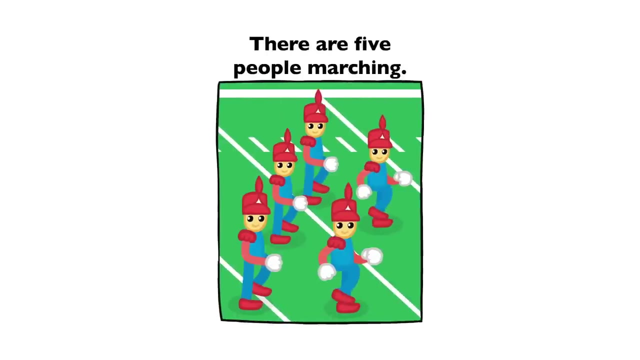 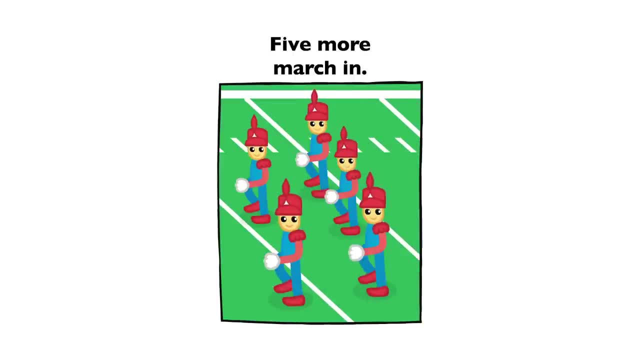 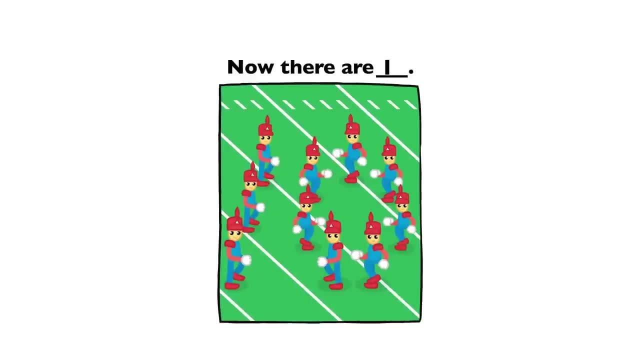 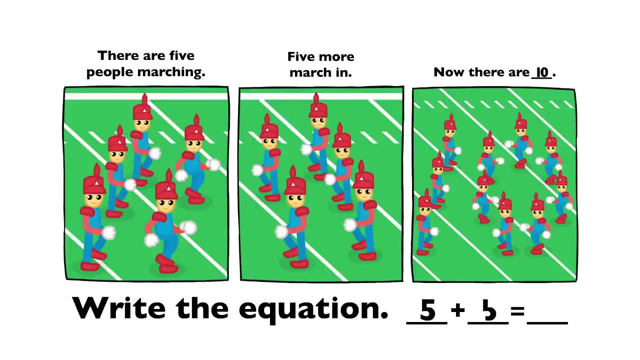 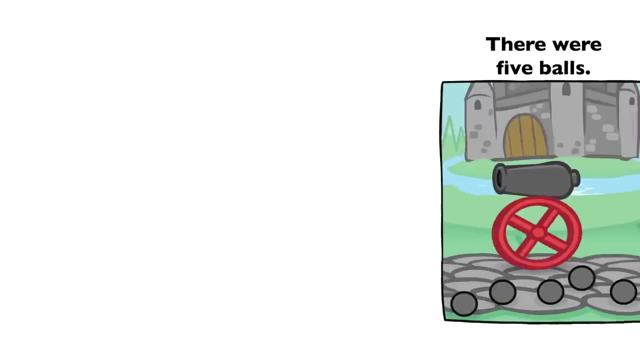 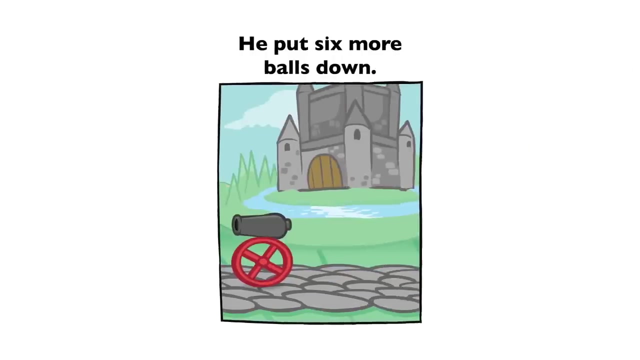 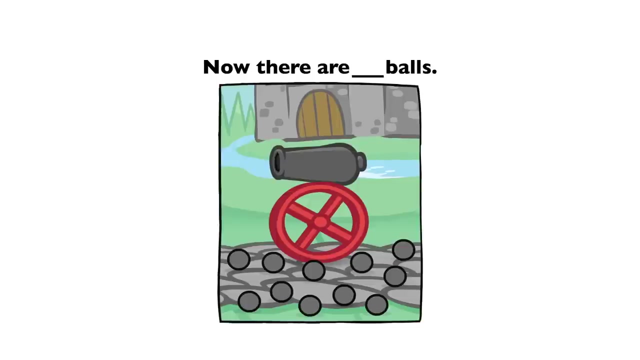 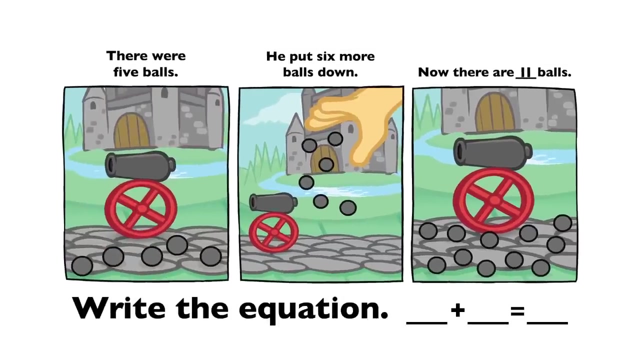 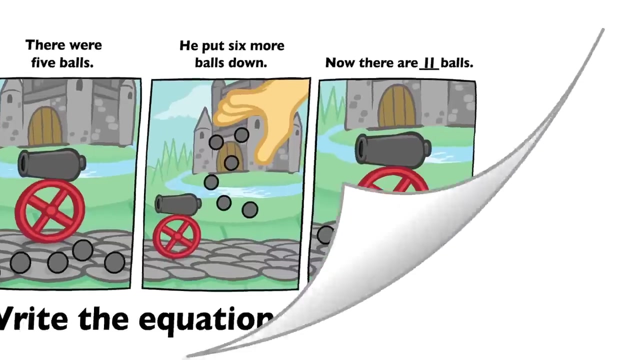 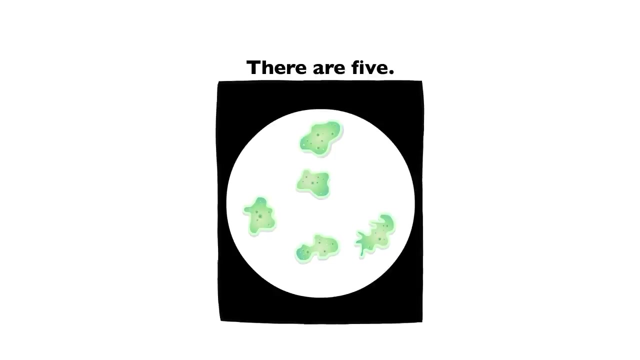 Five plus ten equals sixteen more march in. Now there are ten. Five plus five equals ten. There were five balls. He put six more balls down. Now there are eleven balls. Five plus six equals eleven. There are five. Eight more appear. 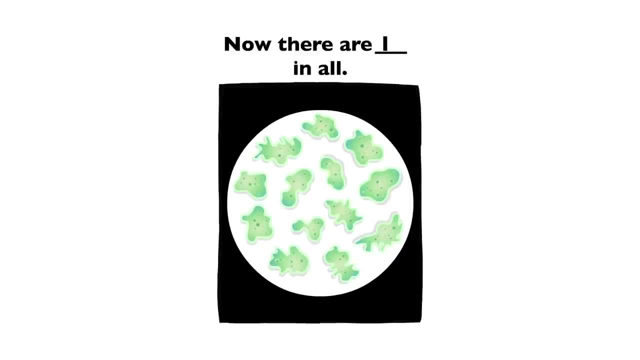 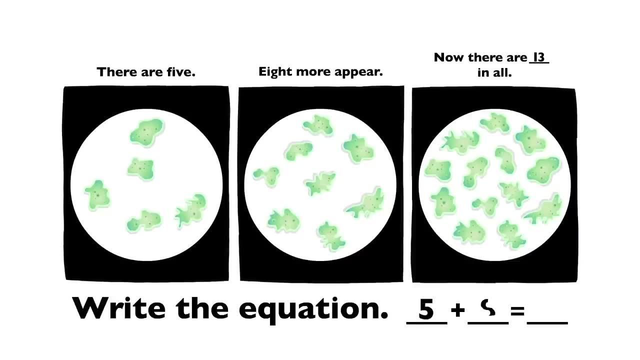 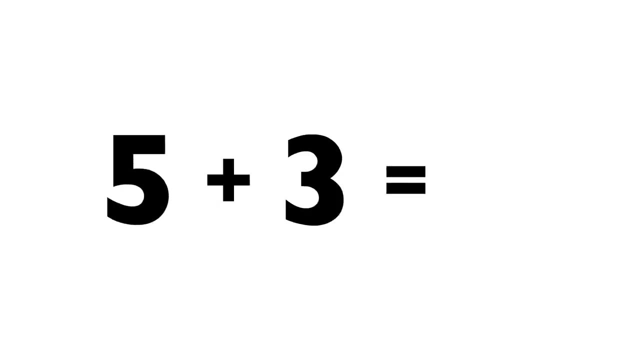 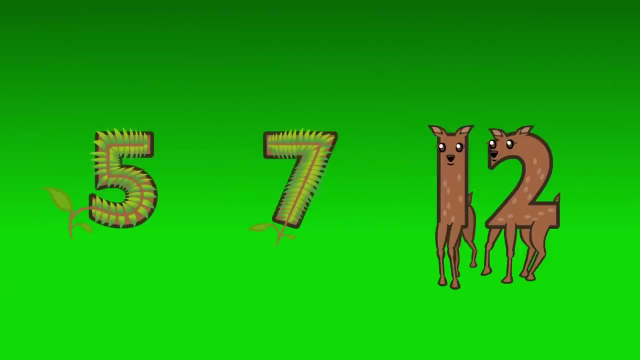 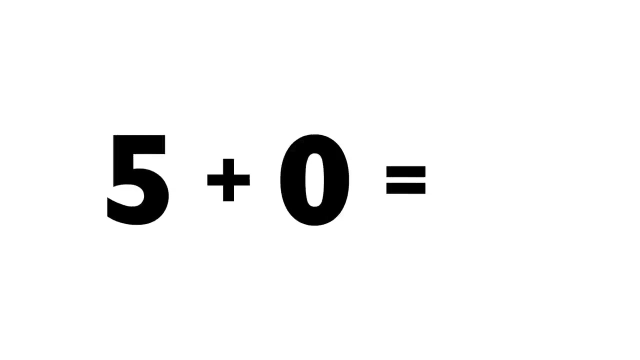 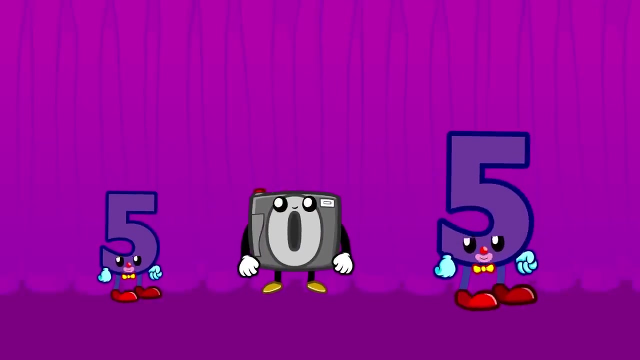 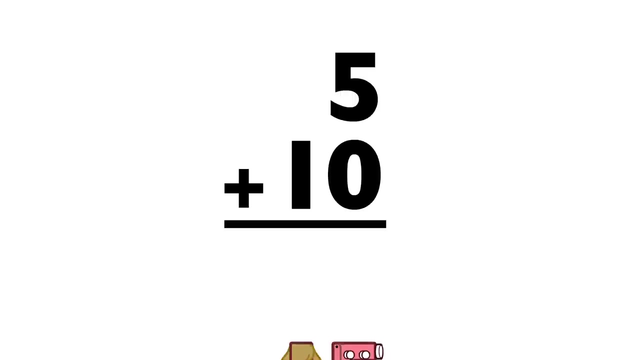 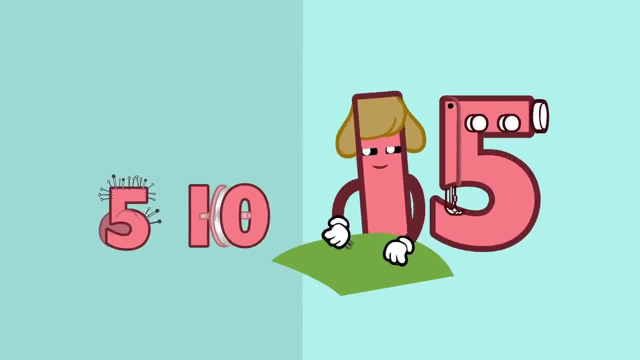 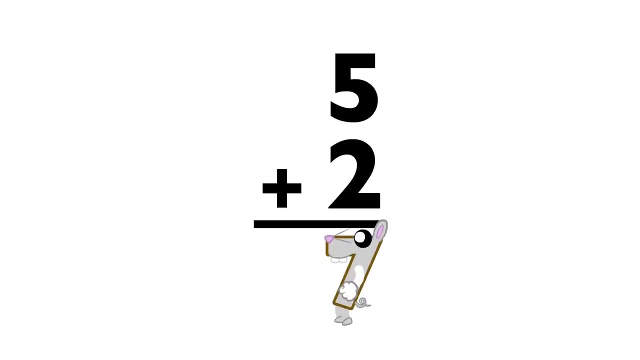 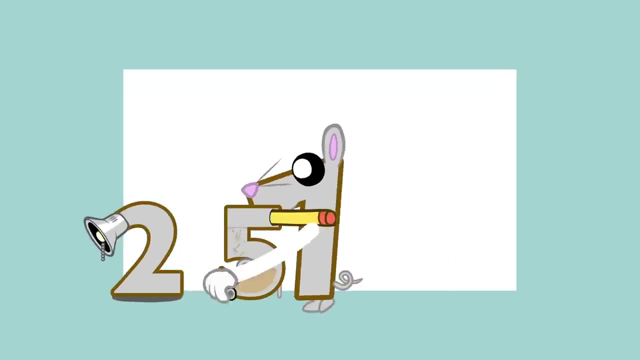 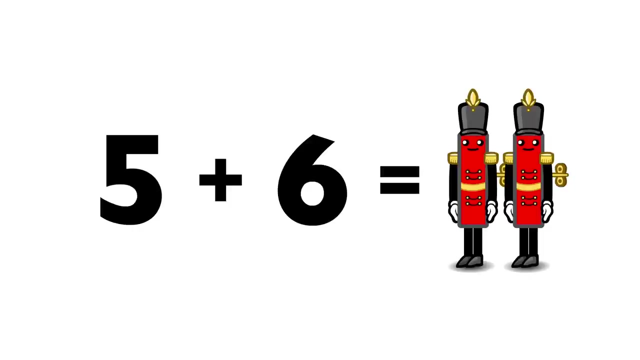 Now there are thirteen in all. Five plus eight equals thirteen. Five plus three equals eight. Five plus seven equals twelve. Five plus zero equals eight. Five. Five plus ten equals fifteen. Five plus two equals seven. Five plus three equals four. Five plus six equals. 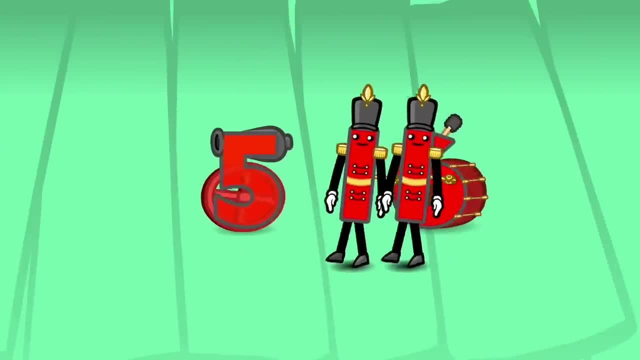 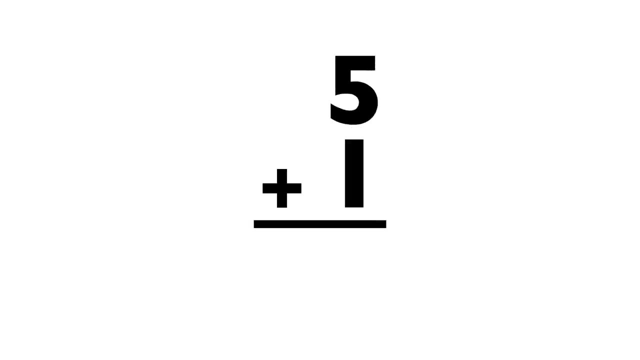 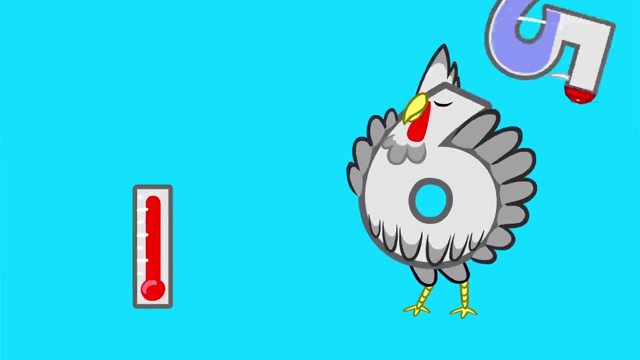 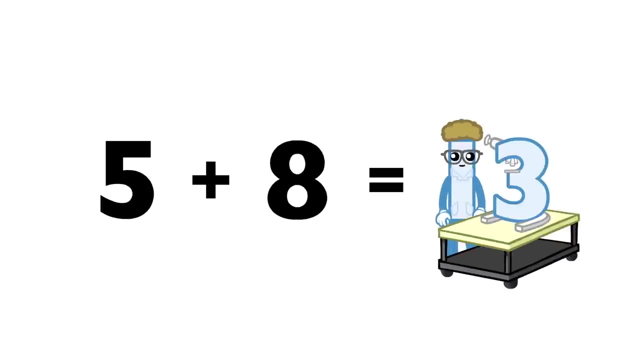 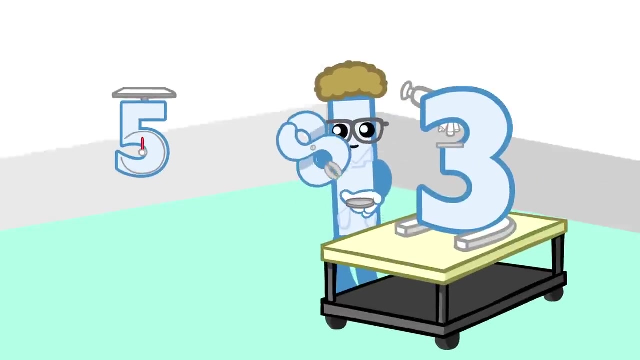 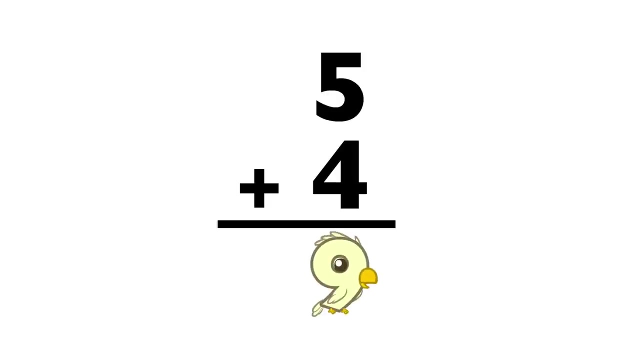 eleven. Five plus one equals six, Six. Yes, Five. Five plus one equals six. 5 plus 8 equals 13.. 5 plus 4 equals 9.. 5 plus 9 equals 14.. 5 plus 5 equals 10.. 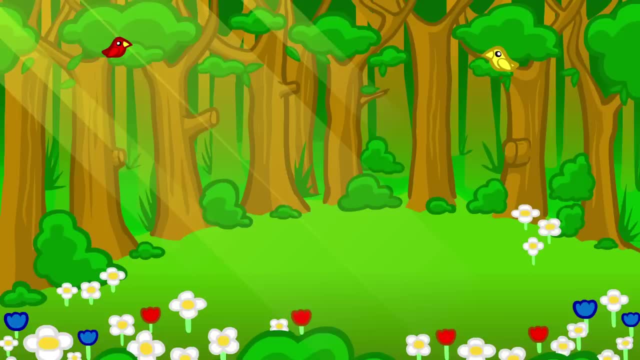 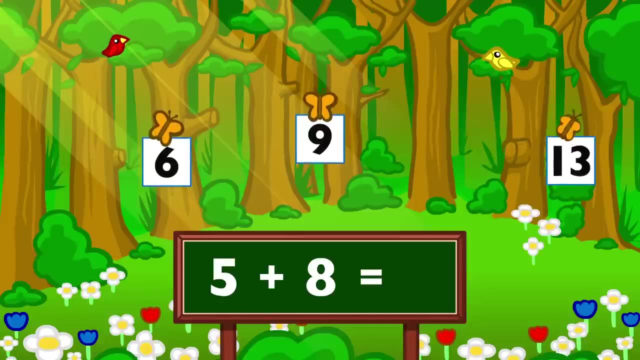 5 plus 8 equals 13.. 5 plus 1 equals 6.. 5 plus 4 equals 9.. 5 plus 4 equals 10.. 5 plus 4 equals 6- equals 11.. 5 plus 2 equals 7.. 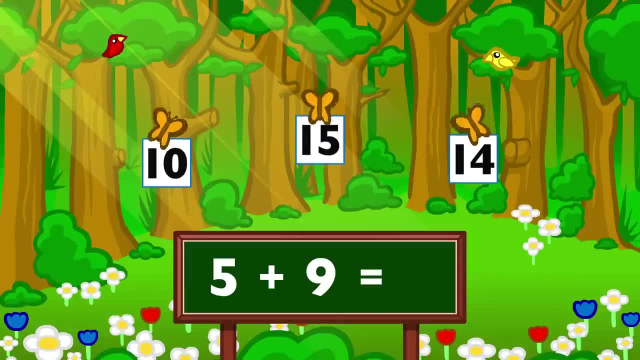 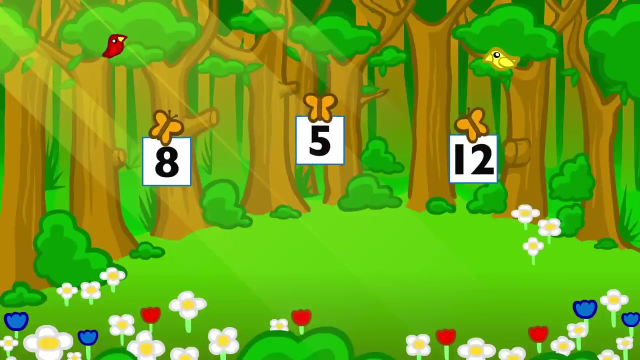 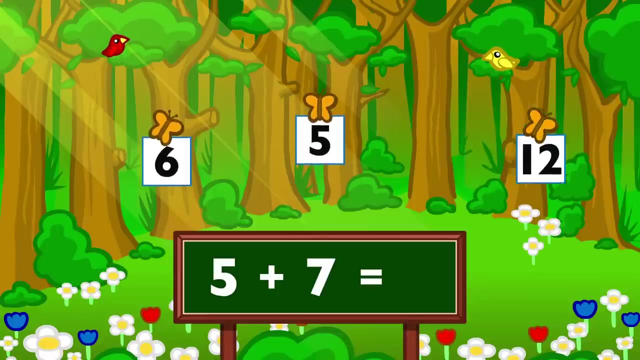 5 plus 9 equals 14.. 5 plus 5 equals 10.. 5 plus 10 equals 15.. 5 plus 3 equals 8.. 5 plus 7 equals 12.. 5 plus 0 equals 5.. 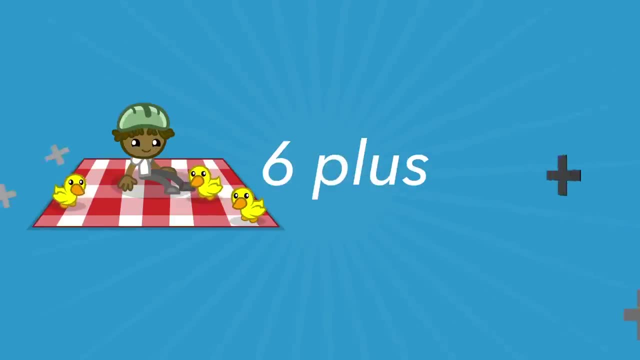 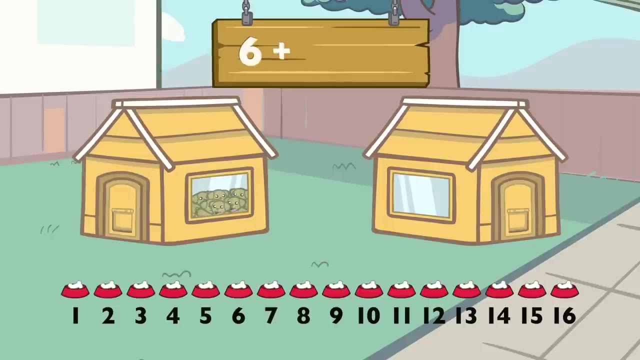 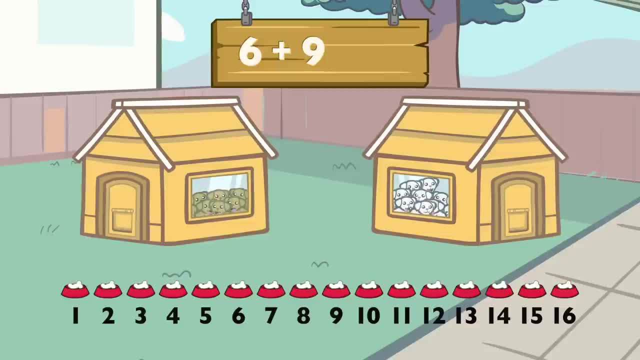 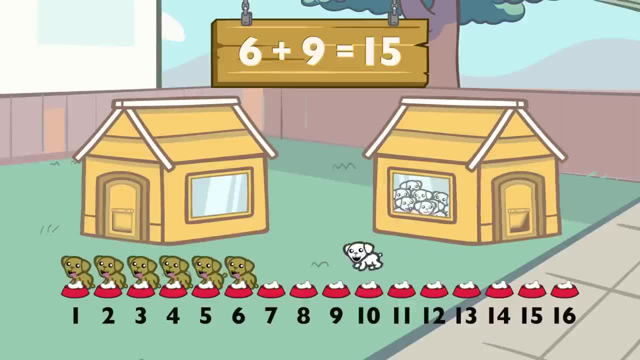 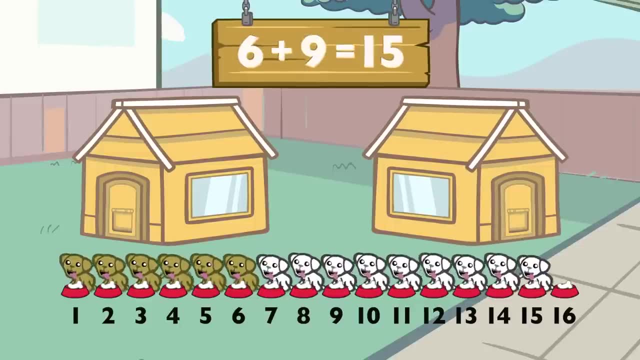 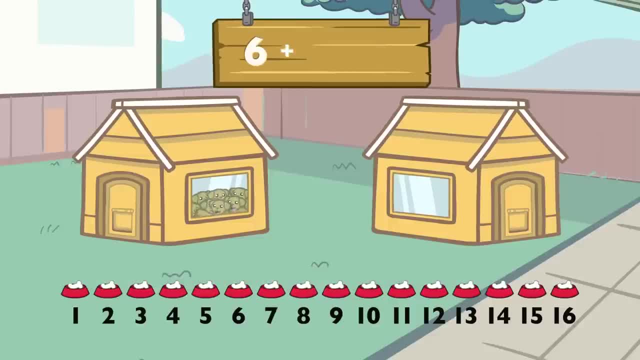 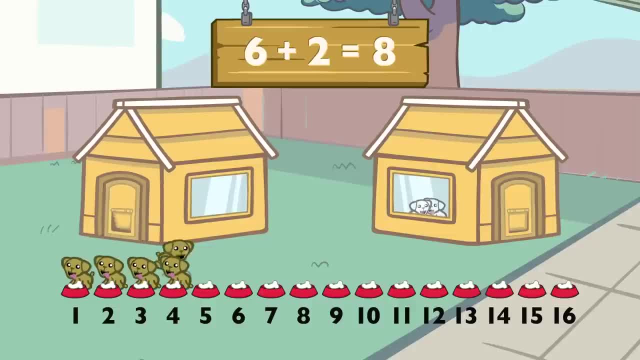 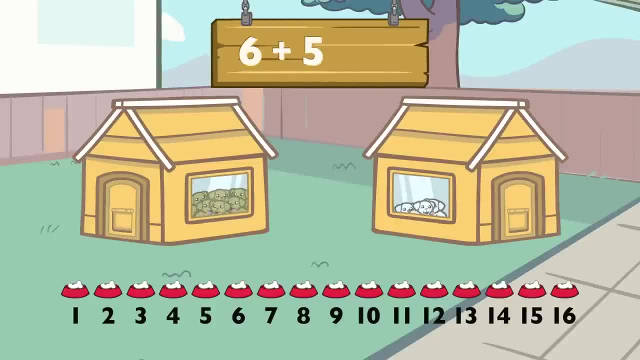 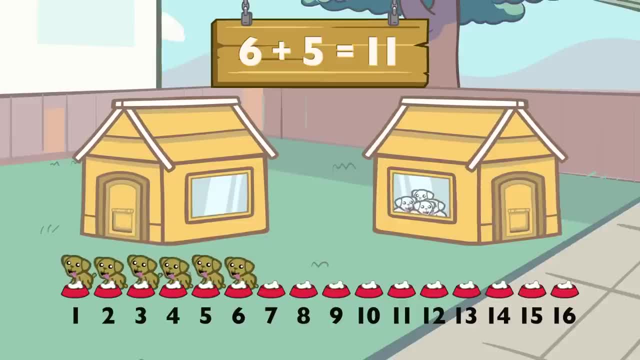 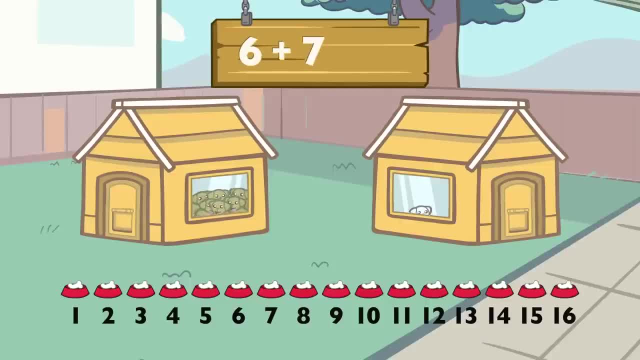 6 plus 9 equals 15. Plus 7 equals 13.. 6 plus 7 equals 13.. 6 plus 1 equals 7.. 6 plus 1 equals 7.. 6 plus 4 equals 10.. 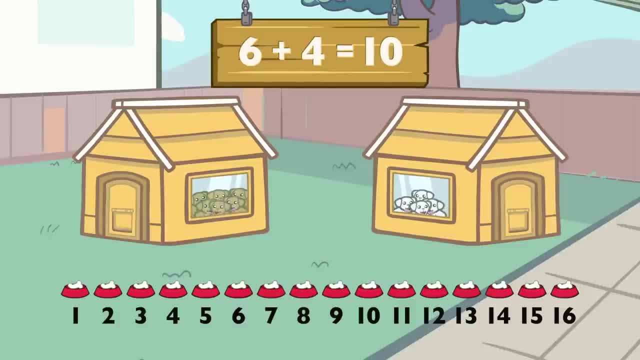 6 plus 4 equals 10.. 6 plus 10. 10 equals 16.. 6 plus 10 equals 16.. 6 plus 3 equals 10.. 6 plus 3 equals 10.. 3 equals 9.. 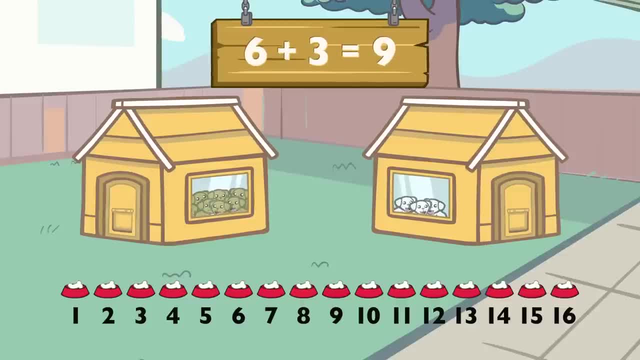 6 plus 3 equals 9.. 6 plus 6 equals 12.. 6 plus 6 equals 12.. 6 plus 6 equals 12.. 6 plus 8 equals 14.. 6 plus 8 equals 14.. 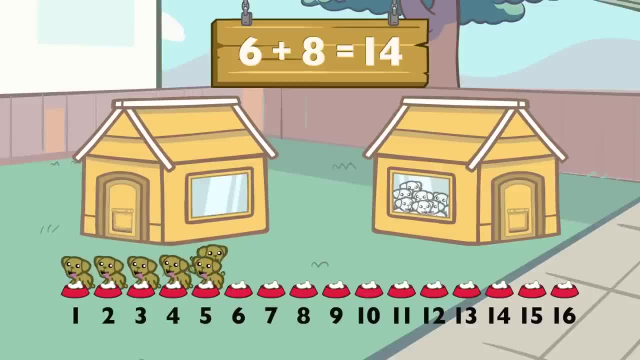 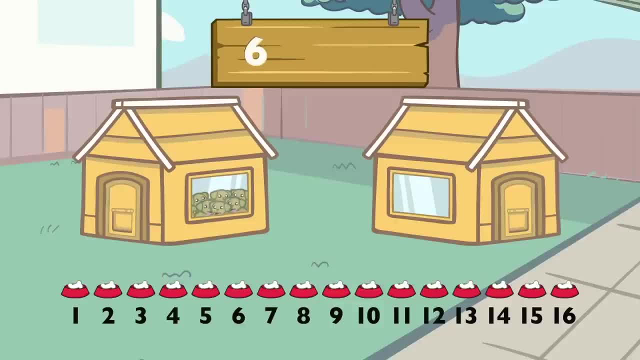 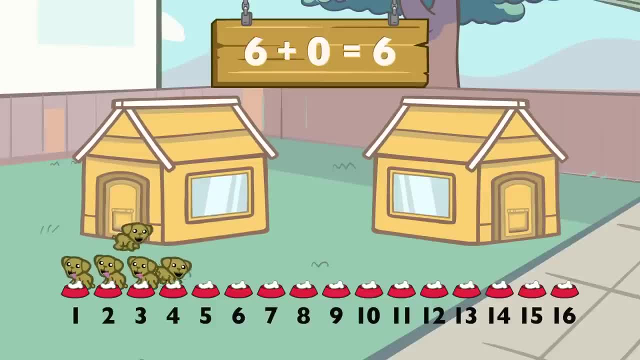 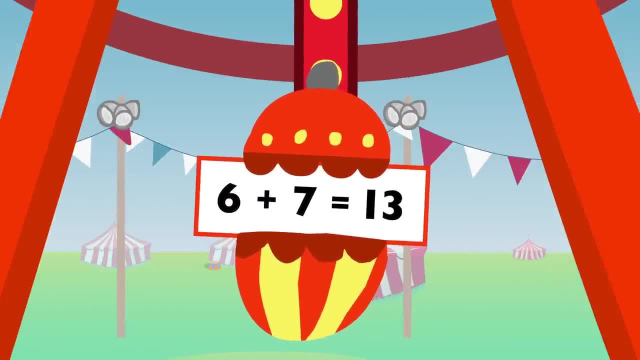 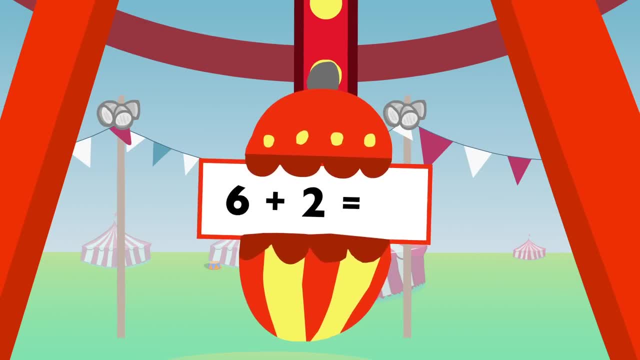 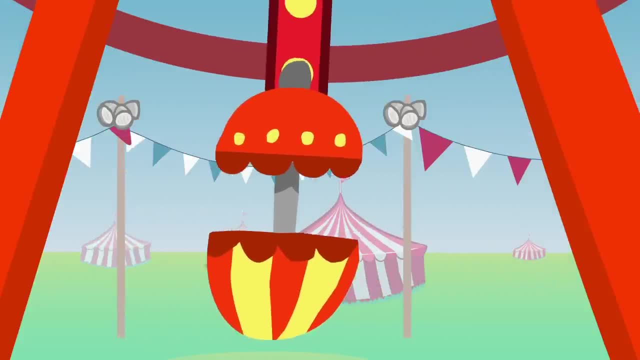 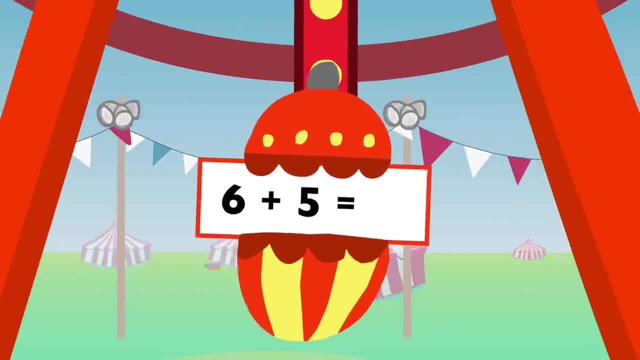 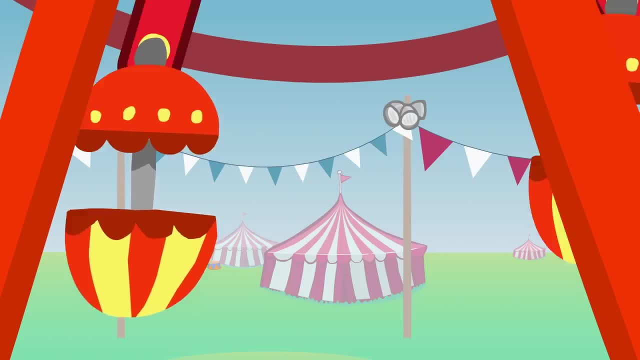 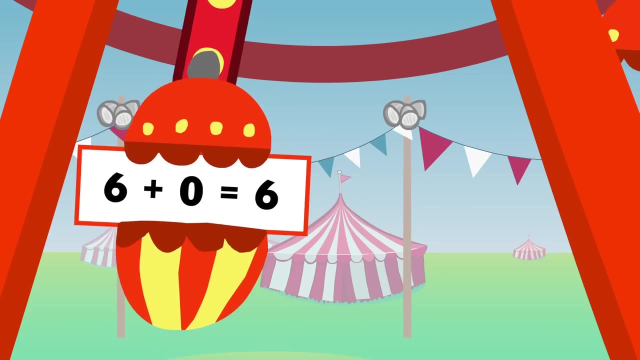 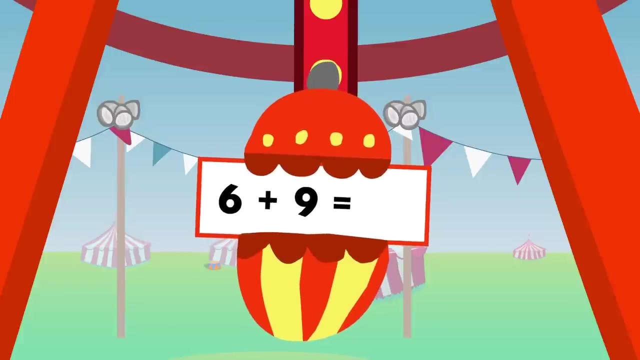 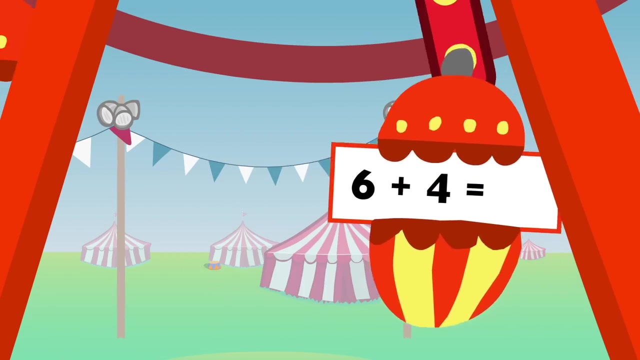 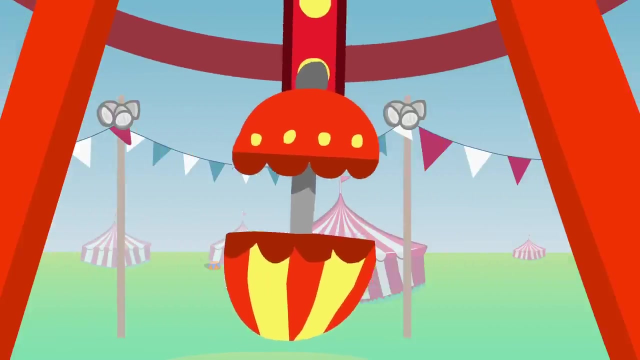 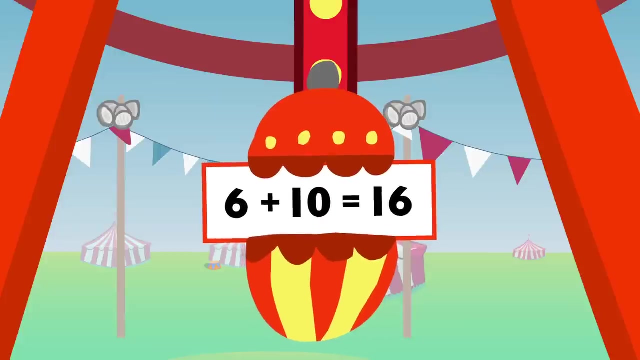 6 plus 7 equals 14.. 6 plus 0 equals 6.. 6 plus 9 equals 15.. 6 plus 4 equals 10.. 6 plus 4 equals 10.. 6 plus 10 equals 16.. 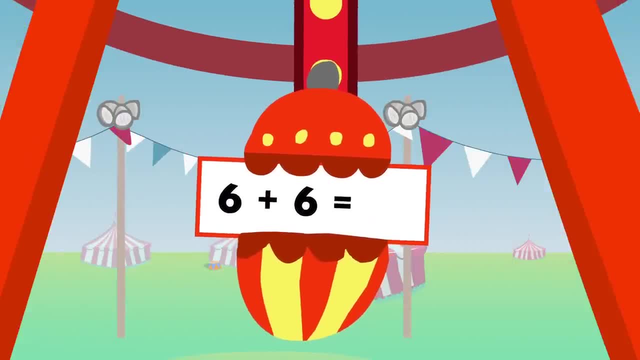 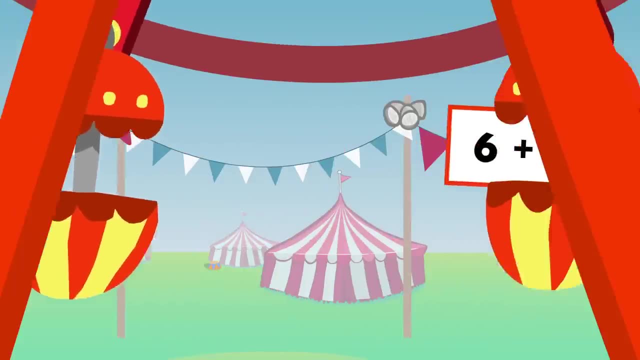 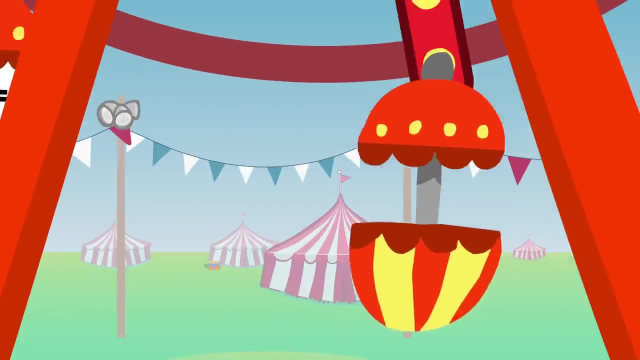 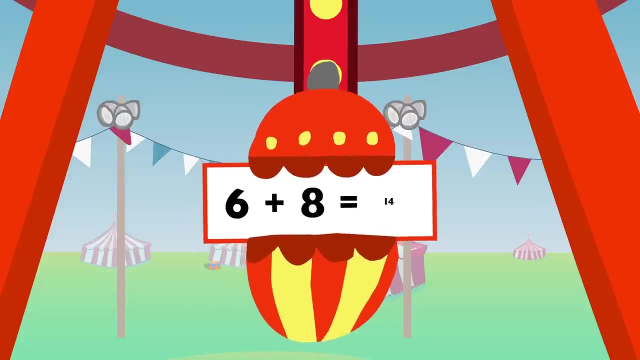 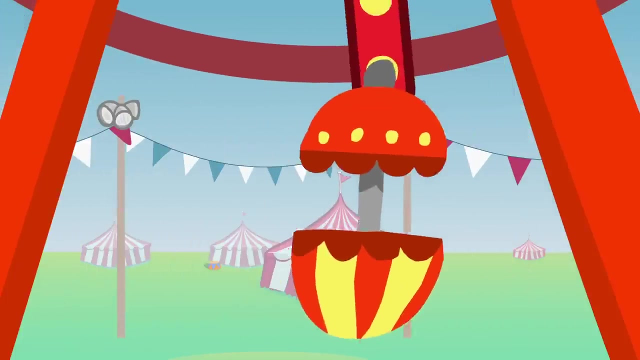 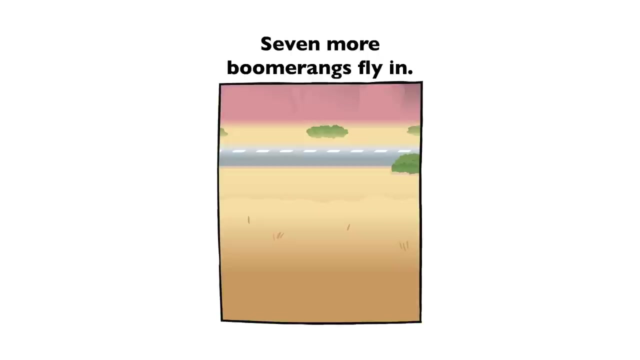 6 plus 6 equals 12.. 6 plus 1 equals 7.. 6 plus 8 equals 14.. 6 plus 3 equals 9.. There are six boomerangs, 7 more boomerangs, 7 more boomerangs. fly in. 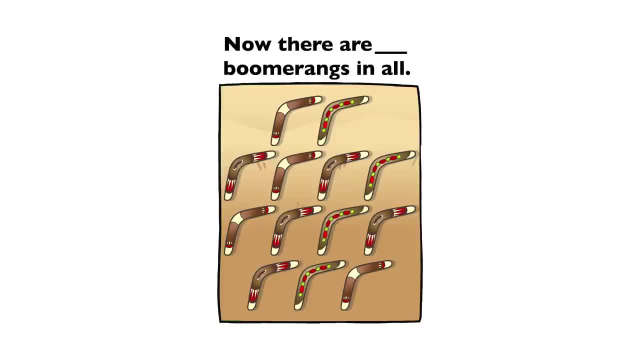 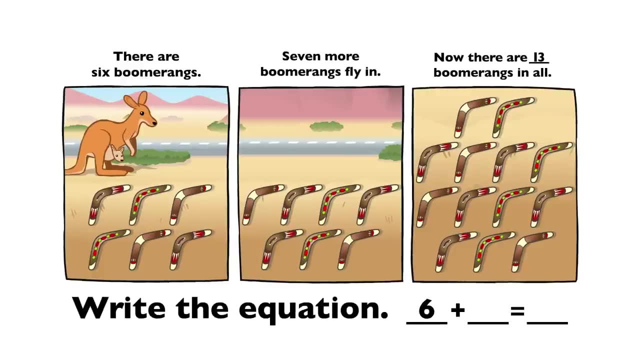 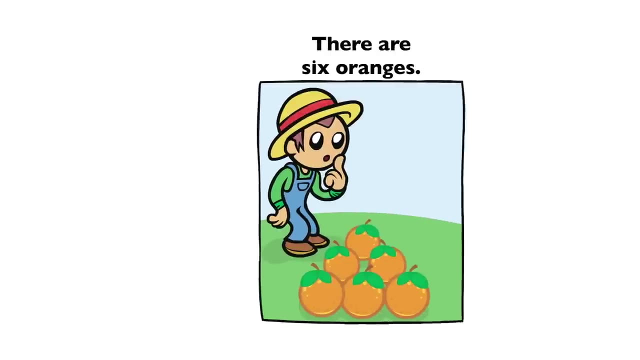 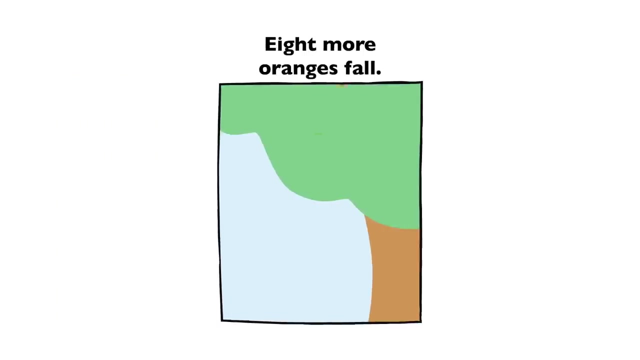 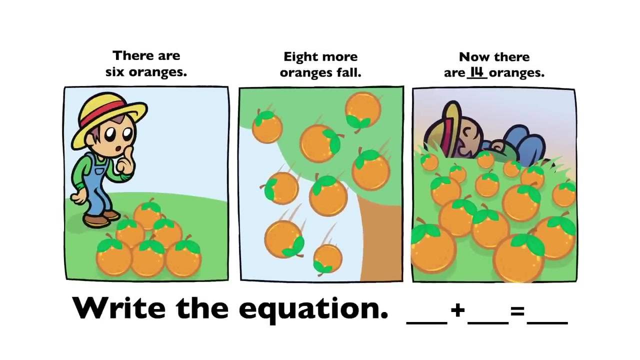 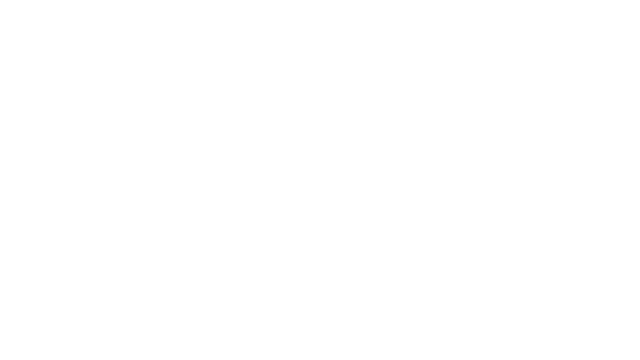 Now there are 13 boomerangs in all. 6 plus 7 equals 13.. There are six oranges. 8 more oranges fall. Now there are 14 oranges. 6 plus 8 equals 14.. There are six peeks. 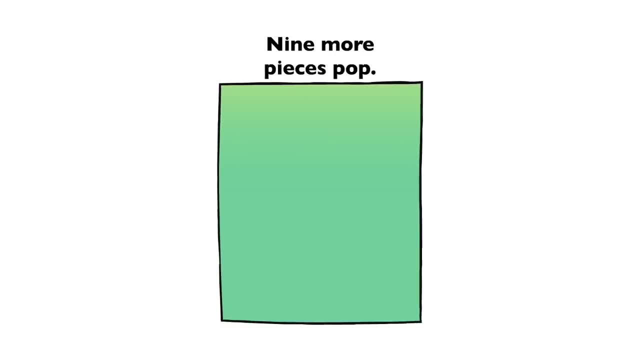 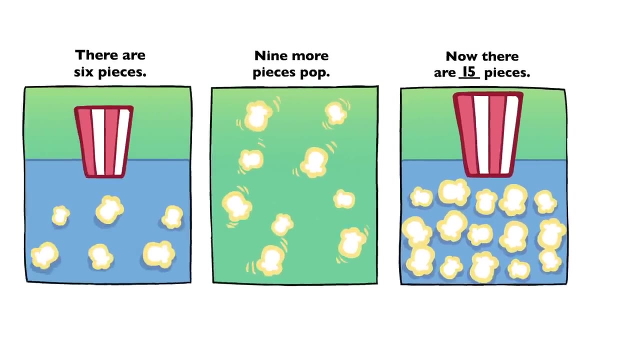 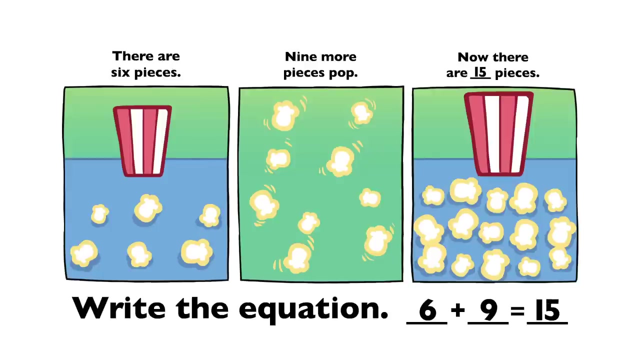 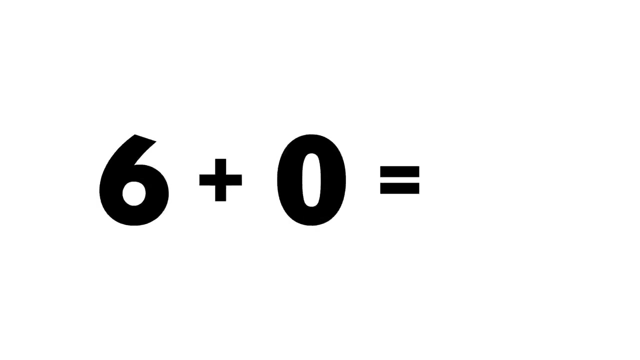 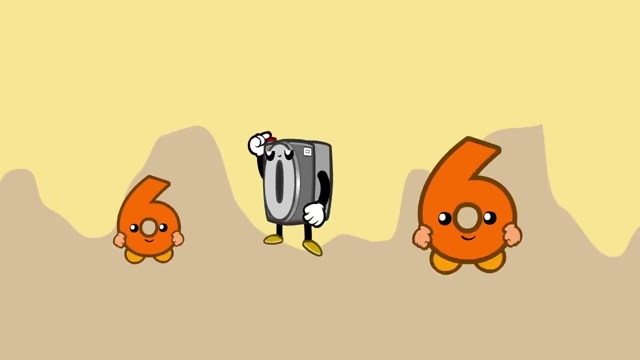 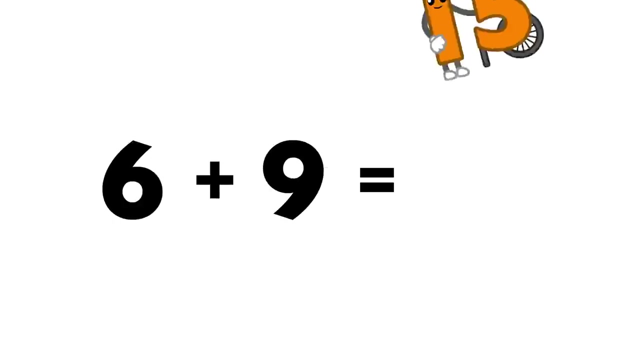 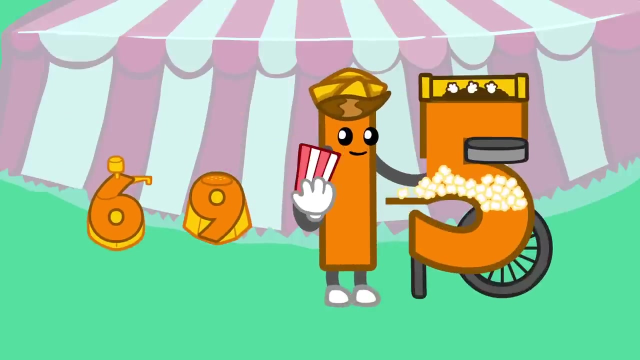 6 plus 8 equals 14.. There are six peeks: 6 plus 8 equals 14.. pieces: Nine more pieces pop. Now there are fifteen pieces. Six plus nine equals fifteen. Six plus zero equals six. Six plus nine equals fifteen. 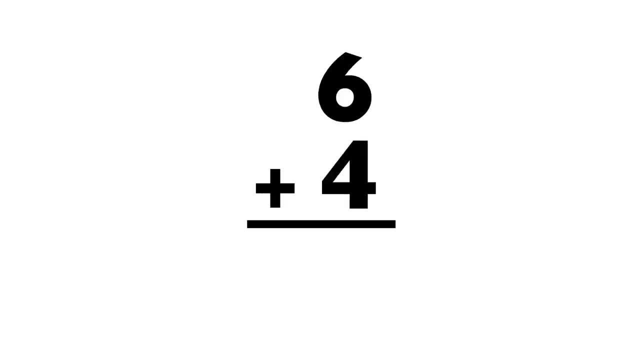 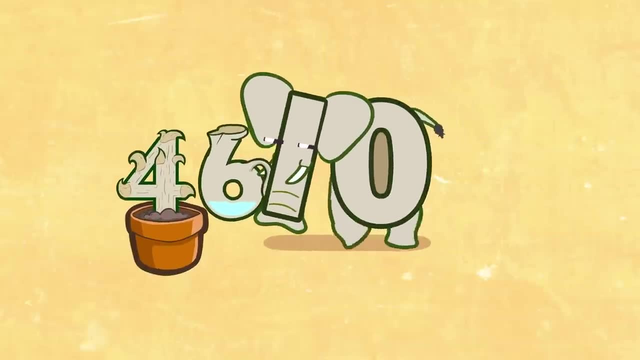 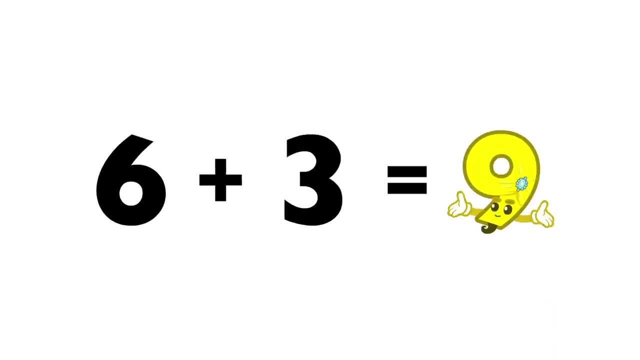 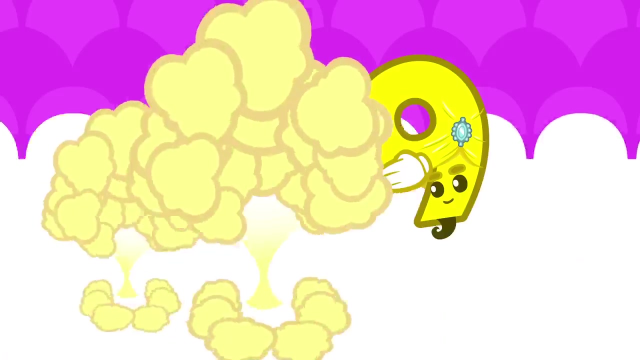 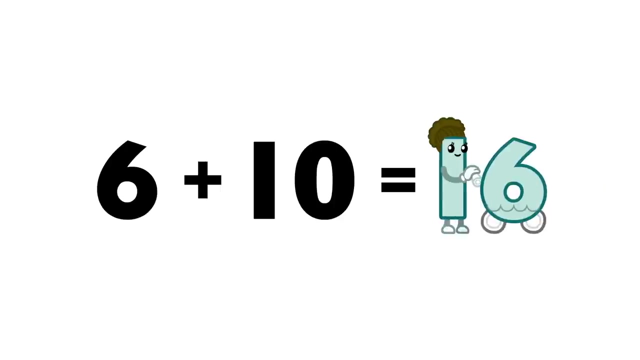 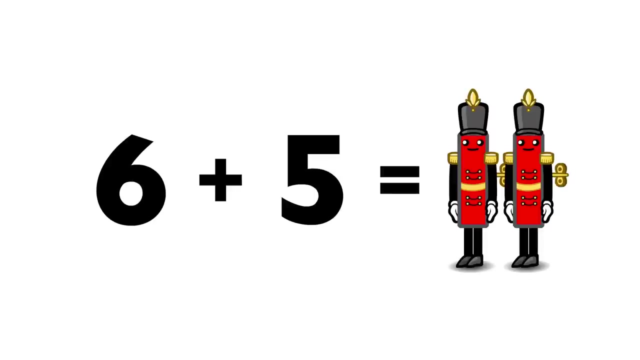 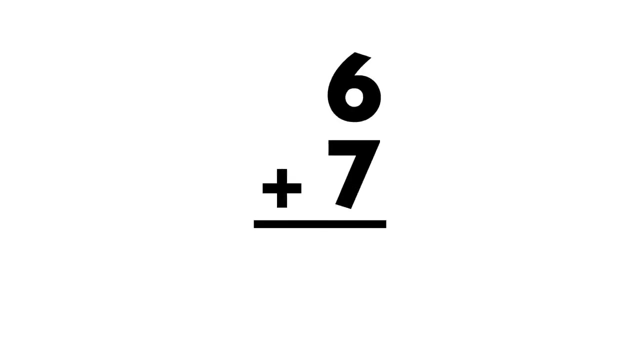 Six plus four equals ten. Six plus three equals nine. Six plus ten equals sixteen. Six plus five equals eleven. Six plus seven equals twenty-one. Six plus ten equals twenty-one One. Oh no, Six plus seven equals twenty-one. Six plus ten equals twenty-one. 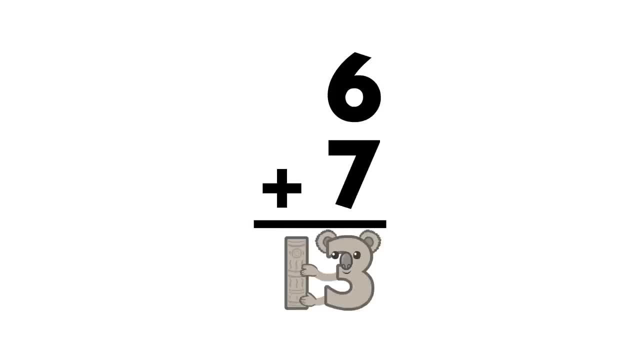 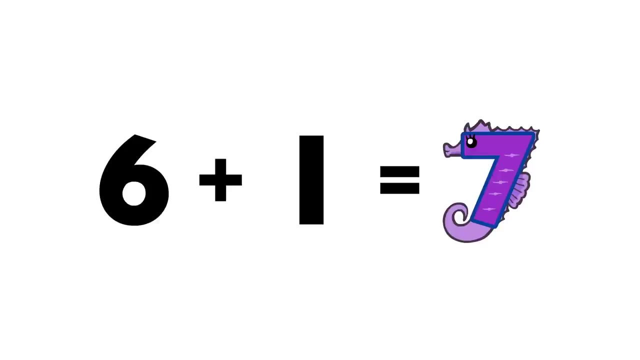 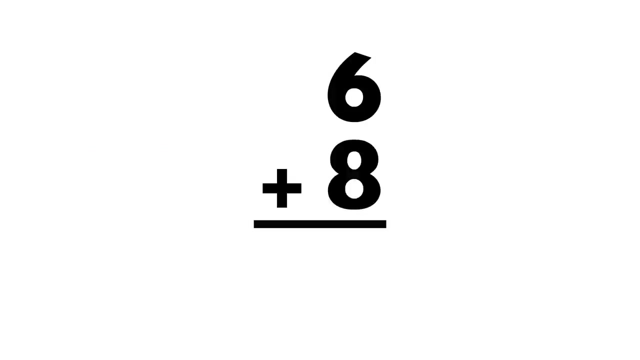 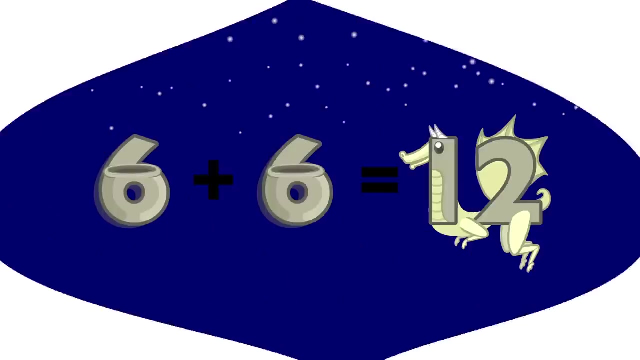 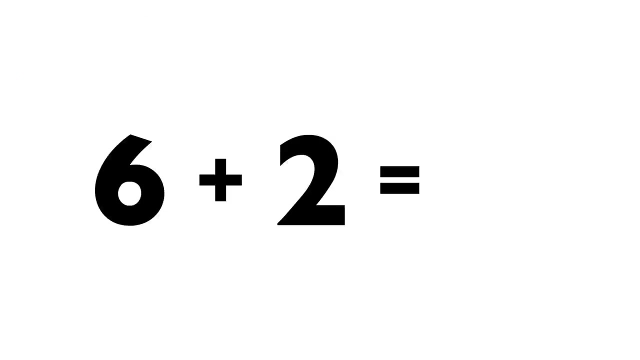 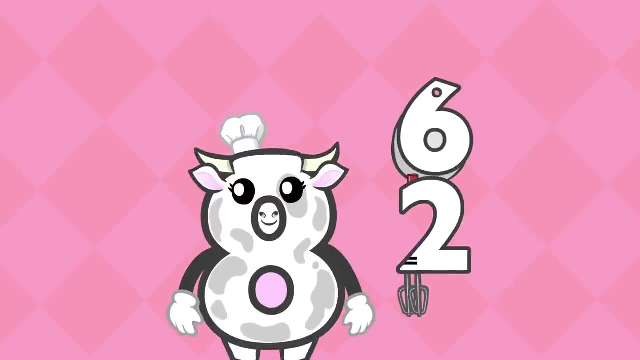 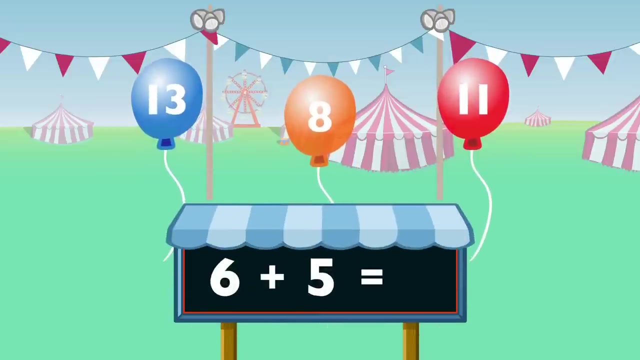 One, Two, Two. Thirteen. Six plus one equals Seven. Six plus eight equals Fourteen. Fourteen Six plus six equals Twelve. Six plus two equals Eight. Six plus five equals Eleven. Six plus seven equals Thirteen. Six plus two equals. 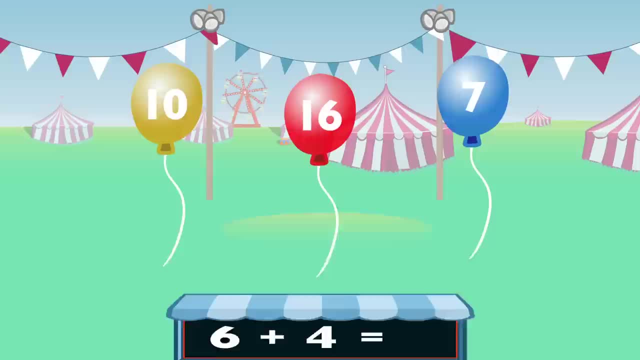 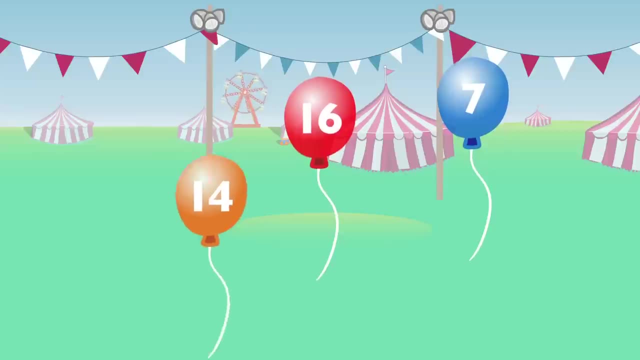 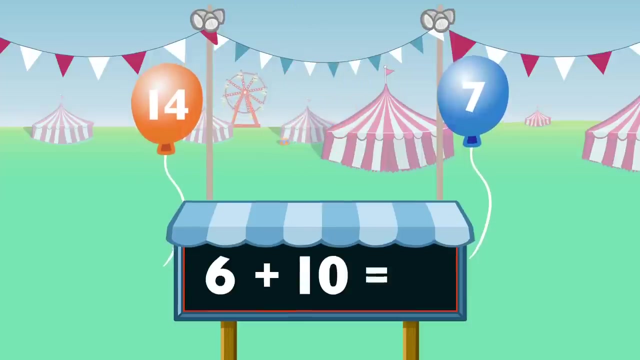 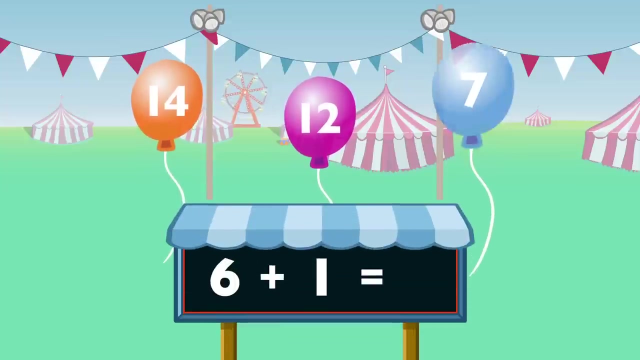 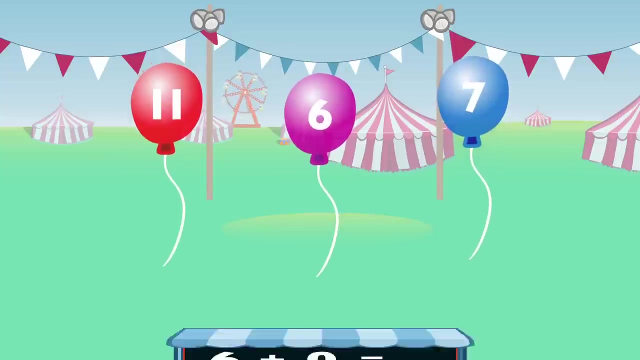 Eight Six plus four equals Ten. Six plus ten equals Sixteen. Six plus one equals Seven. Six plus eight equals Fourteen. Six plus six equals Twelve. Six plus nine equals Fifteen. Six plus three equals Nine. Six plus zero equals. 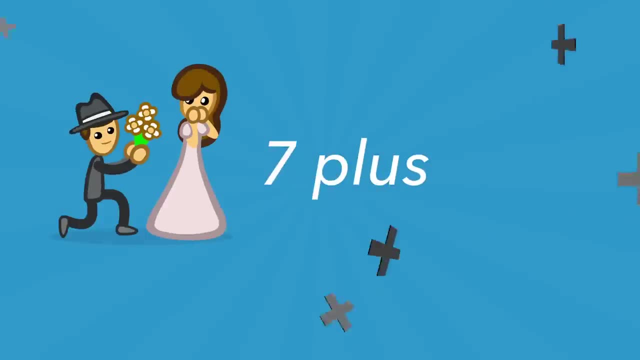 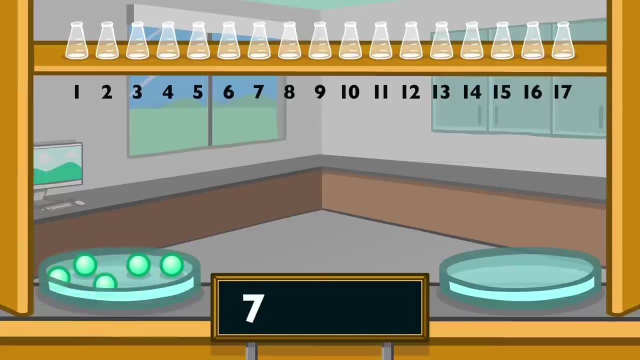 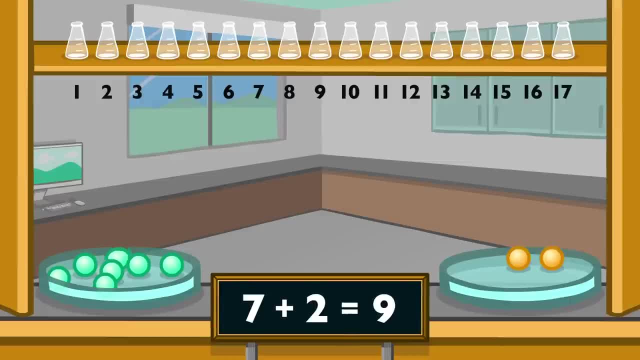 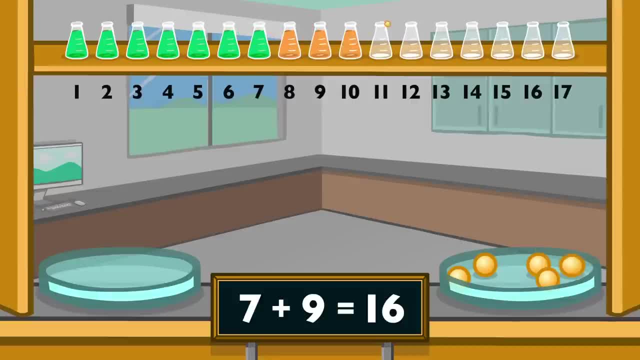 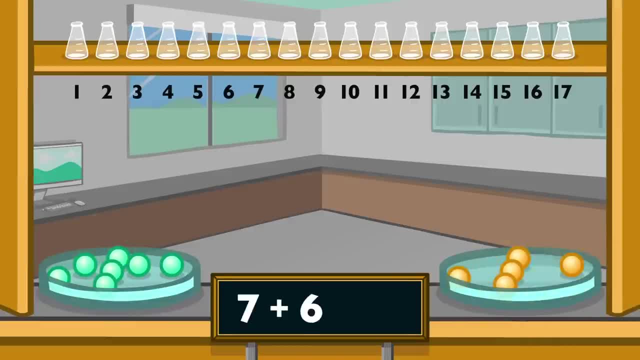 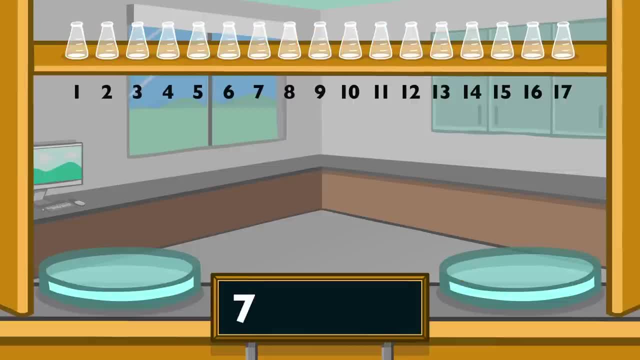 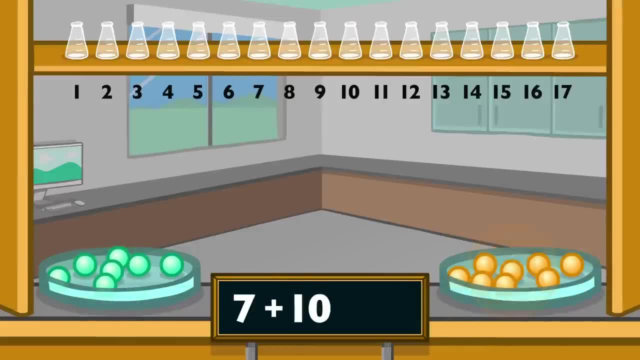 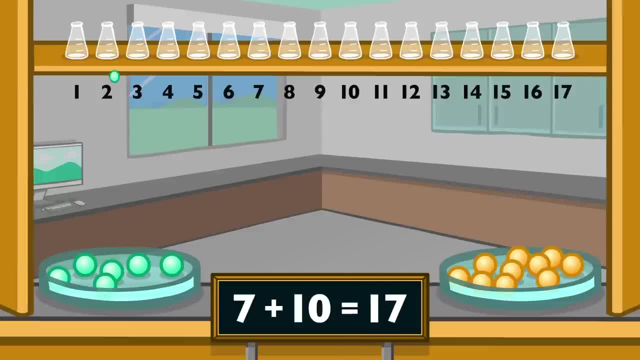 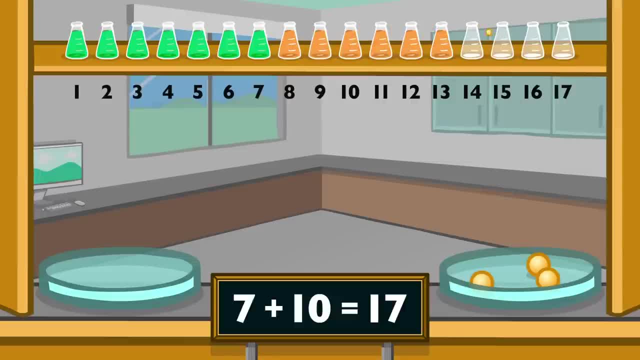 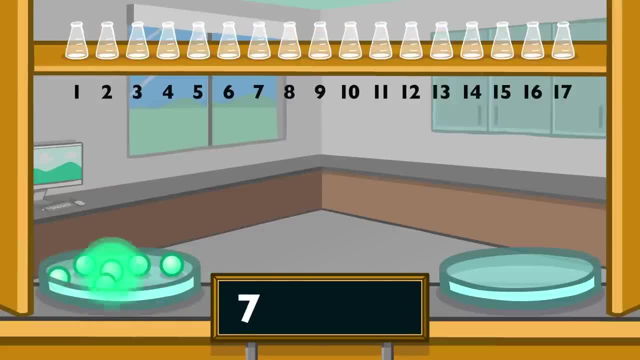 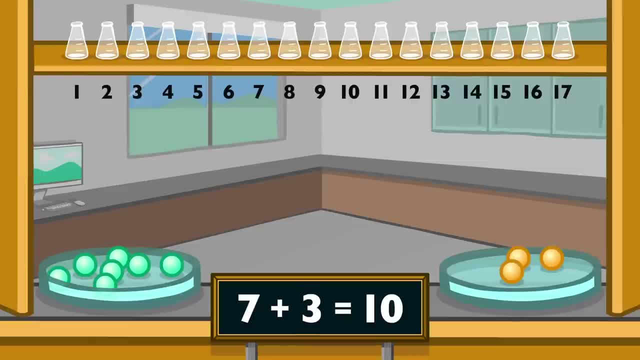 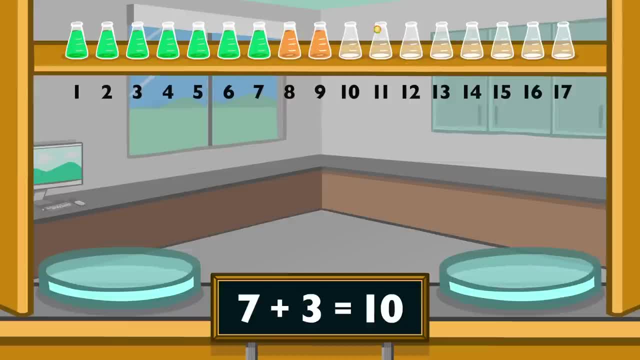 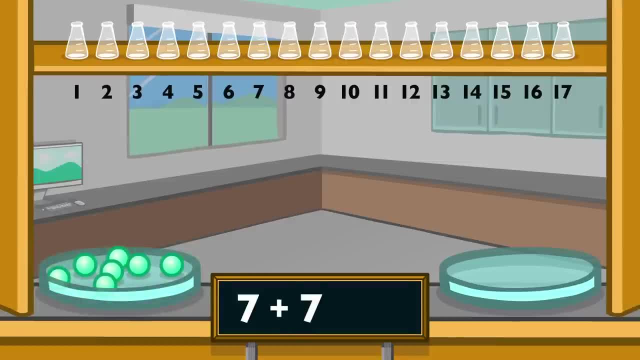 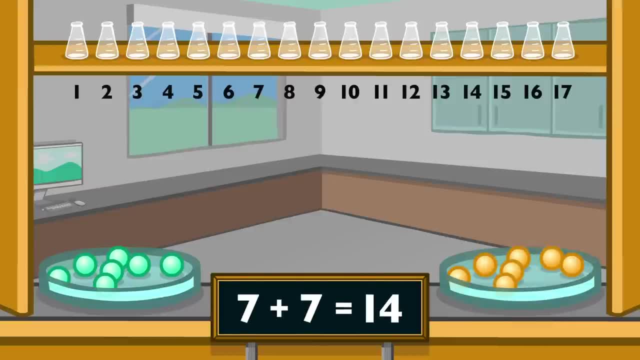 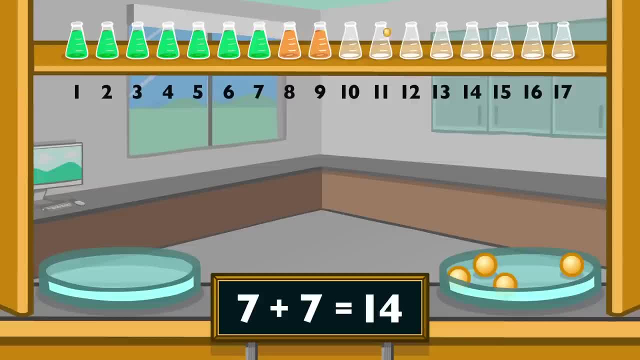 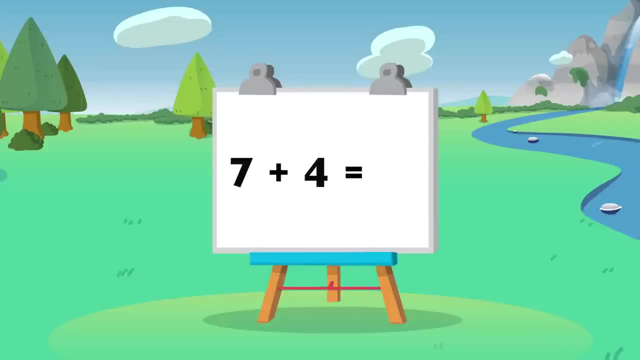 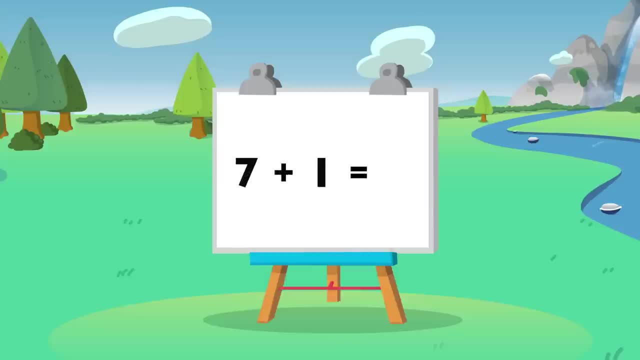 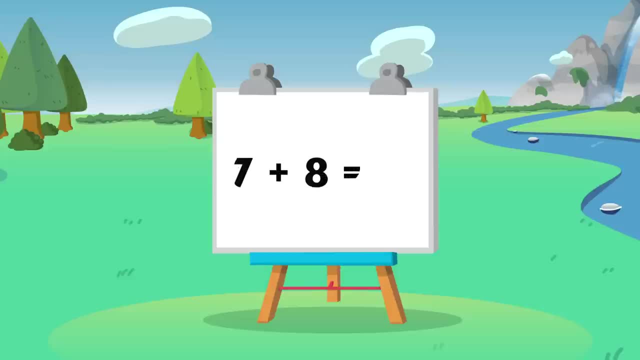 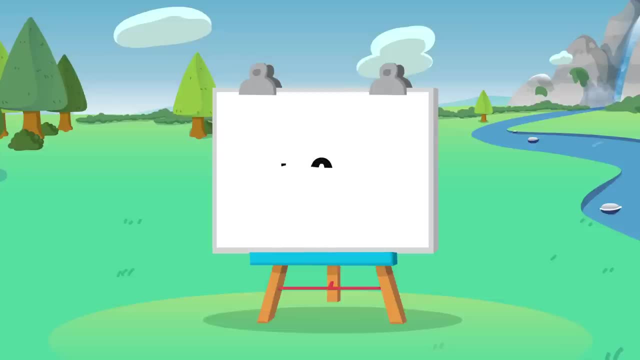 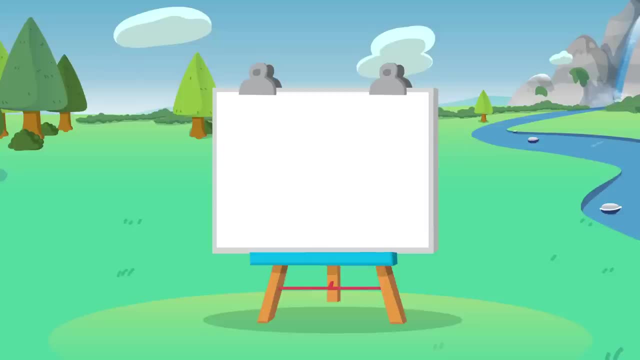 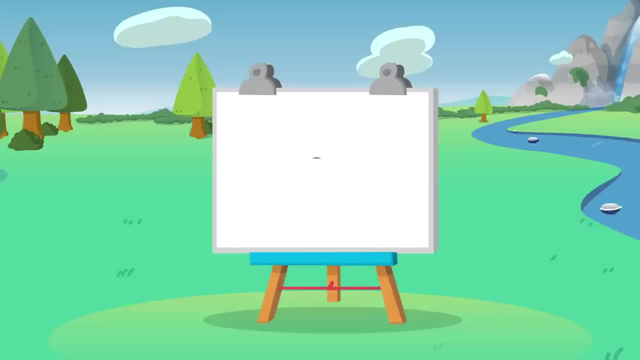 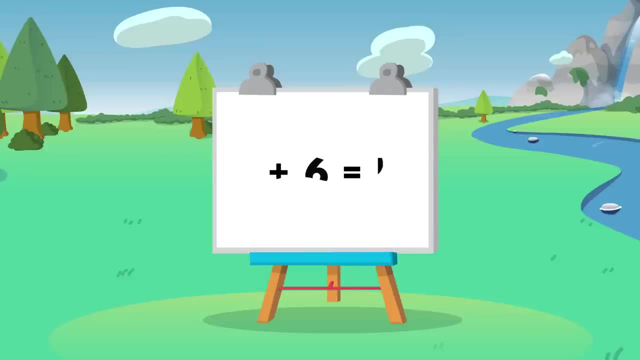 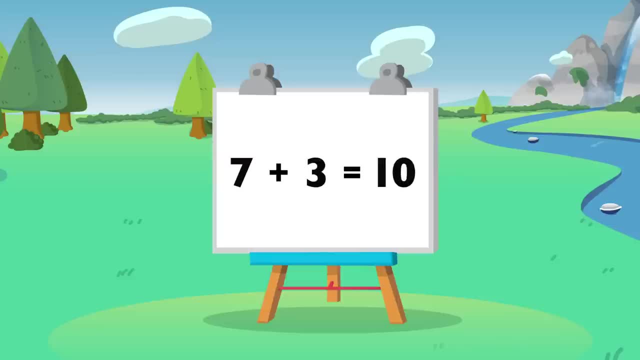 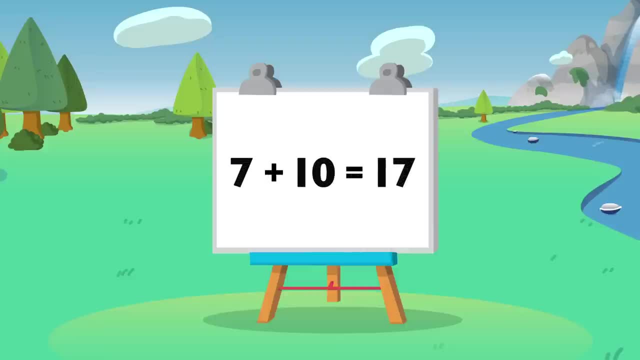 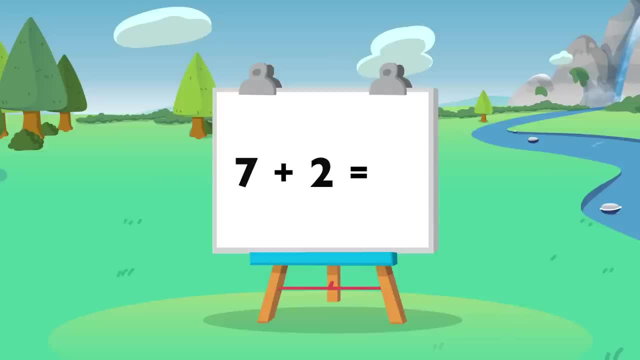 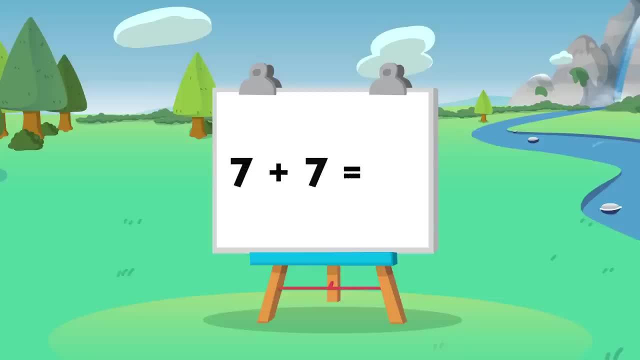 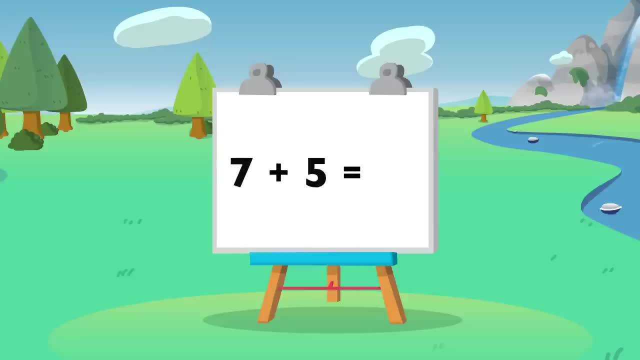 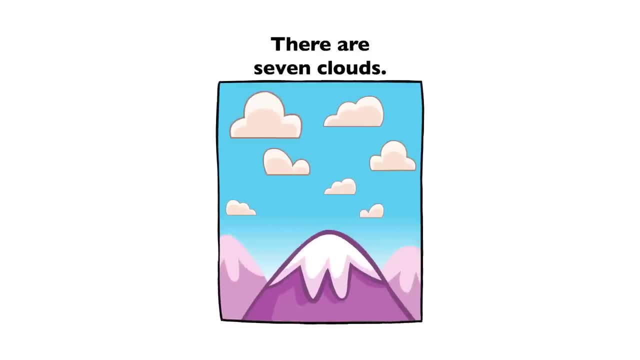 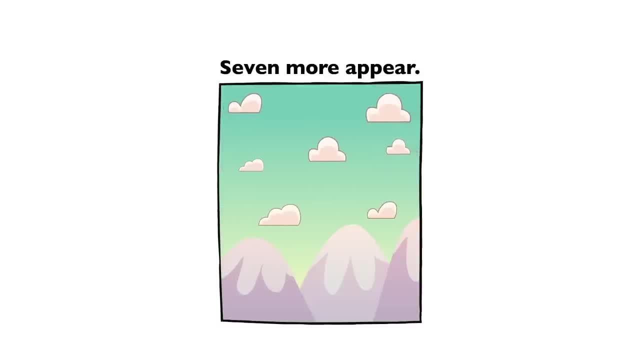 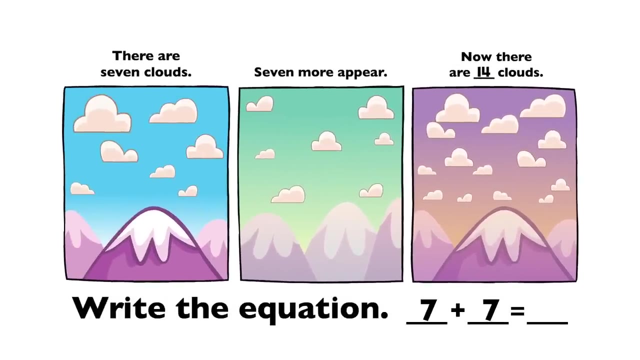 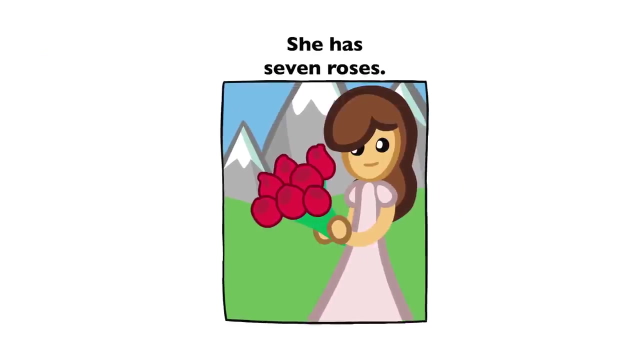 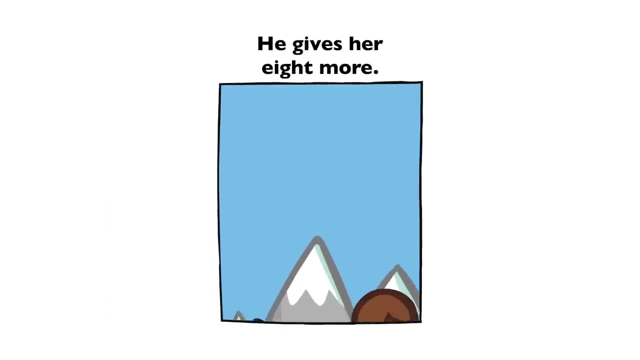 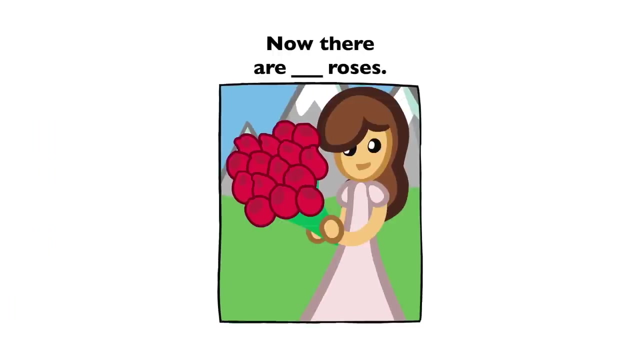 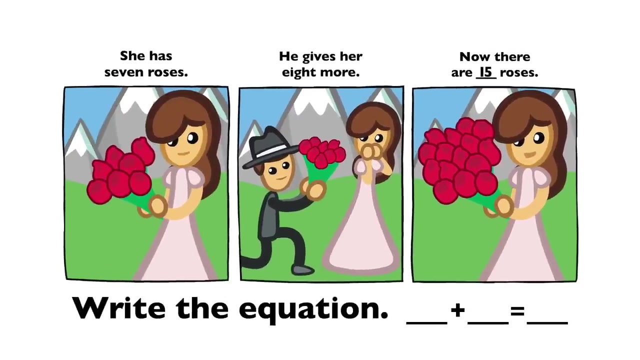 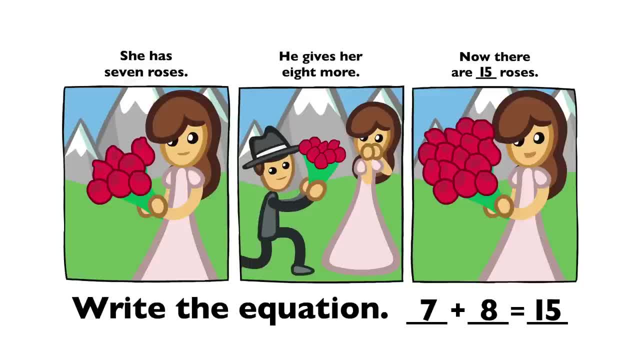 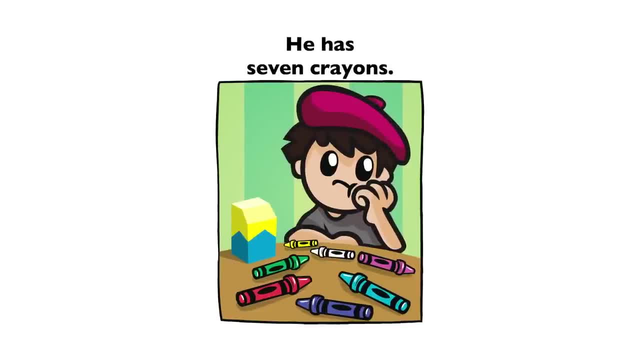 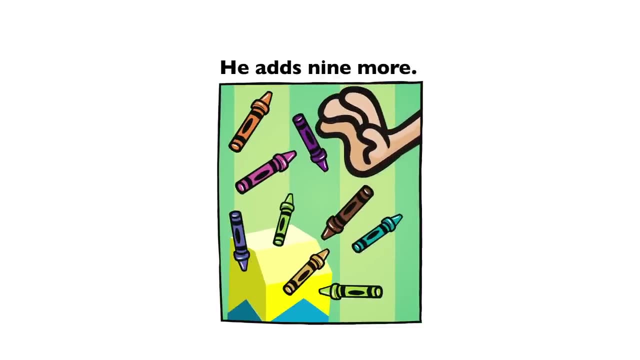 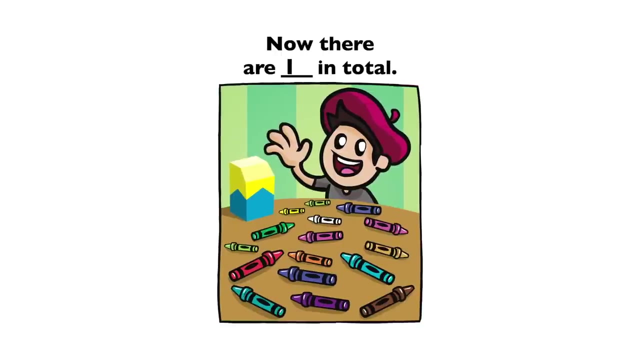 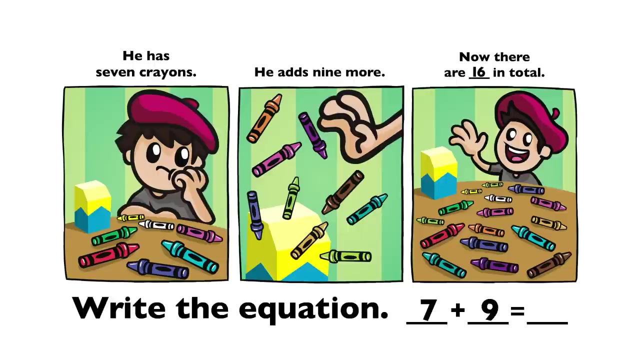 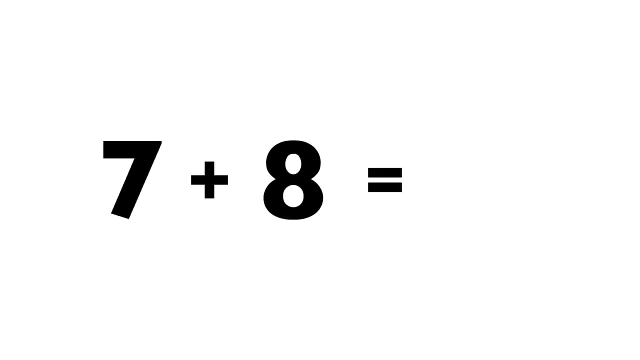 Seven plus eight equals fifteen. He has seven crayons. He adds nine more. Now there are sixteen in total. Seven plus nine equals sixteen. Seven plus eight equals fifteen. Fifteen. Seven plus zero equals seven. Seven plus ten equals seventeen. 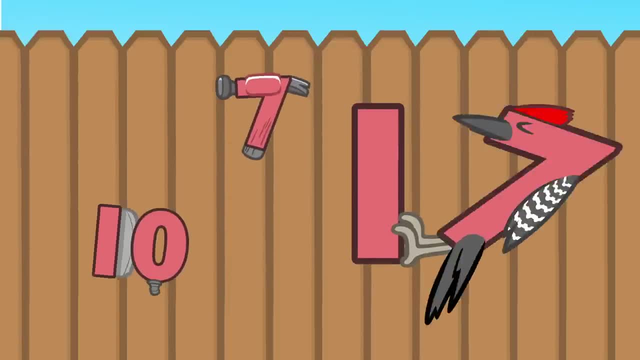 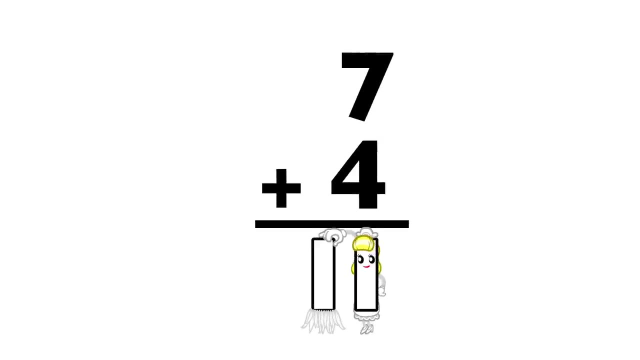 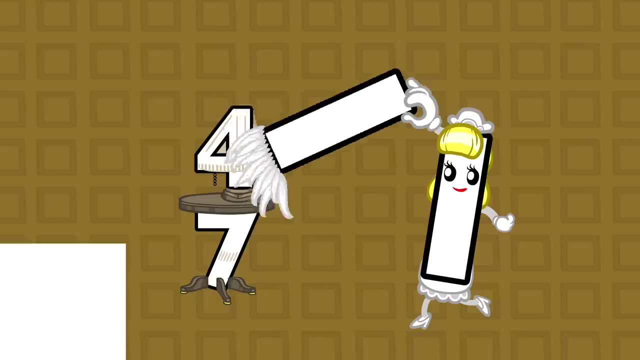 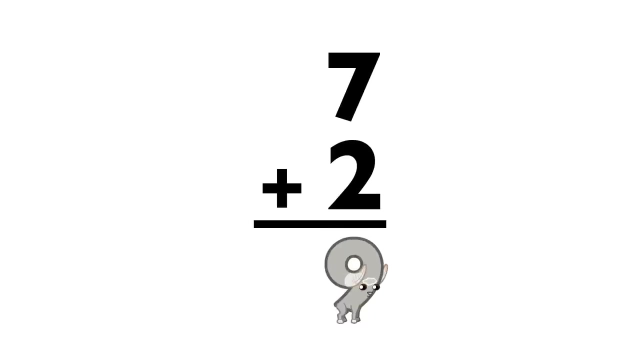 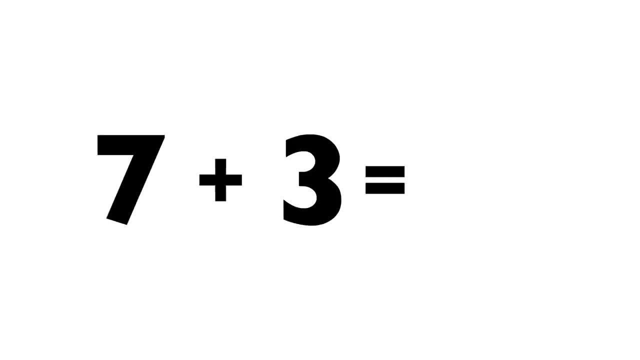 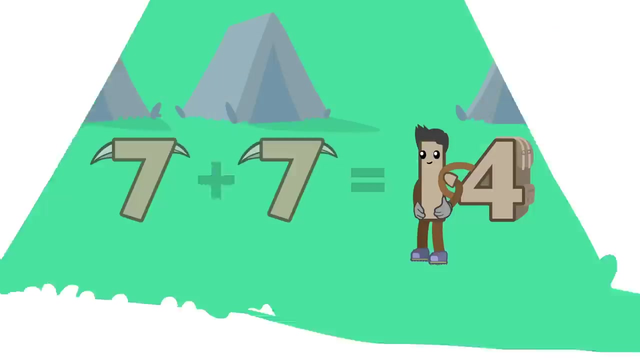 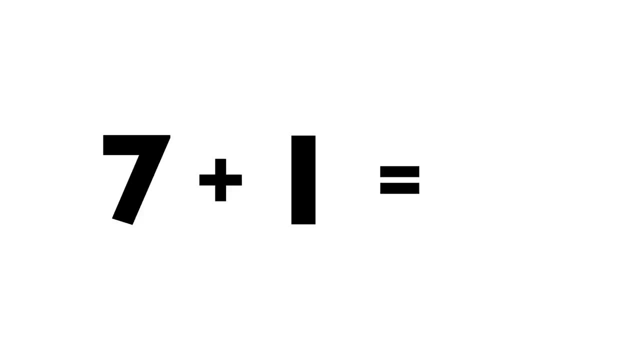 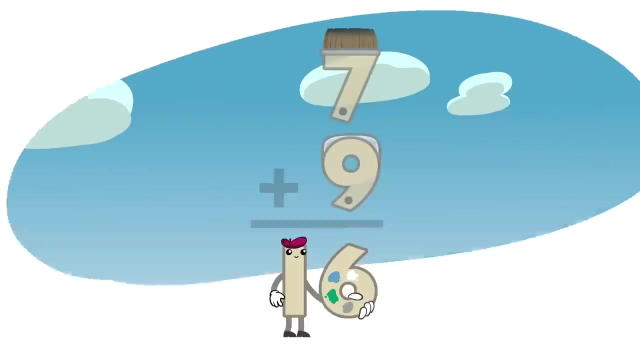 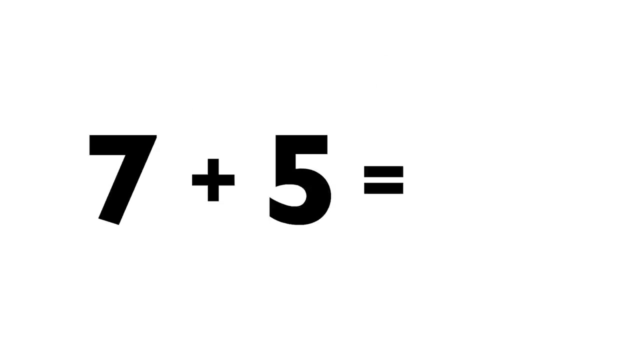 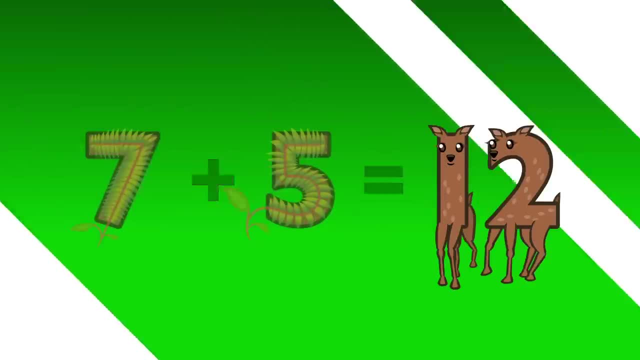 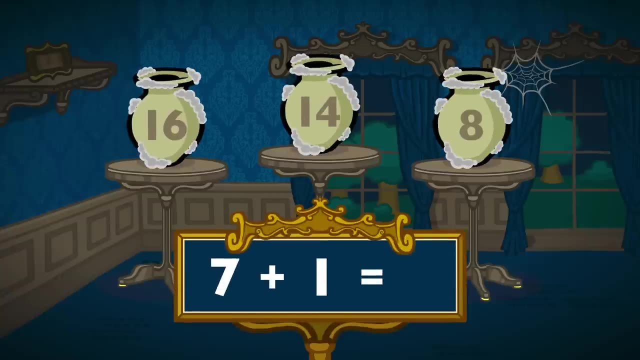 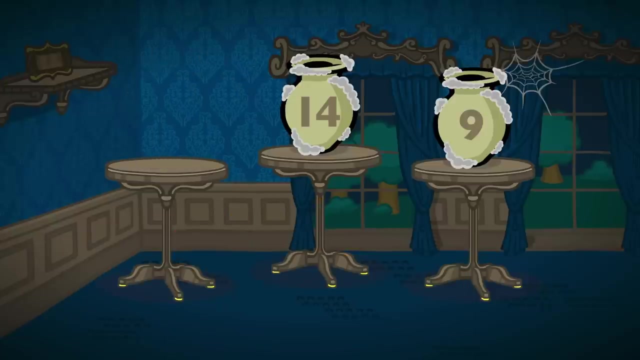 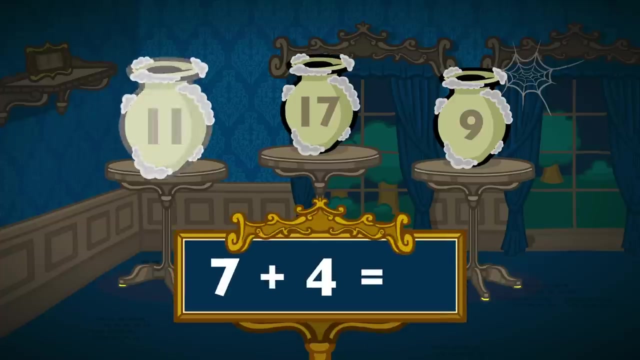 Twelve Seven plus one equals Eight. Seven plus nine equals Sixteen. Seven plus seven equals Fourteen. Seven plus four equals Eleven. Seven plus ten equals Seventeen. Seven plus two equals Nine. Seven plus five equals. 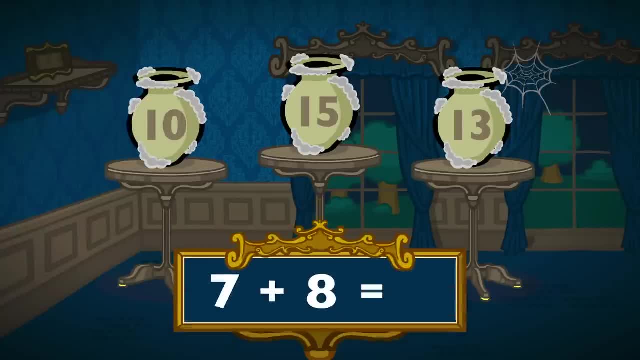 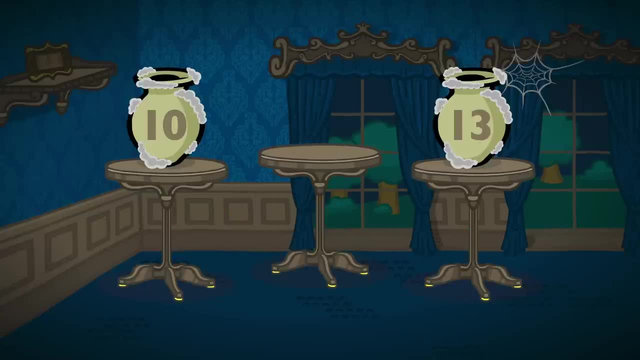 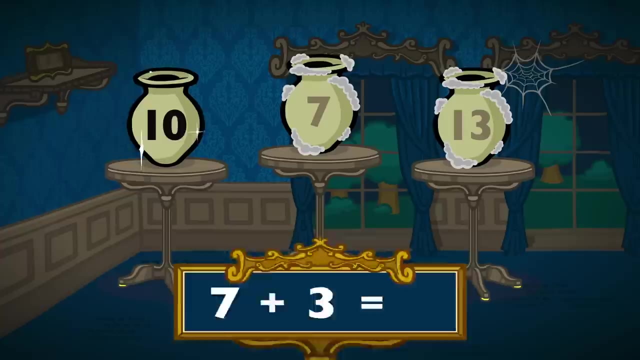 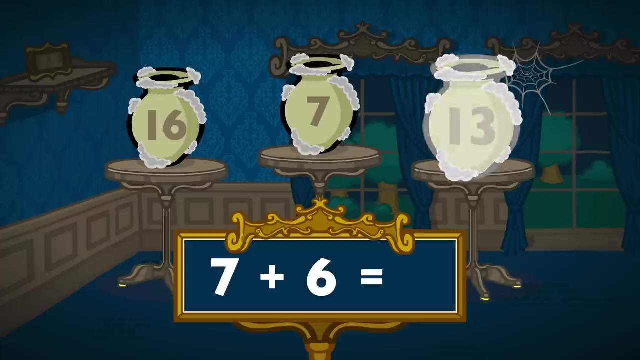 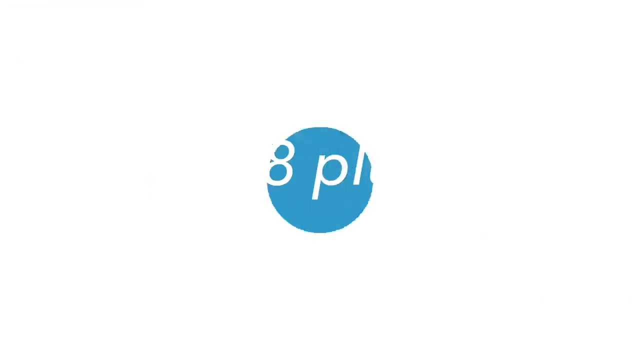 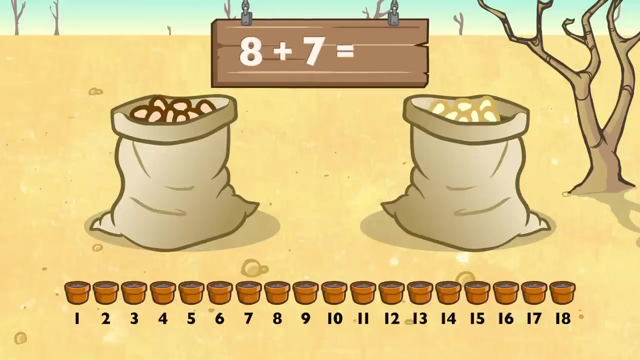 Twelve Seven plus eight equals Fifteen. Seven plus three equals Ten. Seven plus six equals Thirteen. Seven plus zero equals Seven. Eight plus seven equals Fifteen. Eight plus seven equals. Fifteen Eight plus seven equals. 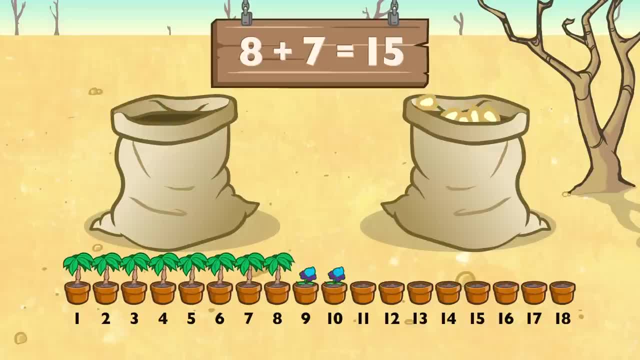 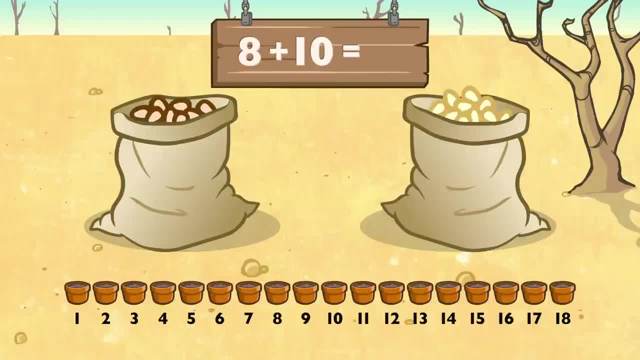 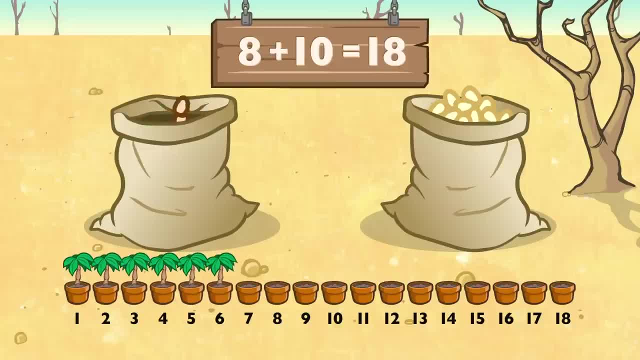 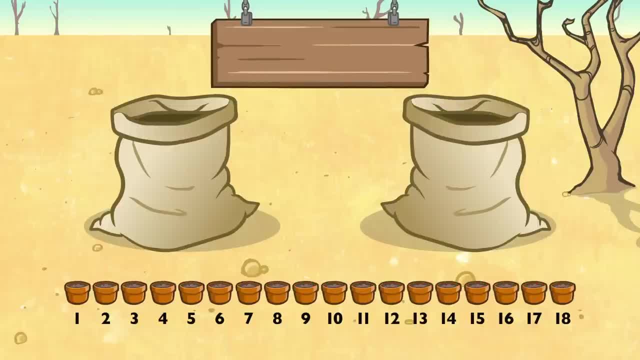 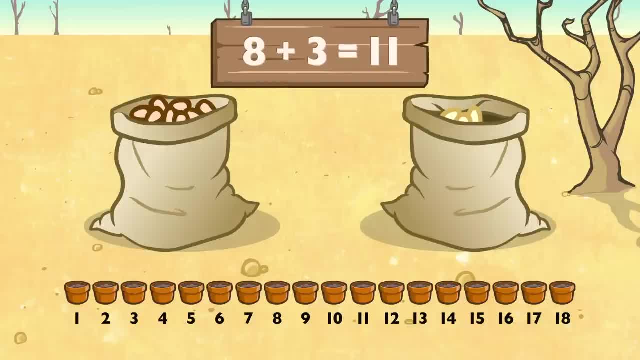 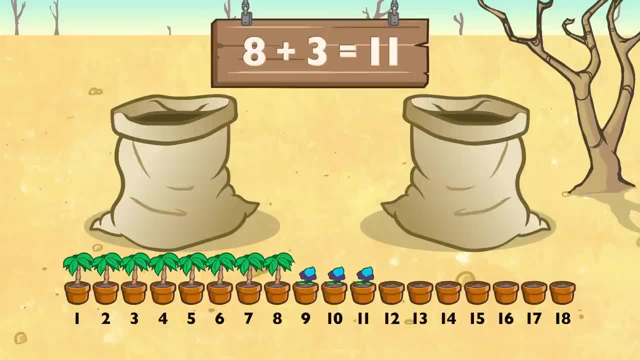 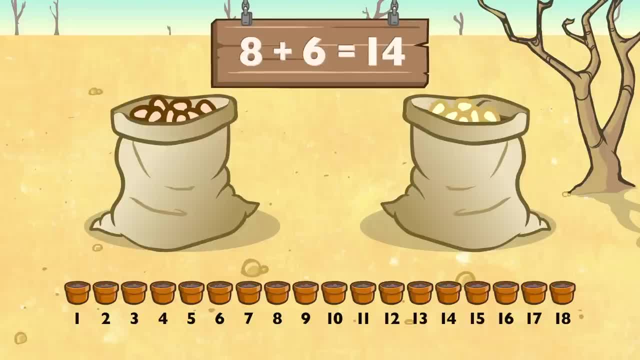 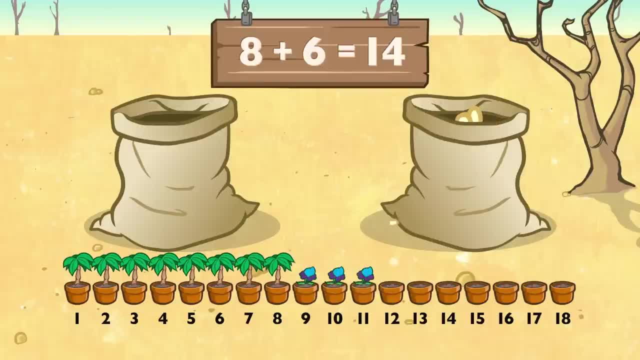 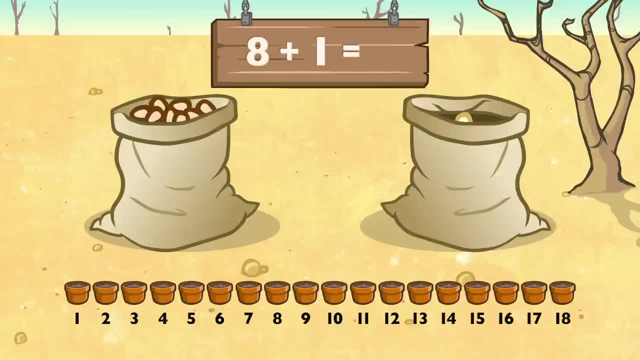 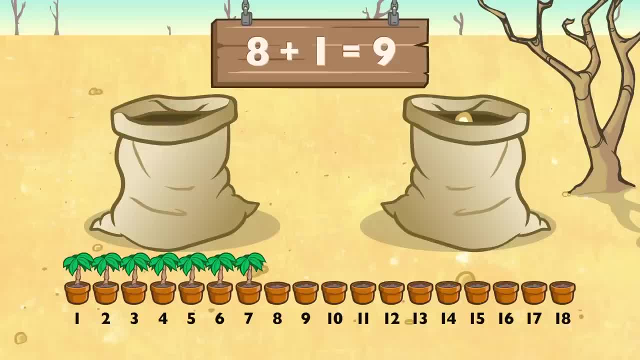 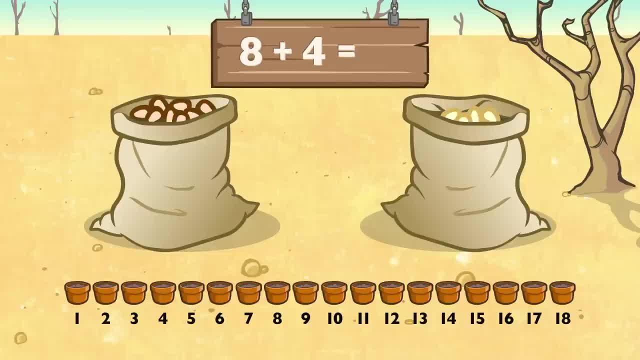 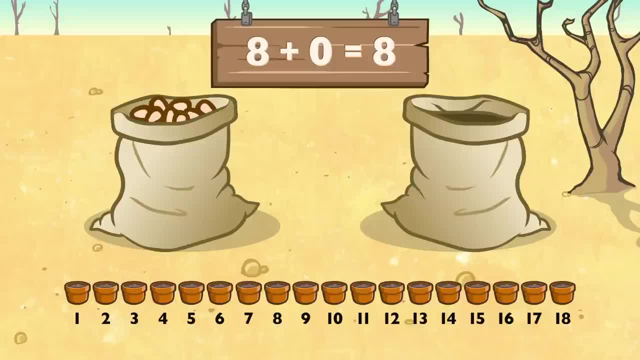 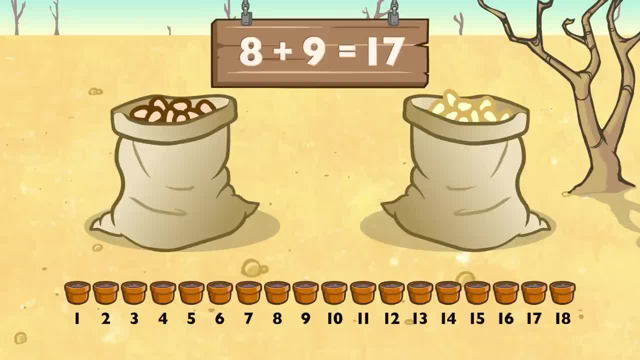 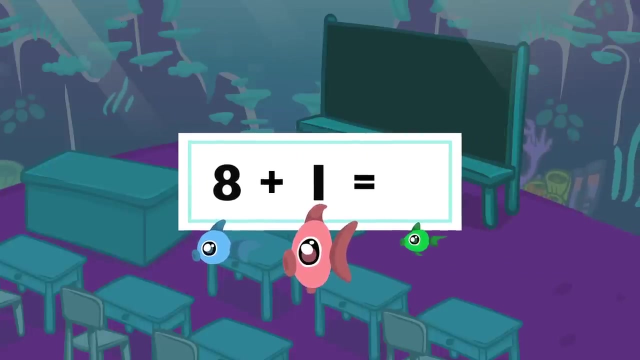 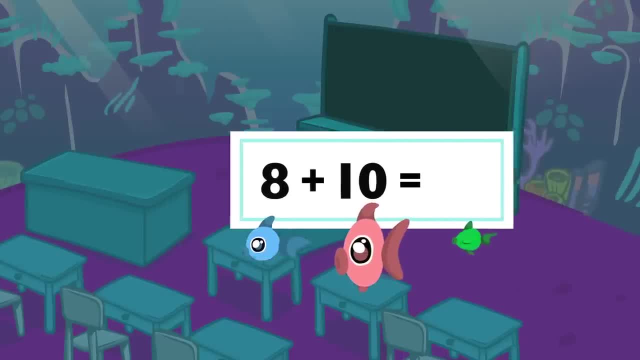 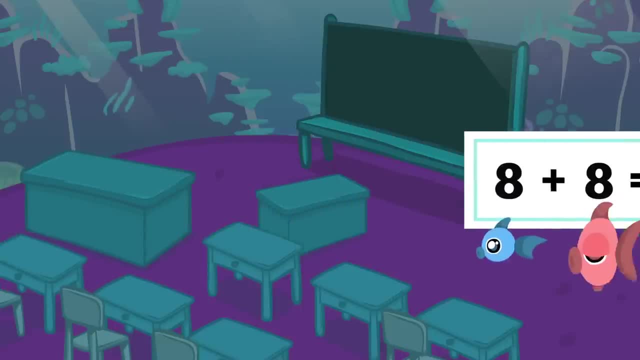 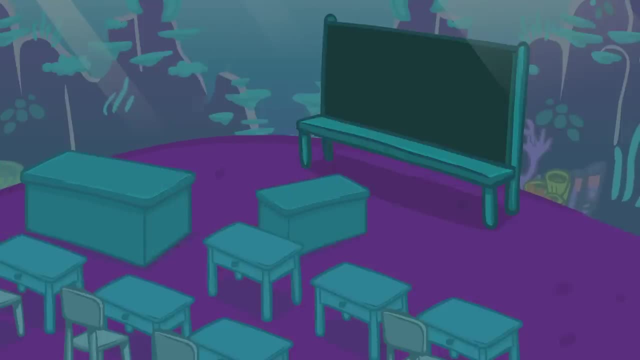 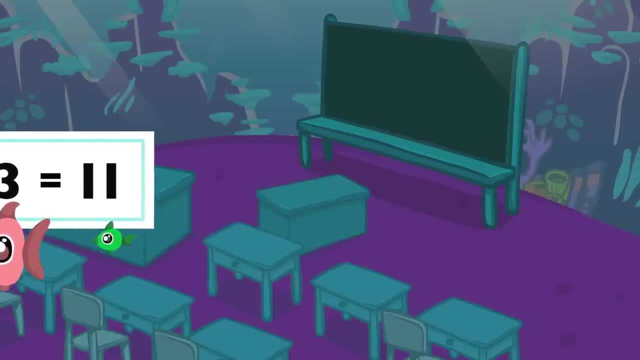 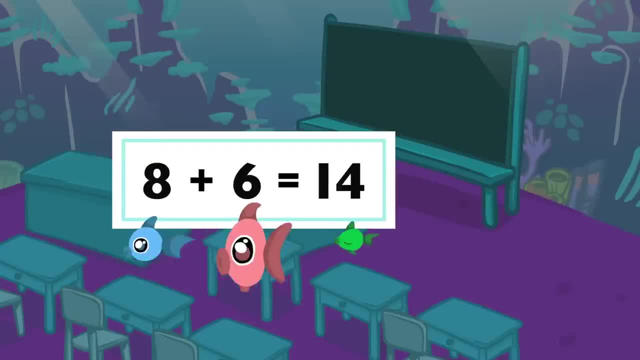 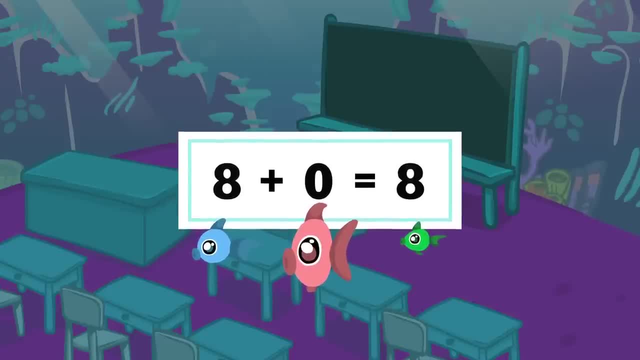 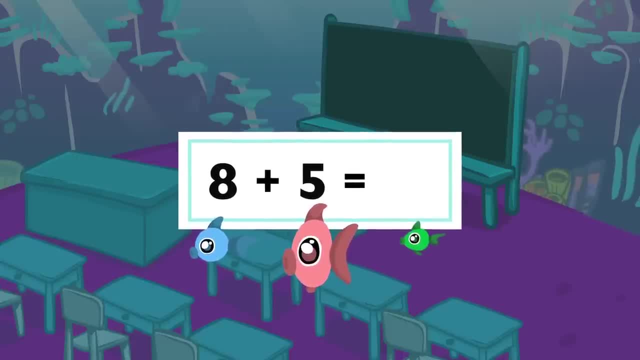 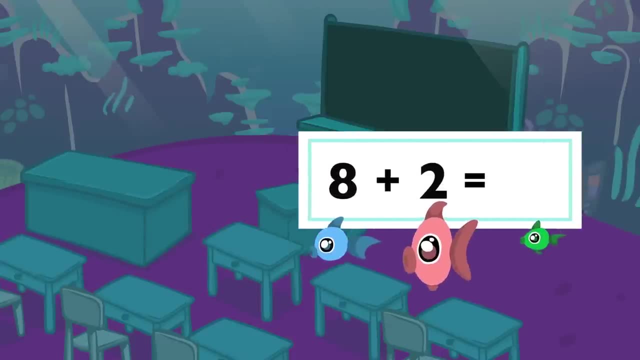 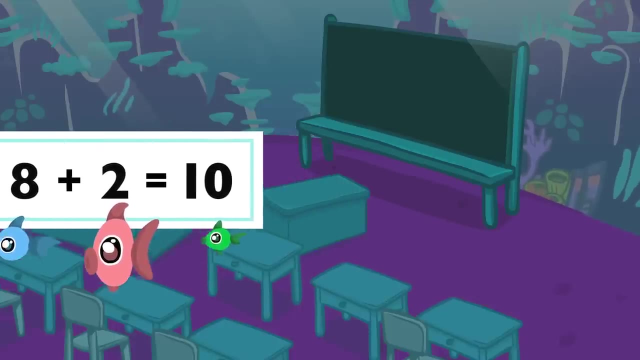 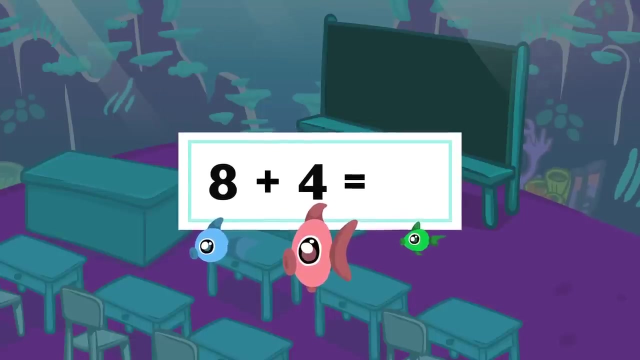 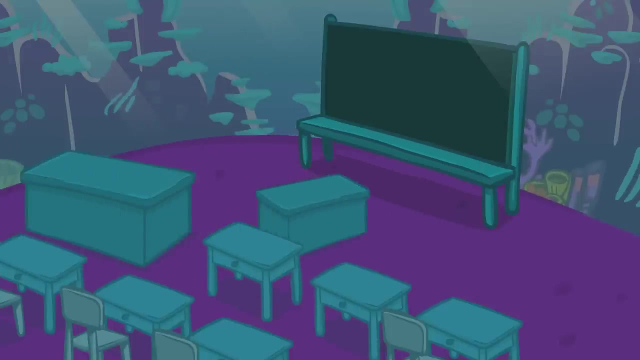 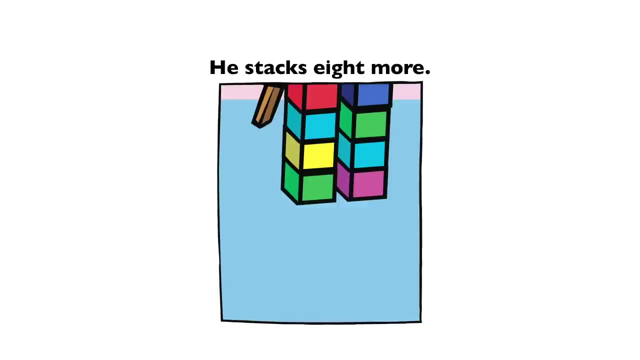 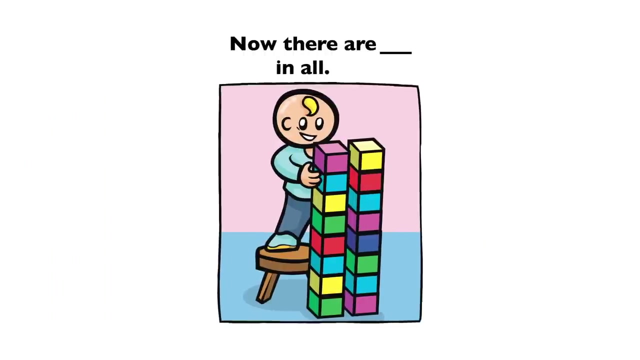 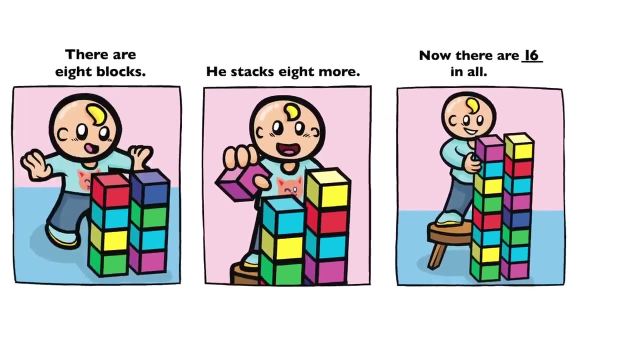 8 plus 5 equals 13.. 8 plus 2 equals 10.. 8 plus 4 equals 12.. 8 plus 7 equals 15.. There are 8 blocks. He stacks 8 more. Now there are 16 in all. 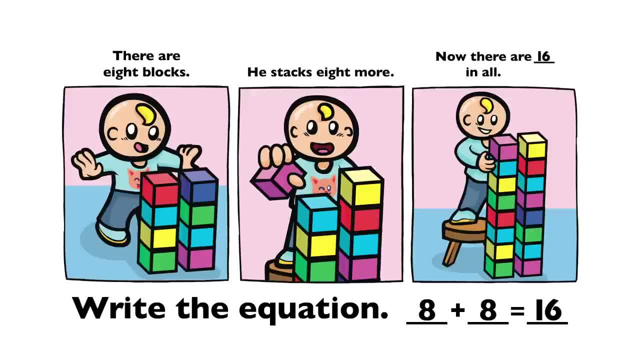 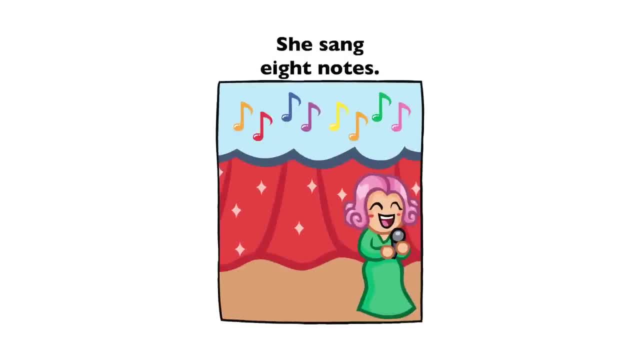 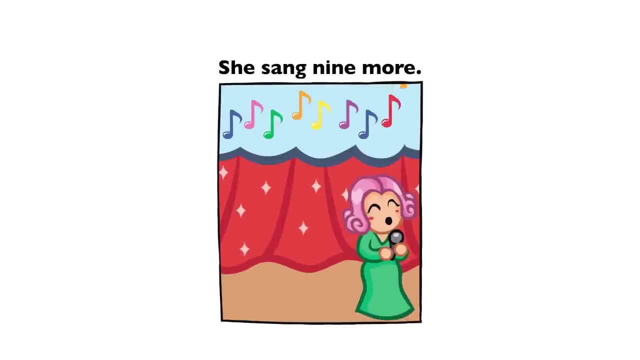 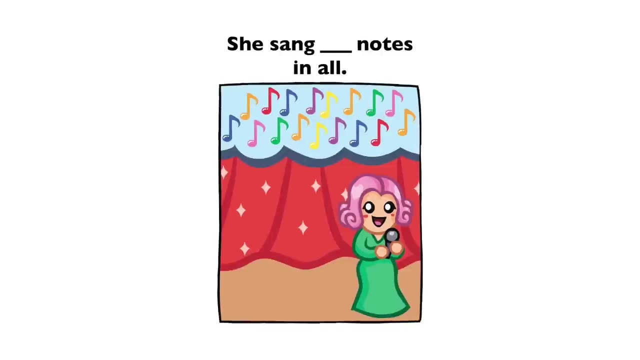 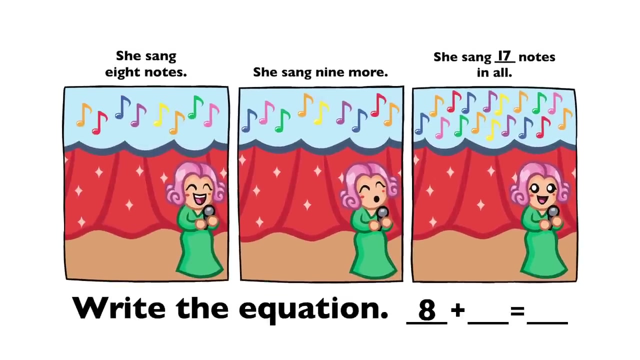 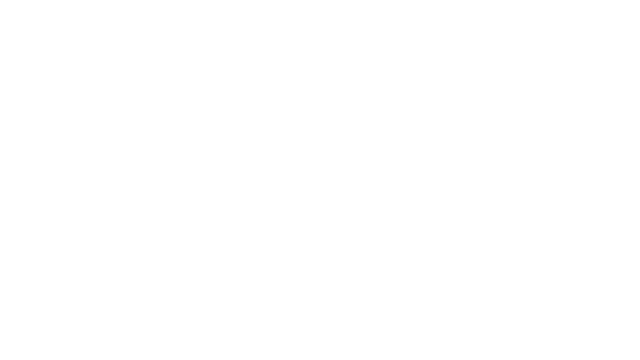 8 plus 8 equals 16.. She sang 8 notes. She sang 9 more. She sang 17 notes in all. 8 plus 9 equals 17.. There are 8 fish. 10 more fish, join them. 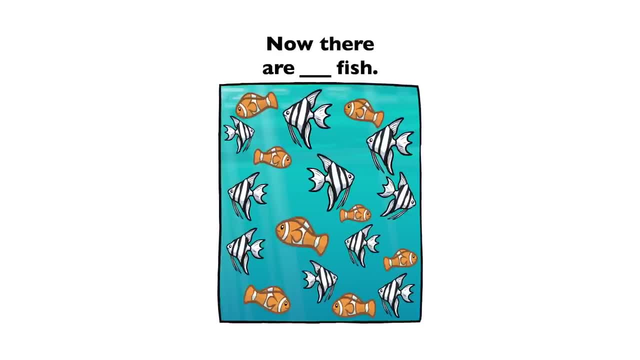 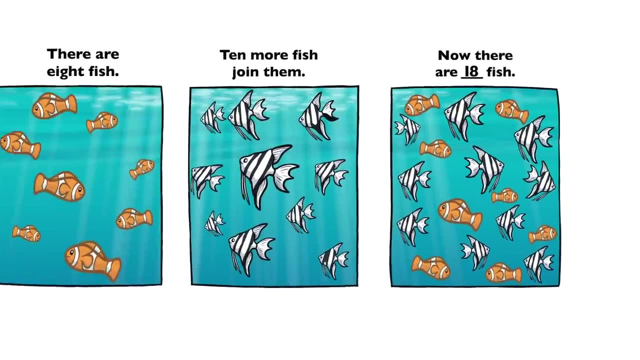 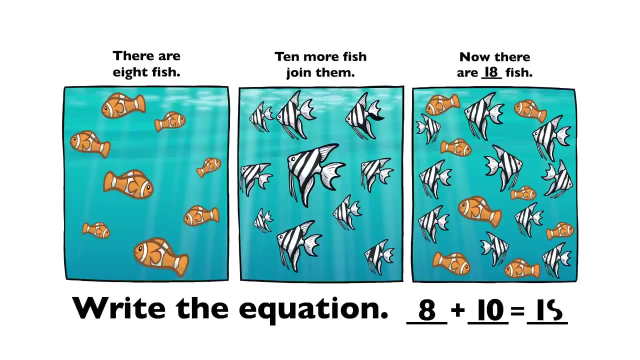 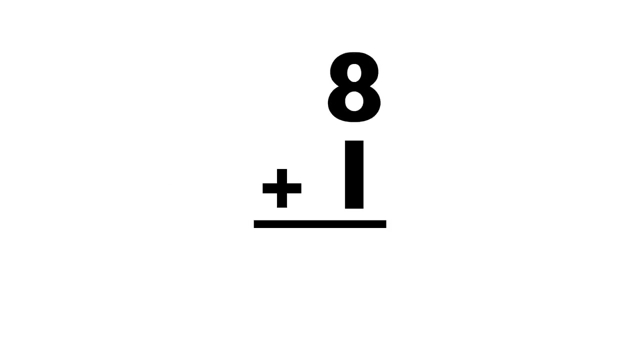 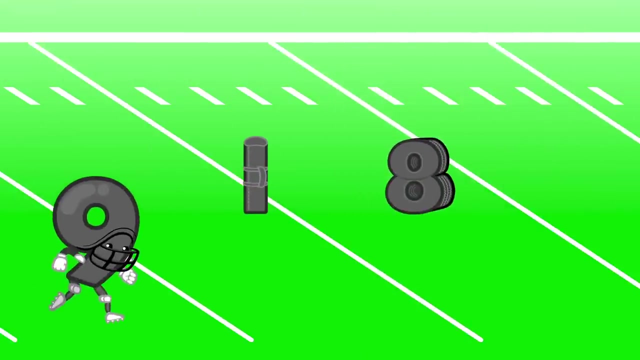 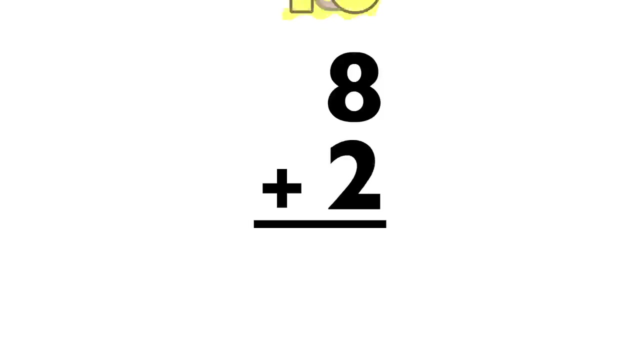 Now there are 18 fish. 8 plus 10 equals 18.. 8 plus 1 equals 9.. 8 plus 2 equals 8.. 8 plus 2 equals 8.. 8 plus 2 equals 8.. 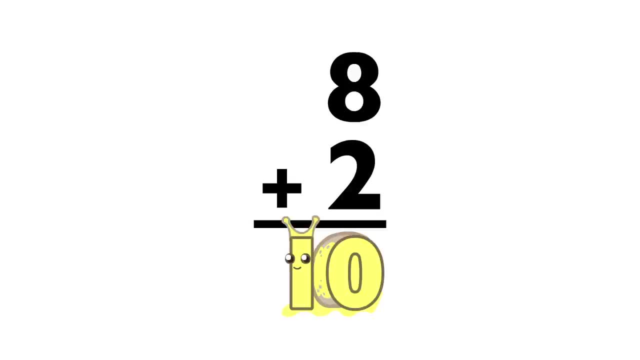 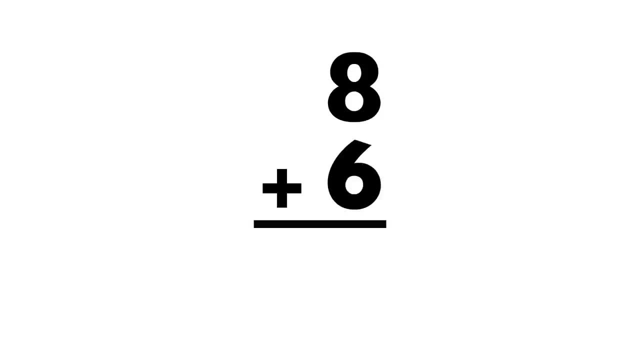 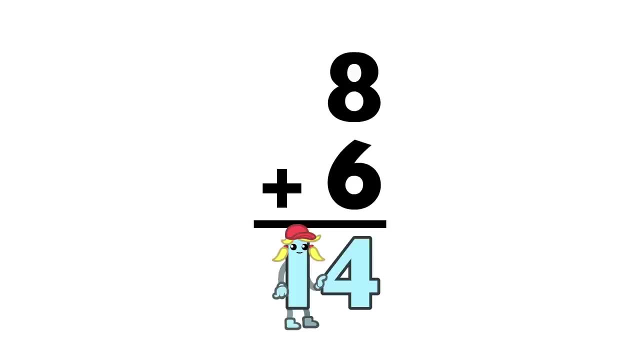 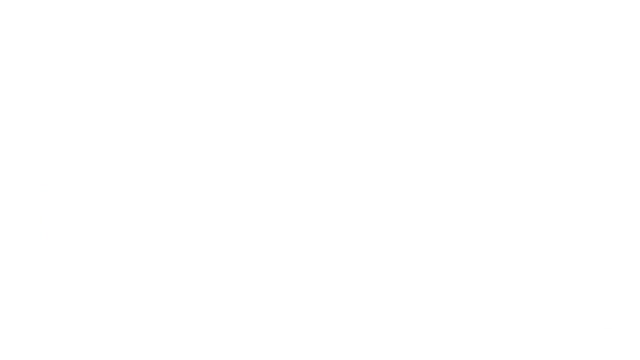 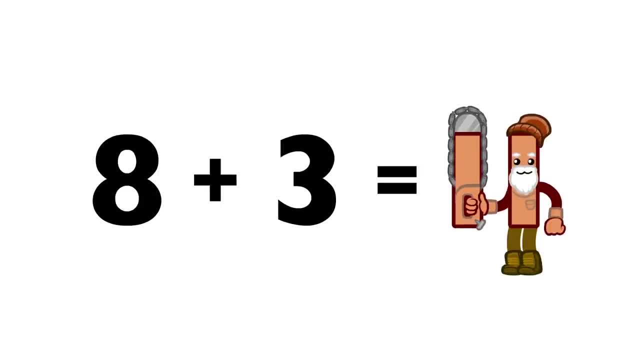 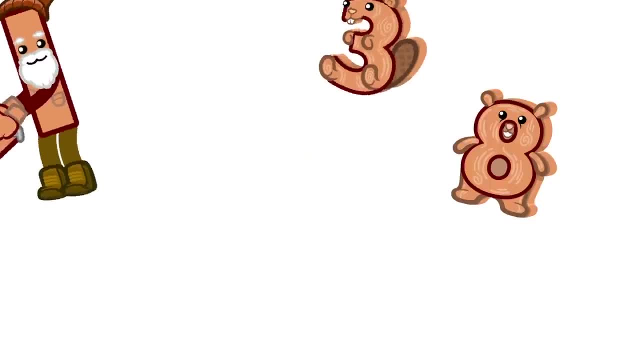 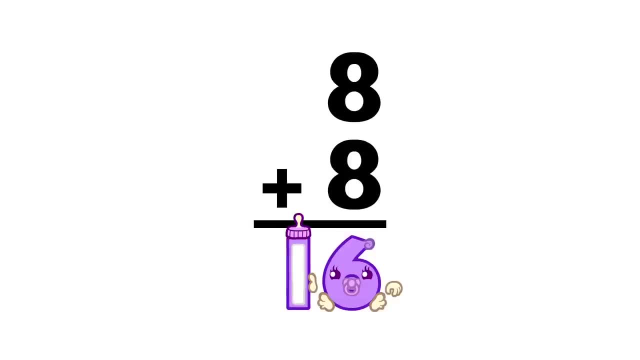 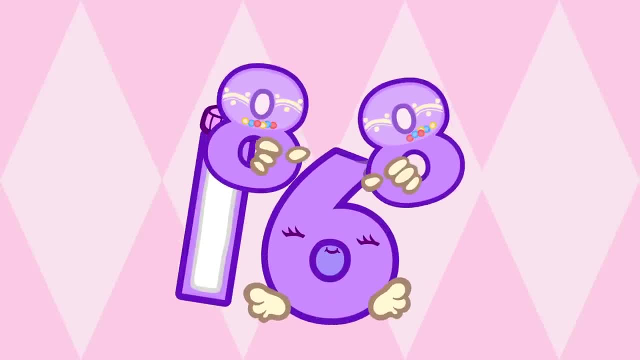 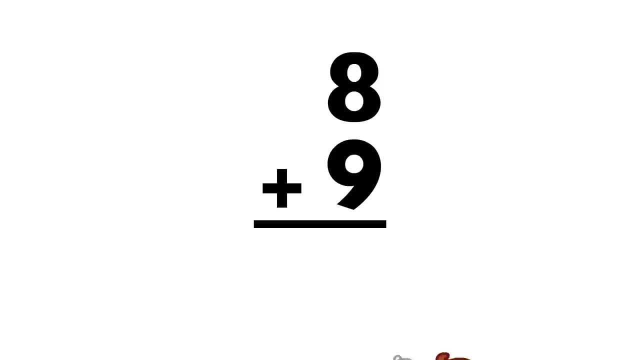 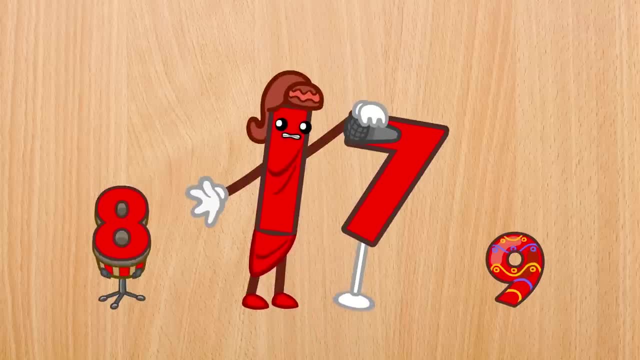 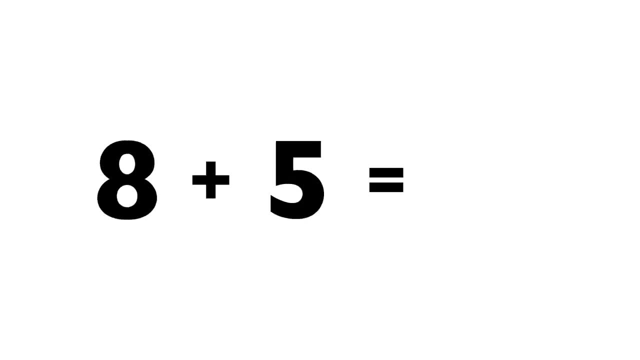 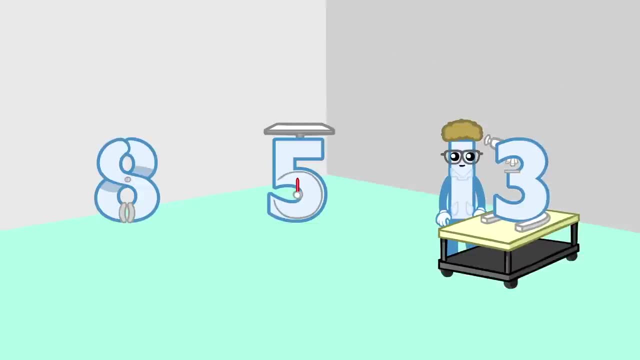 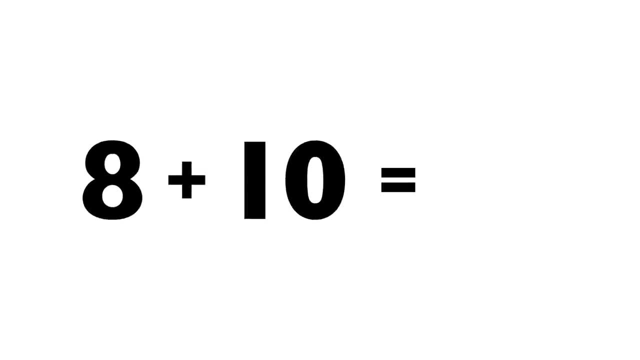 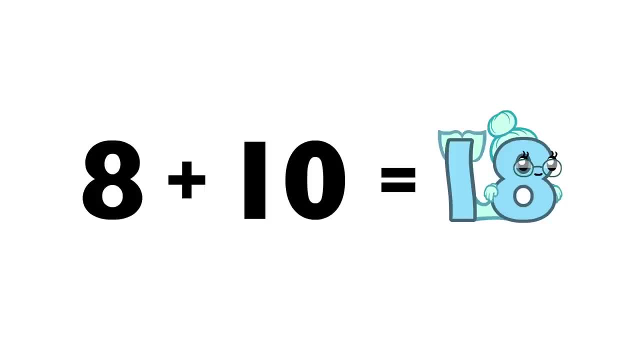 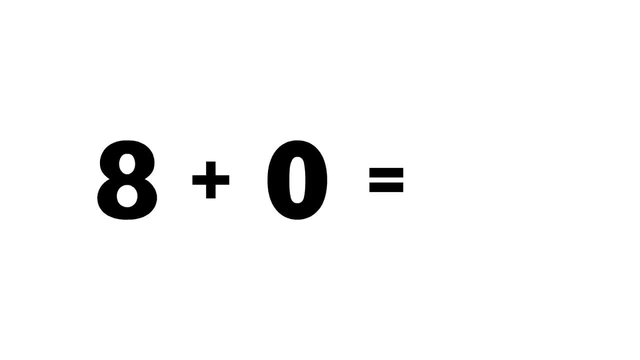 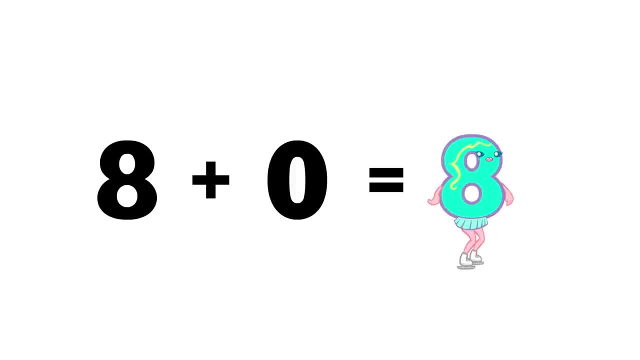 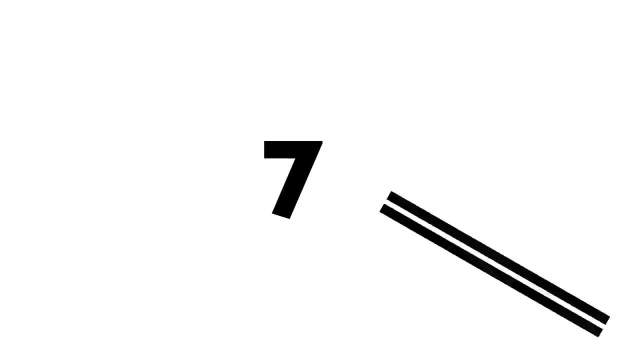 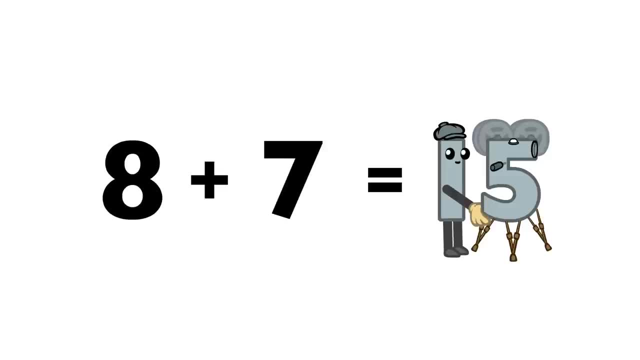 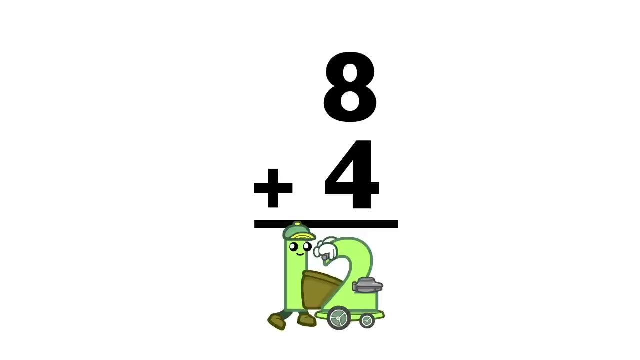 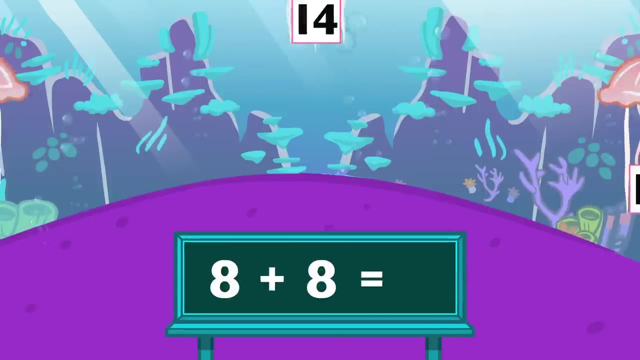 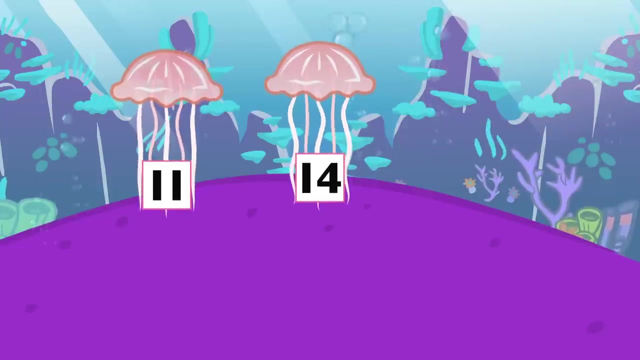 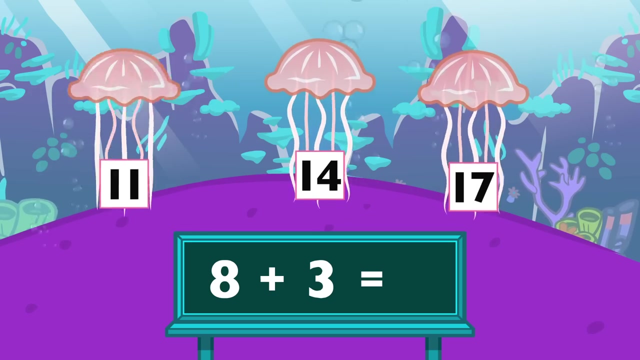 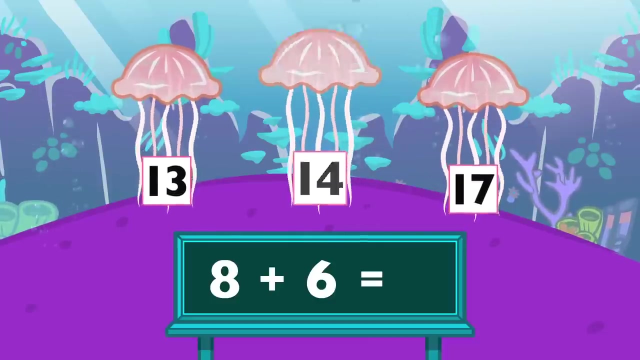 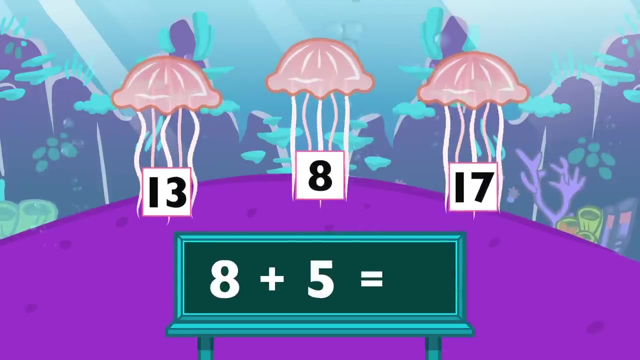 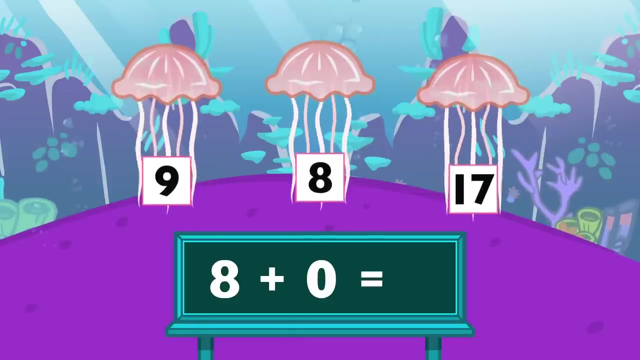 equals 15.. Eight plus four equals 12.. Eight plus eight equals six. Eight plus three equals 16.. Eight plus three equals 11.. Eight plus six equals 14.. Eight plus five equals 13.. Eight Eight plus nine equals 17.. 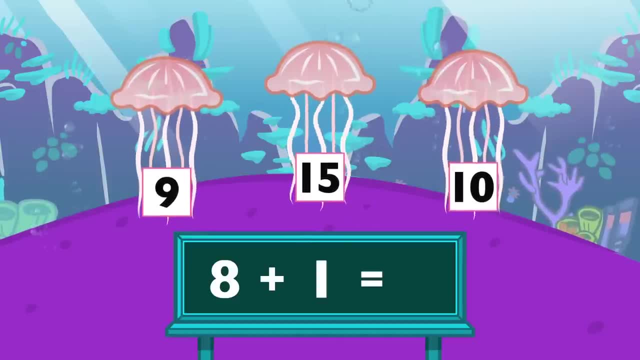 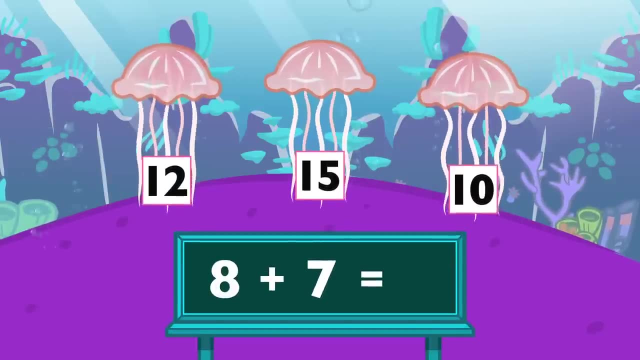 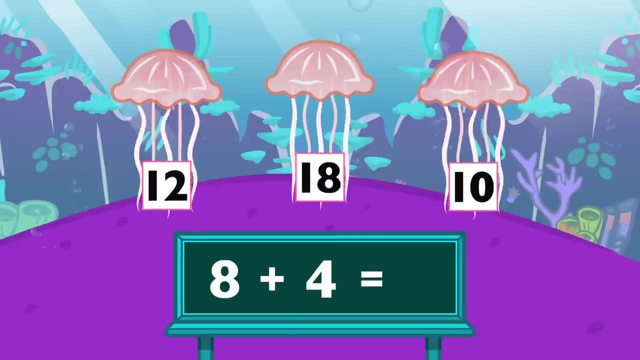 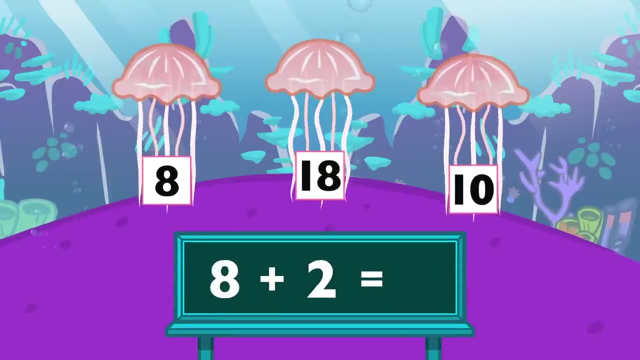 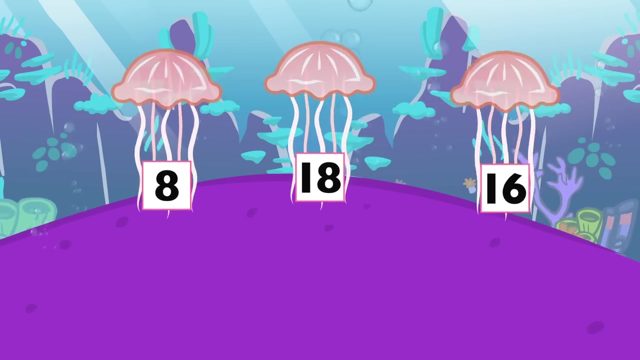 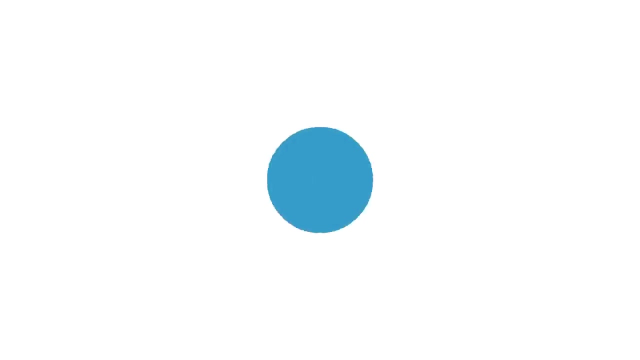 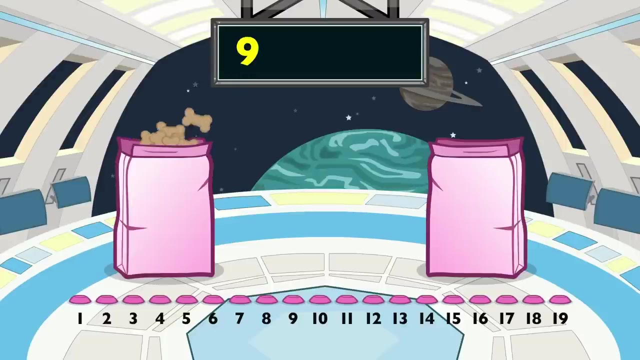 Eight plus one equals nine. Eight plus seven equals 15.. Eight plus four equals 12.. Eight plus two equals 10.. Eight plus ten: equals 18.. Eight plus ten: equals 18.. Eight plus ten equals 19.. Nine plus two equals 11.. 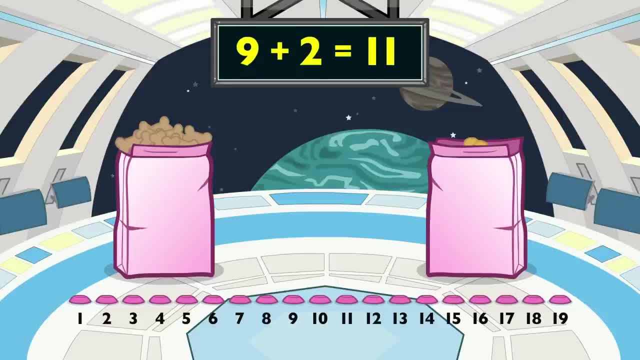 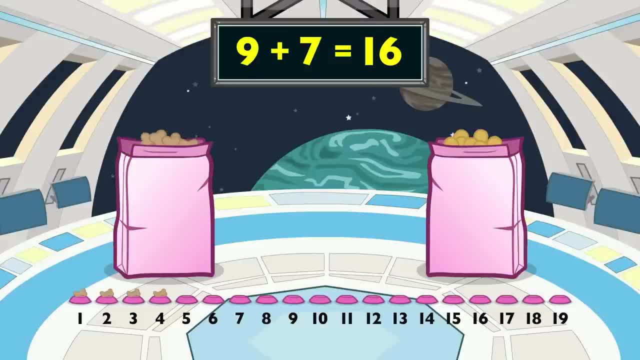 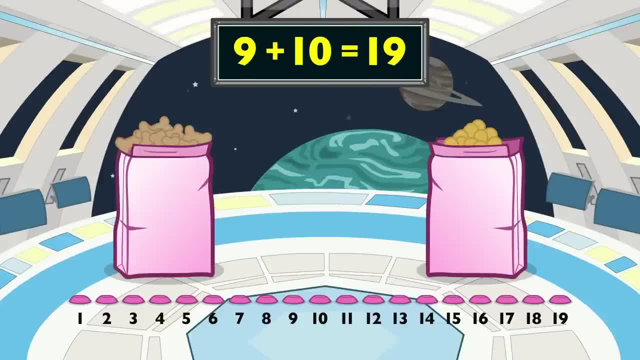 9 plus 10 equals 19.. 9 plus 5 equals 14.. 9 plus 5 equals 14.. 9 plus 5 equals 14.. 9 plus 8 equals 17.. 9 plus 8 equals 17.. 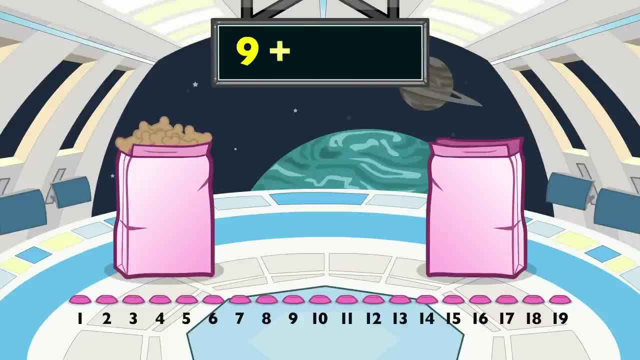 9 plus 1 equals 28.. 10.. 9 plus 1 equals 10.. 9 plus 9 equals 18.. 9 plus 9 equals 18.. 9 plus 0 equals 9.. 9 plus 0 equals 9.. 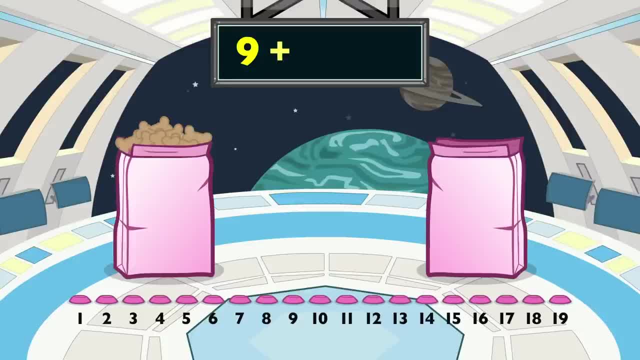 9. 9 plus 4 equals 13.. 9 plus 4 equals 13.. 9 plus 6 equals 15.. 9 plus 6 equals 15.. 9 plus 2 equals 11. 11.. 9 plus 7 equals 16.. 9 plus 4 equals 13.. 9 plus 0 equals 9.. 9 plus 9 equals 9.. 9 plus 9 equals 9. 9.. 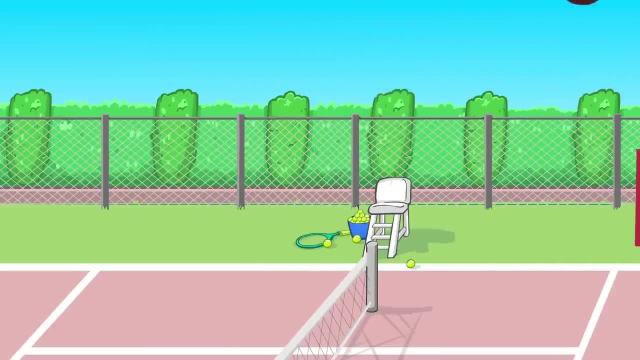 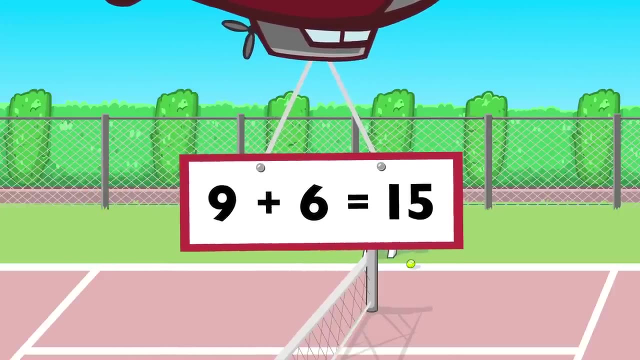 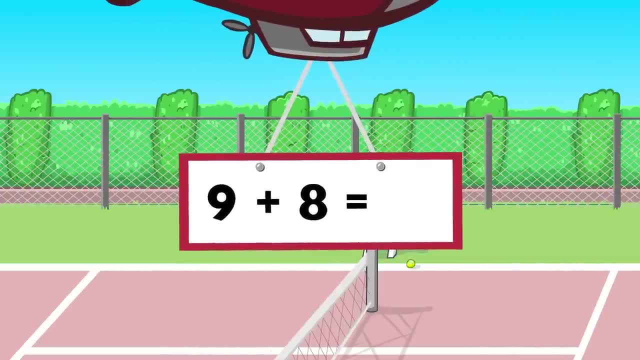 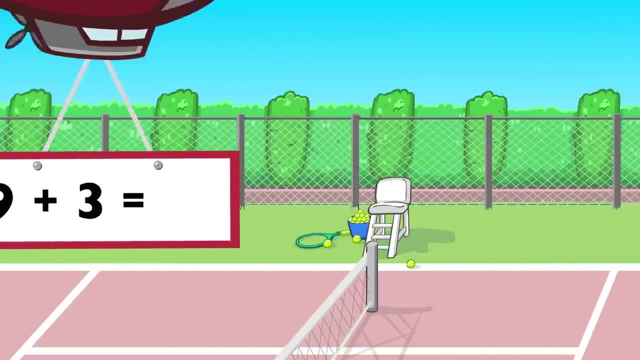 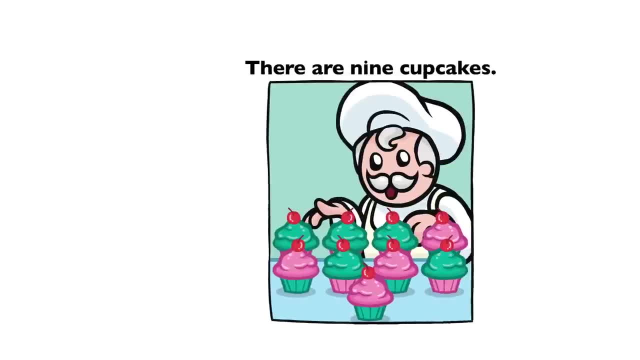 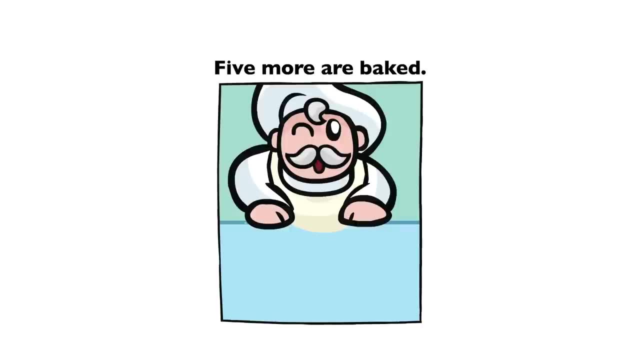 9. 12., 9. 12.. There are 9 cupcakes, 5 more are baked. Now there are 14 cupcakes, 9 plus 5 equals 9., 9., 9. 9.. 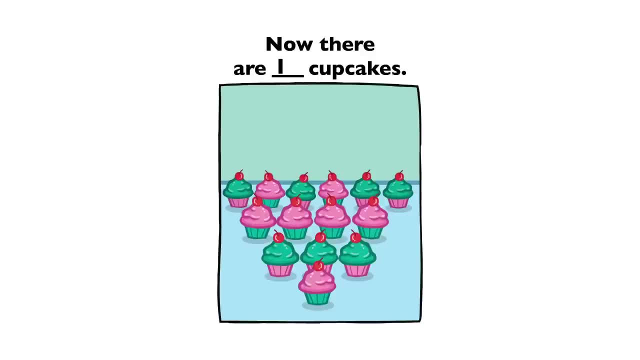 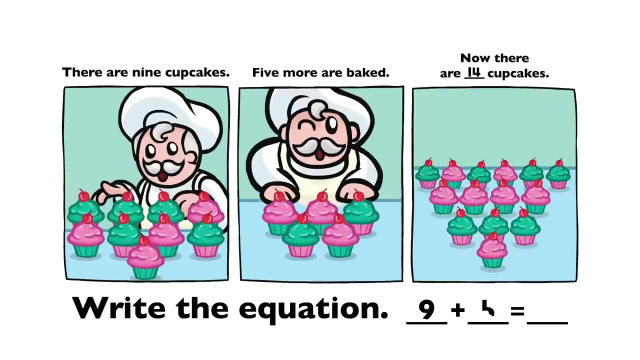 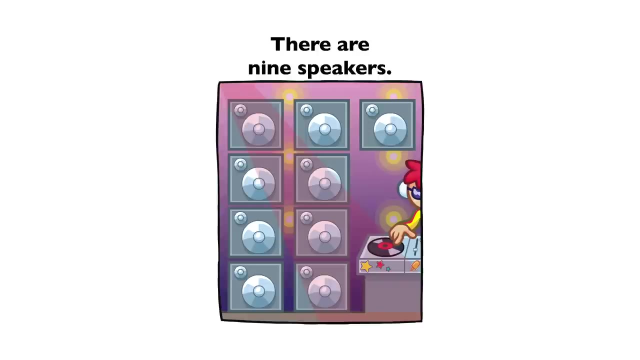 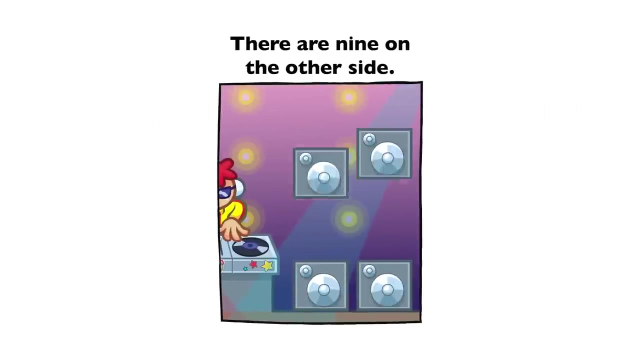 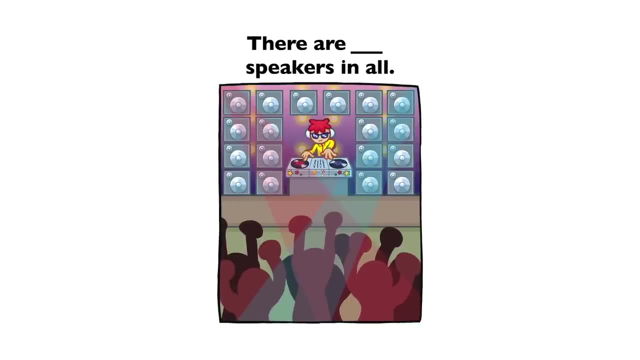 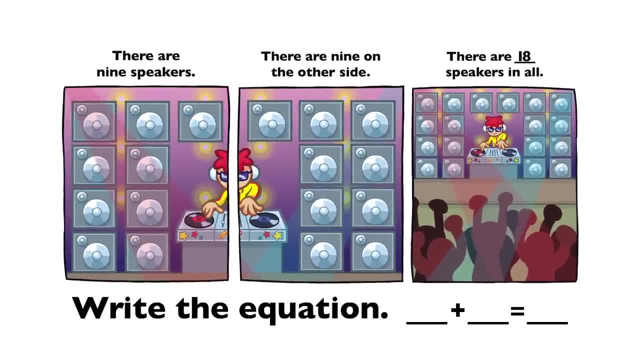 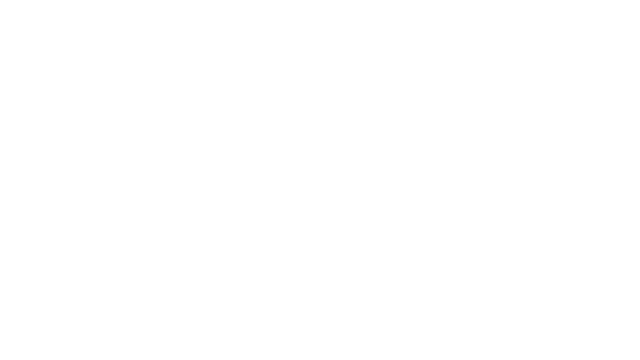 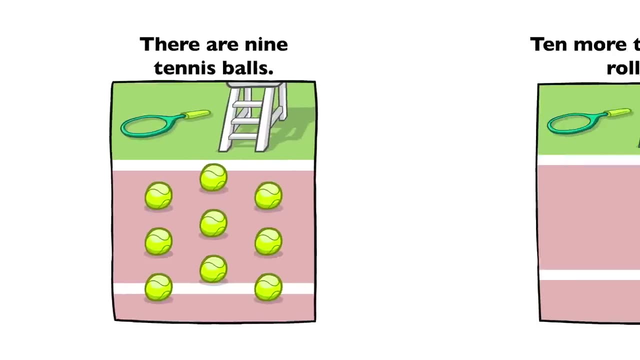 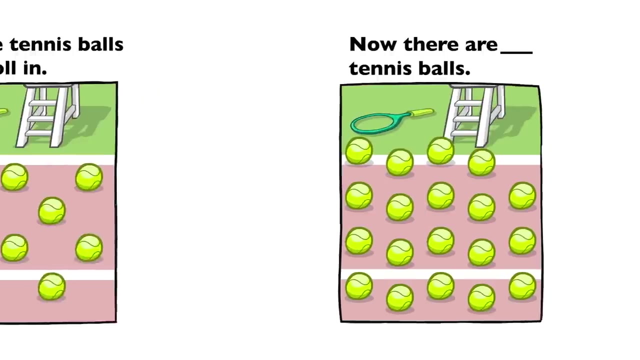 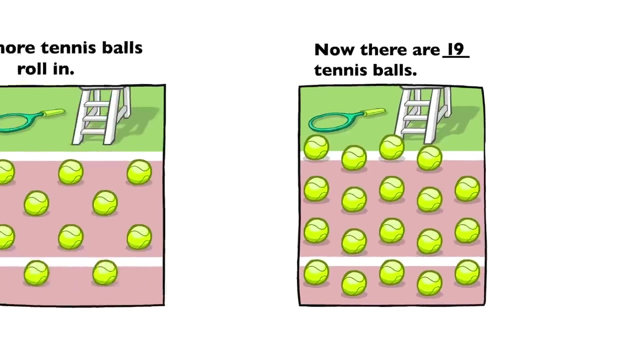 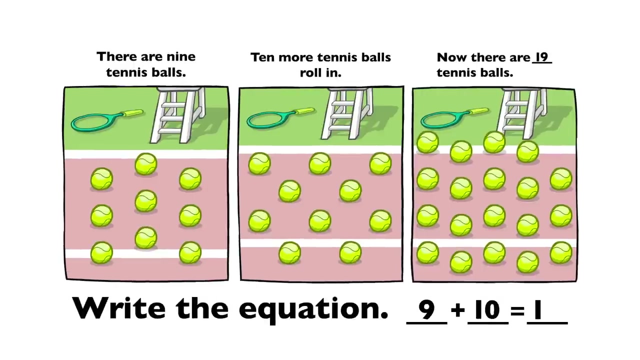 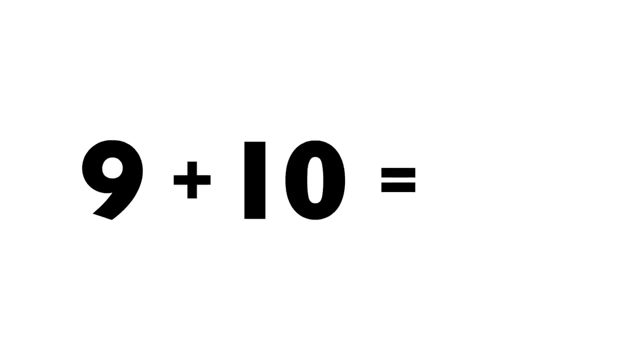 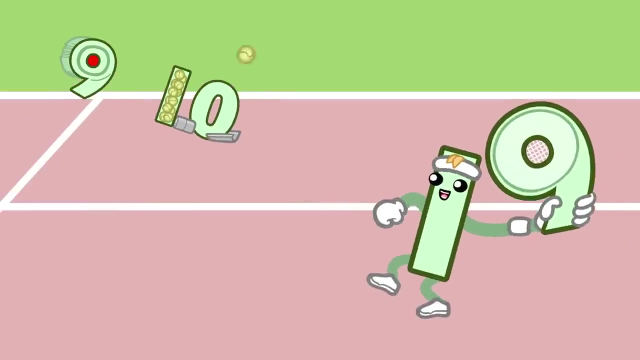 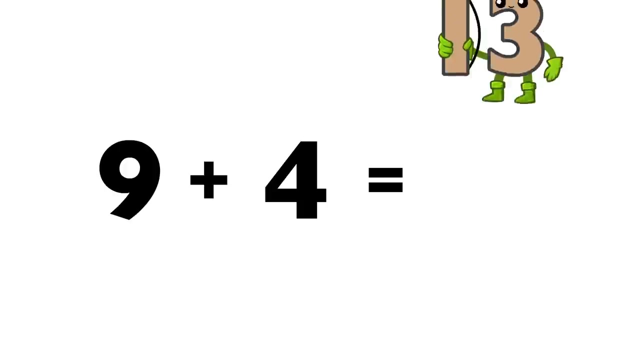 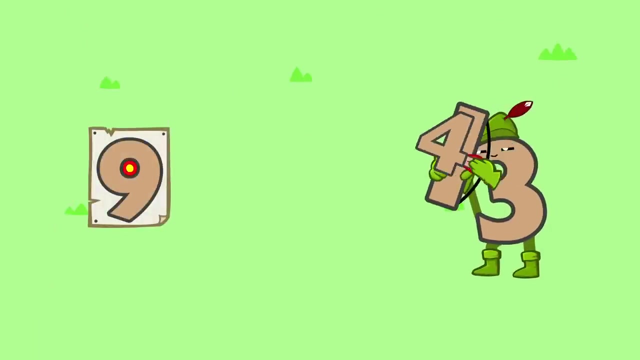 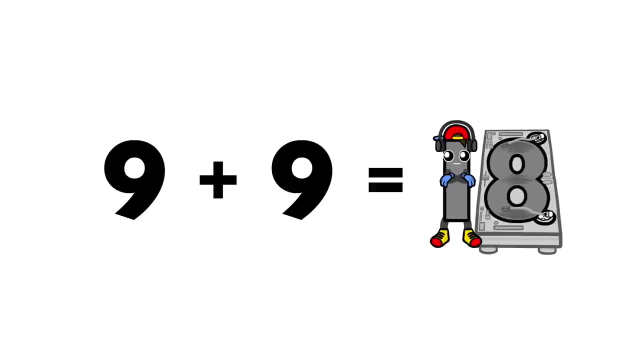 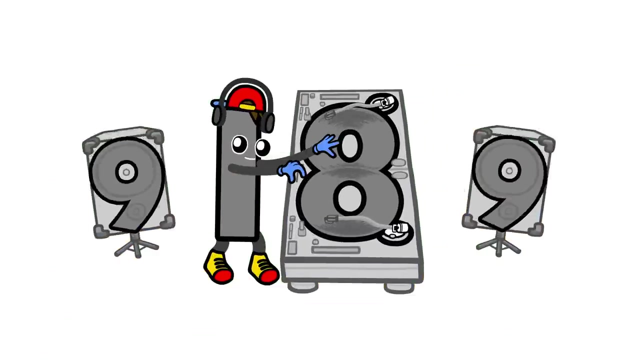 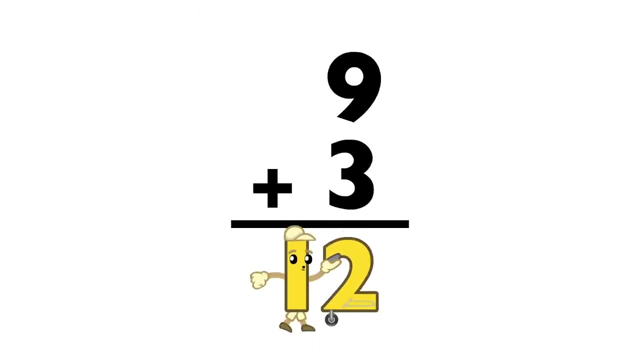 speakers. in all, nine plus nine equals eighteen. there are nine tennis balls. ten more tennis balls roll in now. there are nineteen tennis balls. nine plus ten equals nineteen. nine plus ten equals nineteen. nine plus four equals 19 tennis balls: 13. nine plus nine equals eighteen. nine plus three equals 12. 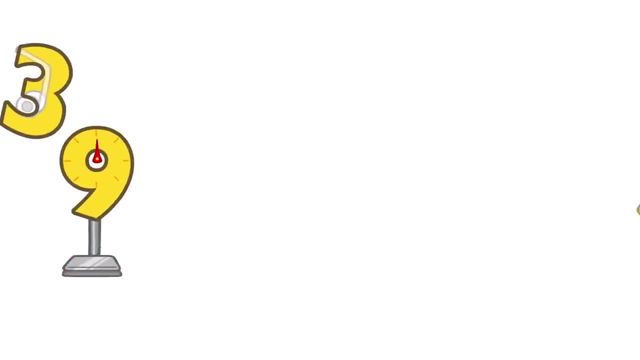 13, 14, 15, 16, 17, 18, 19, 20, 21, 22, 23, 24, 25, 26, 27, 28, 29, 30, 31, 32, 33, 33, 34, 35, 36, 36. 37, 38, 39, 40, 41, 42, 43, 44, 45, 46, 46, 47, 48, 49, 51, 52, 53, 53, 54, 53, 53, 53, 54, 56, 55, 56. 56, 56, 56, 56, 57, 56, 57, 58, 58, 59, 59, 51, 52, 53, 52, 53, 53, 54, 53, 54, 55, 56, 56, 57, 58, 59. 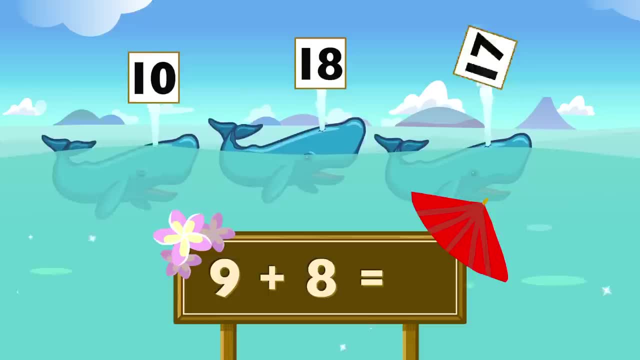 51, 52, 53, 53, 54, 53, 53, 54, 55, 56, 56, 57, 58, 59, 60, 61, 62, 62, 63, 63, 64, 65, 66, 67, 68, 69. 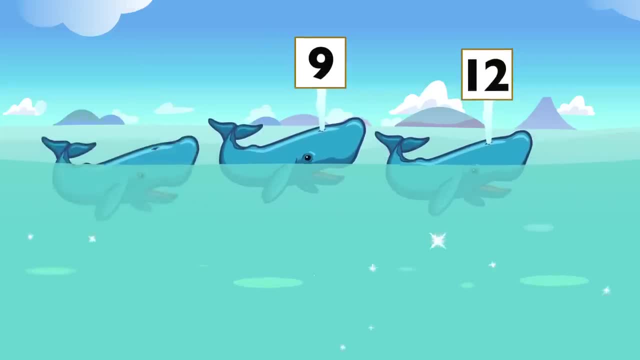 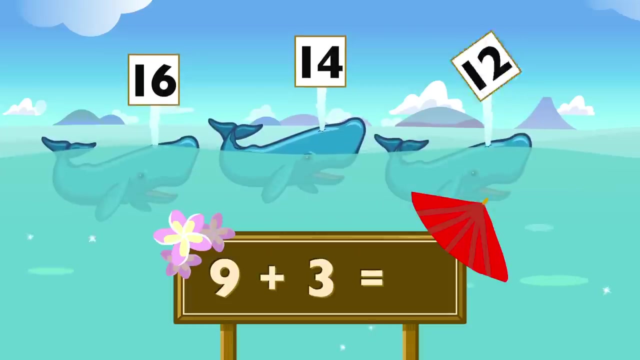 69, 70, 71, 72, 73, 74, 75, 76, 77, 78, 79, 80, 81, 82, 83, 84, 85, 86, 87, 88, 89, 90, 91, 92, 93, 92. 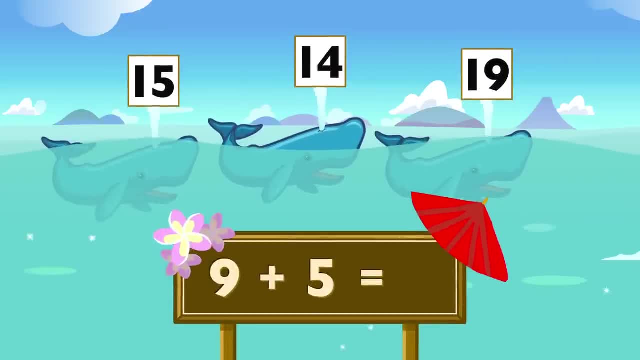 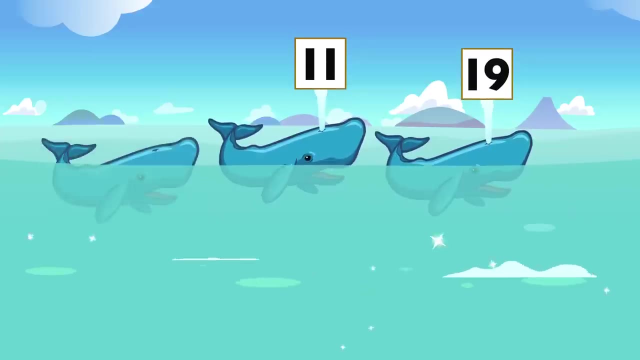 93, 94, 95, 96, 97, 98, 99, 100, 100, 100, 12, 22, 23, 23, 24, 25, 26, 27, 28, 29, 30, 31, 32, 33, 33, 33. 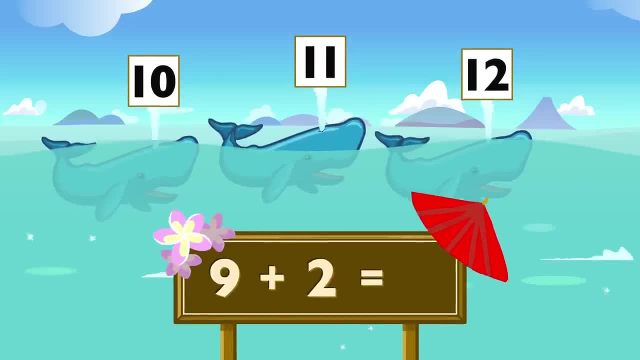 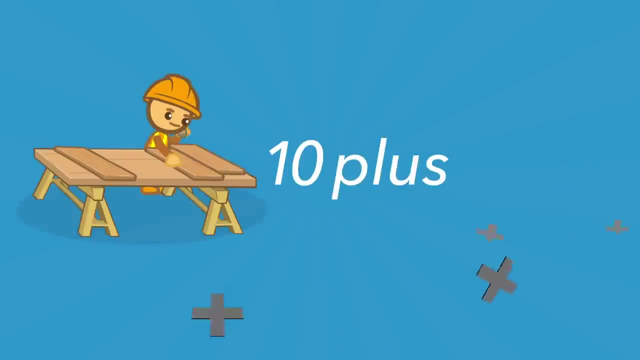 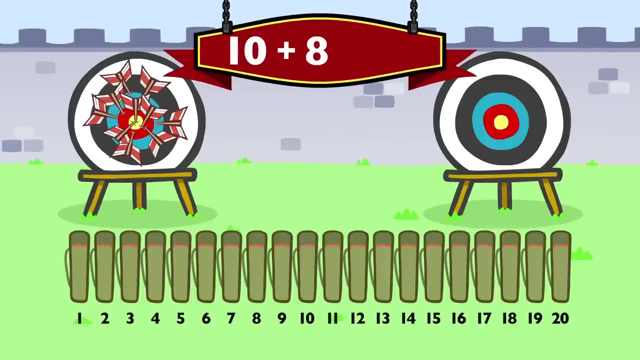 34: 35 equals 11. 10 Plus 8 equals 18. 10 plus 8 equals 18. 10. 10 Plus 6 equals 16. 10 plus 6 equals 16. 10. 10 Plus 0 equals 10. 10 plus 0: equals 10. 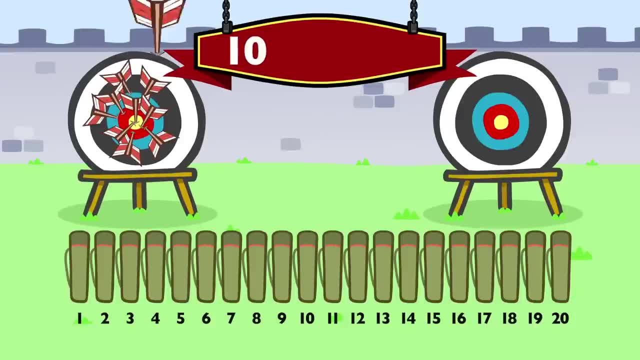 10 Plus 9 Equals 19. 10 plus 9 equals 19. 10, 10 plus 7 equals 17.. 10 plus 7 equals 17.. 10 plus 1 equals 11.. 10 plus 1 equals 11.. 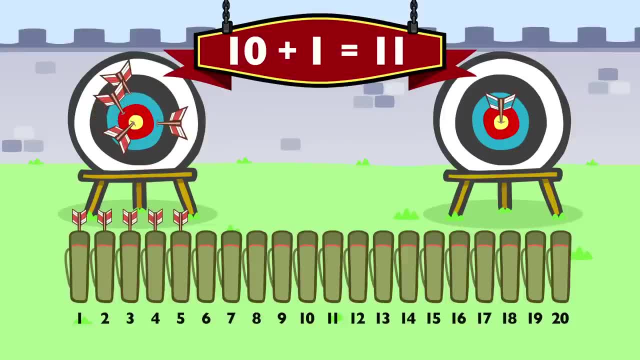 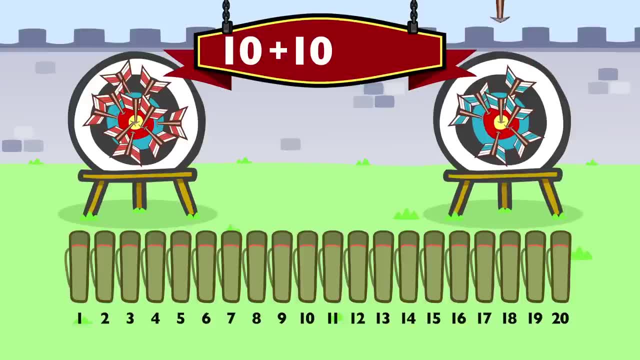 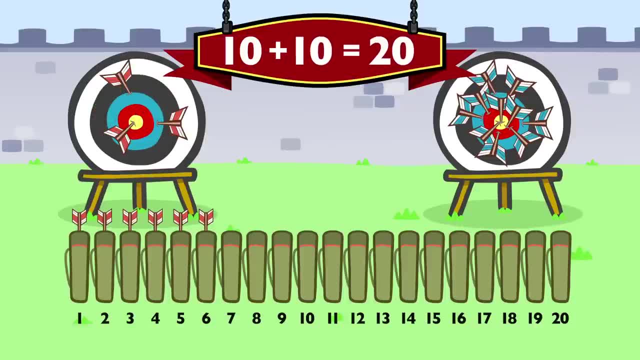 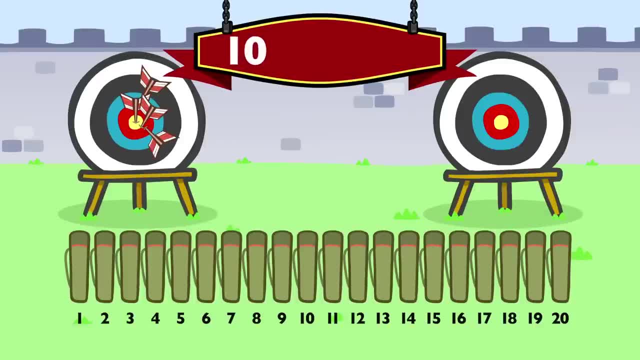 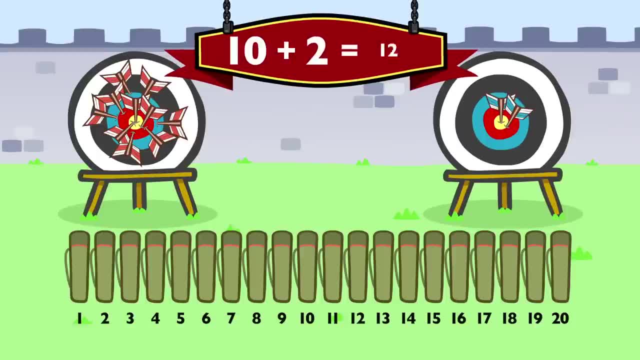 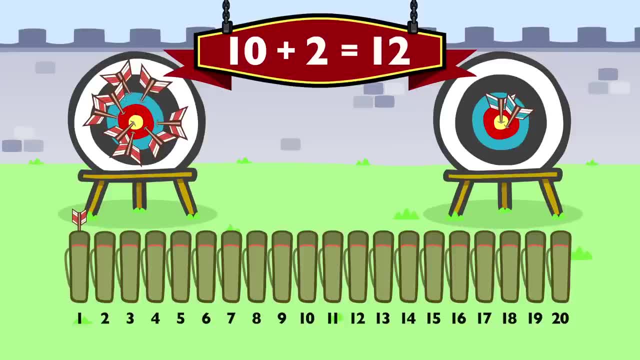 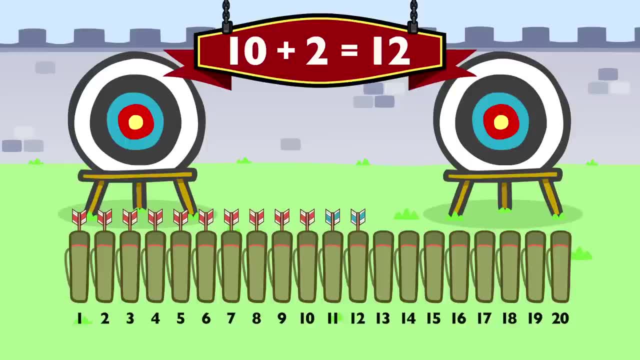 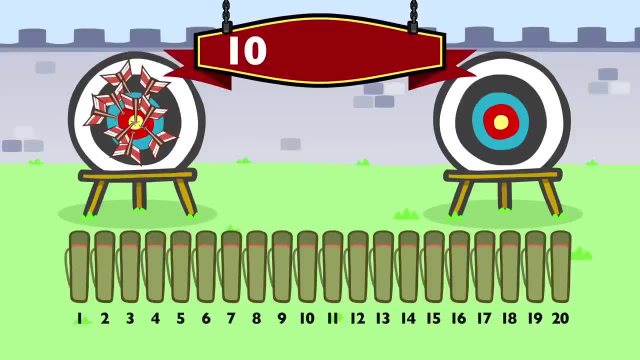 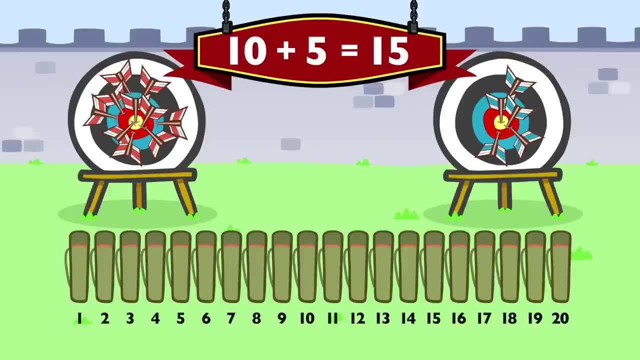 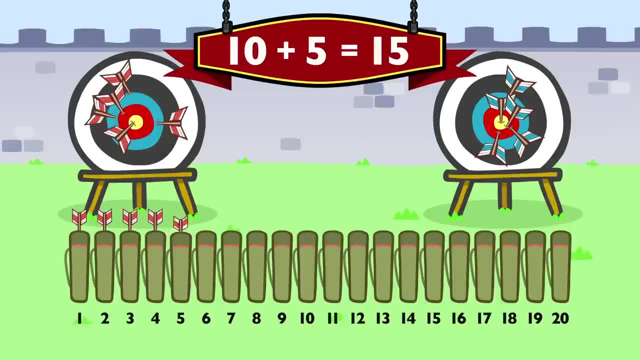 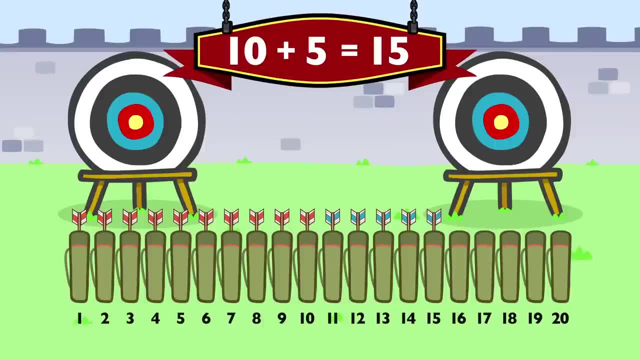 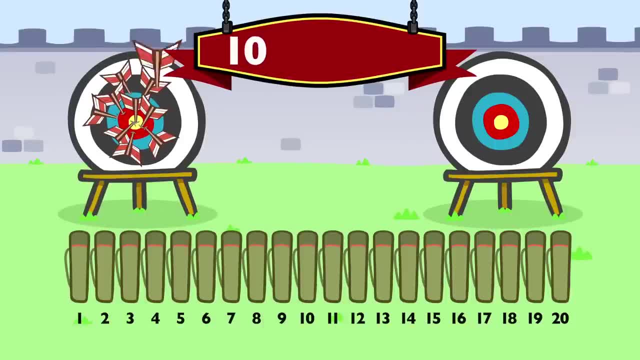 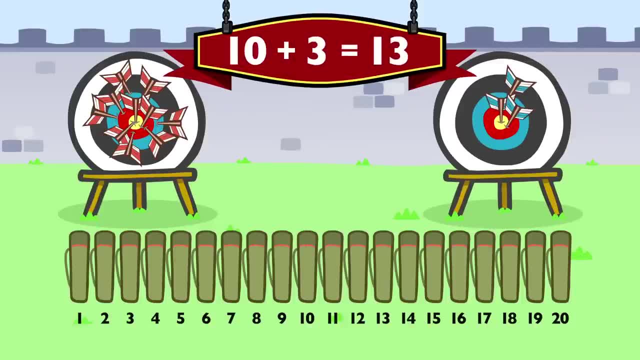 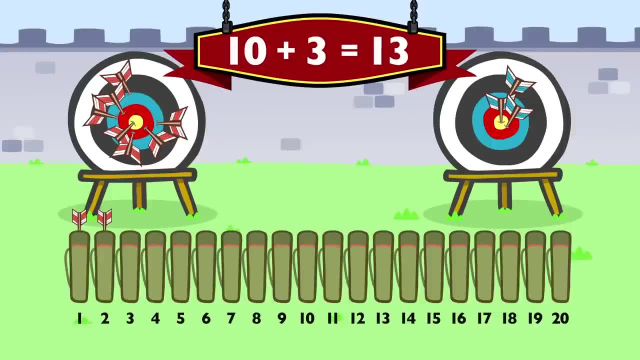 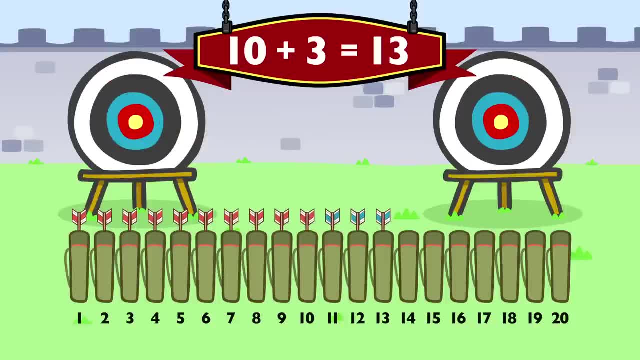 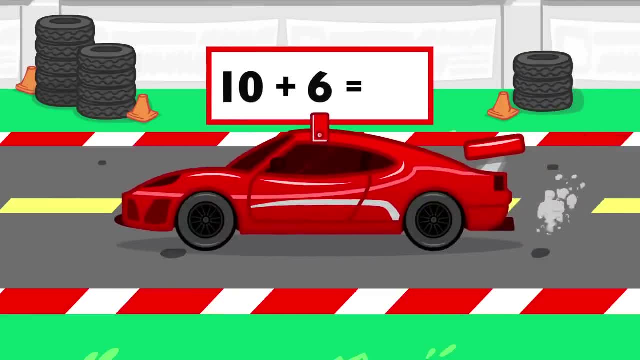 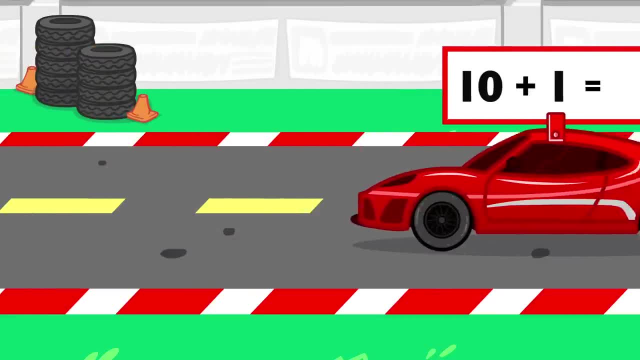 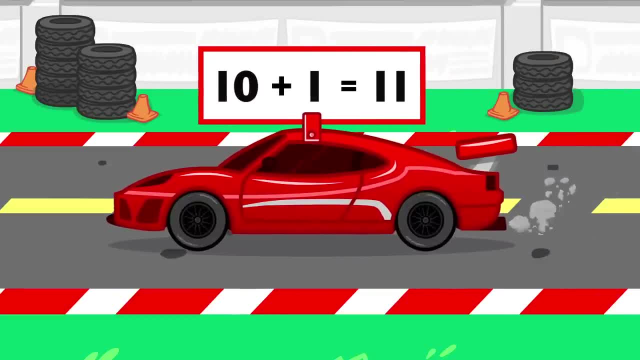 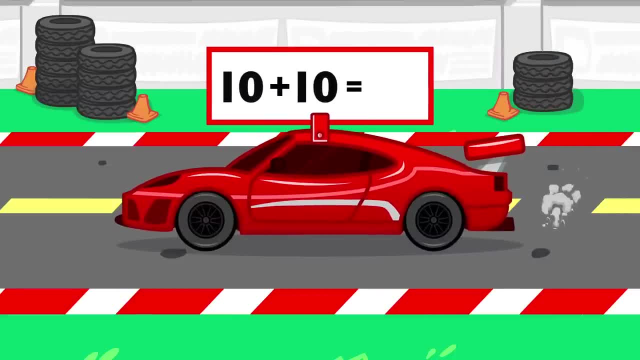 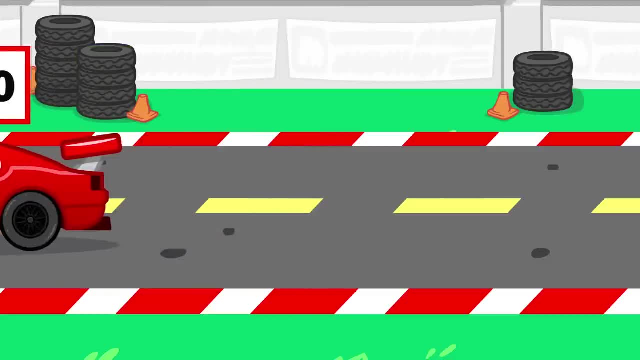 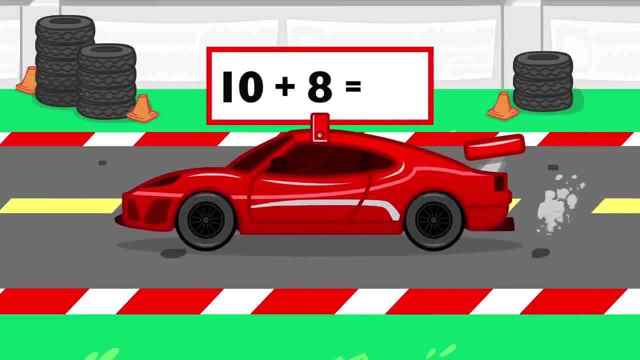 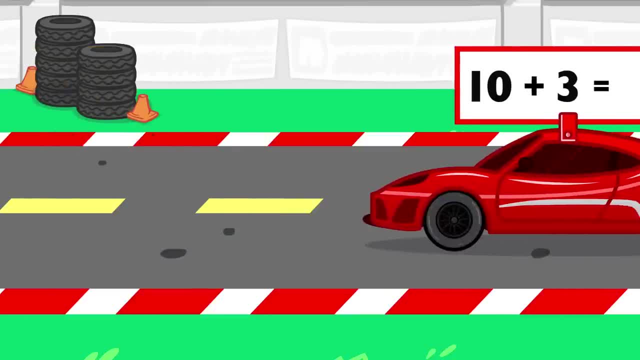 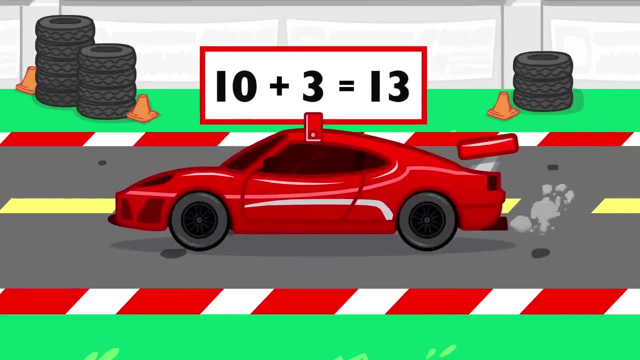 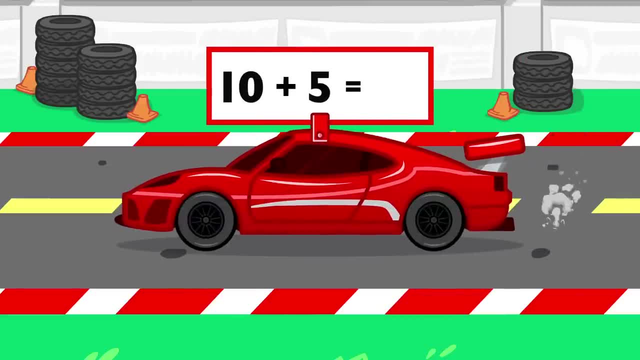 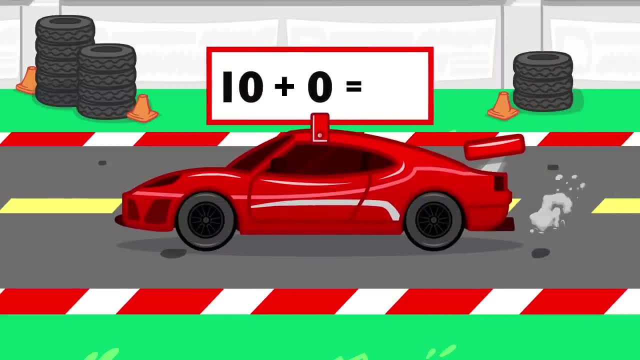 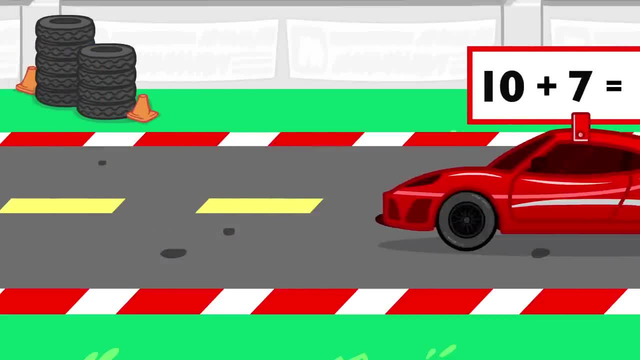 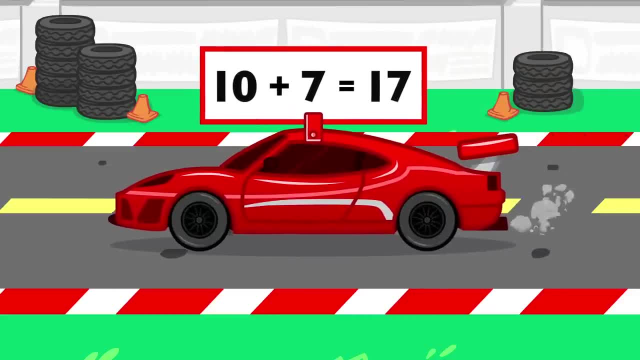 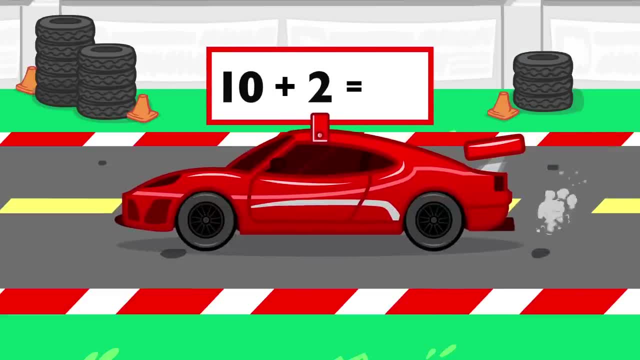 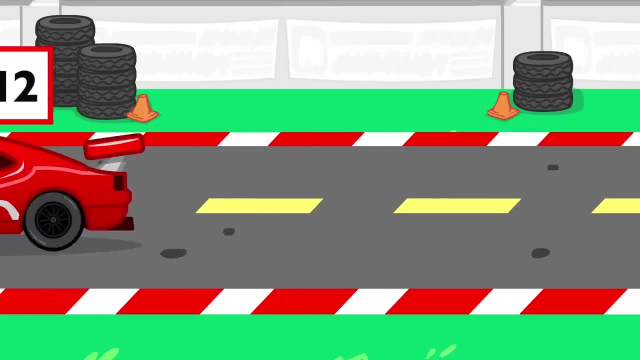 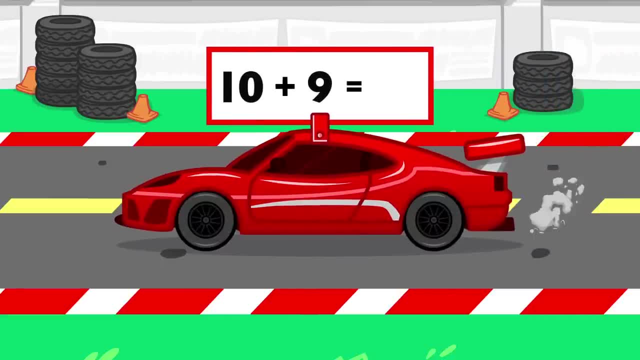 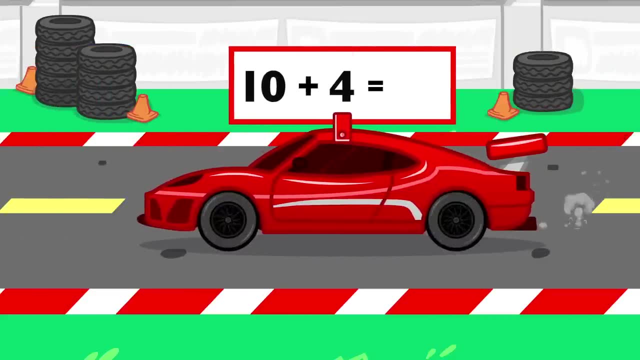 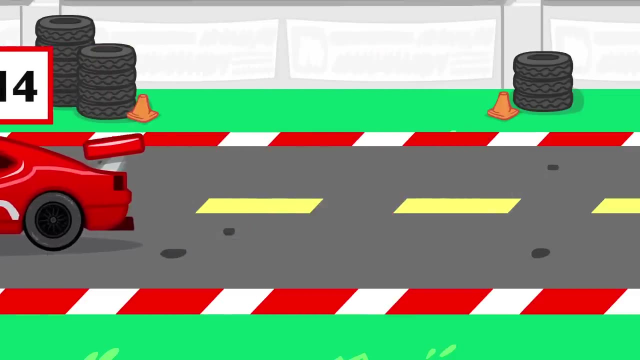 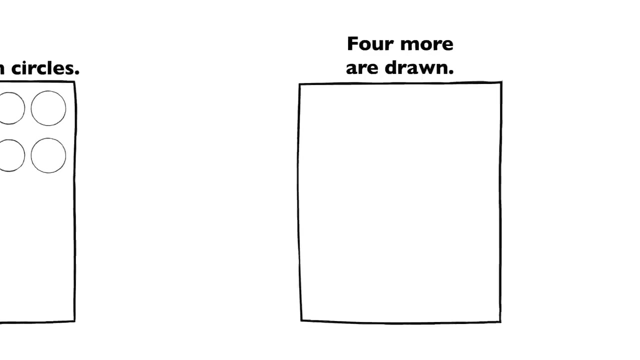 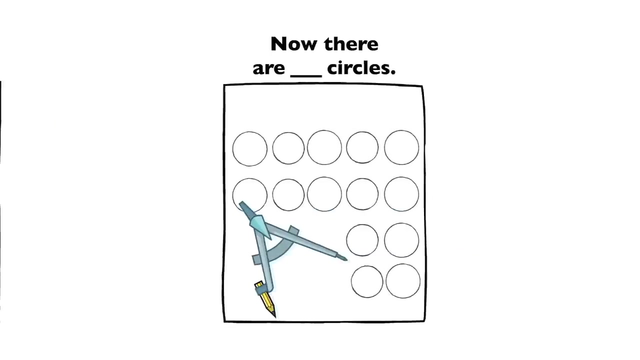 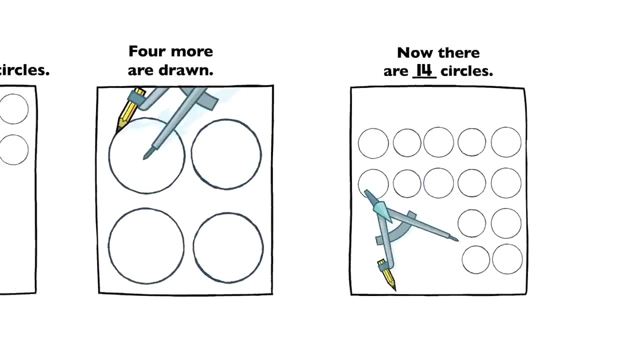 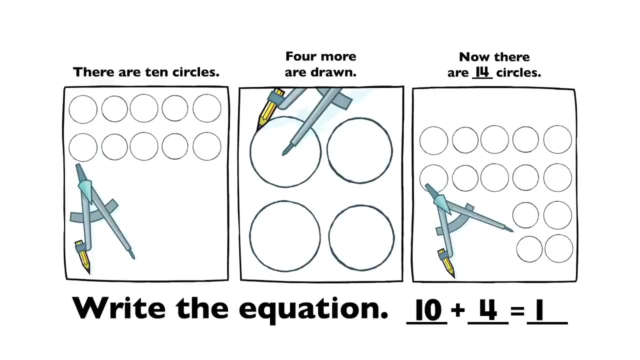 10 plus 0 equals 10.. 10 plus 0 equals 10.. 9 equals 19. 10 plus 4 equals 14. There are 10 circles. 4 more are drawn Now there are fourteen circles. Ten plus four equals fourteen. 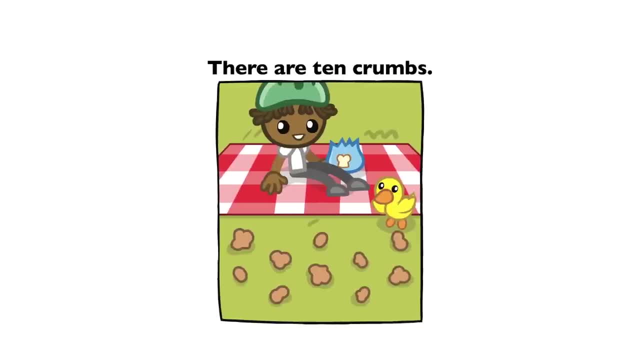 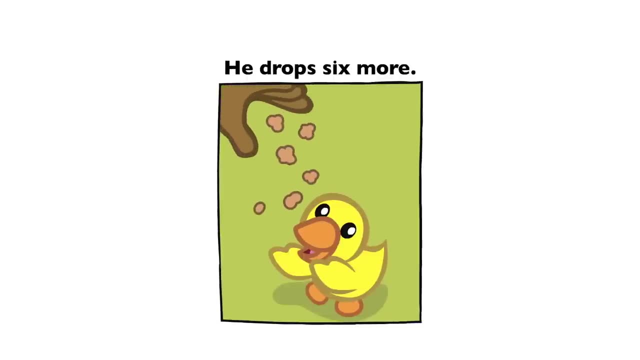 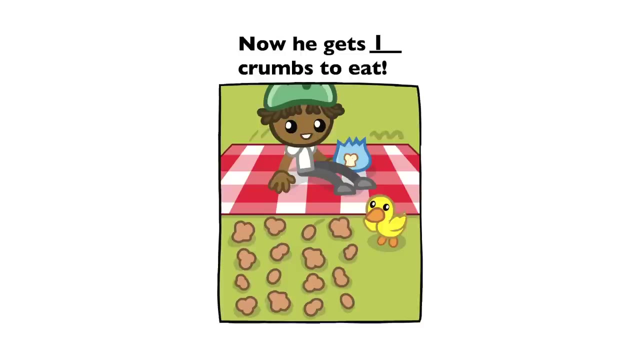 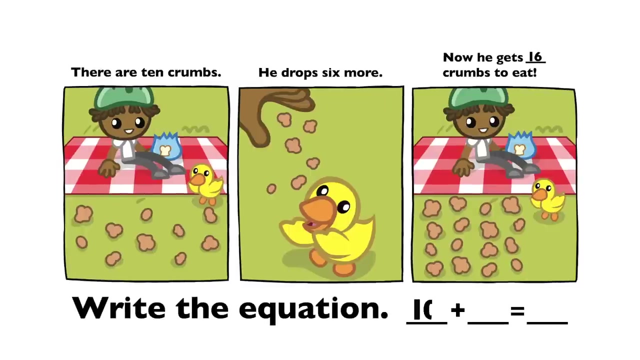 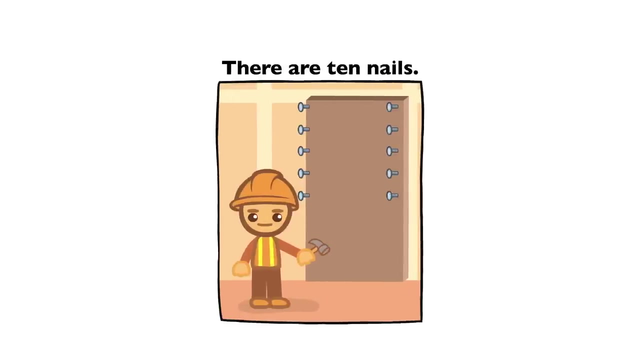 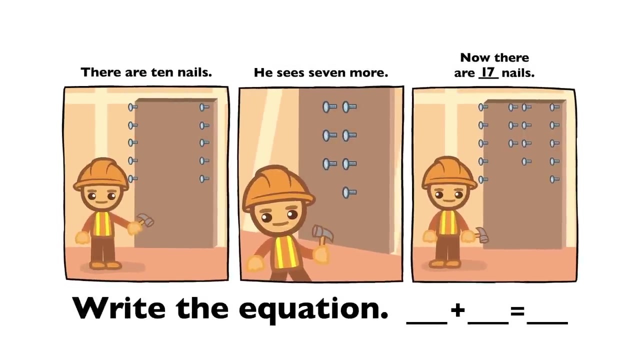 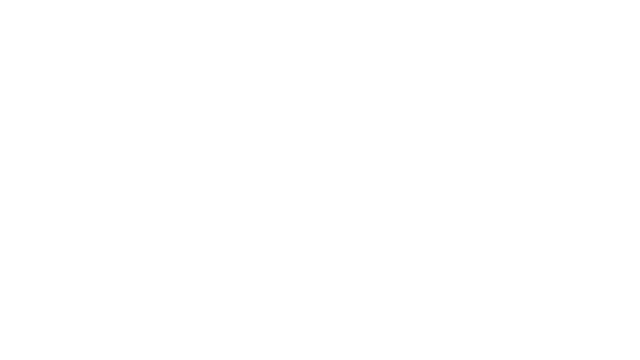 There are ten crumbs, He drops six more. Now he gets sixteen crumbs to eat. Ten plus six equals sixteen. There are ten nails. He sees seven more. Now there are seventeen nails. Ten plus seven equals seventeen. Ten plus ten equals twenty. 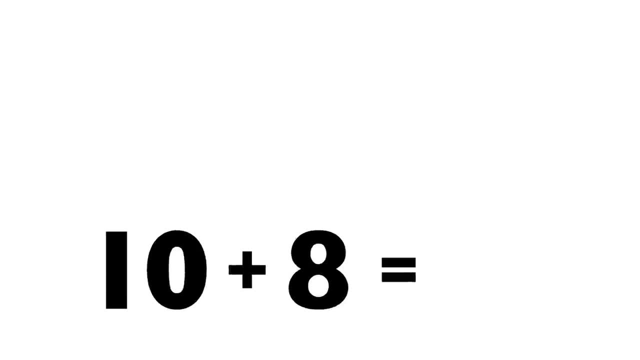 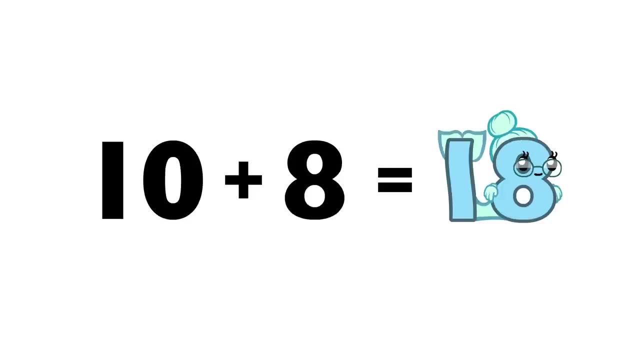 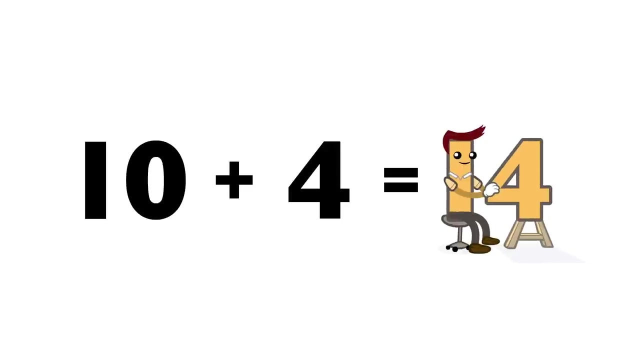 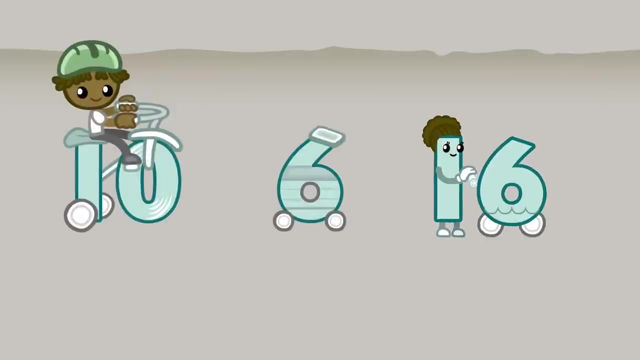 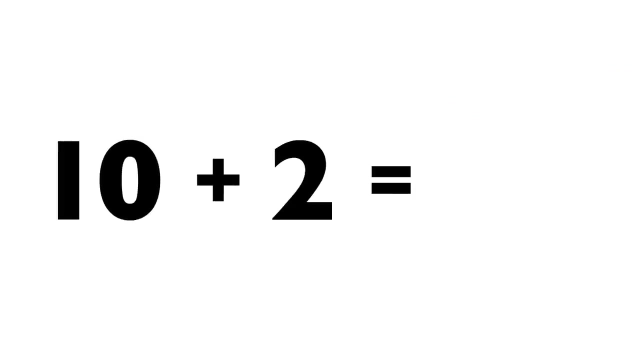 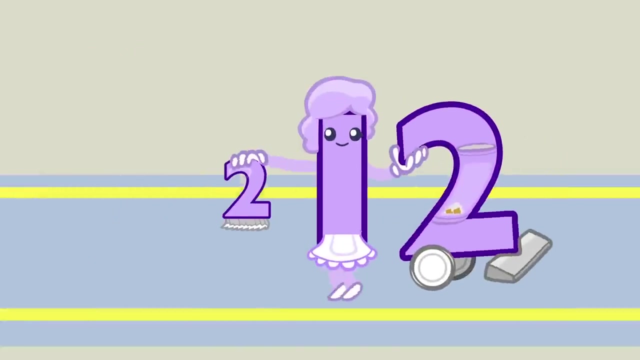 Ten plus ten equals twenty. Ten plus eight equals eighteen. Ten plus ten equals twenty. Ten plus four equals fourteen. Ten plus six equals sixteen. Ten plus six equals sixteen. Ten plus two equals twelve. Ten plus two equals twelve. Ten plus two, equals fifteen. 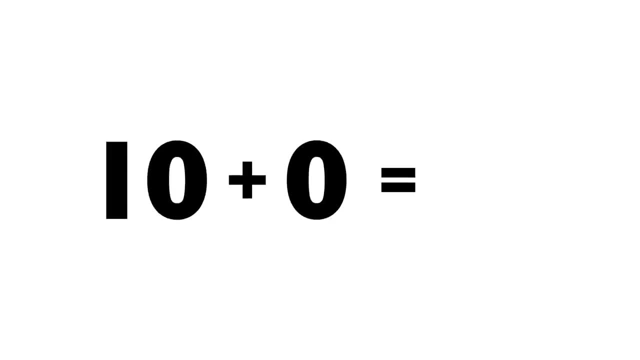 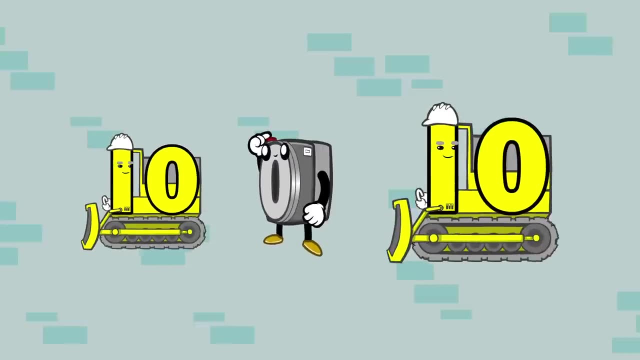 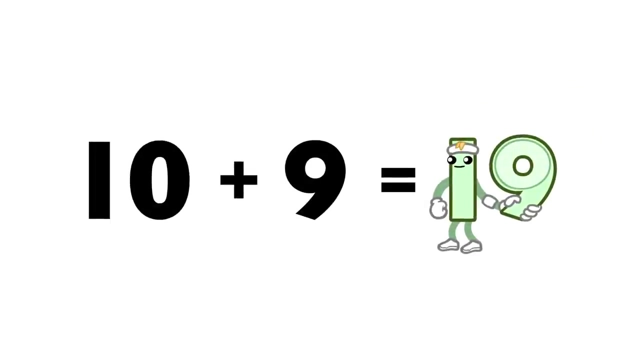 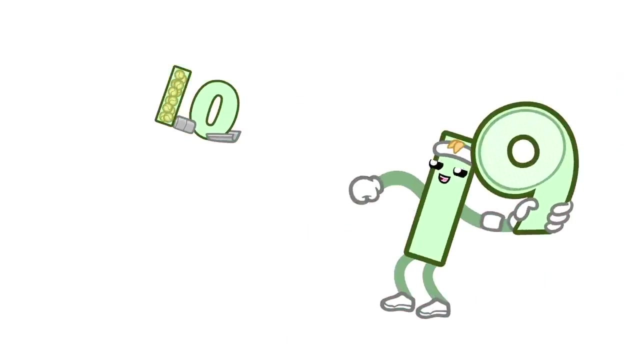 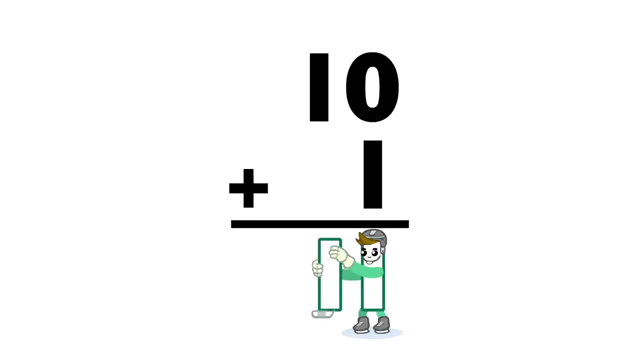 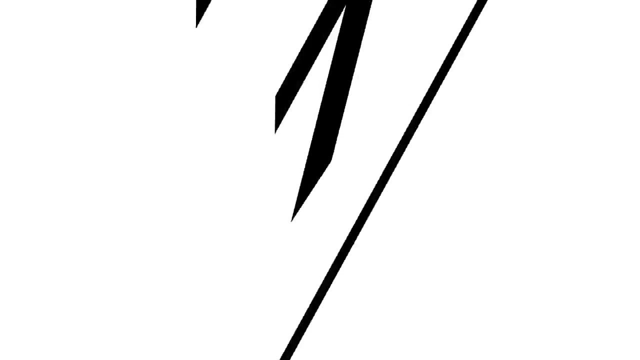 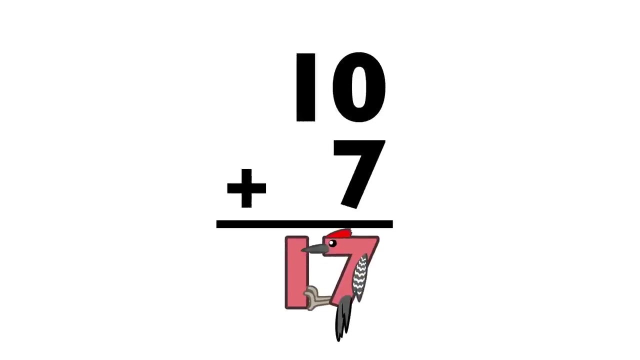 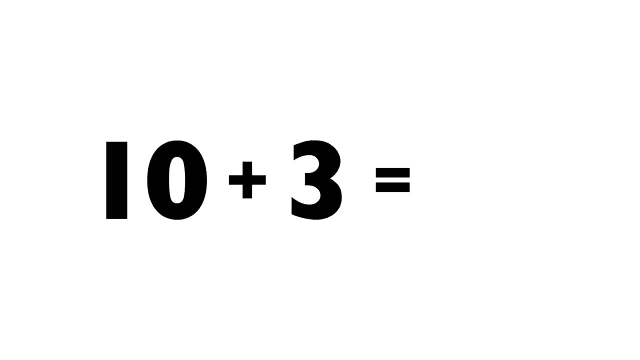 Ten plus zero equals ten. Ten plus four equals. ten Ten plus nine equals nineteen. 10 plus 1 equals 11.. 10 plus 7 equals 17.. 10 plus 3 equals 13.. 10 plus 5 equals 15.. 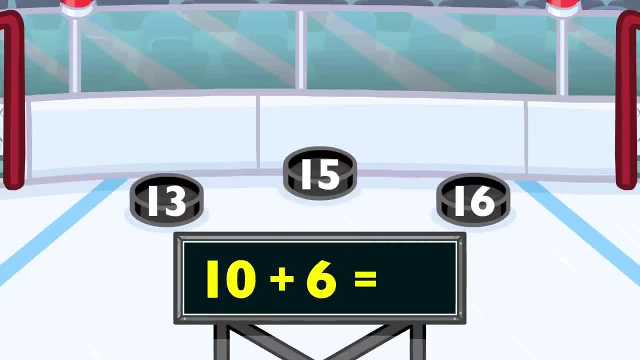 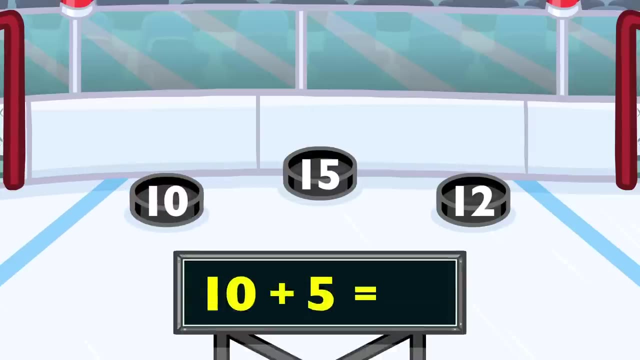 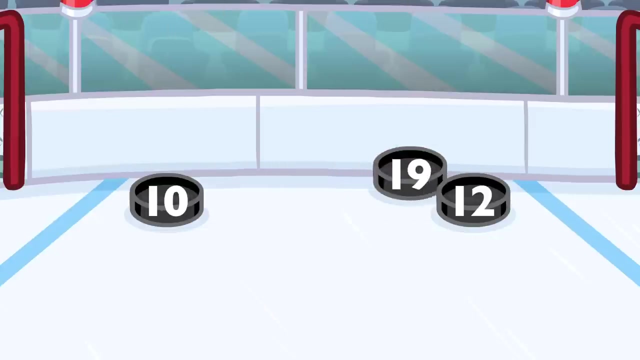 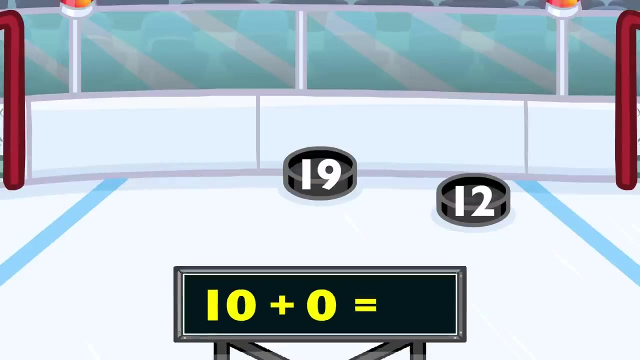 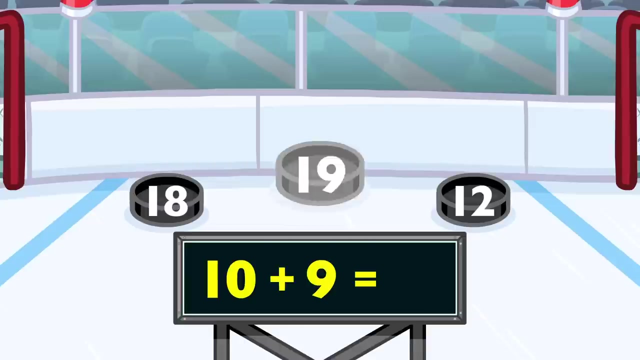 10 plus 6 equals 16.. 10 plus 3 equals 13.. 10 plus 5 equals 15.. 10 plus 0 equals 10.. 10 plus 9 equals 19.. 10 plus 2 equals. 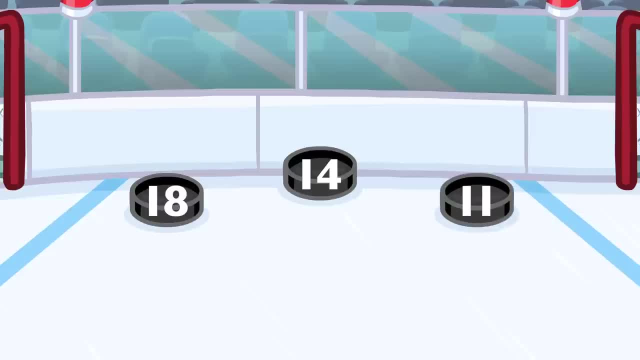 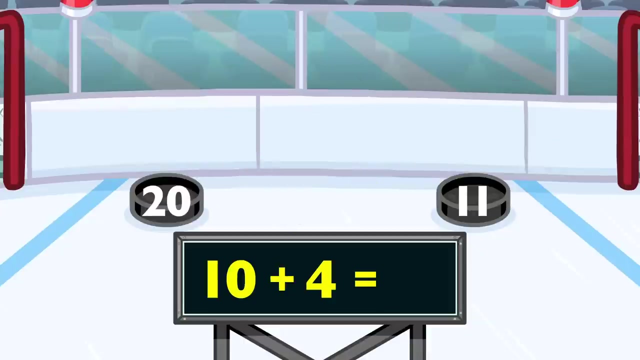 12. 10 plus 8 equals 18.. 10 plus 4 equals 14.. 10 plus 10 equals 20.. 10 plus 1 equals 11.. 10 plus 7 equals 17.. 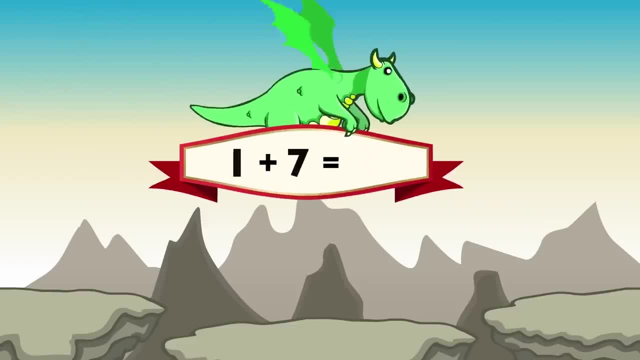 1 plus 7 equals 8.. 2 plus 4 equals 6.. 3 plus 3 equals 6.. 1 plus 2 equals 3.. 3 plus 5 equals 8.. 4 plus 4 equals. 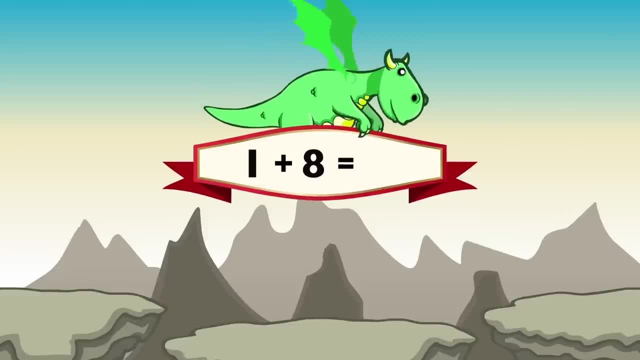 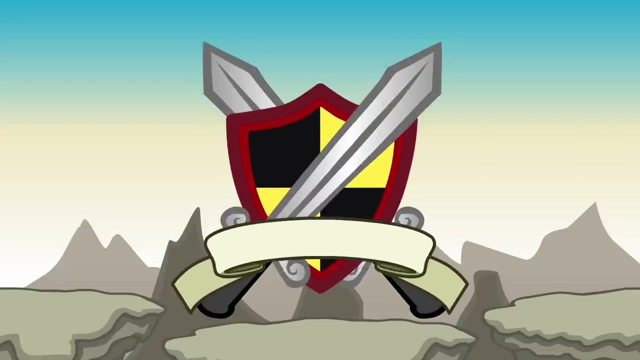 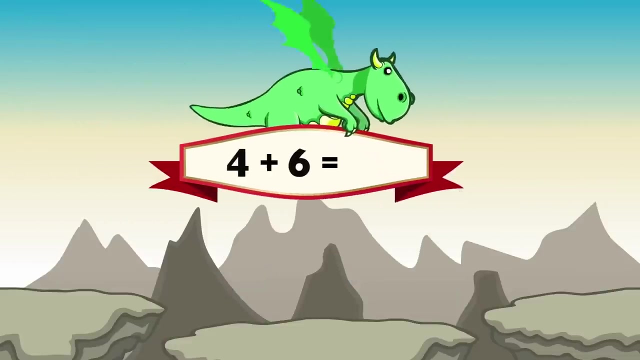 8. 1 plus 8 equals 9. 4 plus 7 equals 11. 3 plus 8 equals 11. 11. 4 plus 6 equals 10. 3 plus 6 equals. 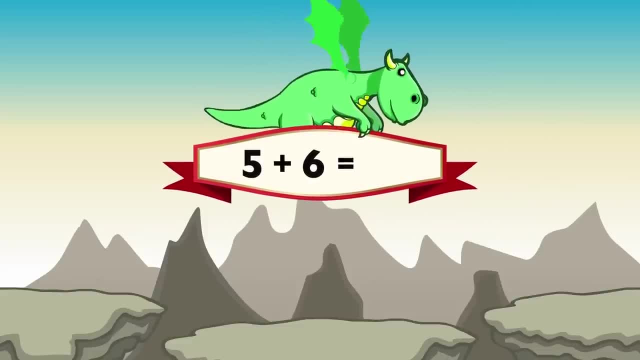 9. 5 plus 6 equals 11.. 4 plus 9 equals 13.. 8 plus 8 equals 16.. 6 plus 7 equals 13.. 5 plus 10 equals 15.. 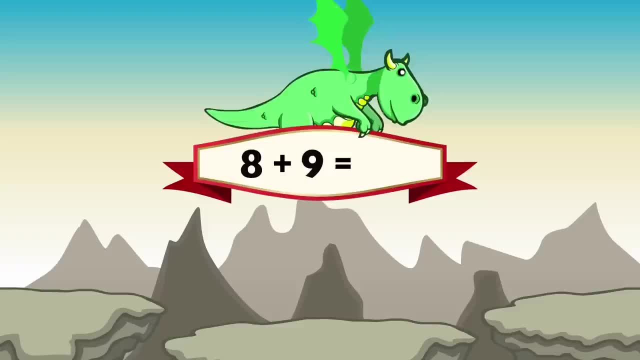 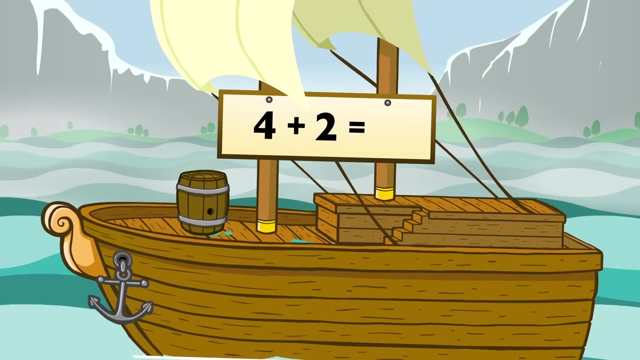 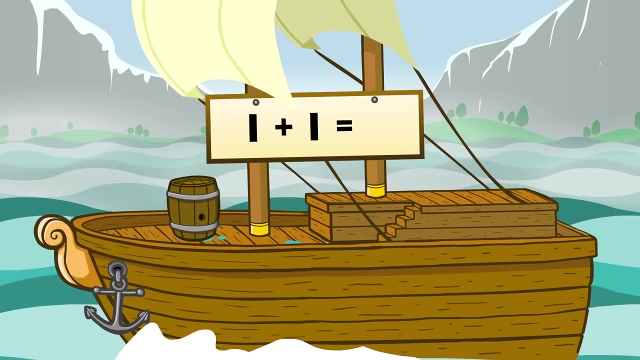 8 plus 9 equals 17.. 5 plus 8 equals 13.. 8 plus 7 equals 15.. 4 plus 2 equals 6.. 1 plus 1 equals 2.. 2 plus 2 equals. 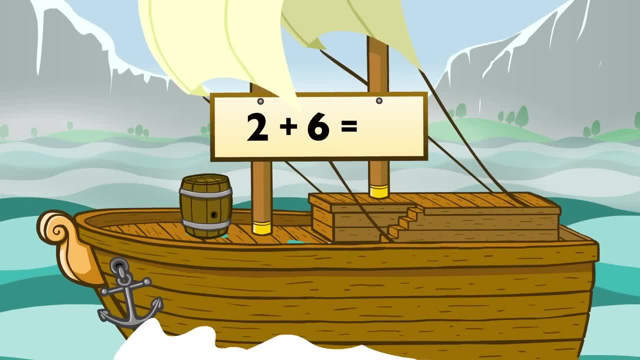 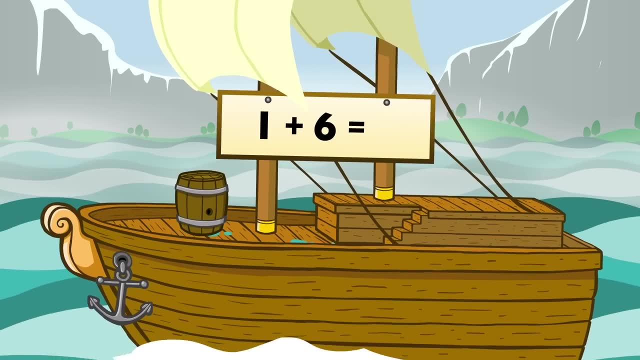 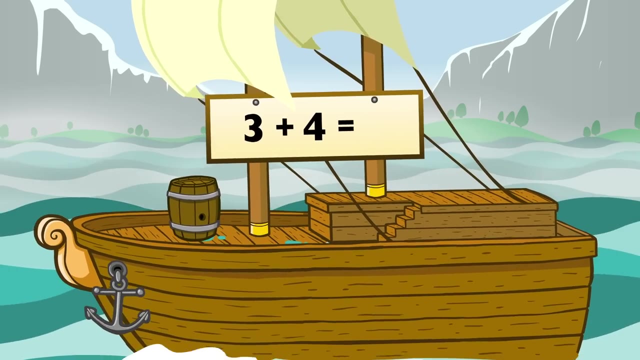 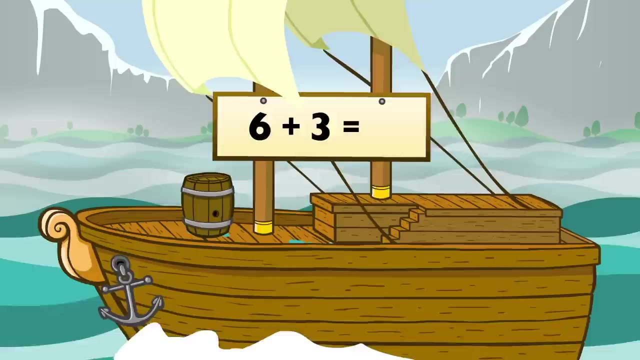 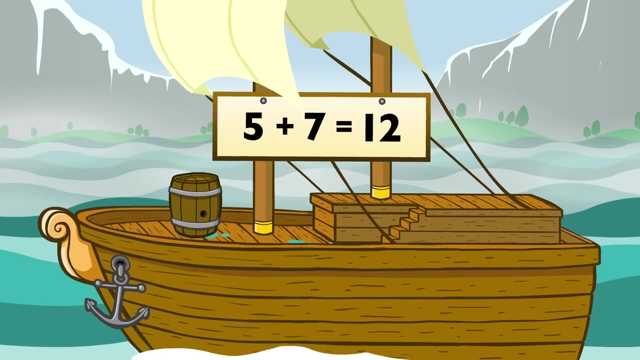 4. 2 plus 6 equals 8.. 1 plus 6 equals 7.. 3 plus 4 equals 7.. 6 plus 3 equals 9.. 5 plus 7 equals 12.. 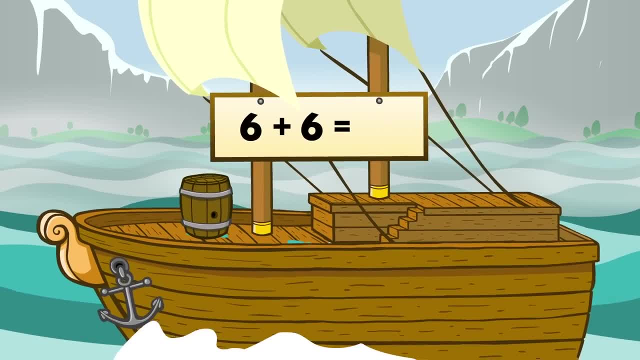 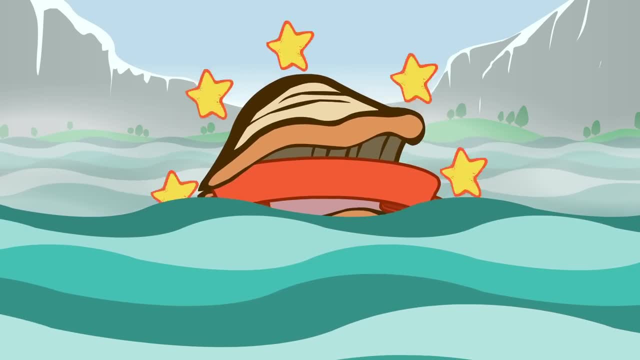 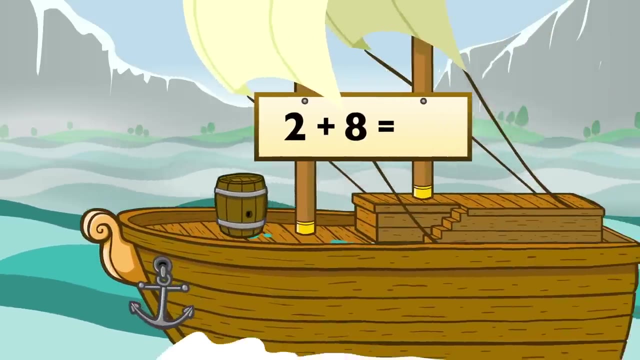 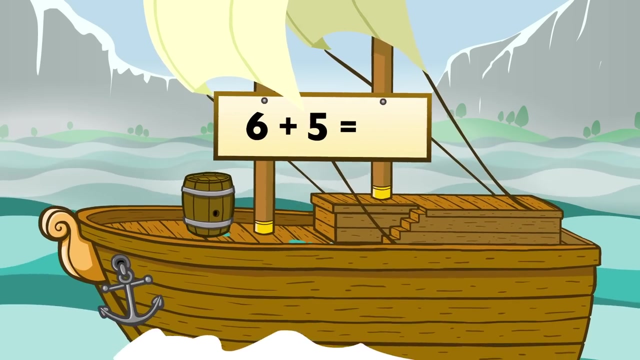 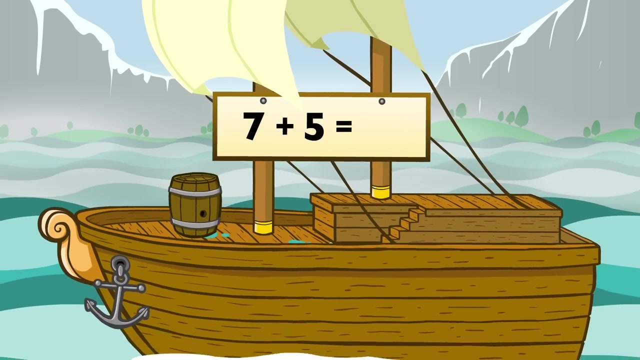 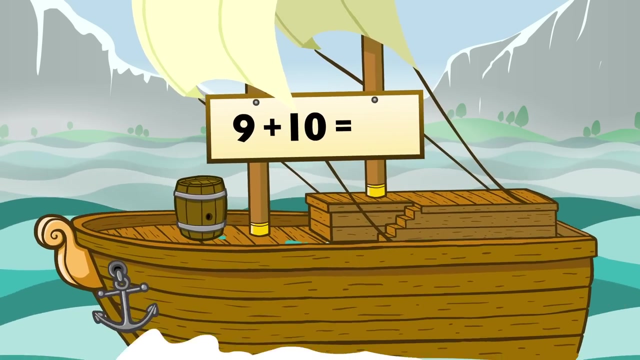 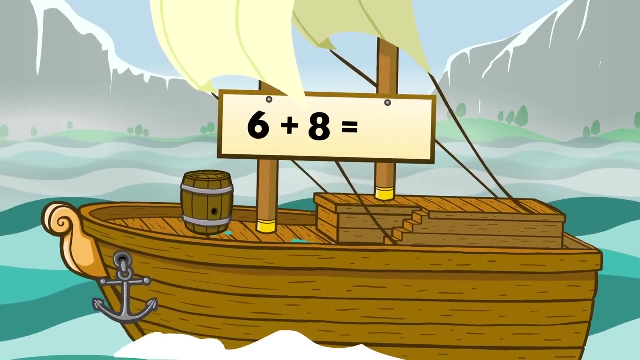 6 plus 6 equals 12.. 2 plus 8 equals 10.. 6 plus 5 equals 11.. 7 plus 5 equals 12.. 9 plus 10 equals 19.. 6 plus 8 equals. 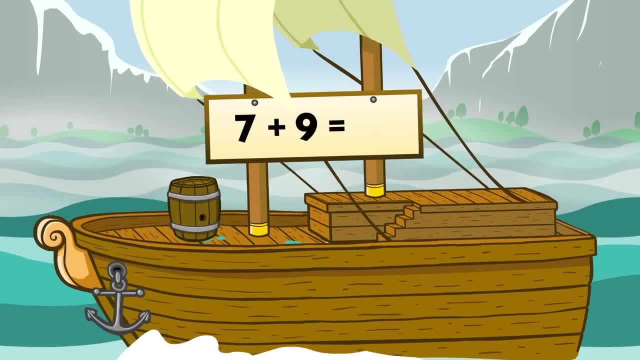 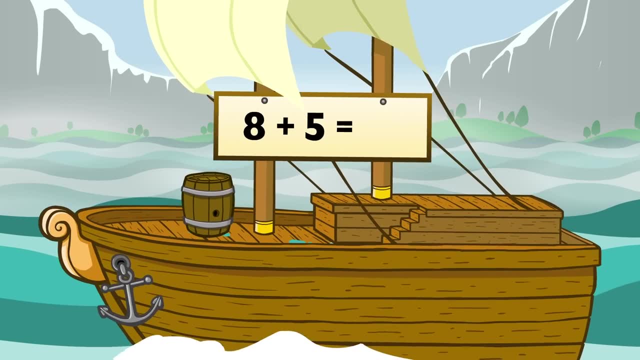 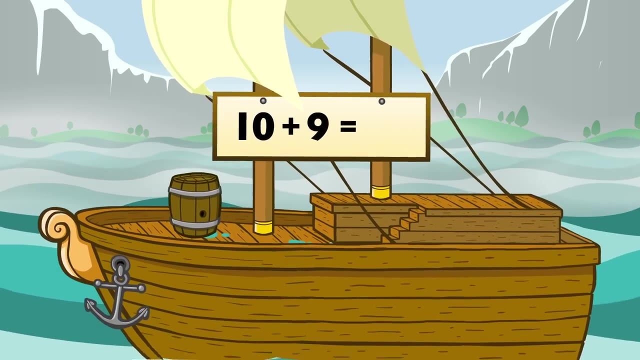 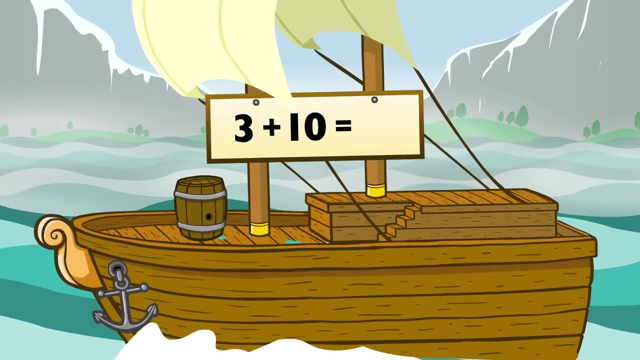 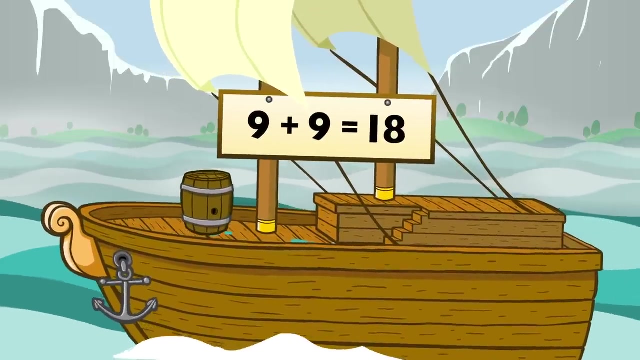 14.. 7 plus 9 equals 16.. 8 plus 5 equals 13.. 10 plus 9 equals 19.. 3 plus 10 equals 13.. 9 plus 9 equals 18.. 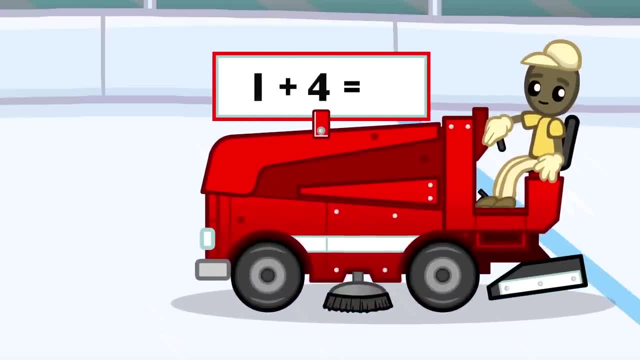 1 plus 4 equals 5.. 7 plus 1 equals 8.. 2 plus 9 equals 11.. 3 plus 7 equals 10.. 7 plus 8 equals 15.. 5 plus 9 equals. 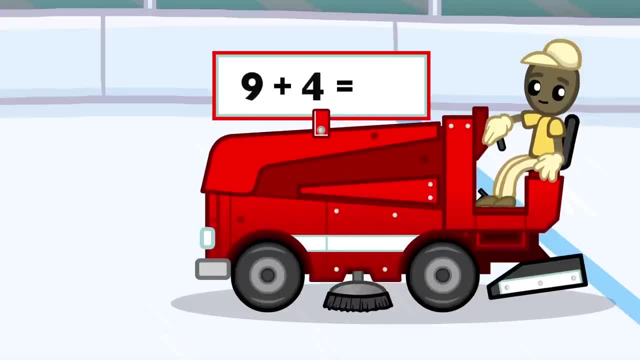 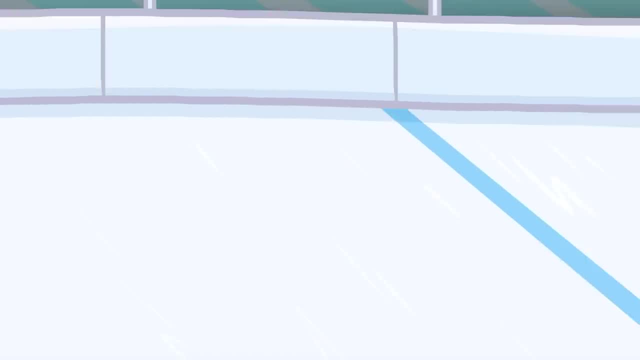 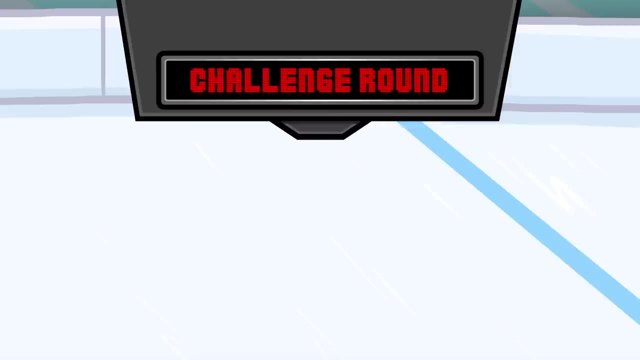 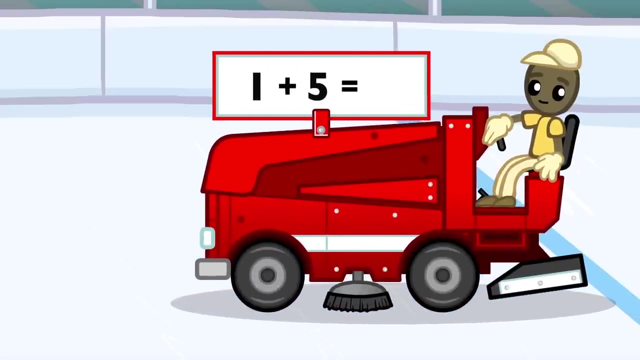 14.. 9 plus 4 equals 13.. 1 plus 5 equals 6.. 6 plus 2 equals 8.. 4 plus 5 equals 9.. 5 plus 5 equals 10.. 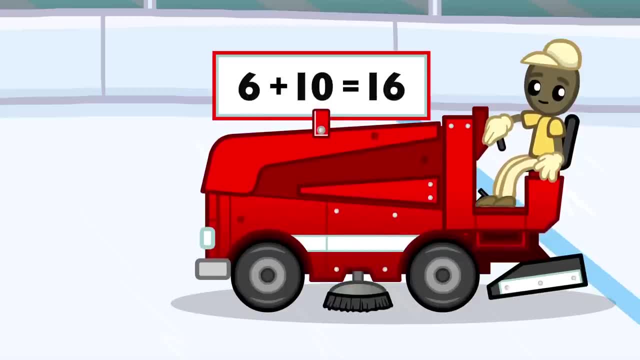 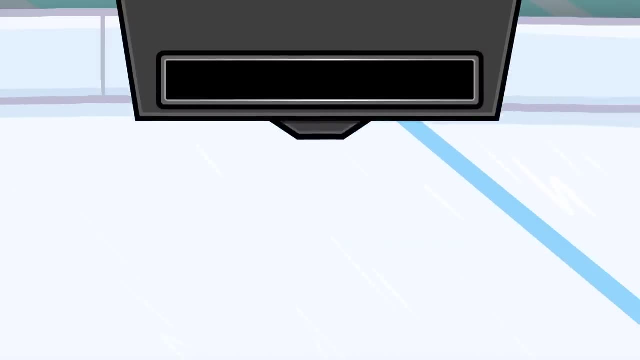 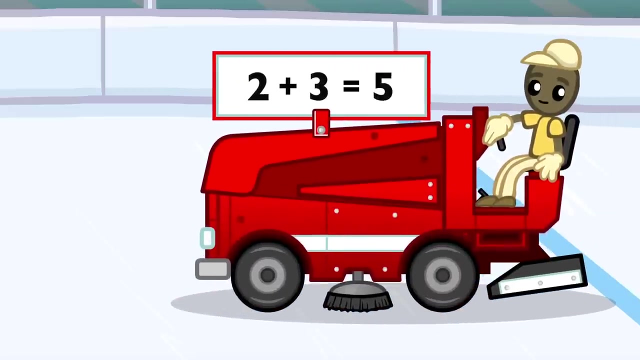 6 plus 10 equals 16.. 7 plus 10 equals 20.. 7 plus 10 equals 17. 17.. 2 plus 3 equals 5.. plus three equals eight. Eight plus one equals nine. 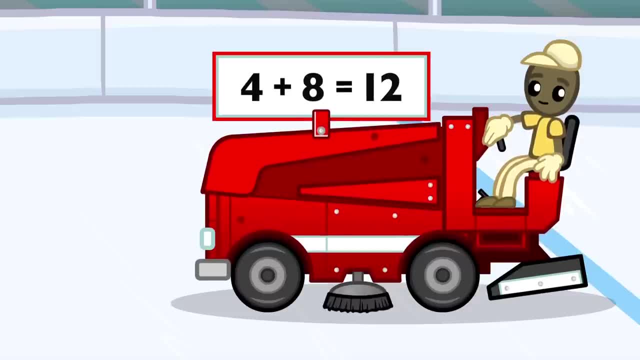 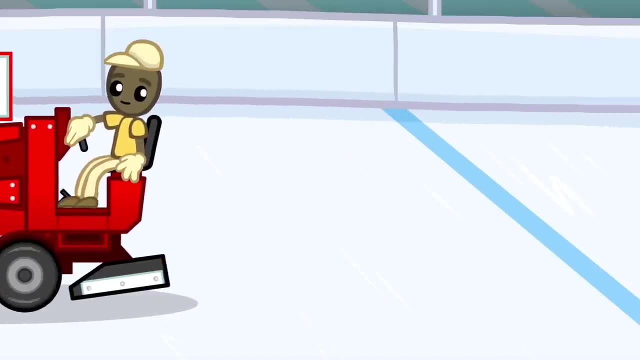 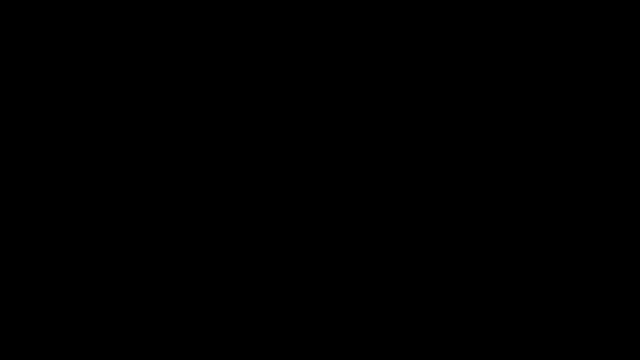 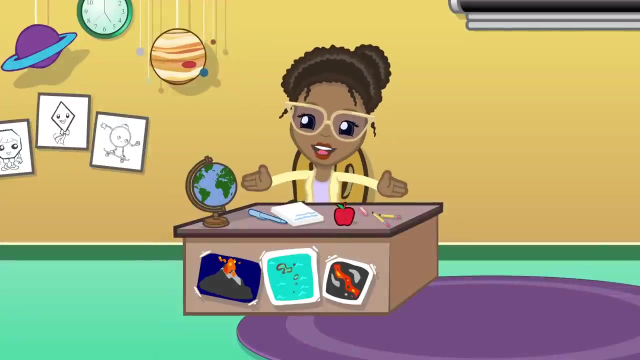 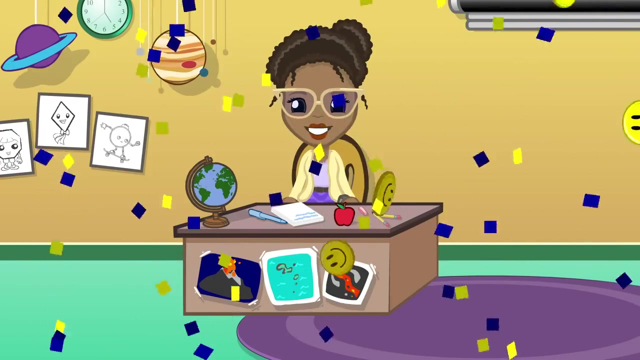 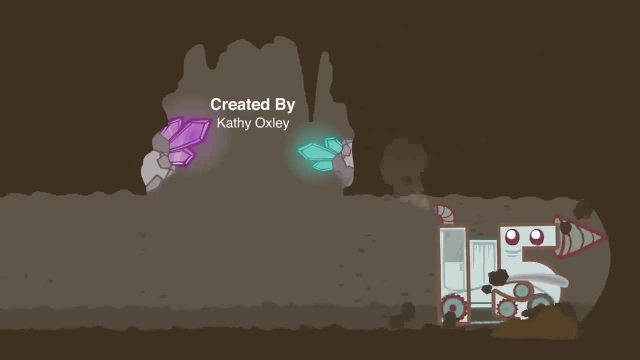 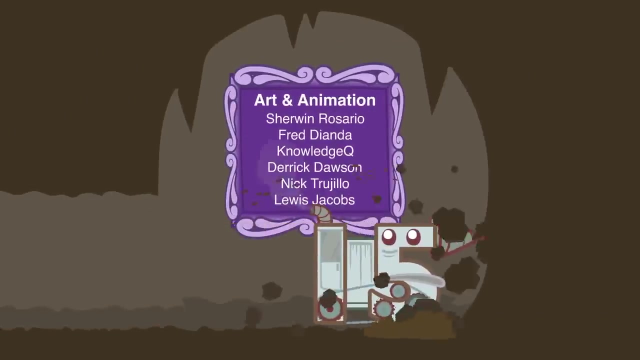 Four plus eight equals 12.. Nine plus eight equals 17.. 10 plus seven equals 17.. Nine plus five equals 14.. Oh hi, It looks like you have made it to the end. Congratulations, and keep practicing. Thank you.